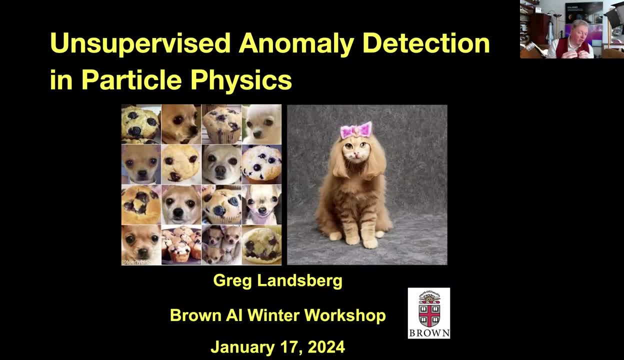 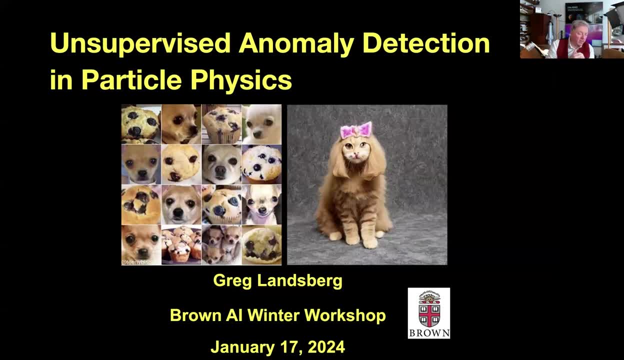 We're going to be using that to really help you run the demonstrations. It uses Google's remote servers for free and it's very easy to use, but it does require you to have a valid Google email – sorry, a valid Google account, Please make. 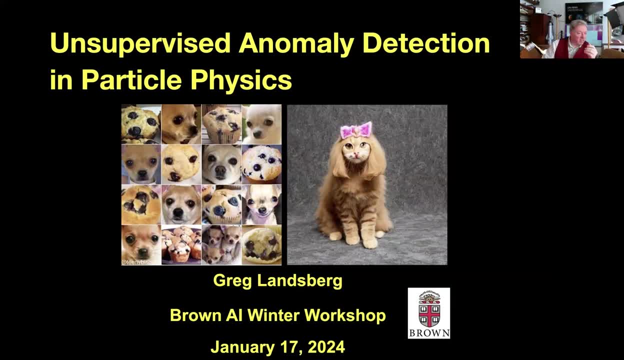 sure you do that. Okay, that was really the admin, according to our remarks. I think I'm going to pass over to my colleague now. Greg Landsberg and Lukasz Gozkoz are the two people that are going to be running this next session over the next two and a half. 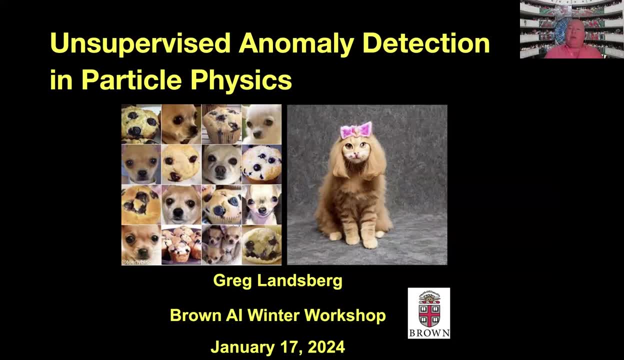 hours. Thank you so much. Thanks, Vic, I believe. actually yesterday Sean opened Google View access to the world, so you don't even have to be registered to be able to copy things from Google Drive, but definitely registering is needed for collapse, as you say, Right? so my name is. 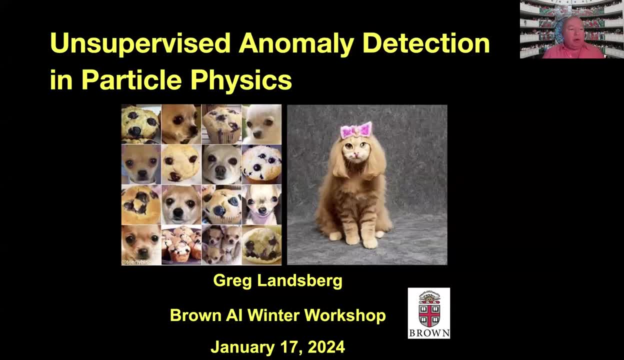 Greg Landsberg. I'm Professor Ed Brown doing particle physics, and Lucas Kouskos is my colleague who will basically run the exercises, and I'll give you the lecture. The title of this talk is Unsupervised Anomaly Detection in Particle Physics, and here are some pictures on how to say 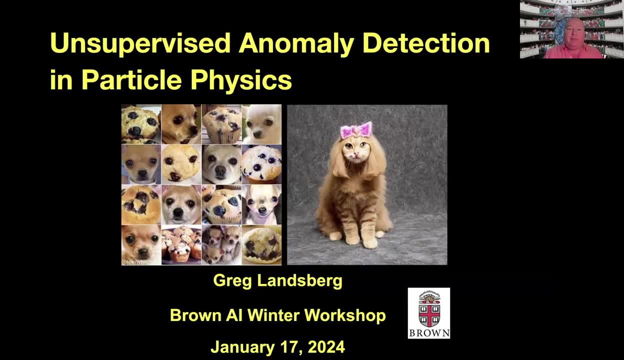 tell the difference between a muffin and a dog, which might not be trivial for a machine. sometimes Also how to synthesize different images. Here you have an image of a cat which actually looks like a poodle. So all these cute things could be done. 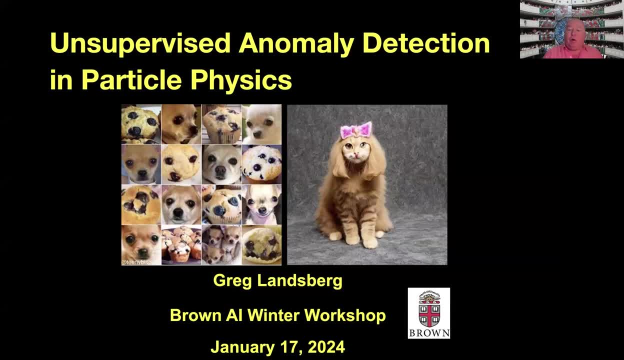 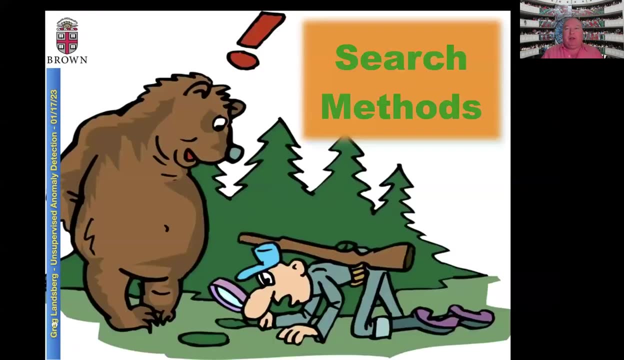 using unsupervised learning, and we are going to talk in many detail about that. But before actually going into the unsupervised learning, I want to talk a little bit about general search methods- Sorry, I didn't finish the outline, but I don't really need it- and tell you a little bit how we do. 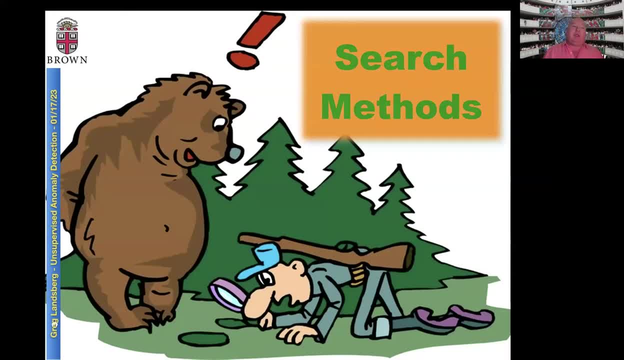 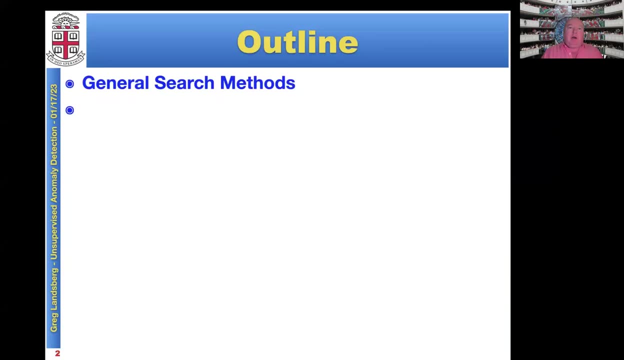 searches for new physics in particle physics, which is the raison d'etre and the main reason for the Large Hadron Collider, where I actually am now, at Soren, near Switzerland, near Geneva, Switzerland, why it was built. So, first of all, let's talk about the search concept. 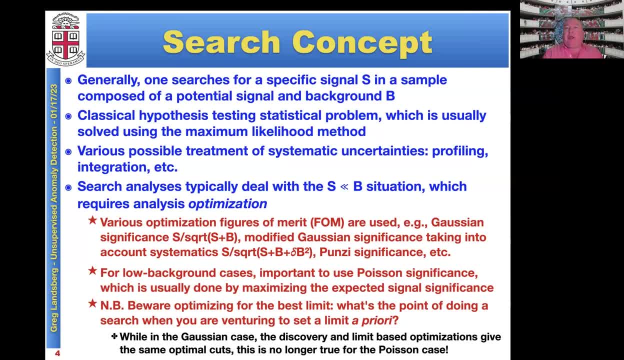 Generally, one searches for a specific signal with certain properties in a sample composed of a mixture of this potential signal and the background. This is a classical hypothesis testing statistical problem which has been solved a century ago, and it is the common solution to this problem is known as maximum likelihood method. One could also treat: 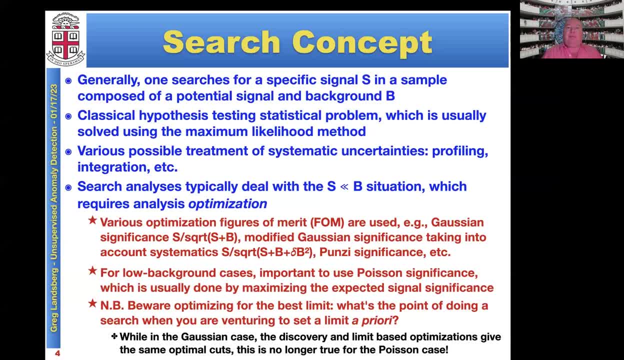 in a different way. uncertainties: There are systematic uncertainties in addition to statistical uncertainties in the maximum likelihood method and there are several different techniques, such as profiling, convergence, parameter integration et cetera. We won't be talking about that. We'll be focusing on machine learning aspects of the search. 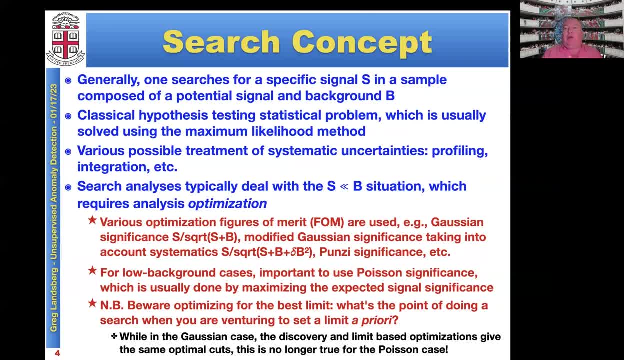 Search analysis typically deals with the situation where the hypothetical signal is much less than the background and that requires the analysis optimization. If you just look at the raw spectra, you won't be able to see the signal because it's typically overwhelmed by the background. There are different ways of optimizing signal versus background and 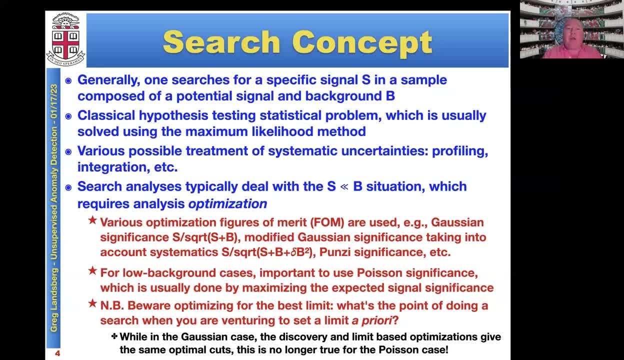 people use various figures of merit, the FOMs, For instance. the most common one for large statistics searches is the FOM. The FOM is the most common one for large statistics searches- is the FOM, For instance. the most common one for large statistics searches is the FOM. 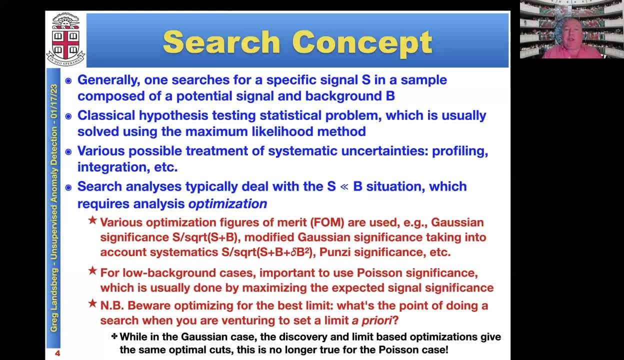 For instance, the most common one for large statistics searches is the GAUSS and significance which is given by the ratio of the signal- expected signal- to the square root of the sum of the signal works background. So if you maximize this thing in the Gaussian case, 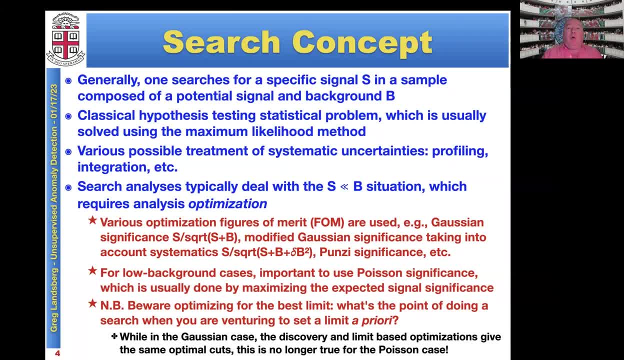 you would maximize sensitivity of your search. There is also modified Gauss and significance, which takes into account the systematics, and this is this formula: where b is modified by adding the variance of b squared, There is a so-called Ponzi secretion of b squared, which is a example of a very linear games. 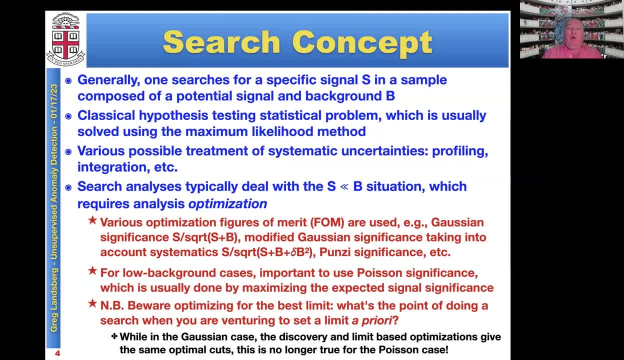 in the performance stage, but it's more likely than not being王 of all. sim っ For a socialanych he is suppose tolor, assimilated with the个, evolved regardless, he willポー傷 in the format, significance scheme, etc. For the low background cases it's important to actually use Poisson. 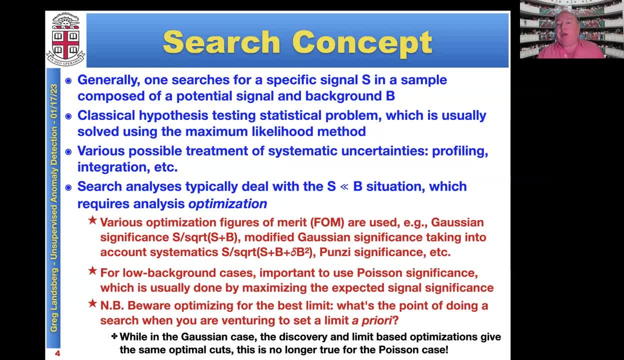 significance, which is usually done by maximizing the expected signal significance with the Poisson statistics. And, of course, whenever you optimize something, you should really optimize for best sensitivity for the signal rather than for the best exclusion for the signal, because the point of every search is to find something and not to set limits. You only set limit if you fail to find. 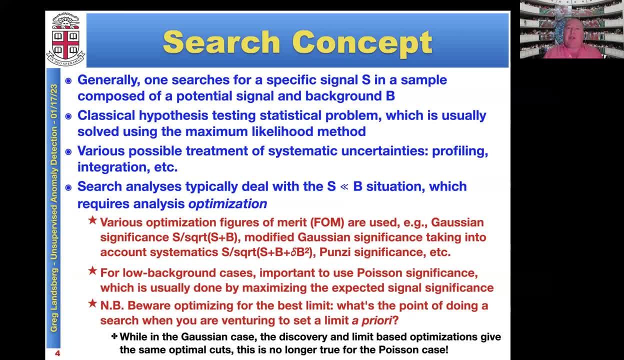 something. So while in the Galassian case the discovery and limit-based optimizations typically give the same optimal points, this is no longer true for the Poisson case, And if you start optimizing for a limit in the Poisson case, you might actually miss the signal, which is obviously. 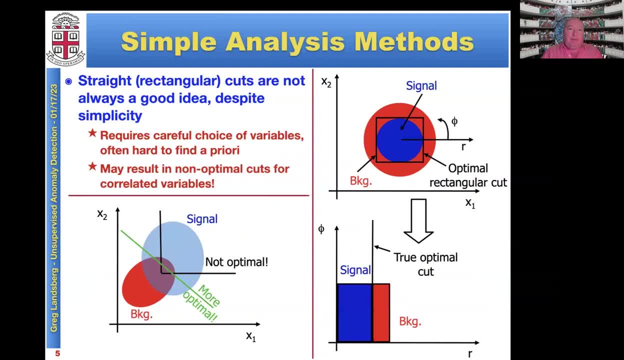 not good. Okay, so we started this business many, many years ago in particle physics And, of course, with the advances of statistical method and more and more powerful computers and various packages, visualization and data analysis packages- our methods of searches increased quite dramatically. 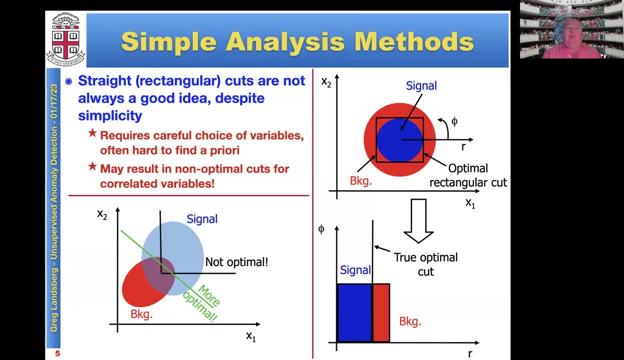 in sophistication. If you look at the papers in particle physics circa 60s and 70s, mostly people would use so-called rectangular cuts. So a rectangular cut in the two-dimensional plane is illustrated on the figure on the bottom left and you see some distribution of the background. 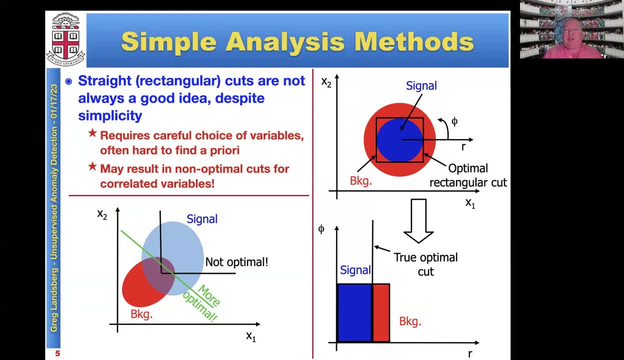 in red some distribution of the signal. In blue. there is some overlap And if you just try to use rectangular cuts- meaning x1 greater than something and x2 greater than something else- you would end up with a very similar situation. So if you just try to use rectangular cuts, 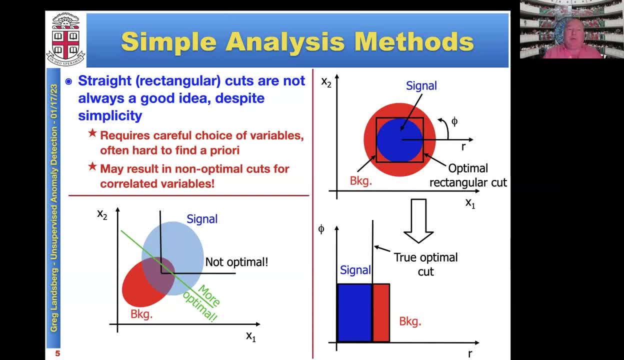 this rectangle which is shown is the black lines here, And clearly this is not the most optimal way to discriminate signal from the background. If, for instance, you correlate x1 and x2 and do something a little bit more sophisticated, like a diagonal cut, you would see much better. 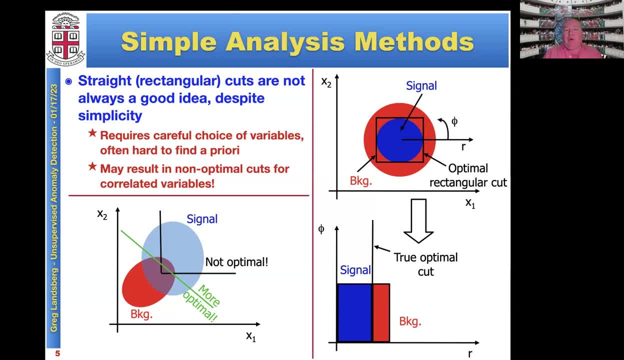 signal-to-background ratio or the signal significance, by doing the green cut, meaning cut, Cutting everything away below and to the left of the green line. But even the cuts which fully decorrelate two variables are not necessarily the best one, For instance, let's look at more. 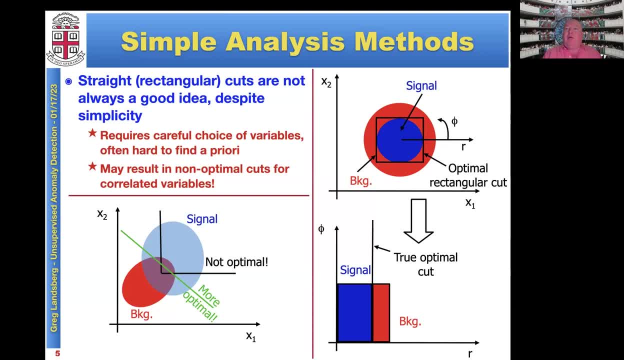 synthetic example top right, where a signal is a circle in blue which is surrounded by the background which has a shape of a donut. Clearly it's a very artificial example, but this just drives the point. So if you try to optimize things with rectangular cuts, 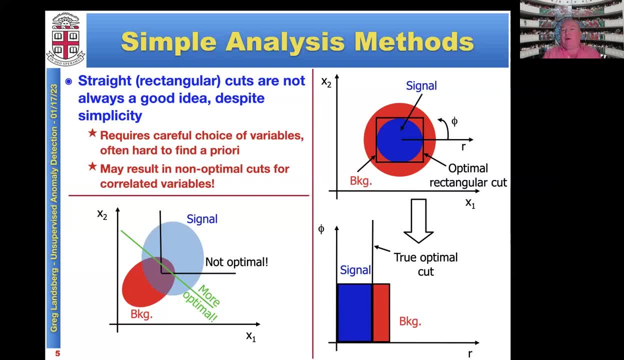 you would get something like the black box as your optimal signal selector, And of course, this is not the best one, because if you transform yourself into polar coordinates, with the origin of the polar coordinate system at the center of the two concentric circles, you could separate signal and background with hundred percent efficiency by simply cutting on 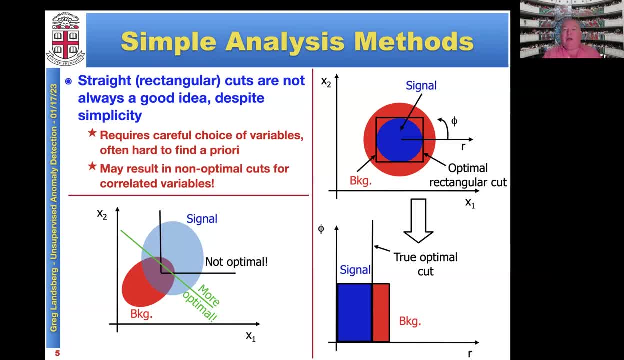 the radius in this polar coordinate system And this becomes a true optimal cut. Of course, this is a classical example where you could use a machine to optimize rather than doing it yourself. especially, it's easy to visualize things in two or maybe three-dimensional space. 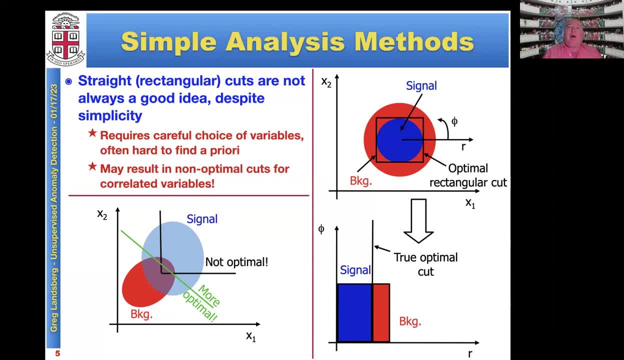 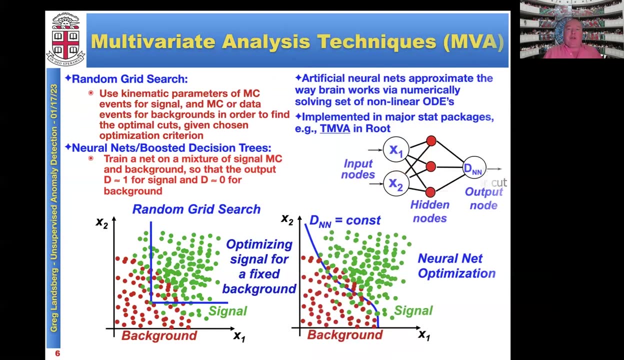 but it's fairly hard to visualize your selections if you have multi-dimensional space with 20 or 30 dimensions, which is fairly typical these days For searches, because you try to really uncover tiny signals under fairly large background. So in this case people actually used already in the 90s of last century. 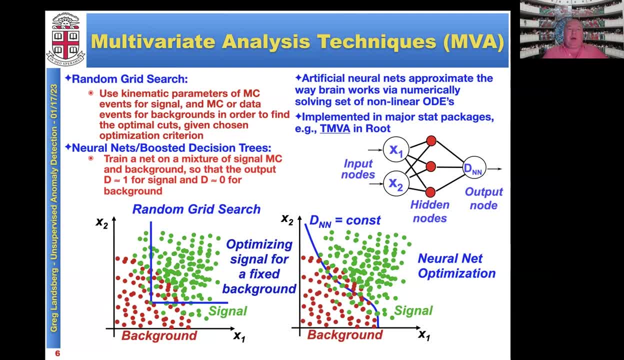 multivariate analysis techniques, And one of the simplest multivariate analysis techniques is random grid search, where you take, say, simulated background events and simulate thelimited signal events And then you just use individual events to pick a point in the multidimensional space And then you will find- you'll loop over all the events and find the 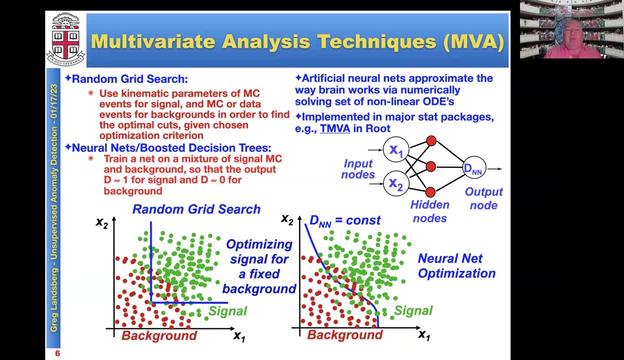 point which gives your optimal figure of merit of this separation of signal to the background And more sophisticated approach is to use multivariate techniques where you use nonlinear relationship, And a classic example of this is: what is this black difference, or a smaller green rather than the middle point is what should be the всп incidents於. 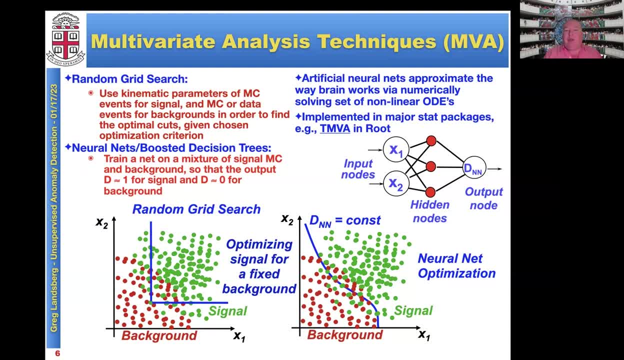 process gradeよ g1: tn2 a in micro grid, inside So related either neural nets or boosted decision trees, and neural nets are typically trained on a mixture of signal, simulated signal, events and background events in such a way that you essentially try to maximize the output of the neural net. the discriminant of the neural net, d to be one for. 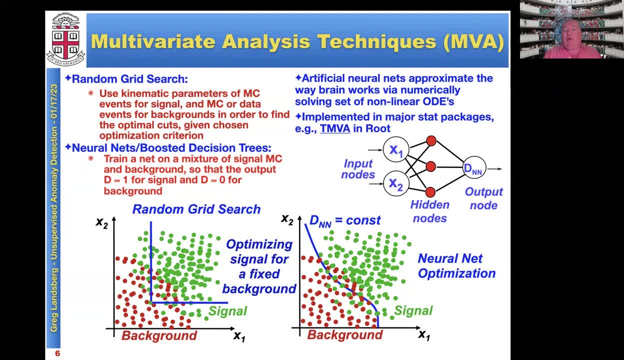 signal and close to zero for the background, and if you do so you get optimal separation between signal and background. in this example, the, the neural net at the constant discriminant value would give you some complicated non-linear contour in the plane of signal and background, and that is. 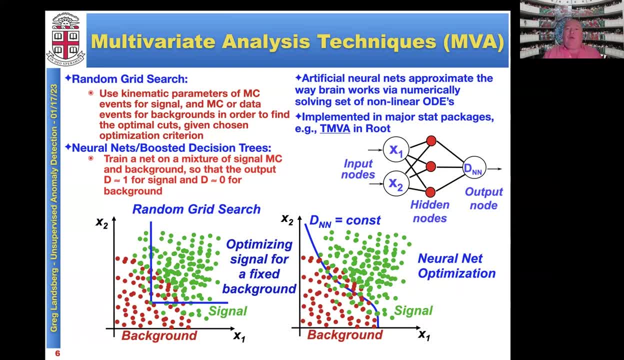 the optimum uh cut the artificial neural net nets essentially proximate uh the way our brain works by numerically solving a set of non-linear, ordinary differential equations, which is done by the artificial neural network. and then the artificial neural network is essentially done by a training of the net and they typically consist of some input nodes. these are the 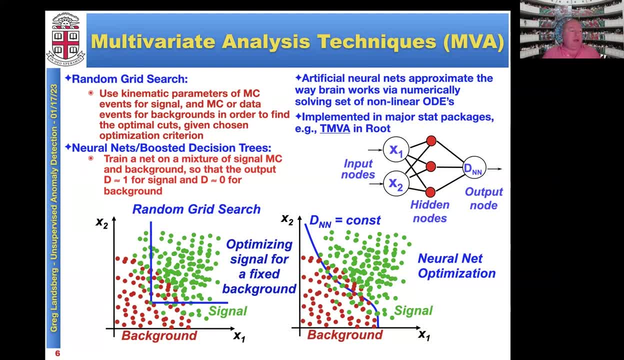 variables which you select to try to discriminate between signal and background, and then there are several layers of hidden nodes where all these non-linear processes happening and finally you output this discriminant. this is the simplest case of a single neural net which discriminates signal against the one, signal against one background that you could. 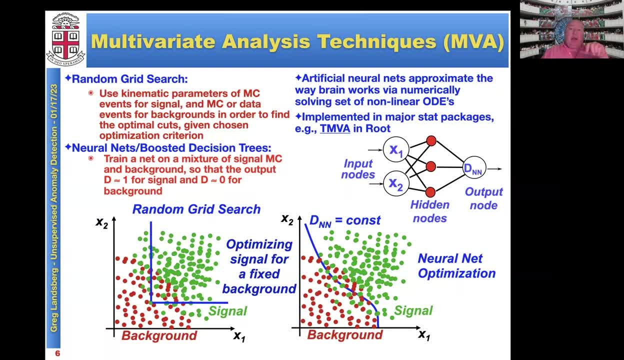 imagine more complicated configurations, and these neural nets have been implemented in major statistical packages. for instance, there is a tmba package in root. root is the soren data visualization system which we often use in particle physics, which allows us to analyze data, store data and then visualize data by displaying various distributions. all right, 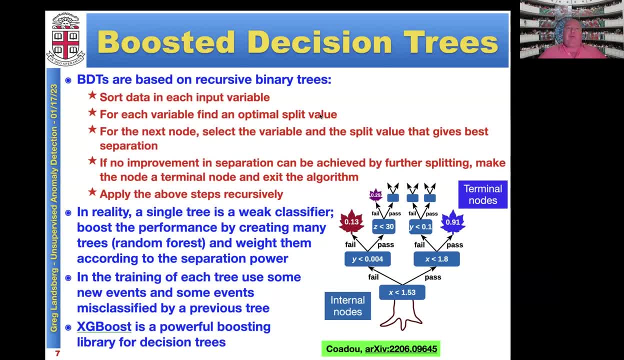 uh, so what are the boosted decision trees? well, boosted decision trees are based on recursive binary trees. you sort data in each input variable- this is x1, x2 and so forth- and for each variable you find an optimal split value. so you ask whether i should take the events where a certain variable 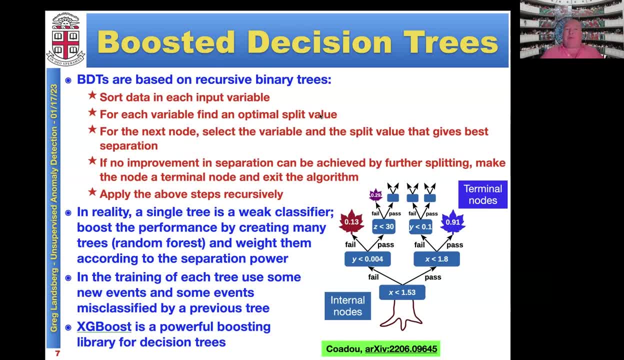 is above a threshold, or and you optimize for this threshold. for the next node, you select the variable and split value that gives optimum separation. and if no improvement in separation can be achieved by further splitting, uh, the node is a terminal node and the exit from this boosted decision tree. 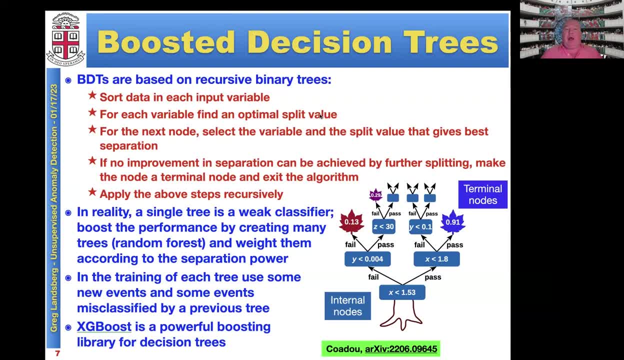 algorithm and these above steps are applied recursively. but in reality, a single boosted decision tree is not a very powerful classifier and we boost the performance of this classify by creating many random trees and weight them according to the separation power. this is known as random forest in the training of 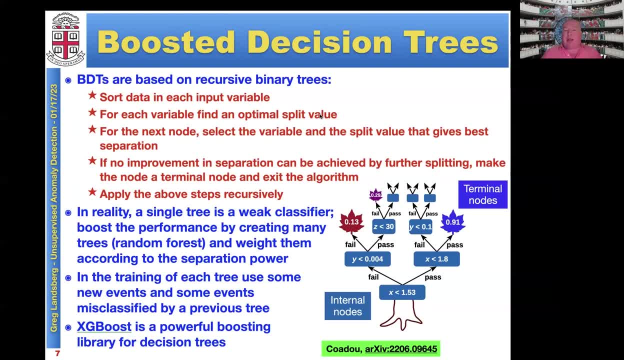 each tree we use some new events and some events misclassified by a previous tree. that's how we do the boosting. so if the first tree is not capable of classifying some of the events correctly, we feed the sample of these events in the other tree and hope that the other tree would be more. 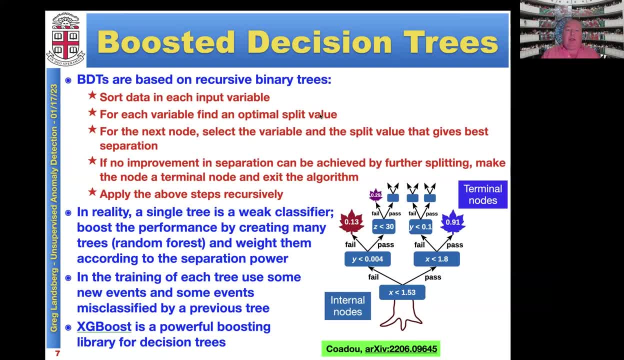 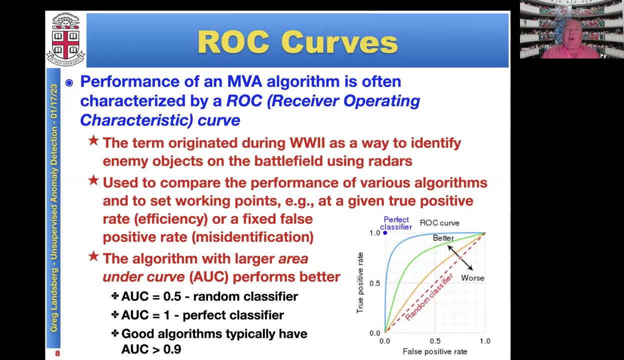 efficient in separating these events, and this is all done semi-automatically. there's a powerful libraries for boosted decision tree. the most commonly used one is xg boost, which is a python library in which you could use standalone way. the performance of a multivariate algorithm is often characterized by a rock curve rock. 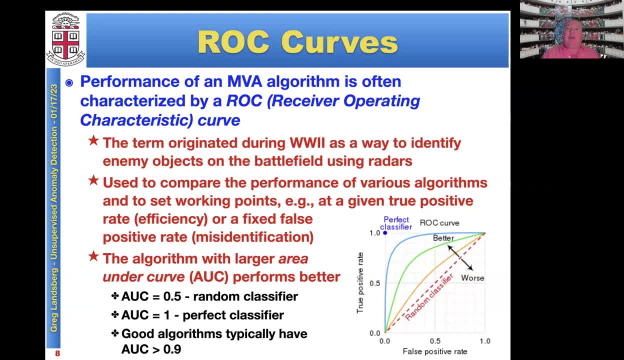 came from world war ii- this is the term which is acronym for vc and it's an over operating characteristic- and essentially this was uh invented during the world war ii to basically to classify the efficiency of radars to identify enemy objects such as aircraft, tanks versus some background objects, and they are used to compare the 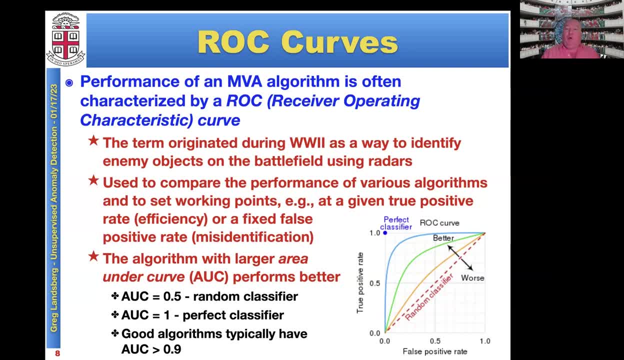 performance of various algorithms and to set working points for a specific algorithm where you could specify a true positive rate, which is how efficient you are in identifying the signal, versus a false positive rate, which is how often you misidentify background for the signal and, as you see on this plot on the right, the closer you are to the top left corner. 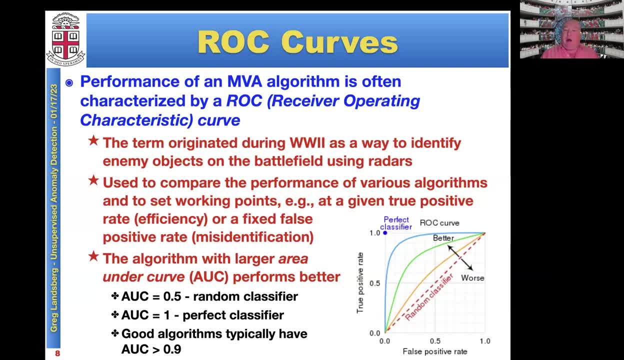 in the performance of the rock curve, the better you classify. a perfect classifier would be given by a dot in the upper right corner, which means that it has true positive rate of hundred percent and zero percent false positive rate. in reality, uh, we never approach perfect classifier, but you see, 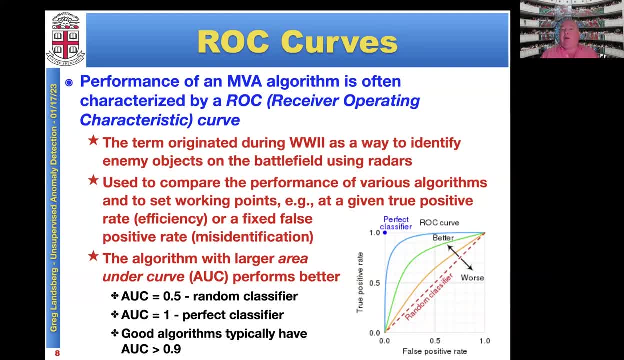 that the blue curve, uh, is doing significantly better than, say, a green curve, which already does better than the yellow curve. and if you just look at the diagonal which connects the lower left and upper right corner, this is the performance of the random classifier. you randomly choose whether to pull. 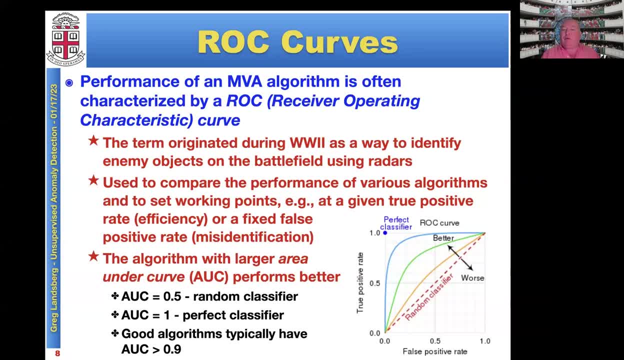 in event signal and background. then you get efficiency and false positive rate, the same which defines this diagonal. so of course any signal selection algorithm should be above this random classifier and hopefully approaches the perfect classifier. good algorithms typically have the area under the curve, which is the basically integral of the 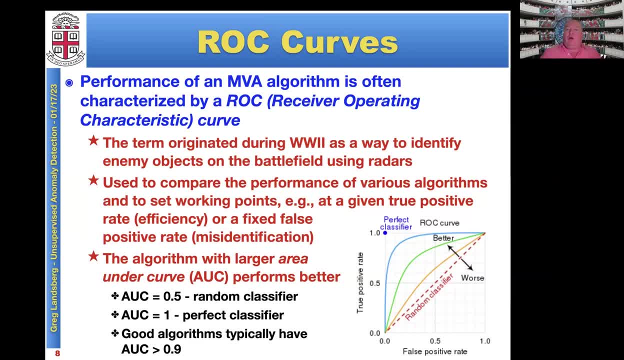 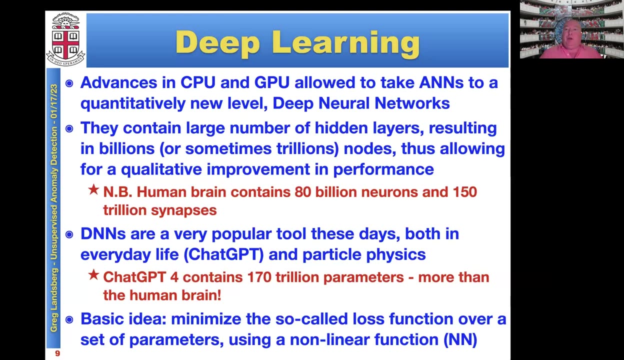 this uh rock curve from zero to one uh greater than ninety percent. so what you see, uh in blue. uh is the classifier this area under the curve about ninety five percent. uh, only five percent of the uh area is above this curve. now the advances in cpu, and particularly gpu, allowed to take. 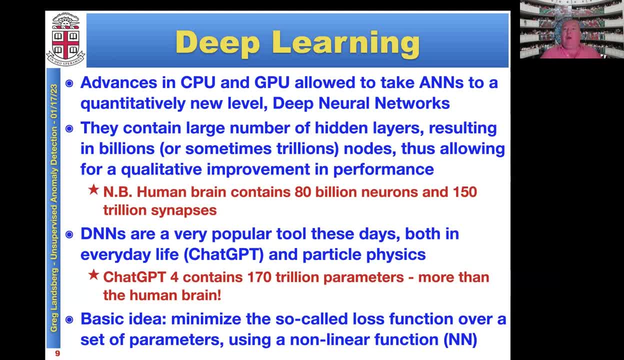 artificial neural nets to quantitatively new level, which we call deep neural networks or dnm. they effectively adjust more complicated complicated uh a n? n's. they contain a large number of hidden layer, resulting in billions or sometimes even trillions nodes, which allowed for a qualitative jump in the performance. things which were not 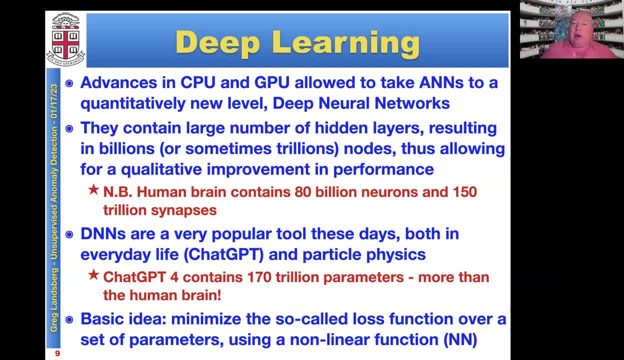 possible with shallow networks with low number of nodes. uh actually become uh walk in the park for these deep neural nets, and that's why artificial intelligence and machine learning became everyday uh think, rather than something esoteric which people use for specific uh tasks and typically in science. now, human brain contains about 80 billion. 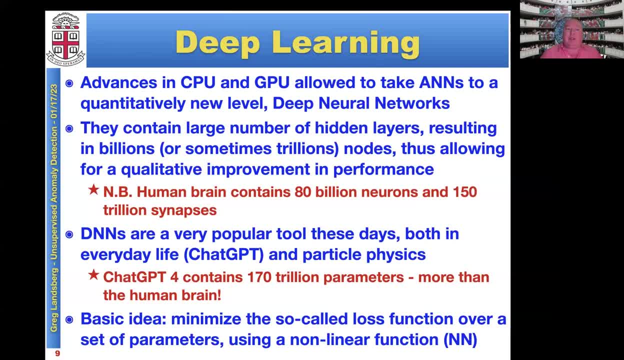 um neurons and about 150 trillion synapses and dnns these days actually over perform uh human brain- brain in terms of the complexity. For instance, chat GPT-4, the latest version of chat GPT, contains 170 trillion tunable parameters, So this is more than number of synapses in the human brain. 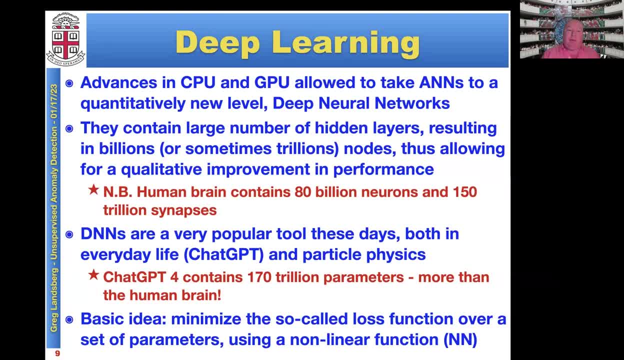 So in principle it would really outperform a human. The basic idea of deep learning is to minimize the so-called loss function over a set of parameters using some nonlinear function which is encoded in this neural network, And optimization of the neural net approaches the 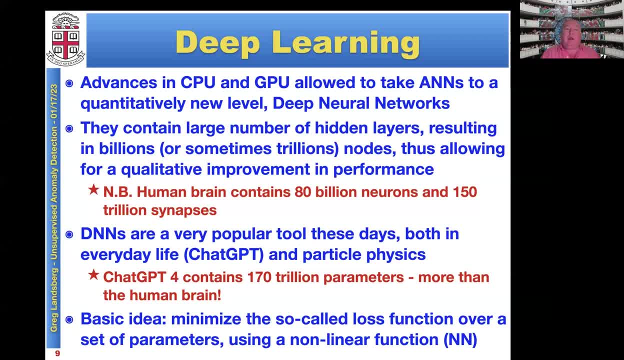 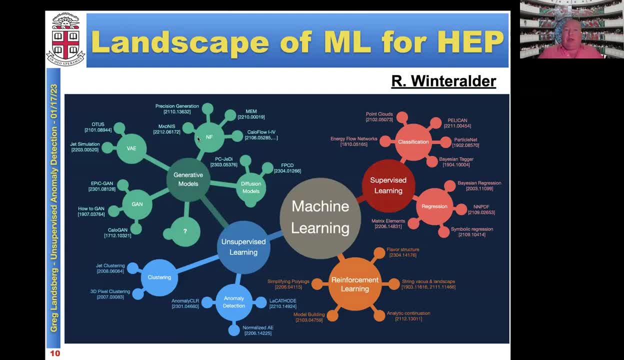 best solution from the point of view of optimization of maximum likelihood. The machine learning in the past 10 years really exponentially increased the use of machine learning in particle physics And this is a slide which was shown at one of the major conferences we have in the field. 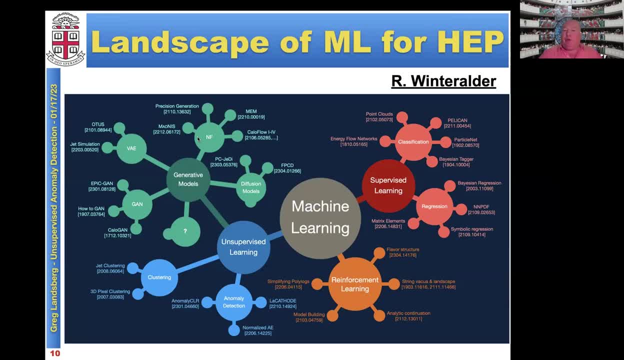 which shows all different type of machine learning and all different applications in particle physics, And the codes you see, like this: nine or 10 digit letters: 0.3,, 0.4, and so forth. The first two numbers is the year when this specific paper was submitted to the archive. 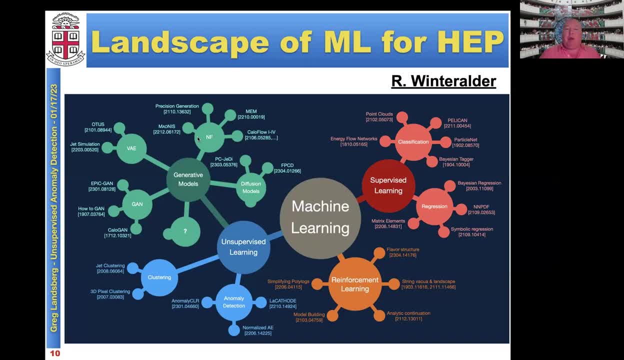 depository And you see that most of these papers have 22,, 23,, 21 as the year. So most of this development really happened, is happening in real time and happened in the last few years. You see only a handful of work which dates back to 2019 or 2018.. 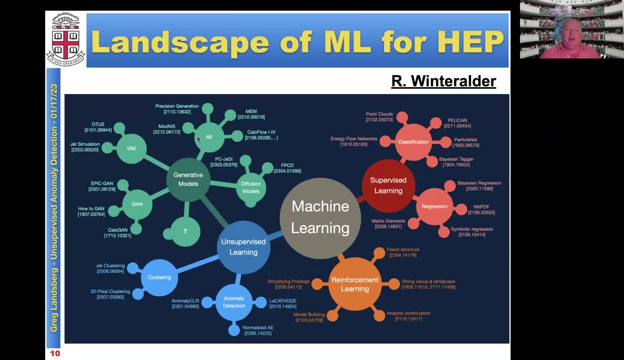 Most of them are really happening in the few years And you see that the landscape is quite large, and what we are going to talk mostly about today is this blue blob, unsupervised learning, And specifically we'll talk a bit about use of unsupervised learning for anomaly detection. 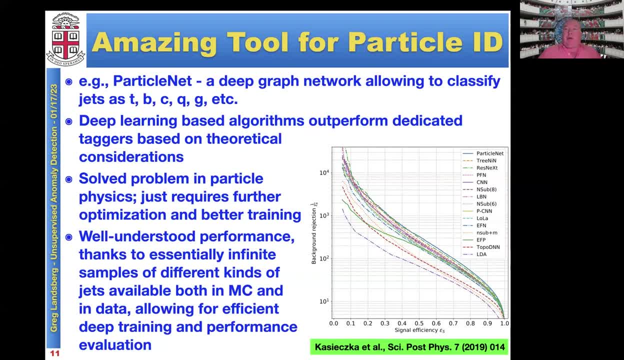 So the neural nets are really amazing tool for many areas of particle physics, in particular, for identification of different particles. A typical question we asked before we could do this is: how do we do this? How do we do this? How do we do this? 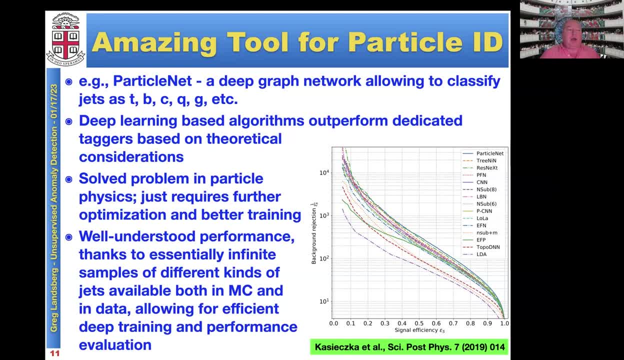 So to do the analysis whether an object we see in a particle detector is an electron or a jet- And sometimes jets look very much like electrons. so you could try to train a deep neural net to figure out whether an object has certain type. 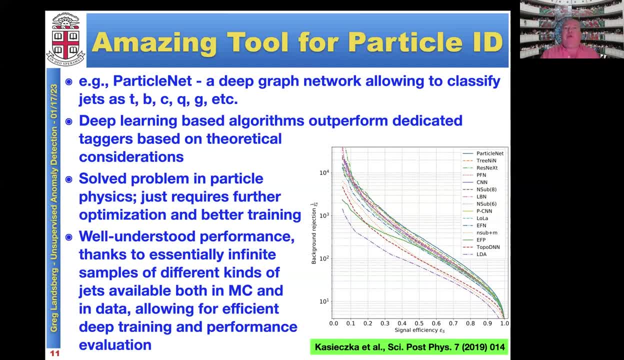 Or if you just look at the jets alone, you may want to ask yourself what is the core content of this jet, What this jet was originated by, whether it was a gluon, a light quark like UDNS quark, a charm quark, a bottom. 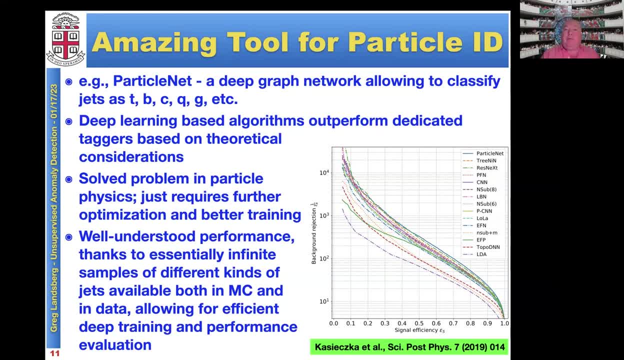 quark, or maybe even the heaviest of all, the top quark, And this deep learning-based algorithm by now outperforms dedicated taggers which are based on theoretical consideration. This is really a solved problem. There is no doubt that machine does better than human brain just by throwing. 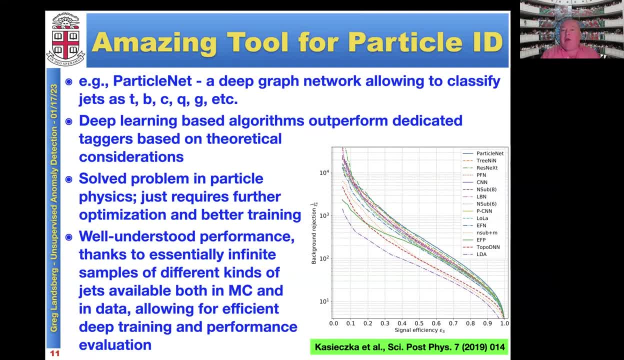 this problem on a huge neural net. These many, many different parameters- outperforms any theoretical basis tagger which uses matrix elements or some theoretical calculations to try to improve the separation between different classes. It has a very well understood performance because essentially we have infinite samples of different kinds of jets or different types of particles available. 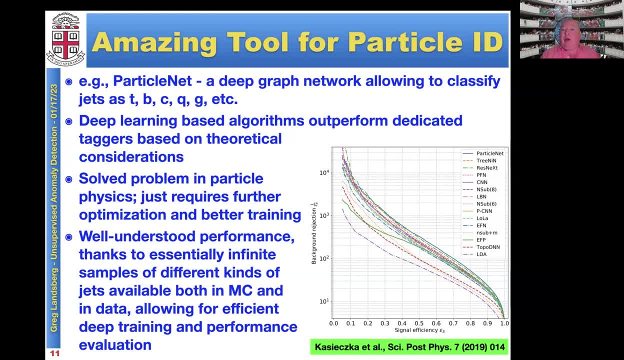 at the LHC So we could test the. we could train neural net on one sample, test it on completely different, statistically independent sample and make sure that all the things which could be pitfalls for machine learning, such as overtraining or picking on wrong features of the data set, are eliminated. 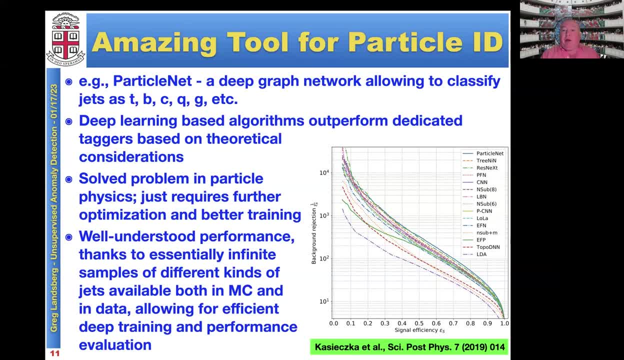 And that really allows us to do very well. This is a plot from one of the reviews which I referenced at the bottom, which shows, for instance, that ParticleNet, the deep graph network, which was largely developed by my co-runner of this session, Lucas. 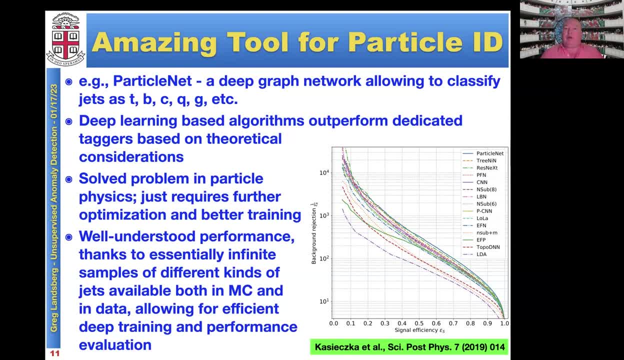 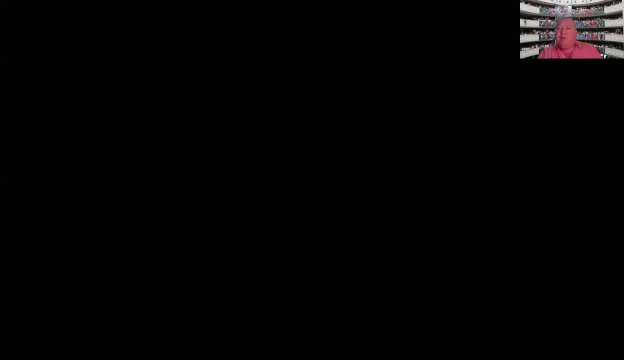 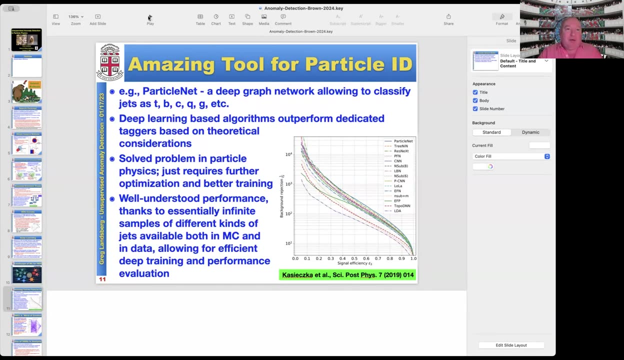 was really giving the best performance in terms of rejecting the background versus tagging the jet of a certain kind. So let me try to minimize the thing. I will switch From the screen mode full screen mode per second because I cannot minimize the window with people, which doesn't allow me to see a full slide. So the ParticleNet. 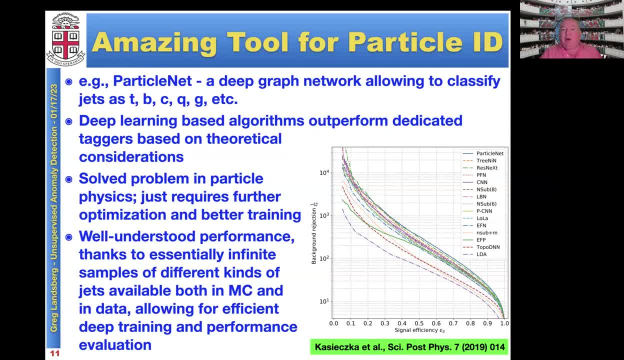 here is basically the line which you see on the very top. This is a rock curve and you could immediately see the ParticleNet has the highest area under curve, which is very good. It's a little hard to see what it is because the y-axis is in the lower bottom part of the figure, which is more than half of this line of the curve, whereas even the moving left corner of the cube Turns out that it is all, or the opposite of the curve, as you ask. I will show a single slide with vertical investigating. We, as teachers, base the hectare for this particular thing. 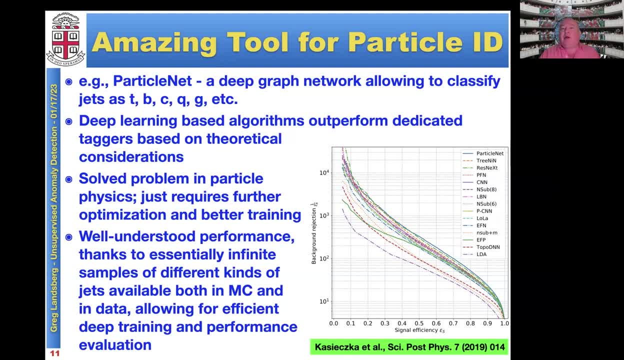 but actually now we will explain how to analyse the weight and weight of the particle in terms of crimes. in this particularới, The y-axis is a log scale, so it doesn't look like the log curves graphically on the previous few slides, but it has a fairly good performance. 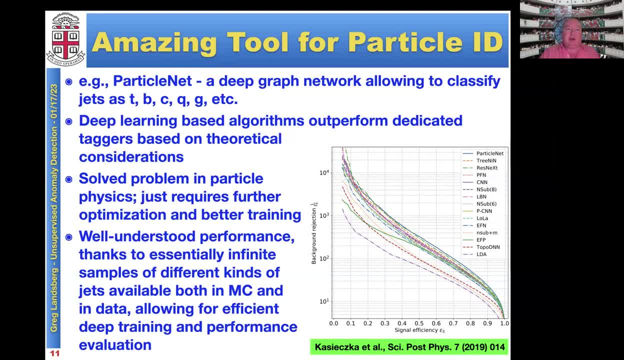 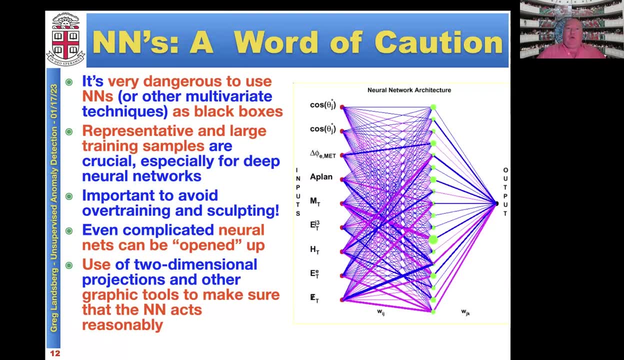 I think it's around 84% area, maybe a curve or something like that. However, neural nets: they are clearly very amazing tools, but they could be very dangerous if they're used as black boxes. It is critical to have representative and large training samples, especially for deep neural nets, who often have billions or even trillions of trainable parameters. 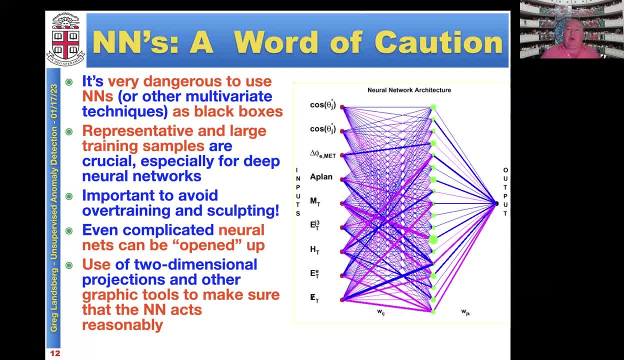 And it's important to avoid the overtraining of the net, where you peak on specific features of trained events which are not necessarily representative of the full sample, or to avoid sculpting. Neural net could actually sculpt some of the distribution, creating artificial peaks like mass peaks. 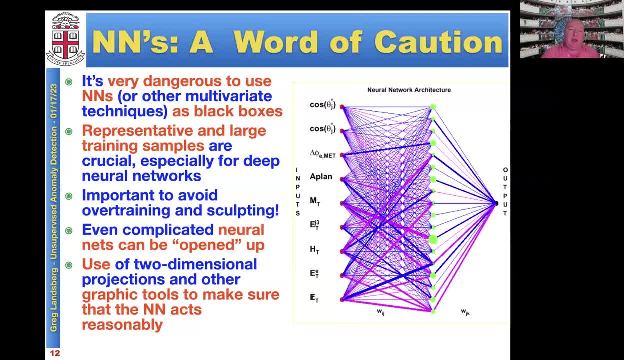 Which you could fool yourself thinking is a signal. Even complicated neural nets can be opened up. This is one example how you could actually visualize one of the networks where the size of the nodes is proportional to the importance of the feature And the thickness of the line is also proportional to the importance of the connection. 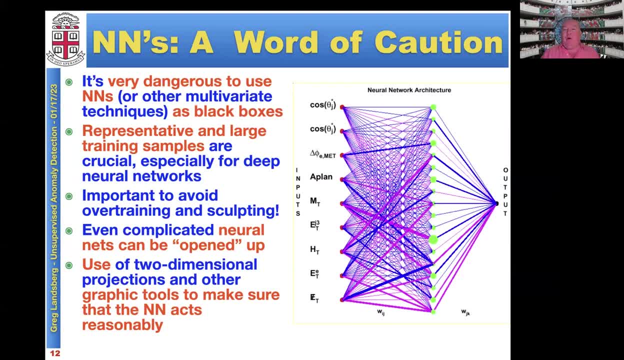 So you see that in this specific example, the node Which is given by the large green circle on one of the output layers is connected mainly to the variable known as MT, which is so-called transverse mass, which tells us that MT has large separation power between signal and the background. 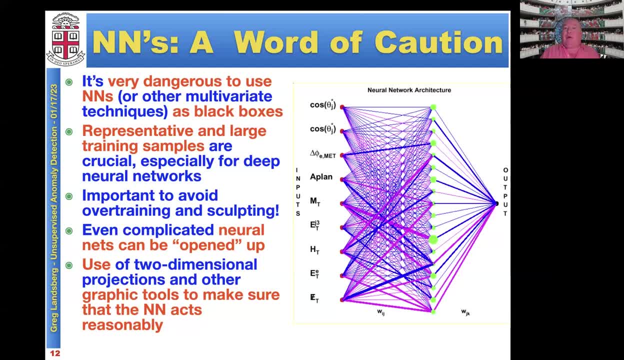 So modern tools allow you to make graphs like that and actually see which variables are most important for the neural net, And you could simplify neural net by removing the variables which do not help your performance, And there are same automatic packages which allow you to do this as well. 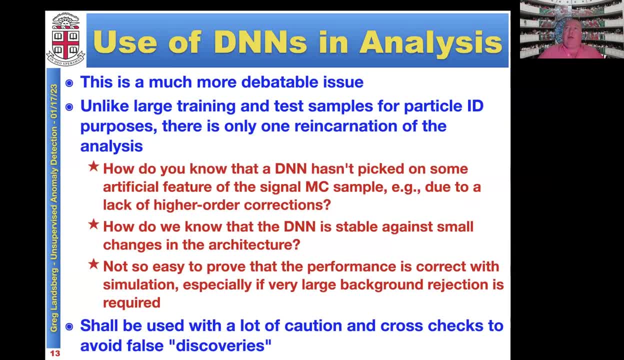 Now we talked about use of the deep neural net in particle ID, But using them in the analysis is a much more debatable issue Because, unlike large training and test samples which are available for particle ID purposes, There is only one reincarnation of the analysis. 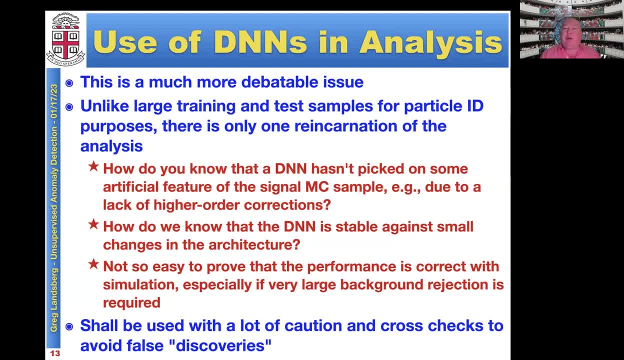 You cannot repeat the same analysis a million times in different statistical samples to make sure that the neural nets are not over-trained. And the main question which you would need to answer if you want to prove that your analysis is done properly Is: how do you know that this deep neural net hasn't peaked on some artificial feature of, say, simulated signal samples? 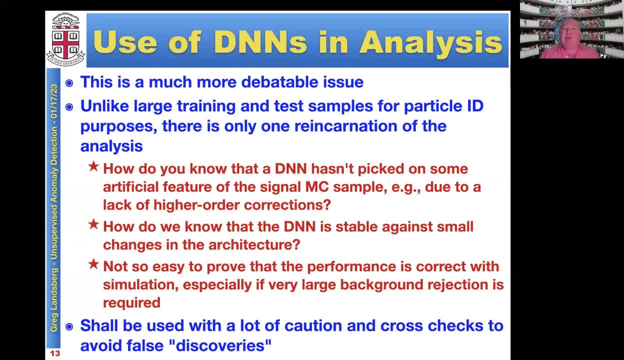 Or maybe it peaked on something Which is due to imperfect simulation, For instance, lack of high-order Feynman diagrams in a specific Monte Carlo generator which you use to simulate the signal. The other issues which you need to address is: how do you know that DNA is stable against small changes in the architecture? 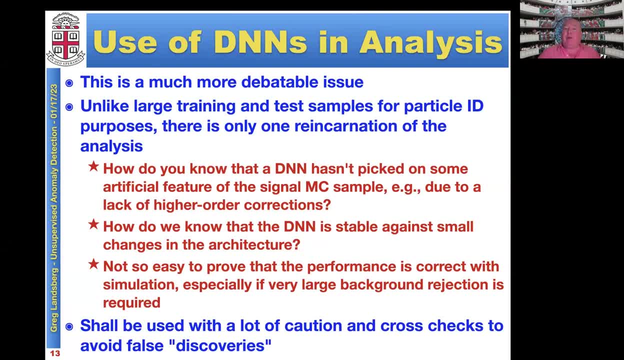 If you change a little bit the number of neurons in one of the layers, you don't expect the output to change dramatically. Things should be more or less perturbative in terms of small changes to the architecture, And it's not so easy to prove that performance is correct with simulation. 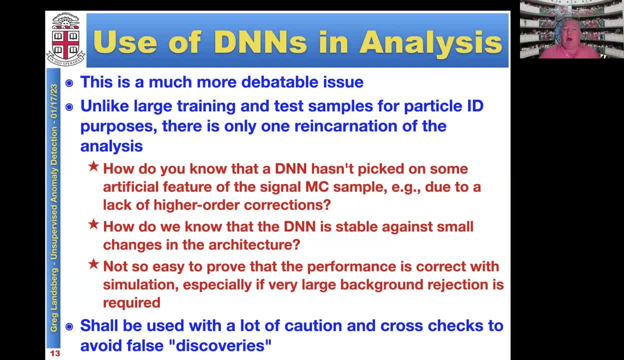 Especially if you work with very large background rejection, Say by a factor of a million, which is often needed Because you become very sensitive to any non-Gaussian tails in any of the distributions of the variables which you use For training this neural net. 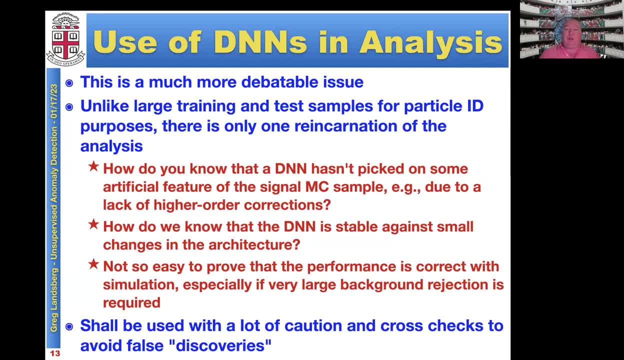 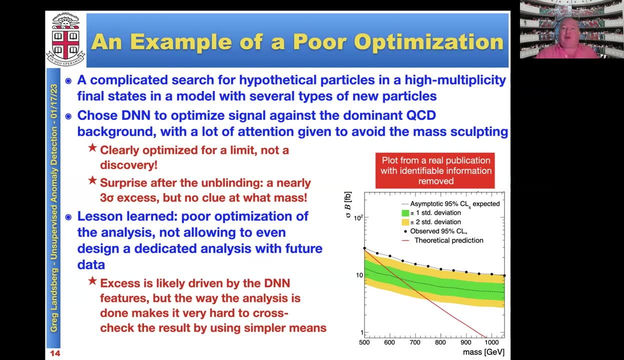 So DNNs in the analysis should be used with abundance of caution And with a lot of cross-check to avoid false discoveries. And here is one real-life example of rather poorly optimized analysis Which actually was published. So it's a real-life example. 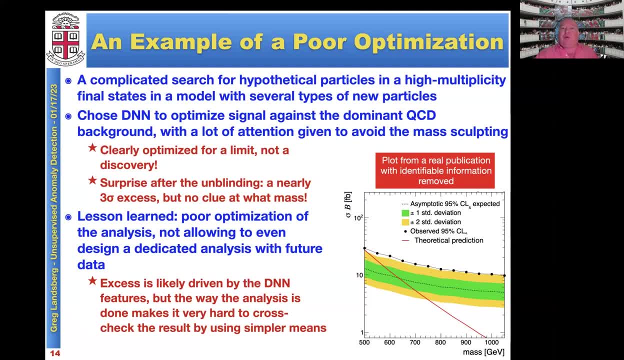 This is not anything synthetic. This was a complicated search for some hypothetical particle In high multiplicity, final state In a model which had several types of new particles, So signatures were very complicated. It had multiple jets. Some of them were jets originating from big quarks. 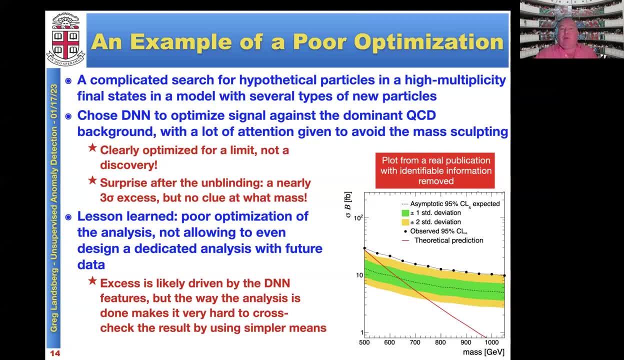 And the authors chose a DNN to optimize signal against the dominant background Which comes just from chromodynamics, production of jets, Which is the major background at the LHC, And they of course were aware of the problems Such as mass sculpting. 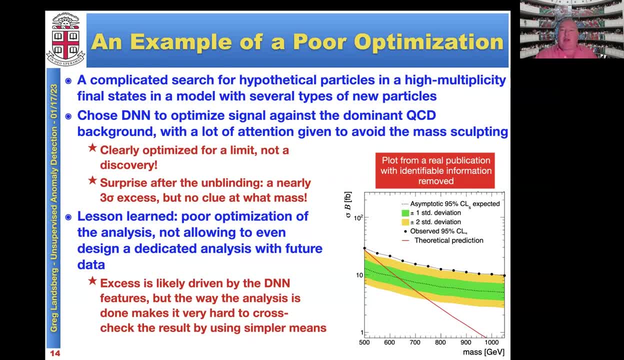 So they put a lot of attention to make sure that the neural net does not learn somehow artificially the mass of the signal from the training sample, Which might create an artificial bump in the application of this data, Even if there's no signal in data. 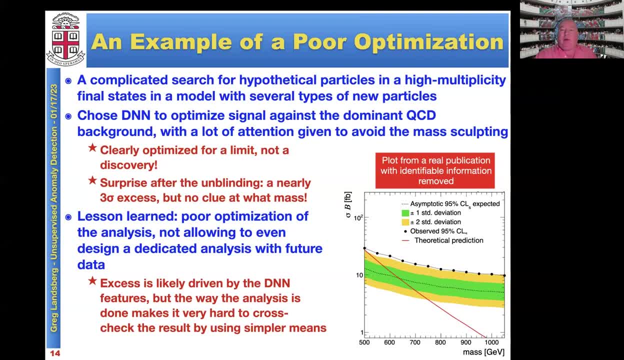 And then, when they opened the box, When they looked at the data, After optimizing everything on simulated samples, They saw a rather surprising result. You see it on the right. So this plot shows you the expected limit for this specific model. This is given by the dashed line. 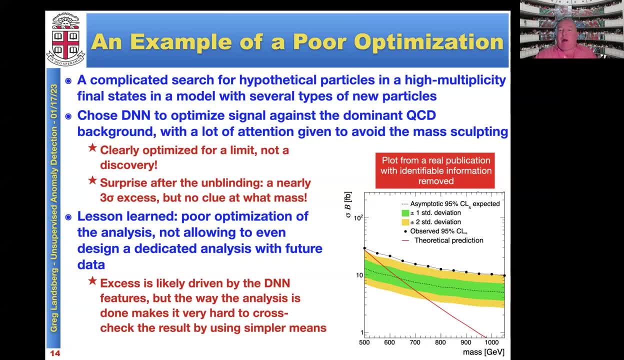 And the so-called Brazilian flag around it. The green and yellow lines represent the one and two standard deviation of the expected limit. So 68% of the cases You expect your observed limit to be within the green band And only in 5% of the cases. 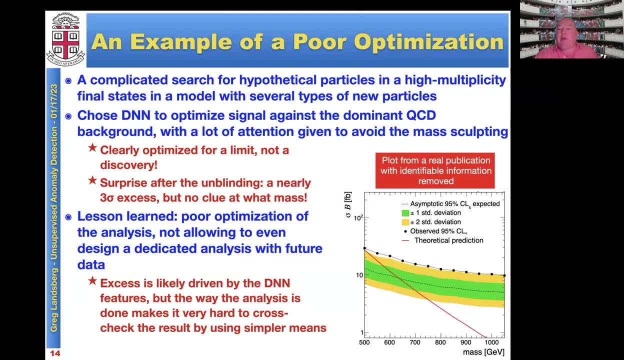 You expect your observed limit to exceed the yellow band And you see that their limit is above the yellow band, Essentially across the entire mass of this hypothetical particle plane, And it exceeds two standard deviations, In some cases nearly three standard deviations. And not only they couldn't exclude this specific model. 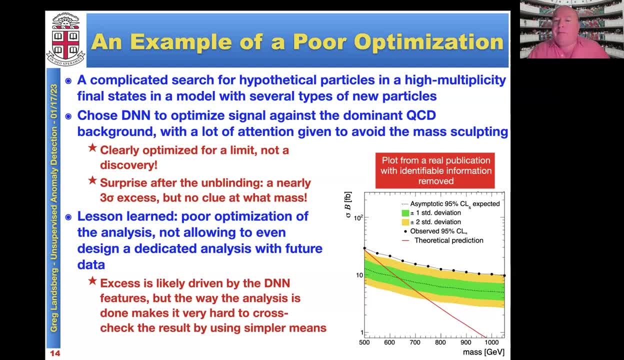 You see that the theoretical prediction is everywhere lower than the observed line. But also, if what they see is a view signal, They have absolutely no sensitivity to the mass. So the analysis was designed in such a way That a 500 GVU particle would give you exactly the same output of the DNN as a 1 TeV particle. 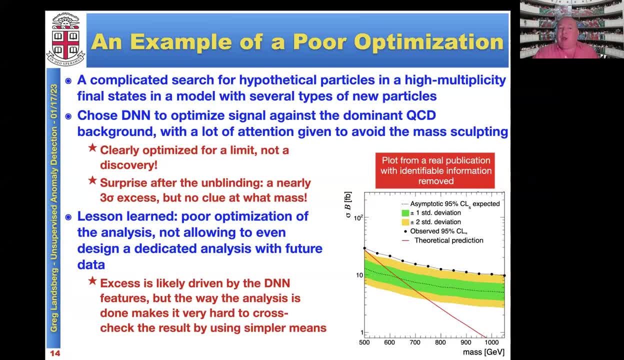 This is not a good thing. This is not a good design, Not a good optimization, Because this is optimization, Essentially, which was trained to give you the best limit. If they didn't see this fluctuation, They would have set a quite nice limit of around 600 something. GV. 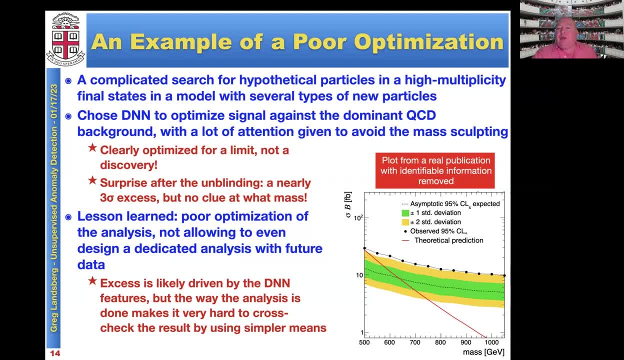 On the mass of this hypothetical particle. That's the intersect of the dashed line And the red line of the theoretical cross section. But not only they didn't exclude anything, They didn't even provide any information where to look for this phenomenon, If the success is real. 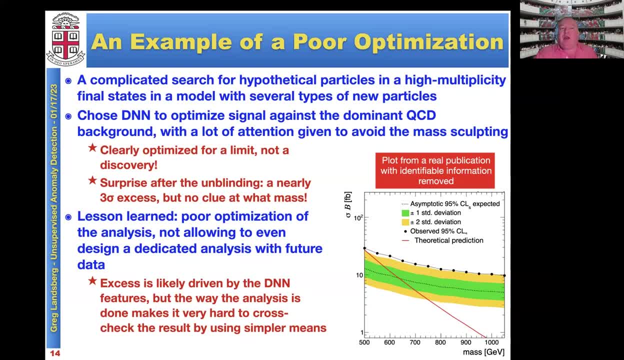 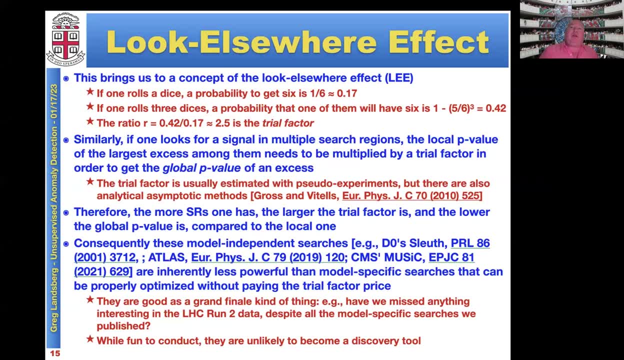 And that's kind of one example of how DNN is not particularly well used in the analysis. This brings me into a concept of Luke Ellesmere effect, Which is also important, And this is essentially the effect of multiple trials, Because when we do searches at the LHC, 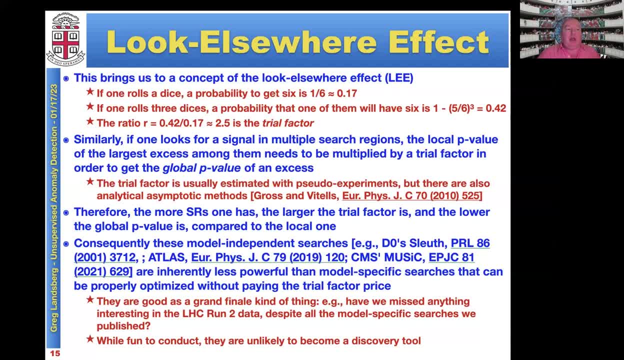 We look at more than one distribution. We look at many distributions, And the more places you look, The higher is the probability that you see an excess Just from a simple statistical fluctuation. So let's do an example: If one rolls a dice, 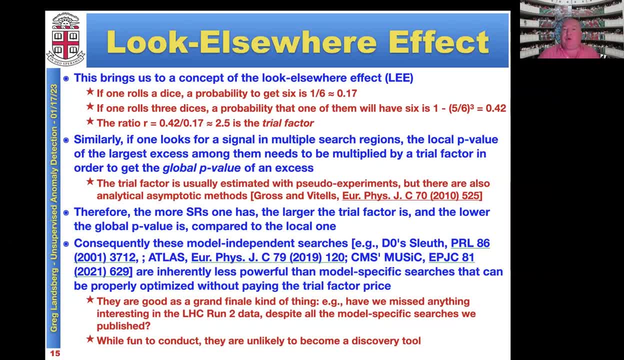 A probability to get 6 is 17%. One six If the dice is not loaded. If one rolls three dices, A probability that any of them will have six Face up Is one minus the probability that it's not six cubes. 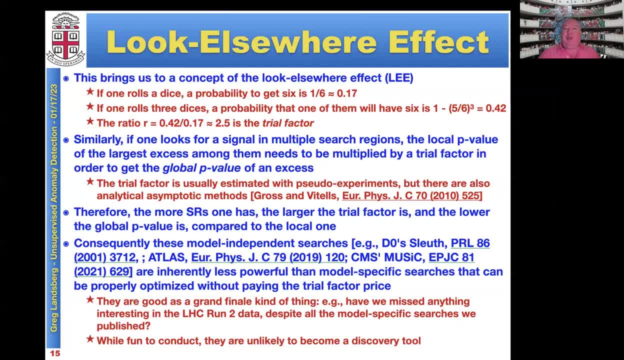 And this is 42%. So if you roll three dices, The probability to get the outcome you want Is two and a half times larger Than if you roll a single dice, And this ratio of 0.42 to 0.17.. 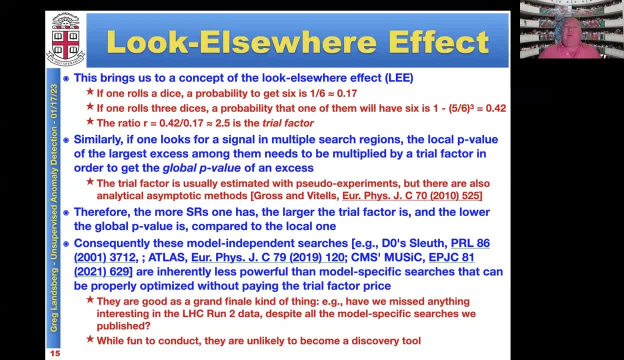 Is known as the trial factor. Similarly, if one looks for a signal in multiple search regions, The local excess Which you see, Which could be characterized by Gaussian p-value, Needs to be multiplied by a trial factor In order to get the global p-value of the excess. 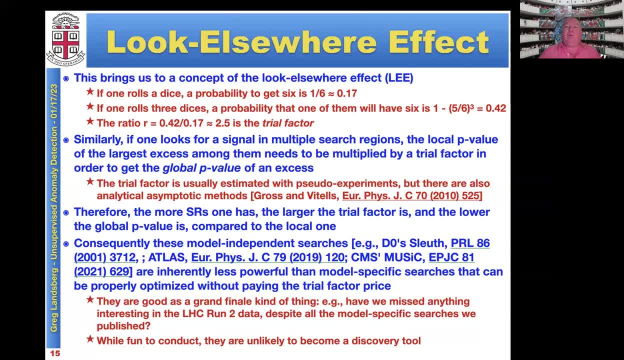 And this trial factor is usually estimated Through the experiments, Where you just repeat the experiment With simulated data, Using different simulated samples Every time. But there are also some analytical asymptotic methods On how to estimate the trial factor And, if you're interested, 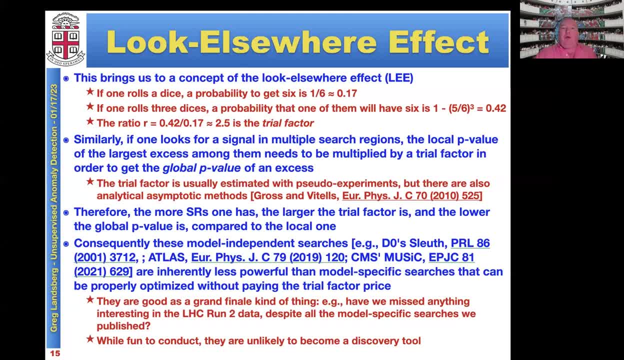 I give you a reference here. So, therefore, The more search regions one has, The larger the trial factor is And the lower the global p-value is Compared to the local one And consequently The so-called model independent searches Which have been attempted. 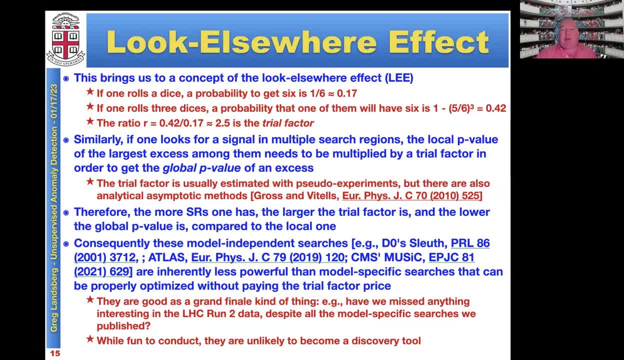 At various colliders, At the LHC By both ATLAS and CMS, And earlier at the Fernweb Teletron By D0. Which look at many, many different places, Trying to find an excess Against the standard model predictions. 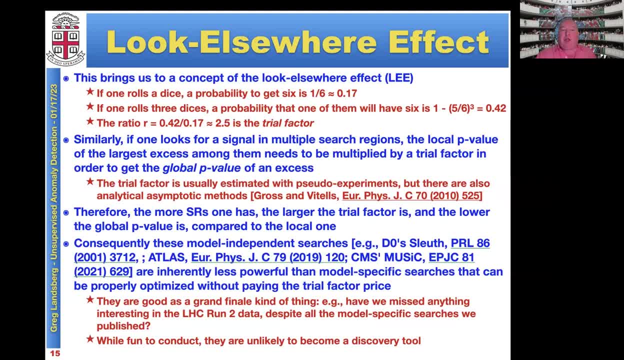 Are inherently less powerful Than model specific searches, Because the model specific searches, When you know exactly what signal you're looking for, You could properly optimize Your search regions Without paying the large trial factor price. And this also become important With deep neural nets. 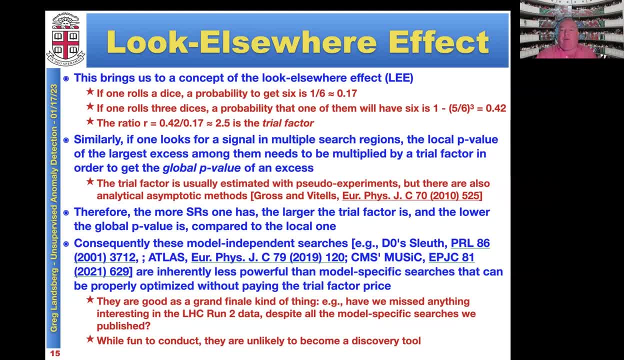 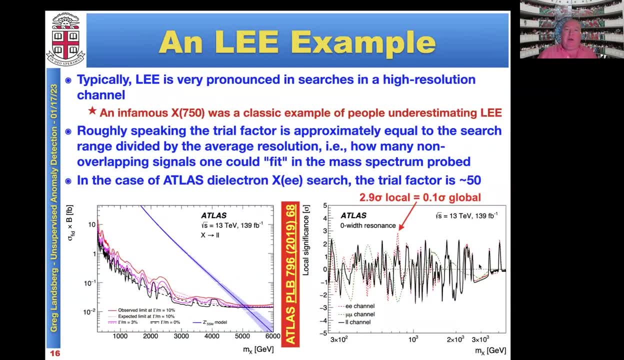 Because this neural net itself Could bring in some trial factors, Due to its complicated architecture And also the various samples used For training this neural net. One example of Lukau sphere effect, Which usually are very pronounced In high resolution channel: 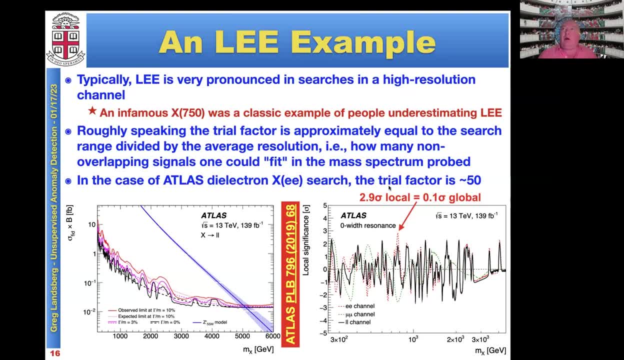 Essentially send the entire theoretical world On a wild chase Of something which never existed. This is an infamous particle Which was called X750. Which, basically, was just A statistical fluctuation And the fact that both Atlas And CMS had an excess. 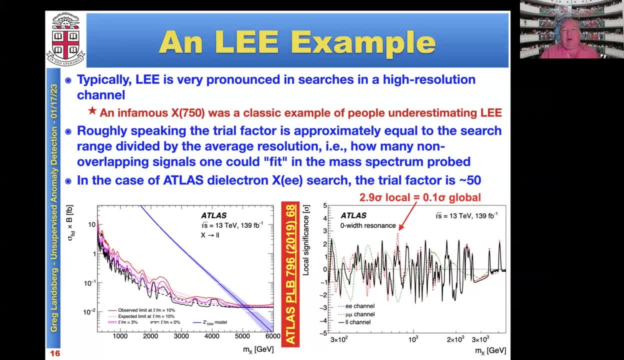 Around the 750 GV Right here. Basically people thought That if two experiments see The excess at the same place, There's no Lukau sphere effect, Because you know, If Atlas saw it at 750 GV, One could just look at CMS. 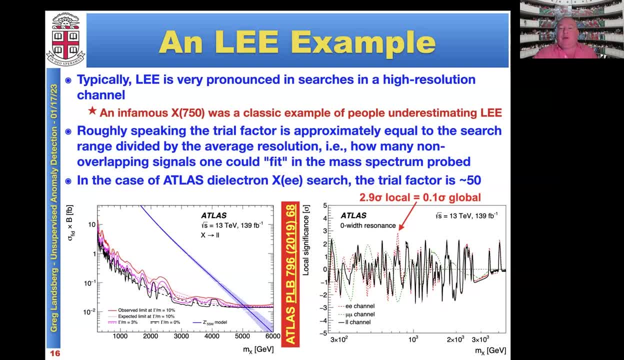 At 750 GV And remove any trial factor. This is, of course, incorrect, Because the fact that Atlas saw it at 750 GV Doesn't preclude That it could have seen it at 900 GV, 2000 GV. 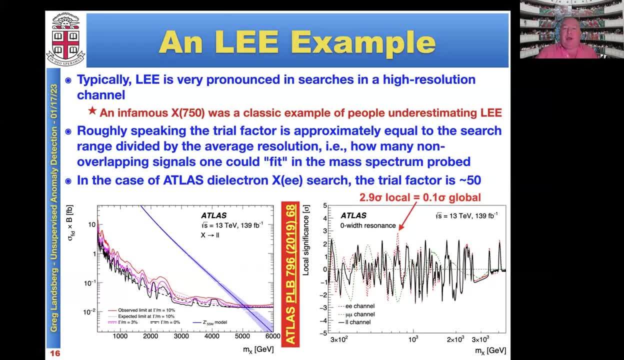 Or any other value, And since you see how quickly The absorbed limit fluctuates Around the expected limit, Which is because This is a diphoton channel Which has very high resolution, So the width of this Statistical fluctuations Is proportional to the resolution. 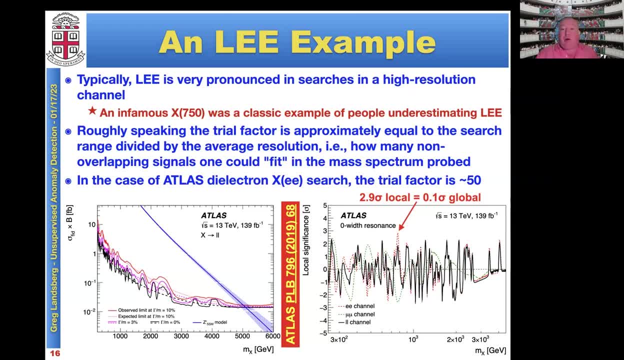 You could see that Actually the Lukau Lukau sphere effect Is quite large And, for instance, The highest point Of excess in Atlas, Which had Nearly three sigma Gaussian significance After this trial factor Turned in something like 0.1 sigma. 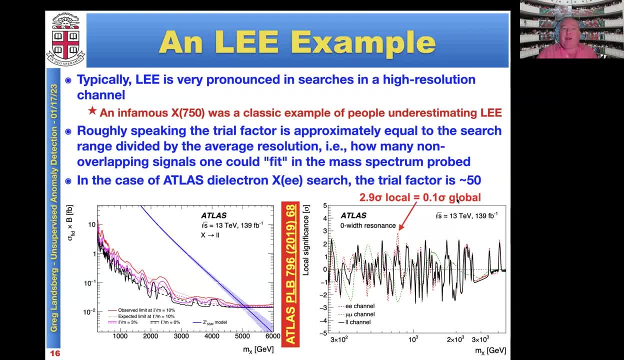 Which is essentially Zero, And This is important to Keep in mind When you do Searches For new phenomena, Because it's easy to Discover something Which doesn't exist Due to these Statistical fluctuations, Which are enhanced. 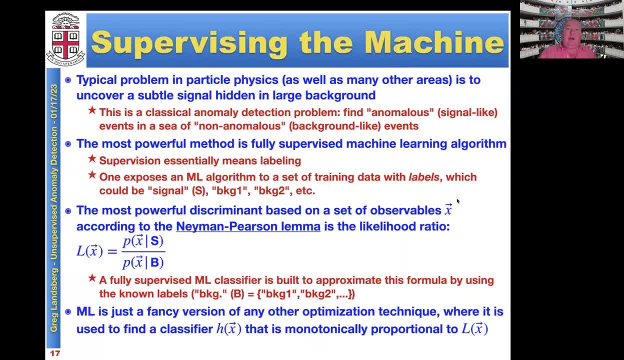 By a large trial factor. Okay, So Now let's move to Real Need of this talk On the machine learning Aspects: How to supervise The machine To properly Do the Background And signal Separation. 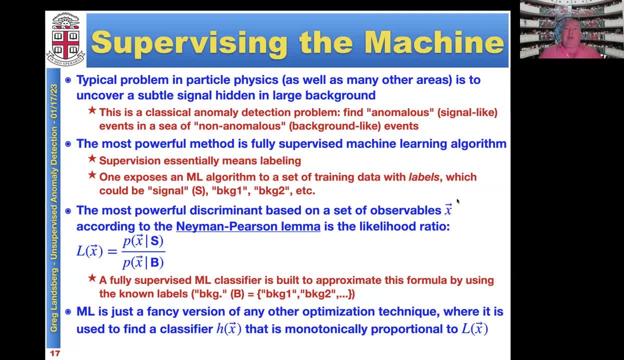 This is a typical Problem in particle Physics And essentially It's a problem Of Uncovering A subtle signal In Large Background Sample, And this is also A classical Enormally Detection Problem. 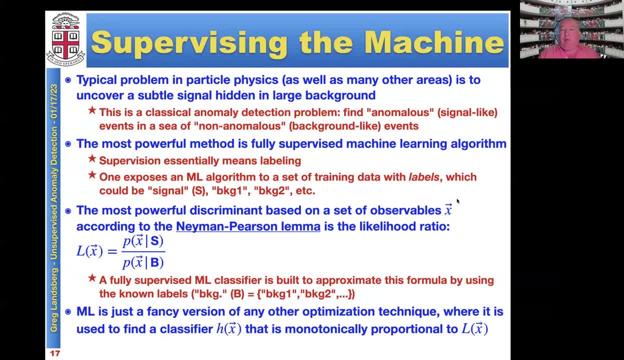 We are trying To find Anomalous Name With signal. Like Events In The Large Pool Of Background. Like Events Is The Fully Supervised Machine Learning Algorithm. 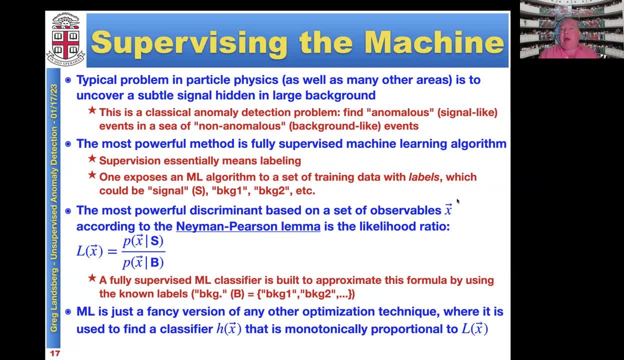 Supervision Essentially Means Labeling. That Means That We Have A Training Sample With The Events, Which A Mixture Of The Background Process, So One 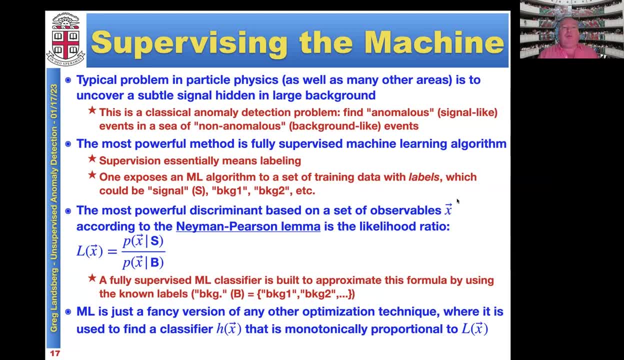 Exposes A Machine Learning Algorithm To Set Of Training Data With These Labels, Which Could Be Signal, One Type Of Background Background, One Background Of 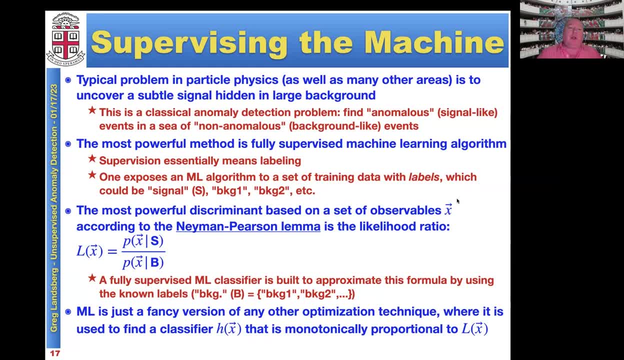 Seeing The Outcome X. Given The Signal Over The Conditional Probability Of Seeing The Outcome X, Given The Background And A Fully Supervised Machine Learning. 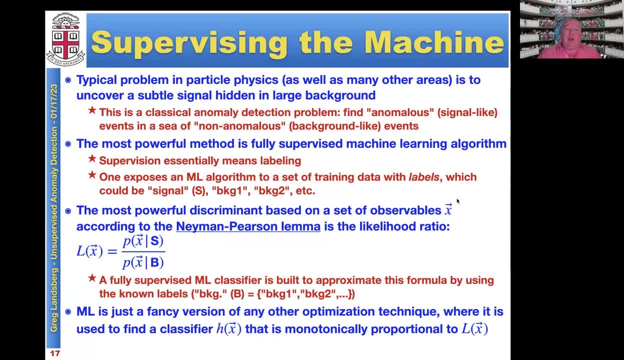 Classifier Is Built To Use Just A Fancy Version Of Any Other Optimization Technique Where It Is Used To Find A Classifier Age That Is Monotonically. 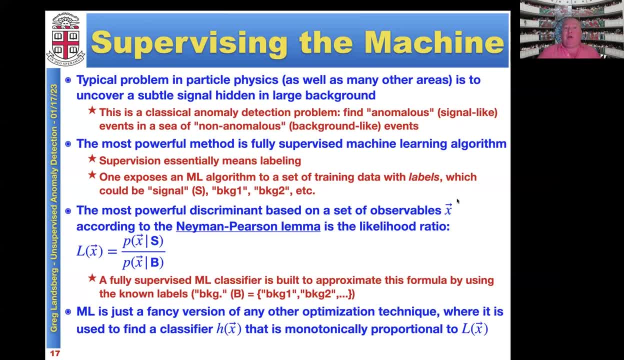 Proportional To The Likelihood Ratio. If You Think Of, The Maximum Of Likelihood Would Correspond To The Maximum Of Such A Classifier Age Of. 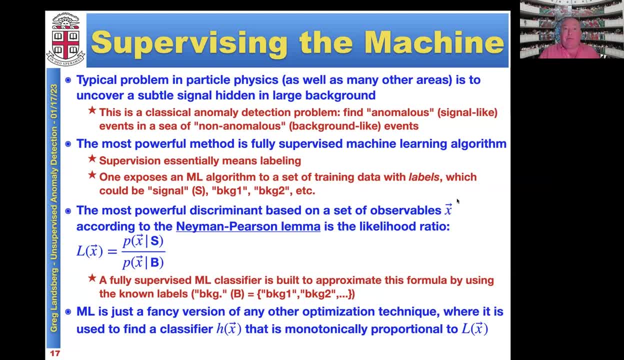 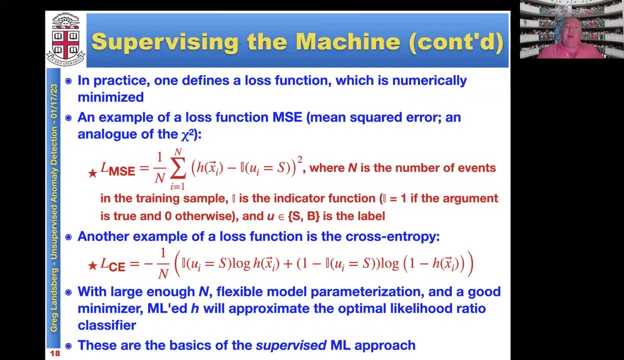 X. So Machine Learning, If You Think About This, Is Just The Example Of Loss Function. Is MSE Or Mean Squared Error? This Is An 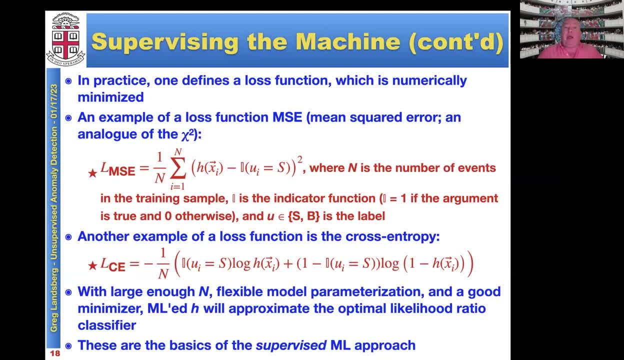 Analog Of Chi Square Statistics. So The Likelihood Ratio, The Loss Function For The MSE, Is Equal To One, If The Argument Is True And 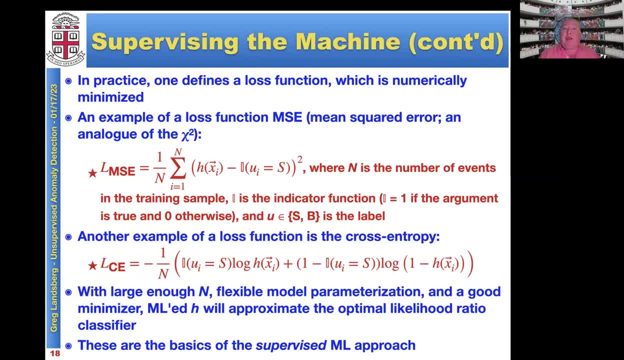 Zero Otherwise. So If The Event On The Issue, Event Number I, Is A Signal Event, The Indicator Function Is Going To MSE. This Is Equivalent. 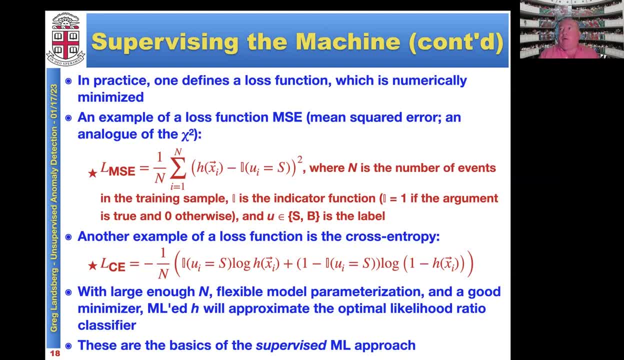 To Maximization Of The Likelihood. This Is For The Same Reason Why Chi Square Is Just The- If You Take The Poisson- Likelihood And 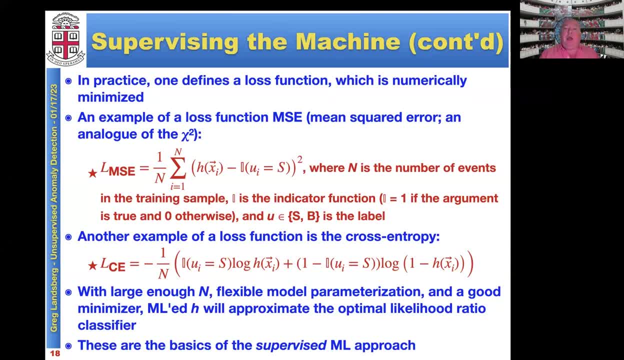 The Loss Function Is Defined In A Different Way, But Again One Can Show That It Essentially Approximate The Optimal Likelihood Ratio Classifier If. 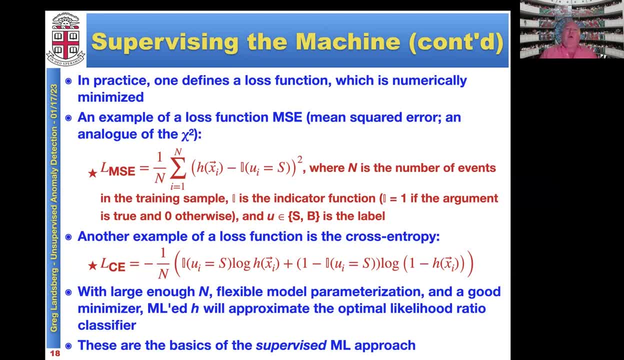 You Have Large Enough Training Sample Being Due To The Background Using Machine Learning Technique, Using The Loss Function Instead Of The Maximum Likelihood Ratio. 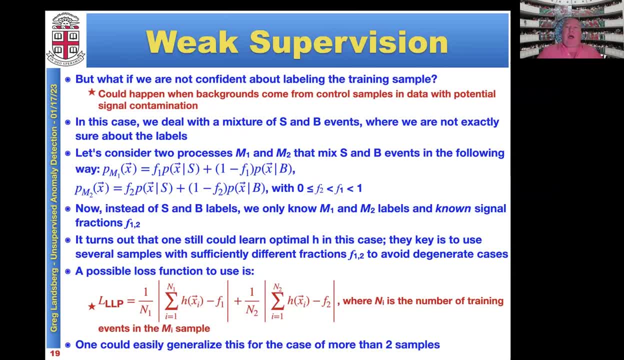 And Optimizing This Loss Function By Minimizing This Loss Function Essentially In Data With Potential Signal Contamination. In Some Cases One Cannot Trust Simulation. 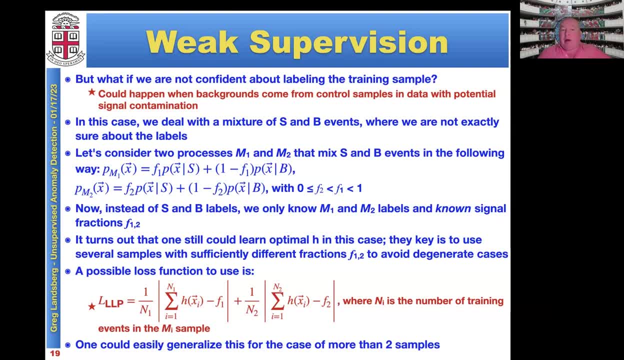 To Simulate The Backgrounds, Because Backgrounds Are Very Complicated And They Might Not Be Properly Simulated And Sometimes It's Just Impossible To. 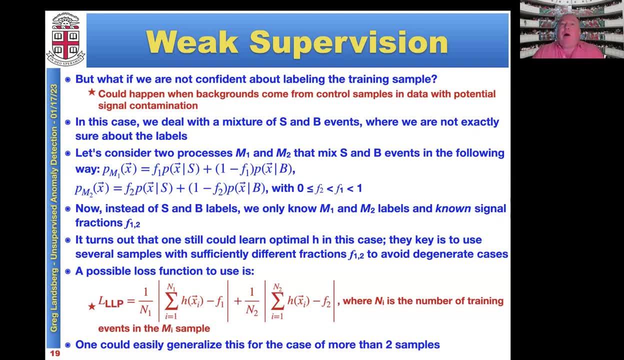 Find A Good Sample Where You Have A Pure Background Without Possible Signal, Or Pure Background Of A Certain Kind, In This Case, Following Probability, Density. 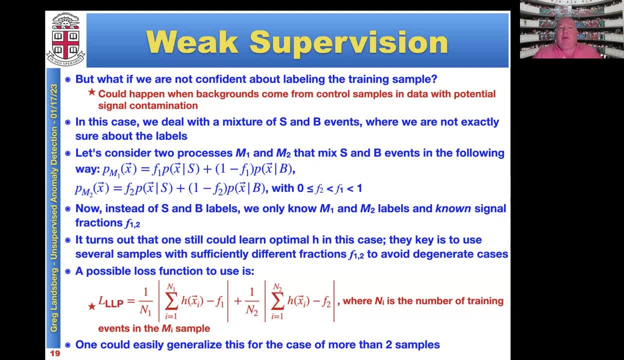 Function, The One Pm, One Of X Is Some Constant F1.. P Of X, Given The Signal, Plus One Minus This Fun, This Parameter. 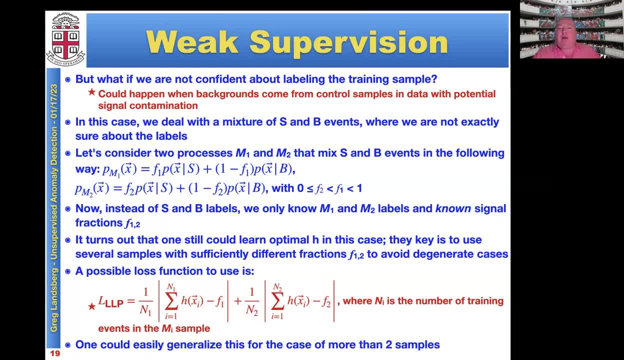 F1. Times, And Both Of Them Are Constraint Between Zero And One, So F1. Is Essentially Fraction Of The Signal In Your Sample And One 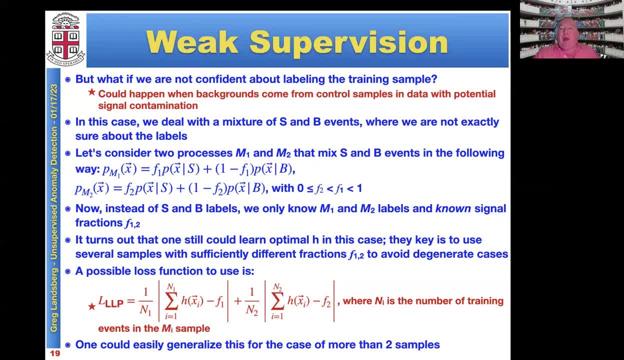 Minus F1. Is The Fraction Of Fraction. So We Know Which Sample We Used, Whether It Was M1. Sample And Two Sample, Because These 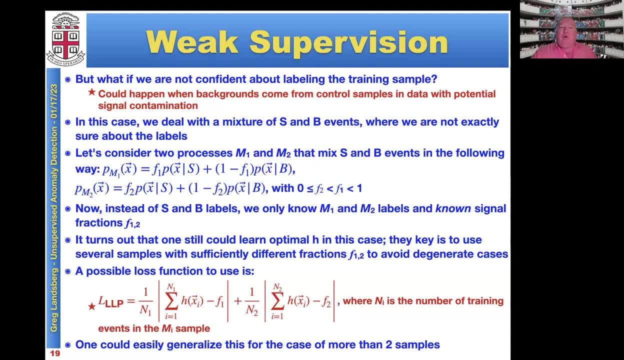 Are Statistically Different Samples, So We Could Label Events As M1.. Which We Could Use To Solve This Problem Is The Essentially The Last Function. 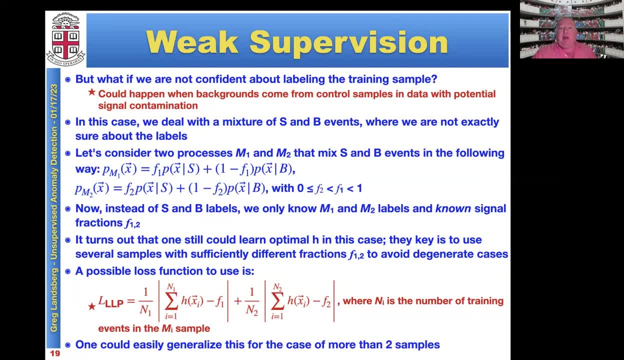 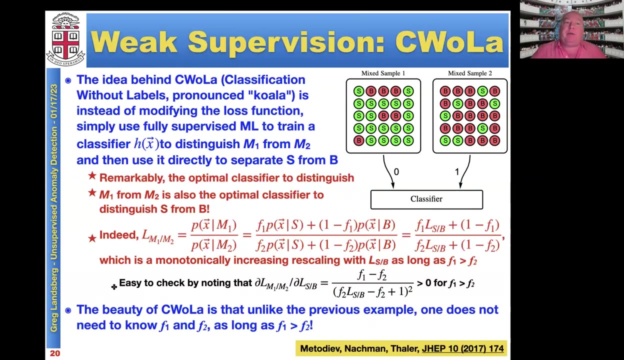 Show Here And One Could Easily Generalize These For The Case Of More Than Two Samples, For The Sample Where You Know Exactly The Labels. 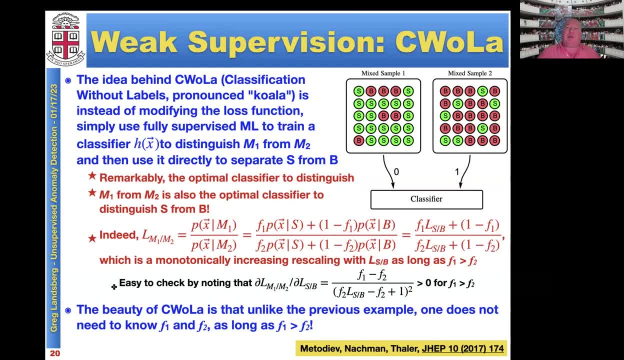 Of Signal And The Background. And This Is The Idea Behind The So Called Classification Without Labels- C, W- That, Remarkably, This Optimal Classifier Is. 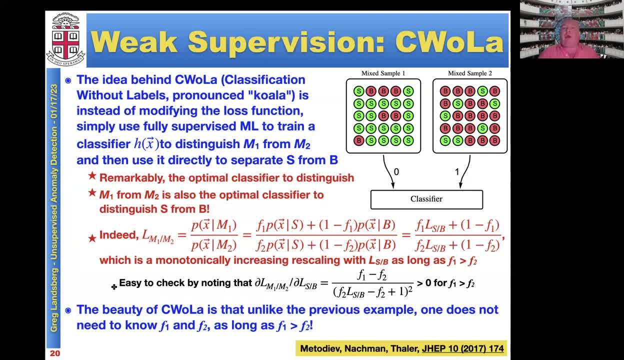 Also Distinguishing Signal Over The Background And We Could Show This Just By Looking At The Last Function For Labels M1. And M2.. Representing 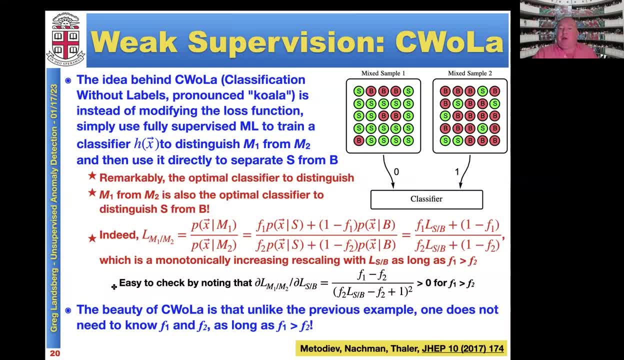 A Likelihood Of S Over B As Long As F1. Is Greater Than F2. And It's Easy To Check That If You Differentiate. 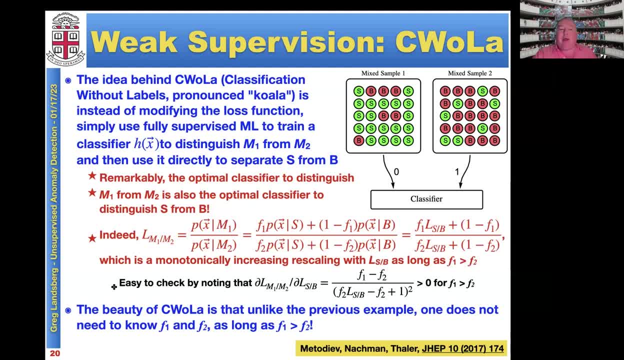 This Likelihood M1.. 2. Over D: M2. And S: M1.. So The Theory Of Quality Approach Is Unlike In The Previous Example One. 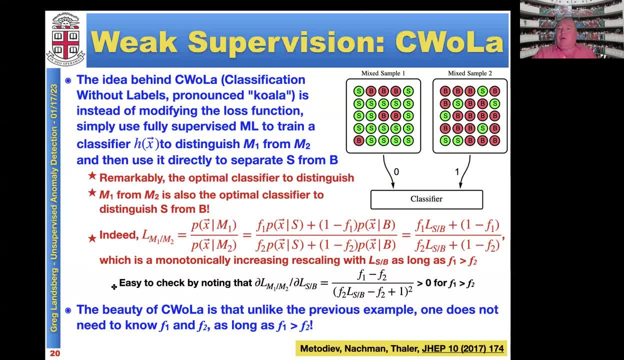 Doesn't Need To Know What F1. And F2. Are As Long As, As Long As You Could Find The Sample Which Have Different Expected. 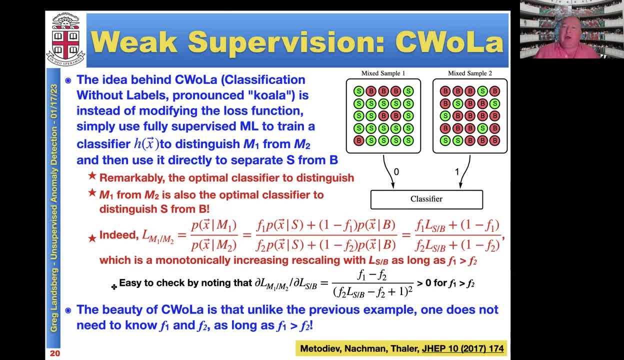 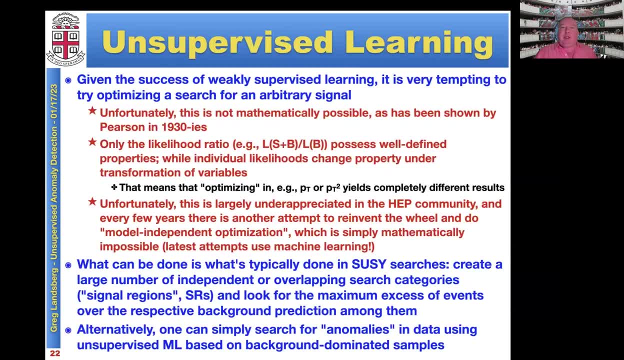 Fraction Of Signal Contamination, Even If You Don't Know Them Precisely. This Big Supervision, The Call A Technique Given The Success Of Weekly 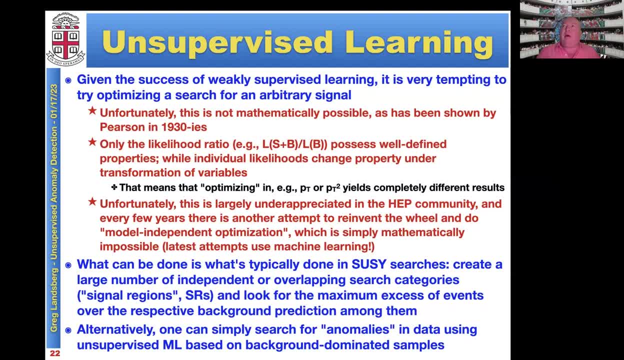 Supervised Learning. It Is Very Tempting To Try To Optimize The Search For An Arbitrary Signal. After All, If I Didn't Need To? 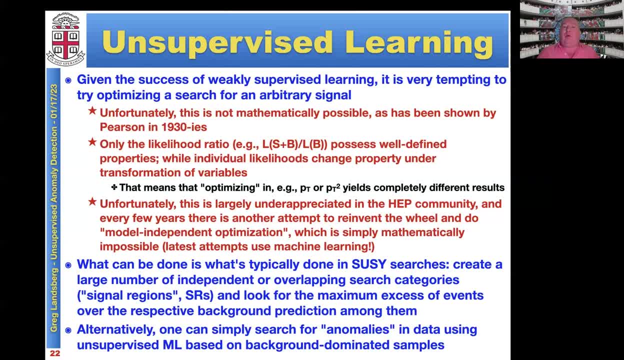 Know What Is The Sign Of Background. Like The Sign Of Background Possesses Well Defined Properties. Individual Like L Of B Essentially Change Properties Under 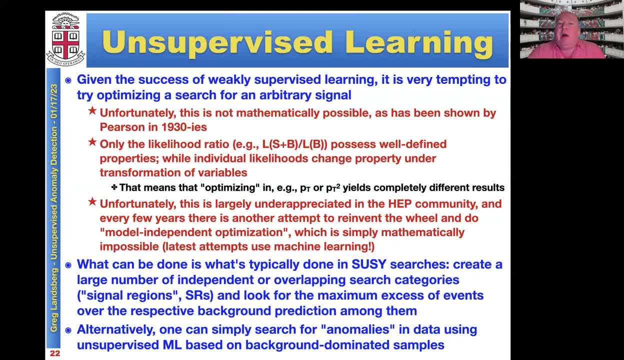 The Transformation Of Variables. So It Is Depending On Whether You Optimize, Say In Transverse, Momentum Of Certain Particle Or The Square Of This Transverse. 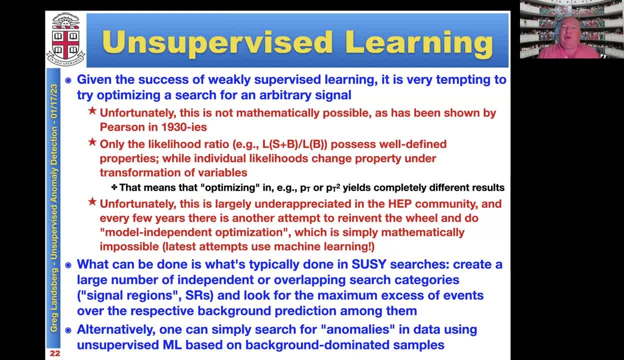 Momentum, You Completely Different Results, Which Obviously Is Nonsense. Of Course Use Machine Learning. So What Can Can Be Done In This Case? How Can? 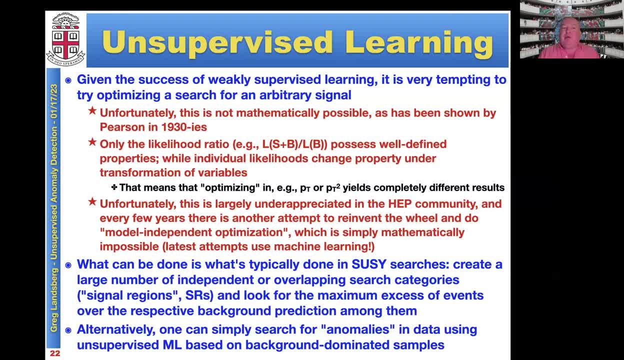 We Do The Machine Learning Which Is Fully Unsupervised In The Sense That Maximum Excess Of Events Over The Respective Background Prediction Among Them. 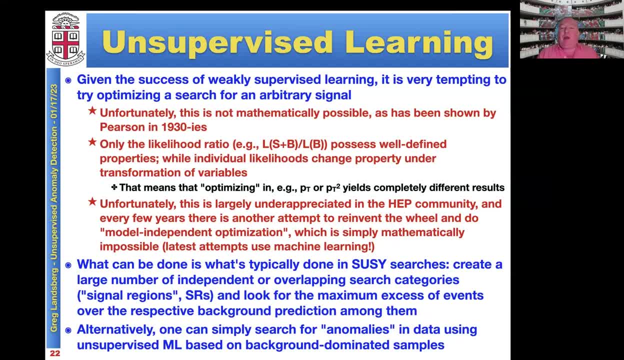 If You Use A Large Number Of This Signal Region, You're Likely Less Sensitive To A Specific Type: Background Dominated Samples, And That's What. 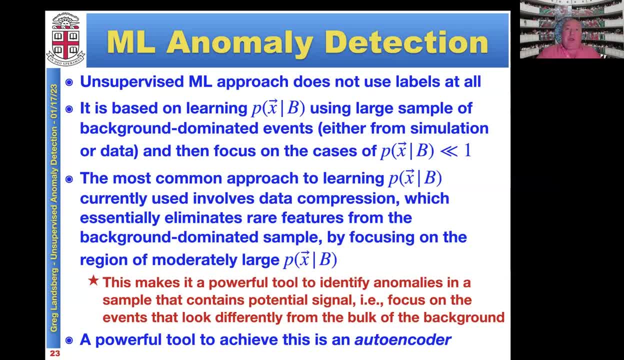 We Are Going To Talk About Until The End Of This Lecture. So What Is The Machine Learned? Anomaly Detection? Well, Unsupervised Machine Simulation. 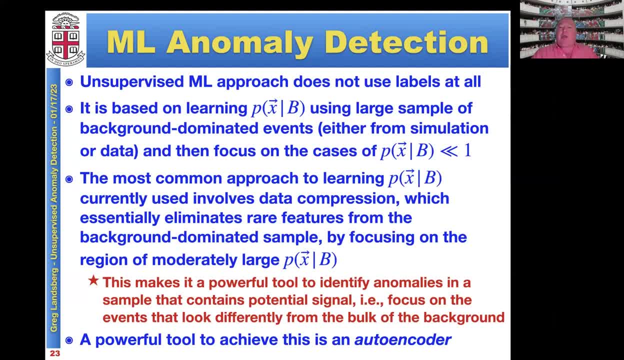 Or From Data. And Then It Simply Focuses On The Cases Of P X B- Much Less Than One. The Most Common Approach To Learning. 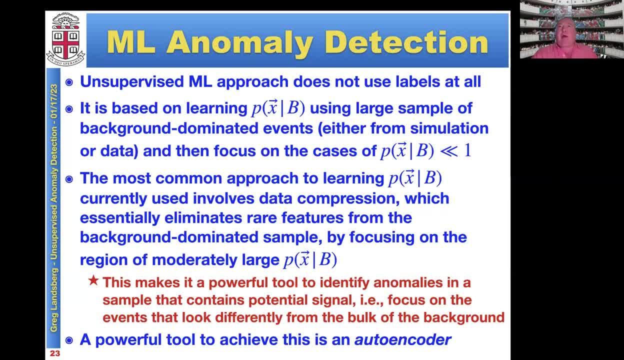 This Probability Density If Your Background Sample Has Small Contamination Of The Signal, If You Compress Information Enough, You Most Likely Won't Be Biased. 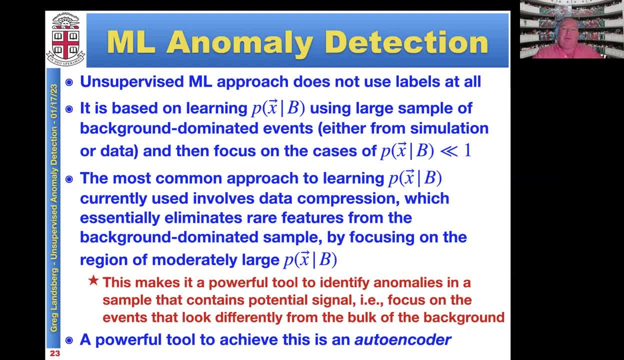 By These Small Contamination Of The Signal And That Contains Potential Signal, Because We Could Then Focus On The Events With Very Low P X. 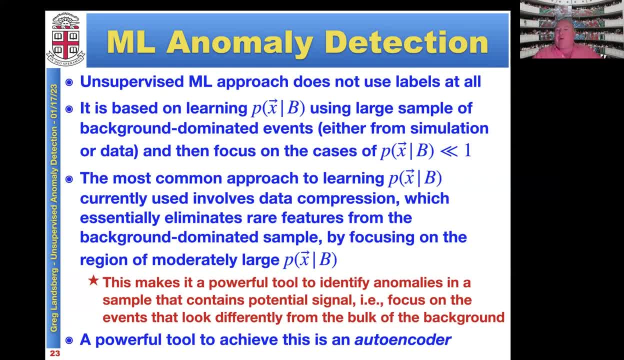 B And Essentially By Doing This We Reduce The Background By Any Amount To Probabilistically Understand What's Going On. But You Could Combine This: 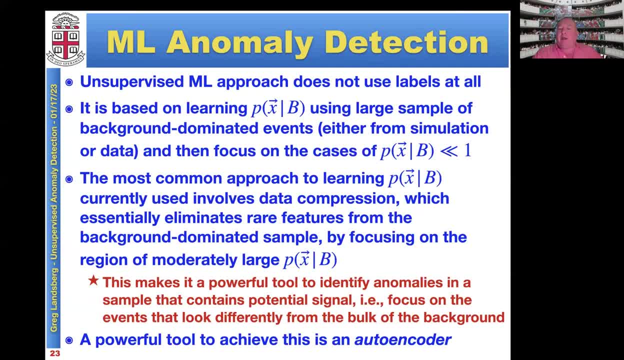 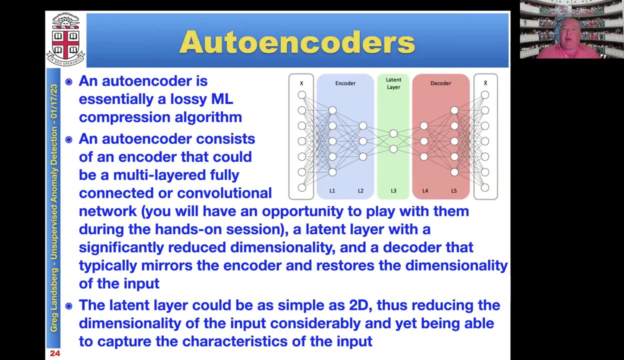 Unsupervised Detection With A Real Ways Of Looking For Signal Using The Other Technique, And That Might Actually Work. What Is The Outer? Encoder Outer. 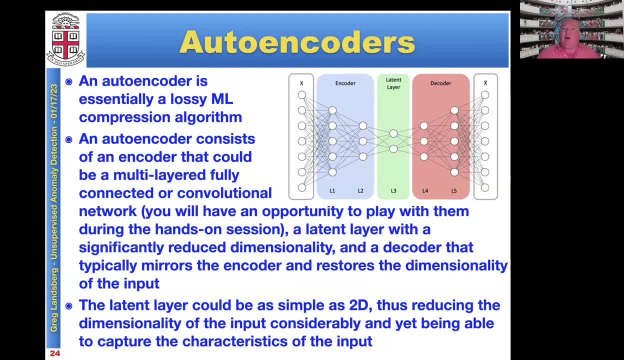 Encoder Is Essentially A Lossy Compression Algorithm Based On Machine Learning. The Architecture Of A Typical Outer Encoder Is Shown On This Slide Decoding. 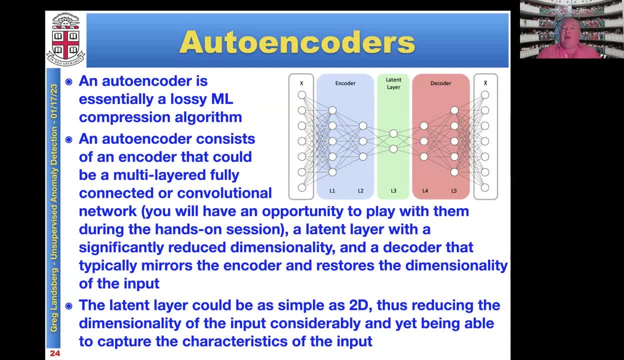 Function Which Essentially Mirrors The Encoder. So The Latent Layer Is The Bottleneck In This Network, And You Could Start With Millions Of Features. 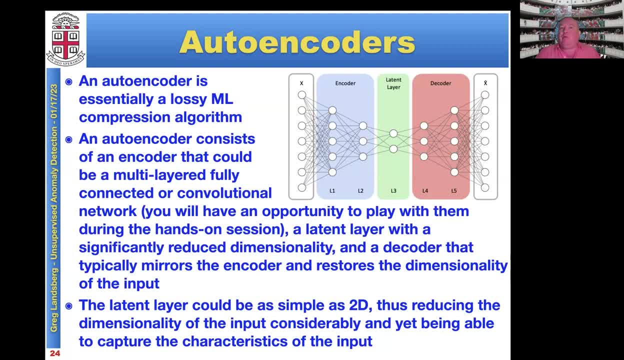 Such As Properties Of The Input X In A Low Dimensionality Latent Space, And Then You Decompress It And You Get The New Set. 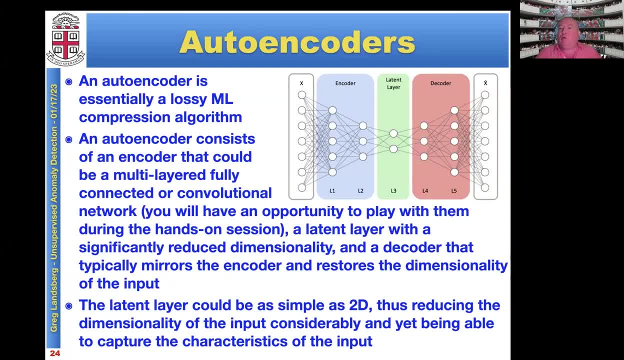 Of Observables X Head And The Idea Is That You Have A Dimension To Low Dimensionality Latent Space And Then Decoding It To The 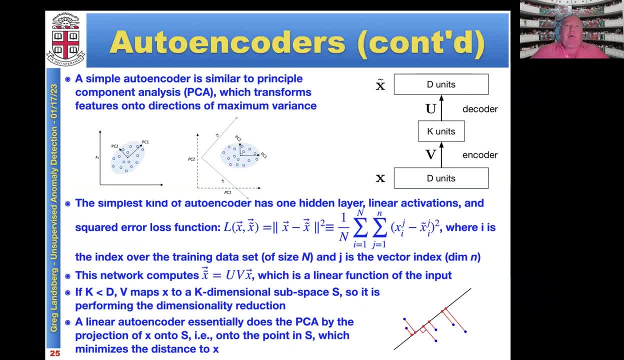 Full Dimensionality Space Of Feature. So Let's Look At Some Of The Examples On How This Is A Variable In Variables X1. And X2.. 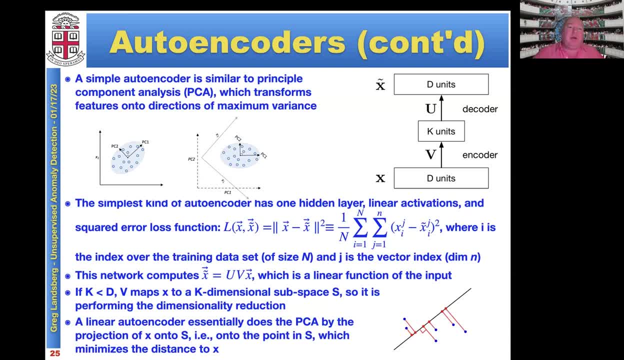 Which You See On The Left Graph. The Principal Axes Are Pc 1. And Pc 2., Which Basically Resemble The Large Semi And Decoding. 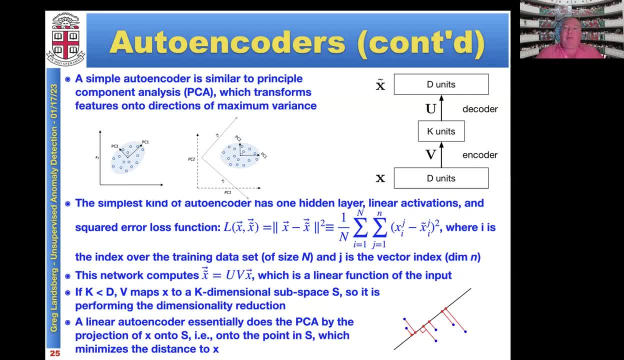 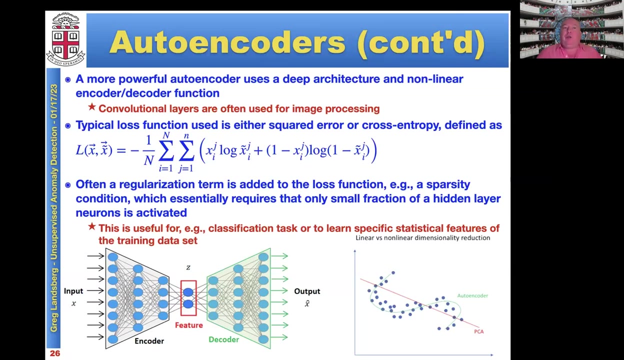 Function. Essentially Does This Principle Component Analysis In More Complicated Out In Quarters Which Do Not Have Linear Activation Functions, Which Could Have Long Linear 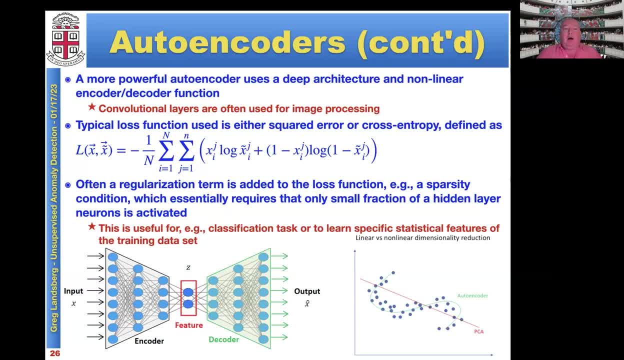 Activation Functions Do. Sometimes These Layers Could Be Convolutional Networks. This Is Often Used For Image Processing Or Image Compression, And The Typical Loss Function 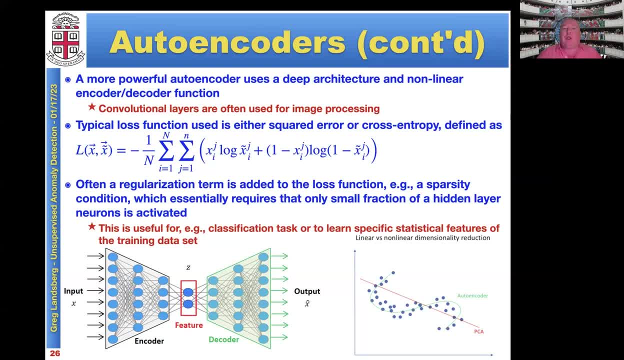 Used For Out In Quarters Is The Big Plots. So You Maximize, You Minimize The Loss Of Information When You Go From X To 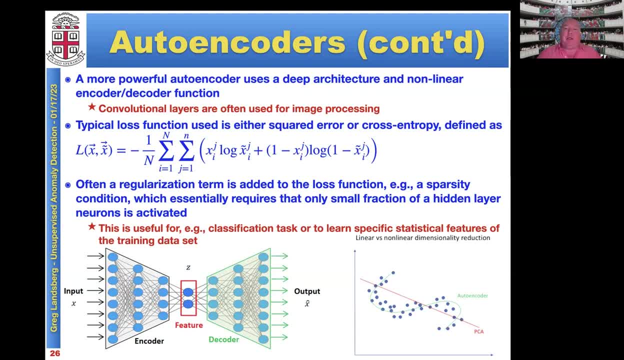 X Tilda Or X Hat. Sometimes People Also Add Begalization Trends To, For Instance, For Classification Tasks Or To Learn Specific Statistical Feature Of. 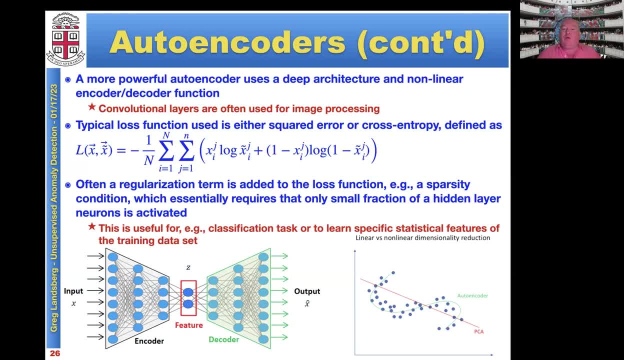 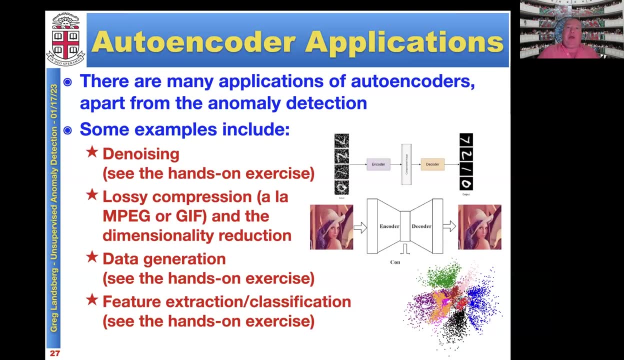 The Training Data Set. And You See On This Example That, Unlike The Principal Component Analysis, Which Is Different Applications Or Encoders Apart From The 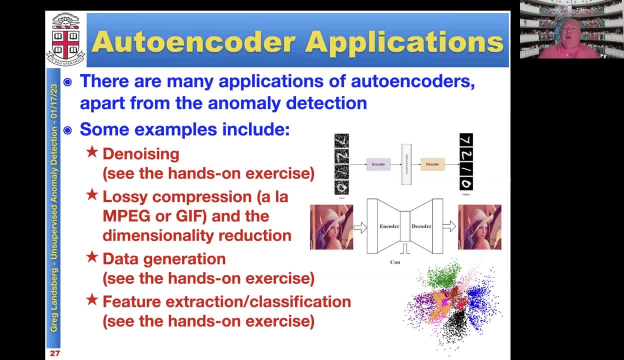 Normally Detections. Some Examples Include Denoising. You Take The Image Which Has A Noise, Editing You Encoded, You Decode It Magically. Noise Is. 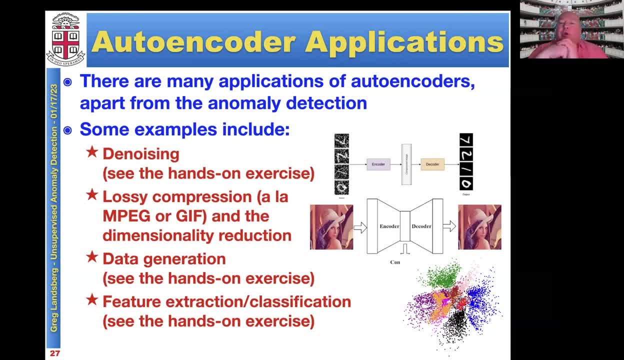 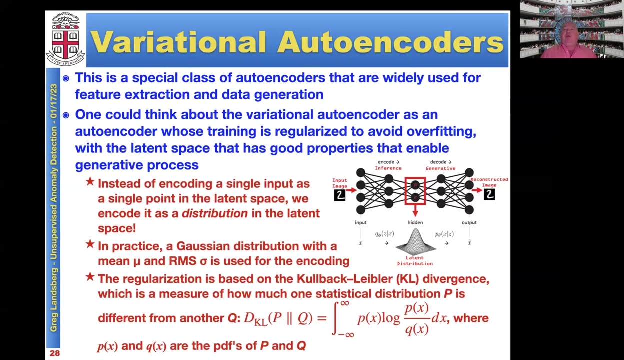 Not Based On Machine Learning, But You Could Do It While Machine Learning Techniques. This Could Also Be Used For Data Generation And We'll Talk. 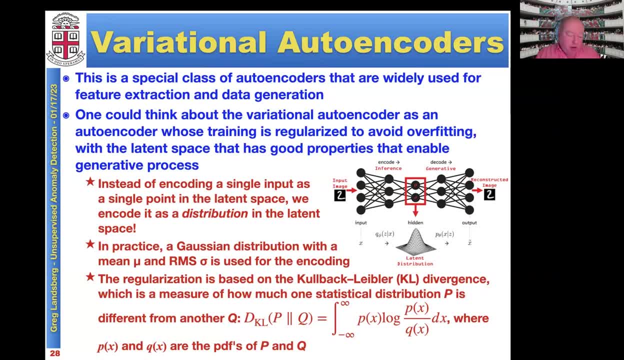 About This For One Encoder. This Is A Special Class Which Is Widely Used For Feature Extraction And Data Generation. One Could Think About Variation. 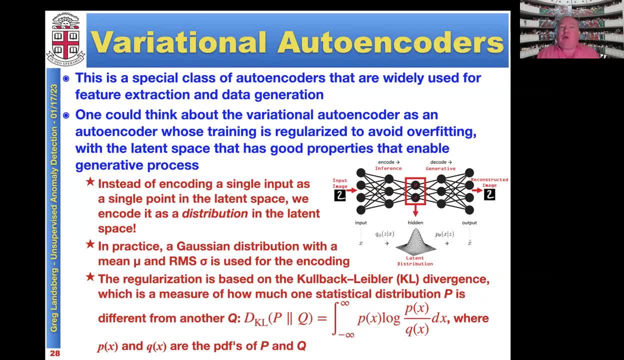 Out Encoder As A Regular Out Encoder Whose On To Two Similar Features, And This Could Be Achieved By Using A Special Loss Function When 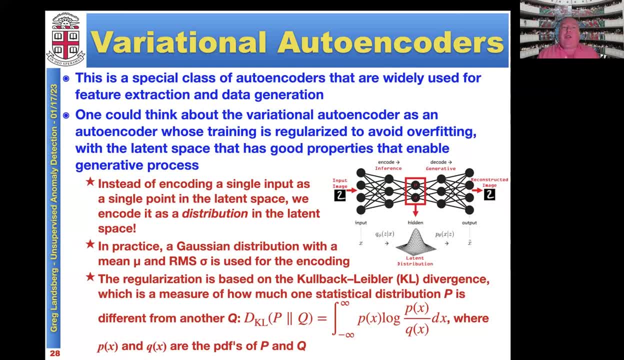 You Essentially Deal With The Training Of The Out Encoders And By Essentially A Distribution With No Parameter In The Latent Space And In Practice. 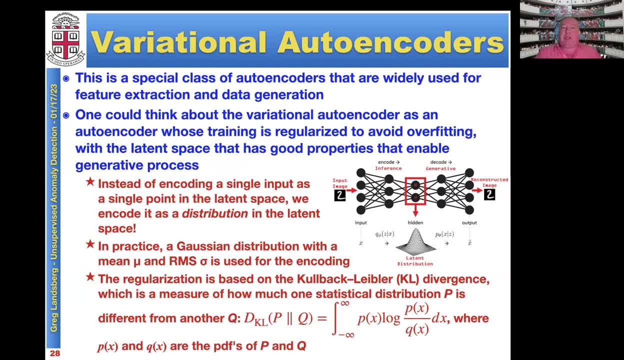 Typically A Gaussian Distribution With The Mean Mule And RMS Sigma Is Used For The Encoding The Legalization Term Which Is Added To Train This. 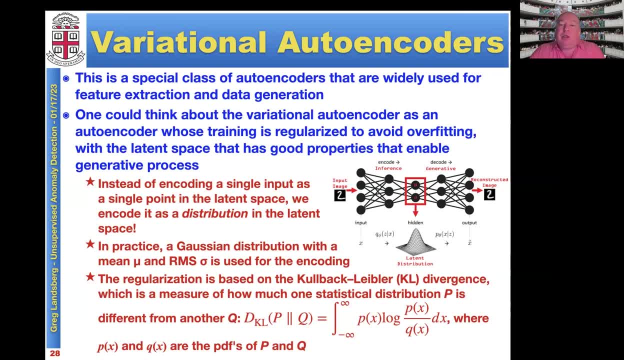 Out Encoders Is Based On The So-called Kubik, Leibler Or KL Divergence, Which Is Very Often Used In Machine Learning Approaches For 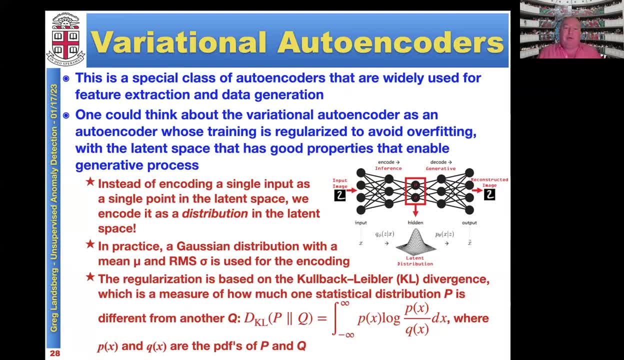 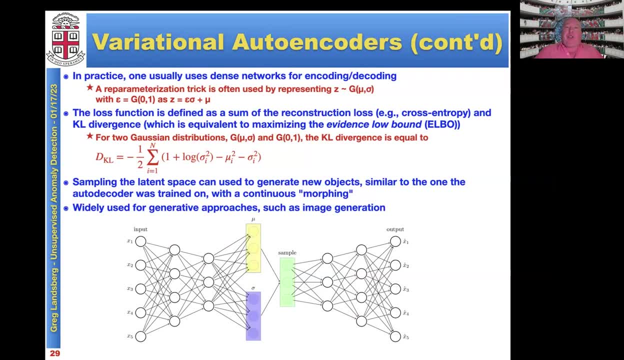 Distribution Of Big P And Big Q. In Practice One Usually Uses Dance Networks For Encoding And Decoding, And Typically People Use The Reparameterization. 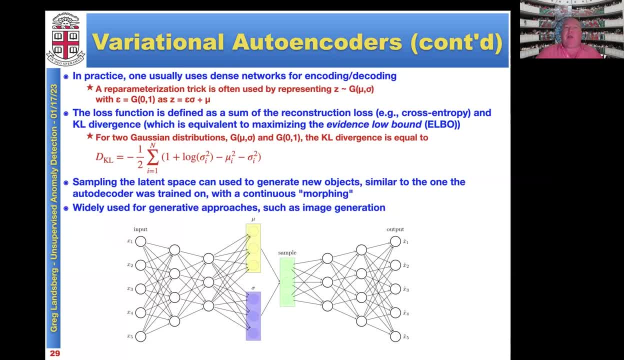 Trick By Representing, By Replacing And Then Transforming One Gallus Into Another, Through This Linear Equation And The Log Function, The Lost Functions For 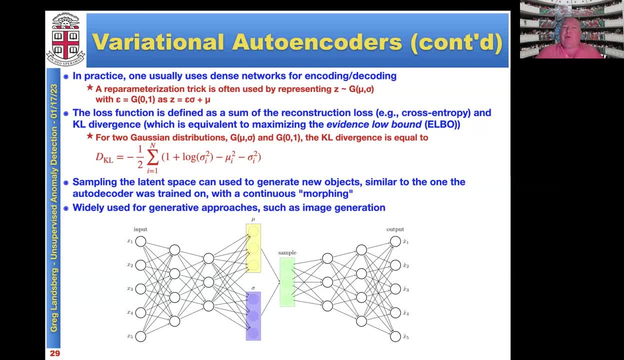 These Out Encoders Is Typically Some Of The Reconstruction Loss And The Divergence Is Given By This Form Over The Points And By Minimizing. 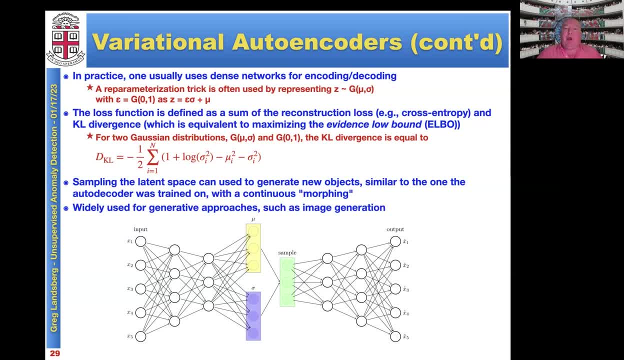 The Loss, Which Is Some Of The Reconstruction Loss, And This Decale Loss You Essentially. You Train Out Encoder And Then You Take A Random. 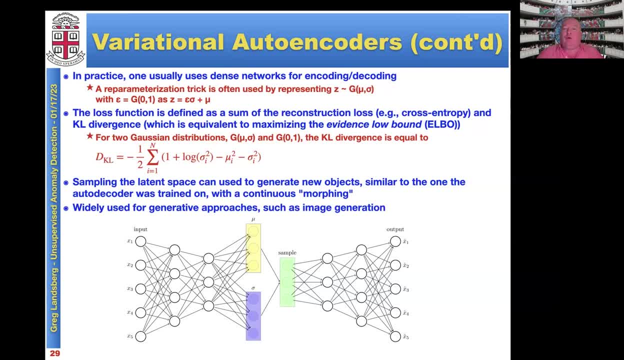 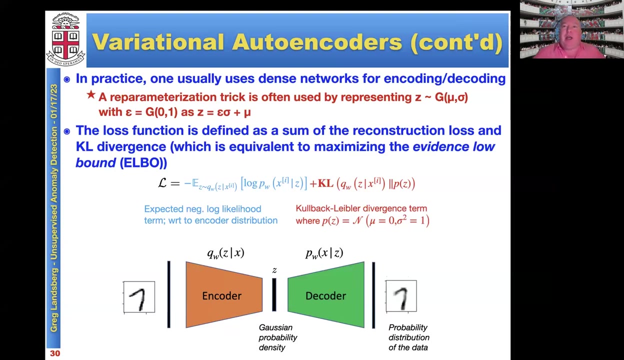 Point In A Latent Space And Run Decoder On This Point To Find A New Image, And This New Image Features. This Is How The 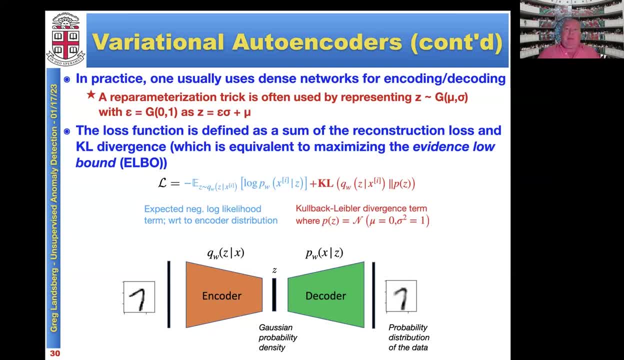 Image Of The Cap Which Looks Like A Poodle Was Generated On The First Slide. So Basically, We'll Learn A Little Bit About Variational. 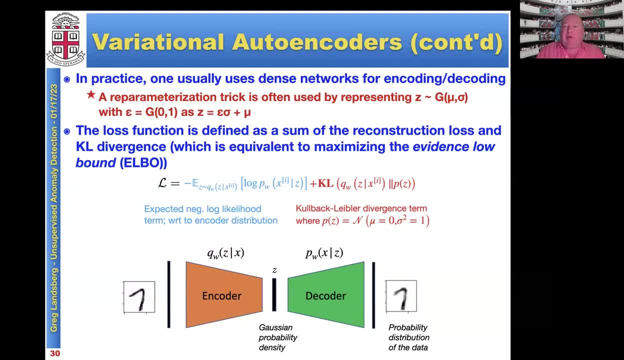 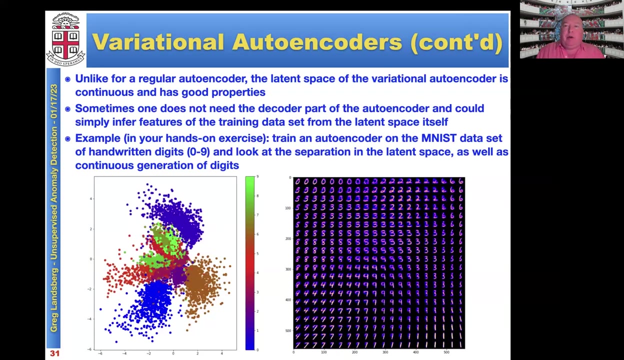 And Particle Physics. I Actually Have Several Examples In The Talk, But I'll Focus Just On One Example Which Shows You How To Avoid This. 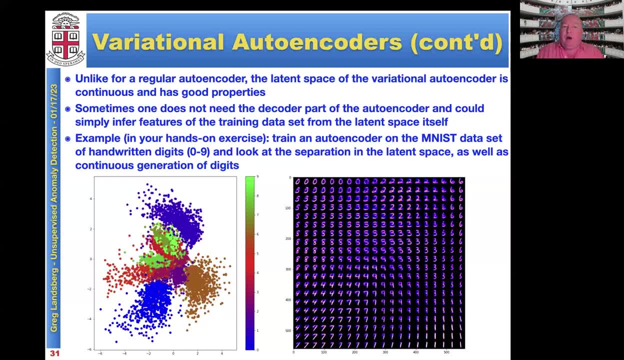 Problem Of Optimizing Against Through The Hands-On Exercise. So What You See On The Left Is Actually The Picture Of The Latent Space Where 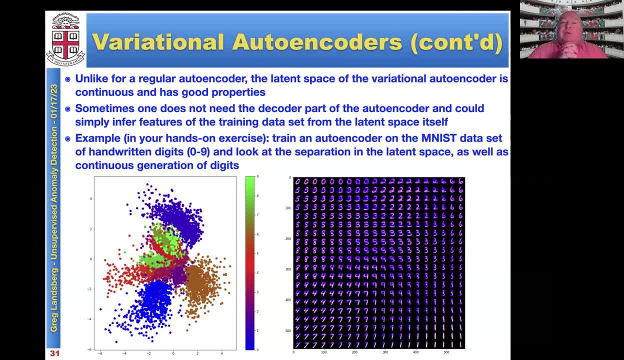 You Train. The Outer Encoder On The Large Sample From Zero To Nine Are Clearly Separated In Different Blobs In This Latent Space And 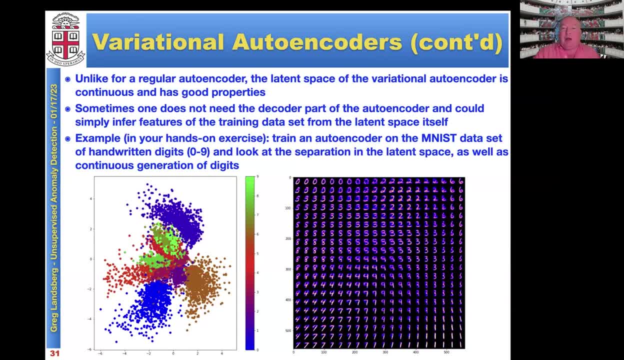 If You Take A Random Point In This Latent Space, You Could Start Generating Aspects Of The Outer Encoders, Whereas In The Areas Where 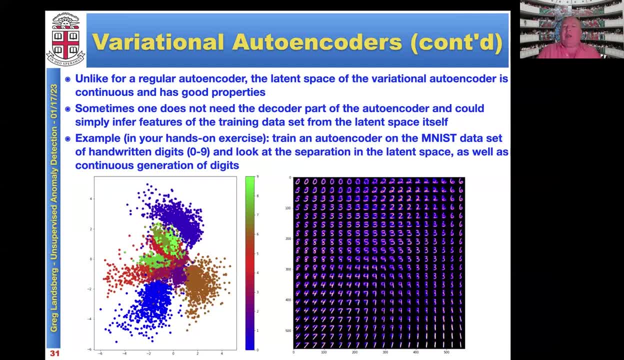 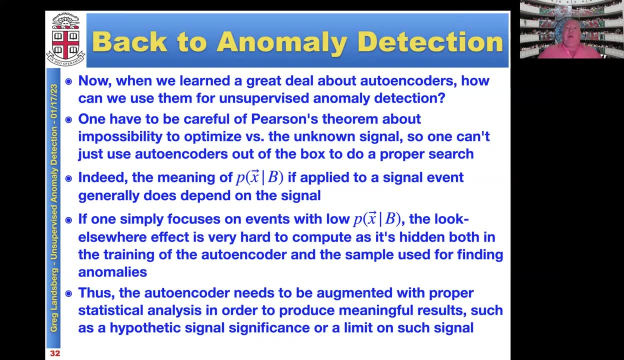 The Blobs Are Not Overlapping, You Typically Get Something Which Looks Very Much Like The Images On Which You Encoder. Is How We Practically 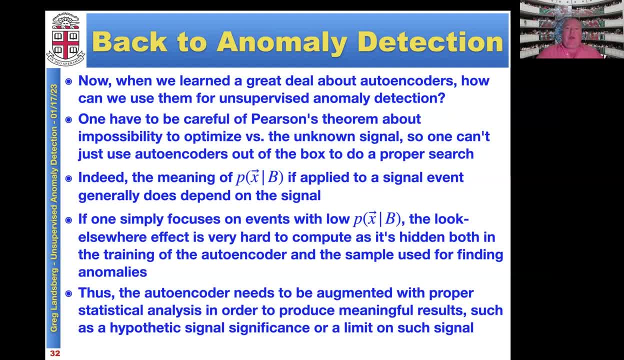 Use Them For Unsupervised Anomaly Detection To Avoid This Pearson Theorem Pitfall. Well, Essentially, What It Means Is That We Focus On Events. 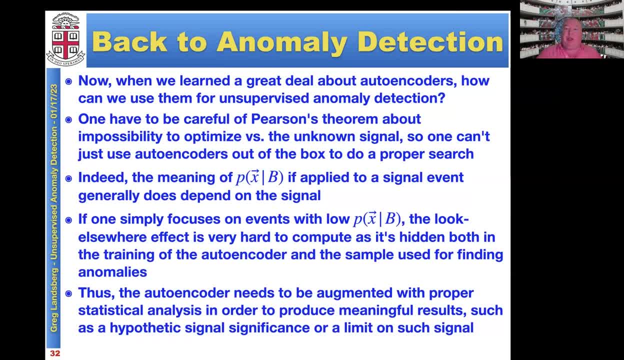 With Low Some Signal Against The Background. But The Way We Use Unsupervised Anomaly Detection Is Simply To Remove Large Chunk Of The Background. 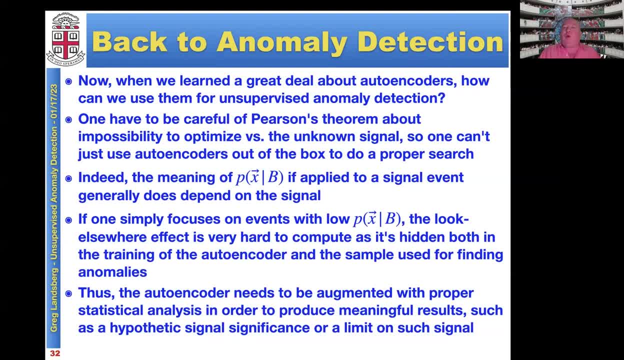 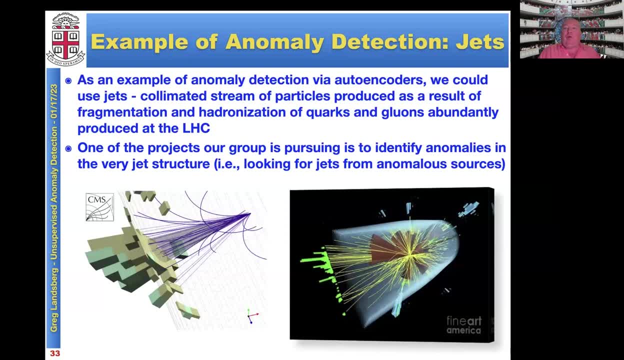 So We Increase The Purity Of The Sample Of This Is What We Are Trying To Do With Brown: Mainly Anomaly Detection Of Features. 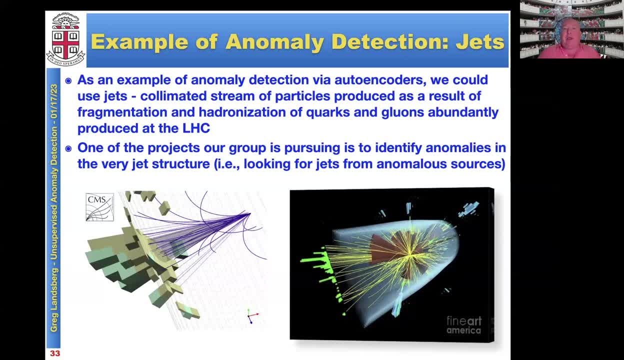 Of The Jets Which May Not Be Caused By No Sources, May Be Caused By Some New Physics Or Some Detector Malfunction, But Essentially 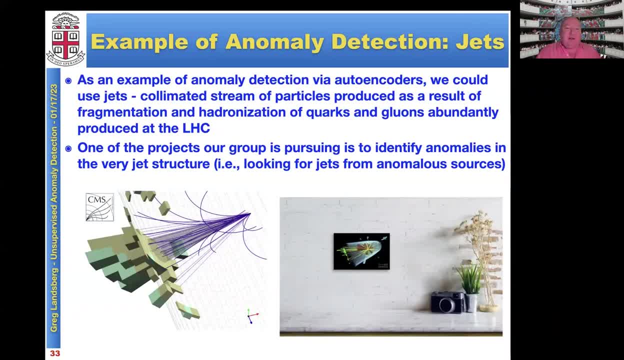 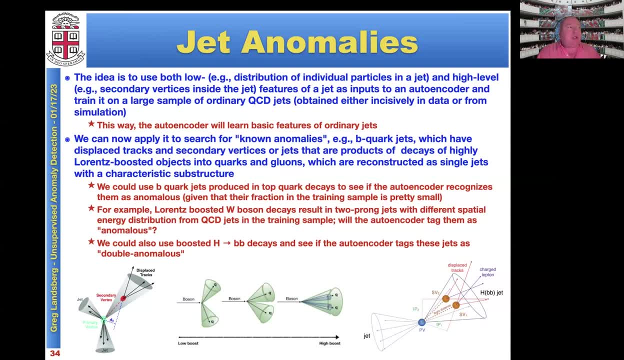 What We Want To Do Is To Find The Jets Which Don't Look Like A Regular Jets From Q, C, D Processes. So This Way: 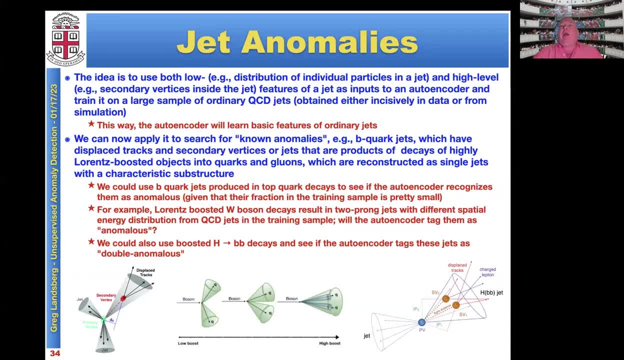 We Could Train Out Encoder On The Properties Of Ordinary Jet And Then Apply Them To Jet And Data And Look At Inside The Calorimeter. 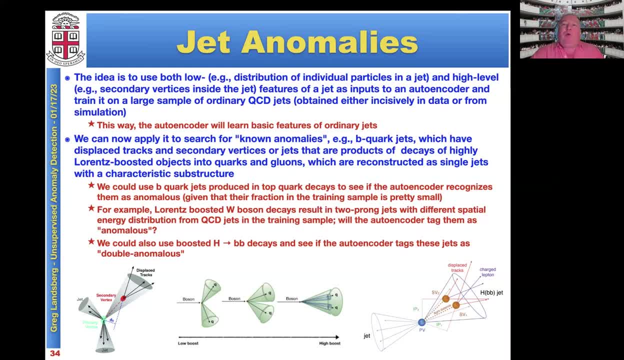 Of The Particle Detector Or Something Else, And The Way We Could Actually Understand That Our Anomaly Detection Does. The Right Thing Is That We 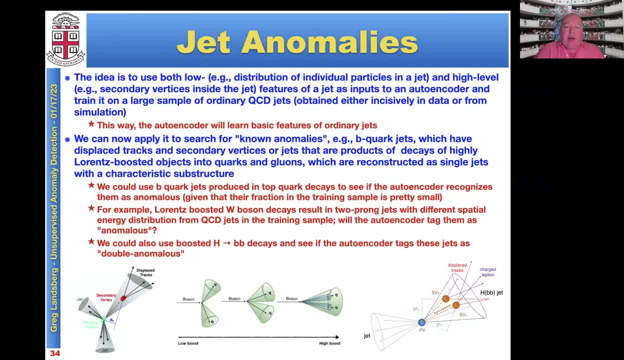 Could Do And We Could Understand That The Particle Of The Calorimeter And The Particle Of The Particle Of The Particle, So The Particle Of 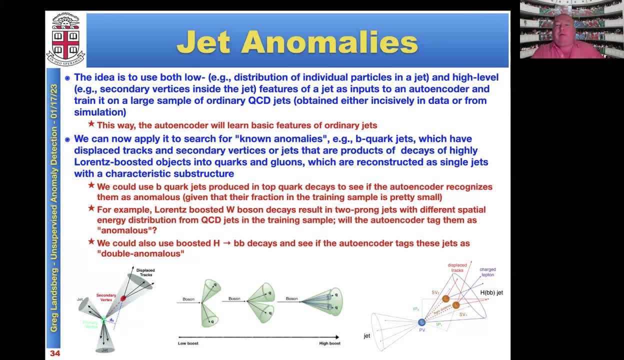 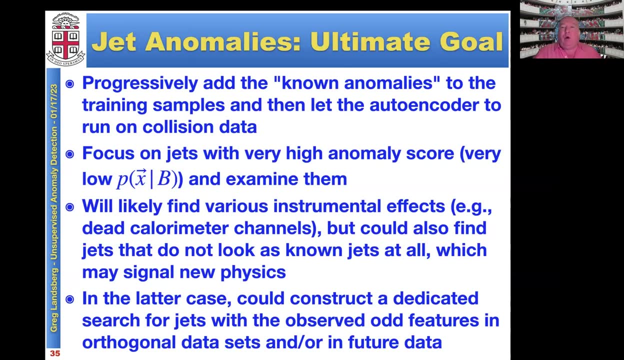 The Particle Is A Structure because it has both two centers of gravity and these displaced tracks and secondary vertices. And just to show you, and essentially the idea would be to progressively add the known anomalies to the training sample until we run out of all the known anomalies, 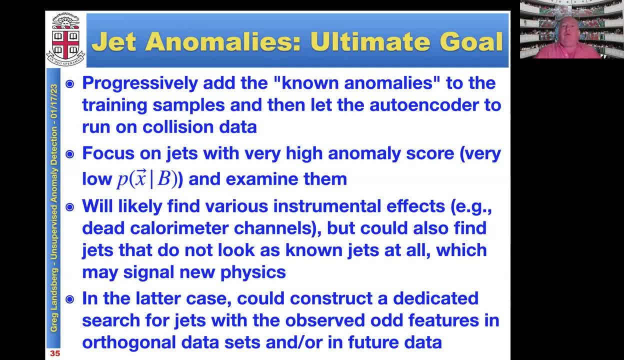 and then let our encoder to run on the collision data and find the events which do not look like ordinary jets, And then one could either construct dedicated search by examining feature of these events, or one could identify some malfunctions in the detector and be used in real time as the data quality monitor tool. 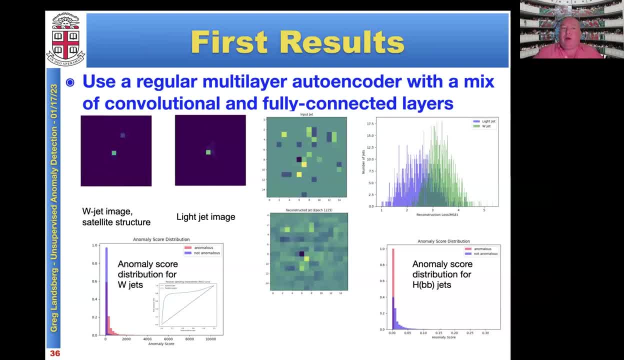 So the first things we did is training the autoencoder on these jets from QCD and then applying them on jets from the decays of boosted W boson. You see that the W boson jets have two centers of gravity. this blob on the left. 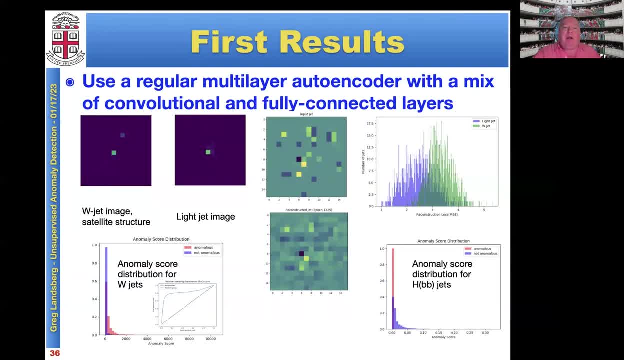 and this blob on the right. The light jet has a single center of gravity. The middle set of plots is your typical input jet and then the decoded image of this jet through the autoencoder And then, if you look at the anomaly score between, say, W jets and QCD jets, 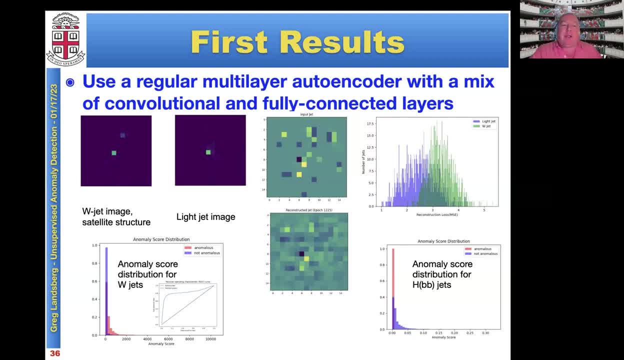 you clearly see that the W jets are recognized as anomalous because the pink distribution is much wider than the blue distribution, which is the the jets typical to the training sample. So that's an example of how the encoder would look for anomalies, although it never was trained on W type of jets. 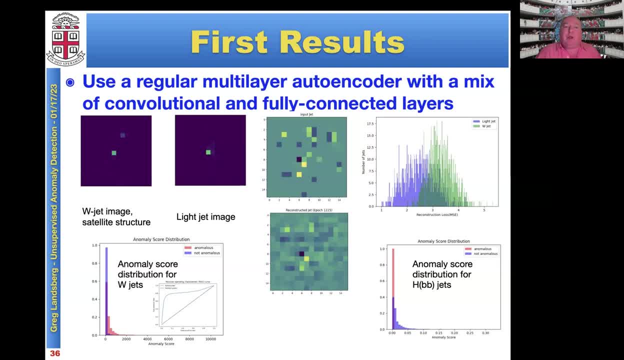 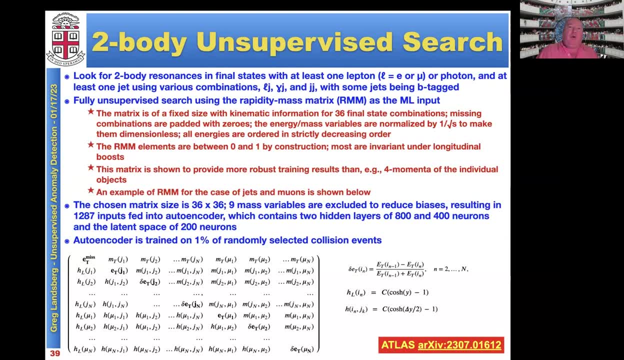 it nevertheless recognizes them as being different from the jets on which it was trained. And one example of this search for the search which was just published last summer by the Atlas Calibrations, is essentially the search. they look for two body resonances in final states. 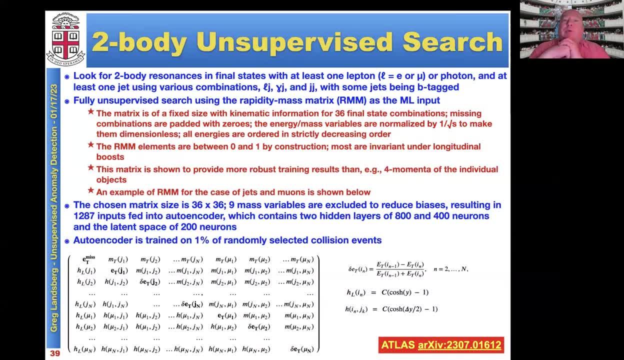 which has at least one lepton or photon and at least one jets. So what they did? they look at different configurations, say invariant mass of a lepton and a jet, or photon and a jet or two jets, And some of these jets may be even identifying. 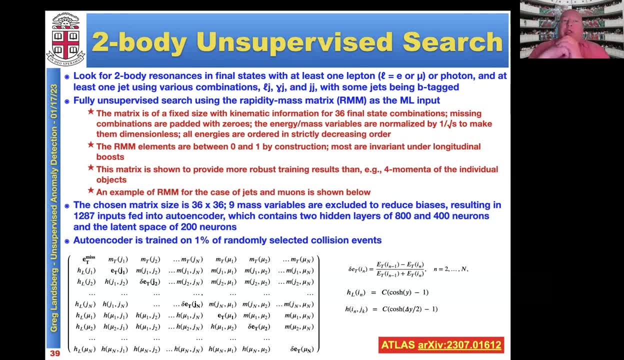 as B type jets and B type. So this is a fully unsupervised, unsupervised search which uses the so-called rapidity mass matrix, which is a certain way of parameterizing kinematic properties of leptons, jets and photons. in the event. 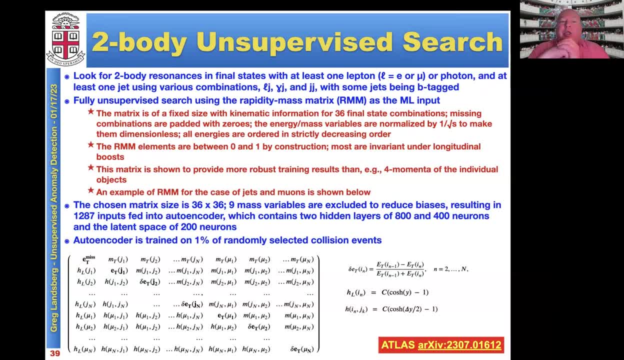 I won't go into detail of this, but essentially it uses either Lorentz invariant or close to Lorentz invariant variables, which makes sense because basically we expect that new physics does not depend on the boost of the system. So if you train your network on variables, 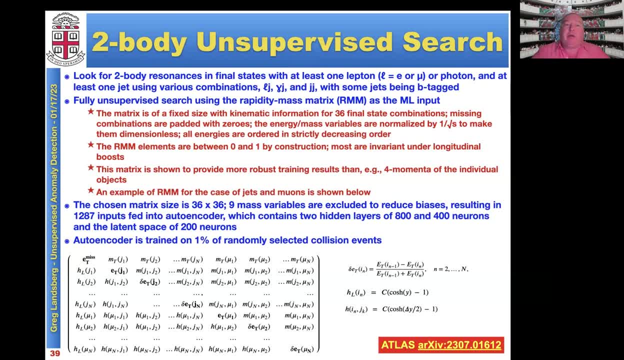 with good Lorentz invariance properties you make the network much more robust And essentially the chosen matrix was have a size of 36 by 36, with a few elements set to zero, And that was nearly 1300 inputs. 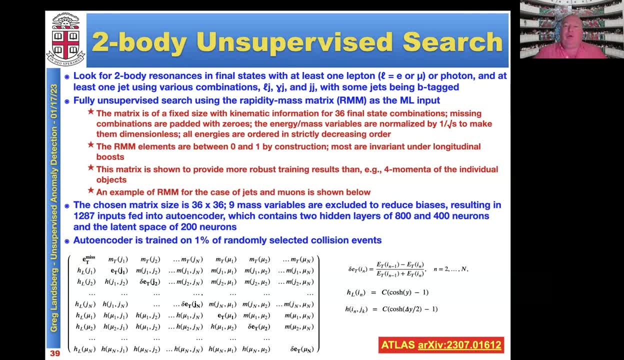 which were fed in the autoencoder, which contained two hidden layers of 800 and 400 neurons and a latent space of 200 neurons. So the dimensionality reduction was about factor of six. You go from 1300 inputs to 200 dimensionality. 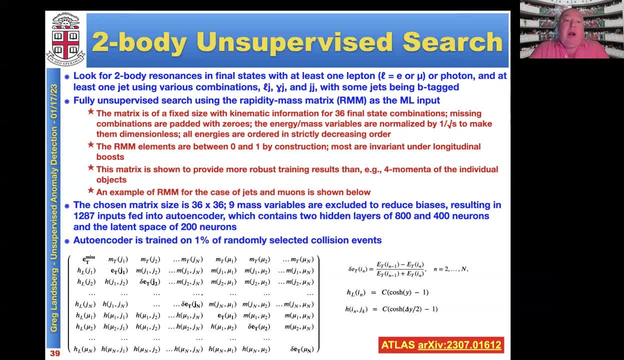 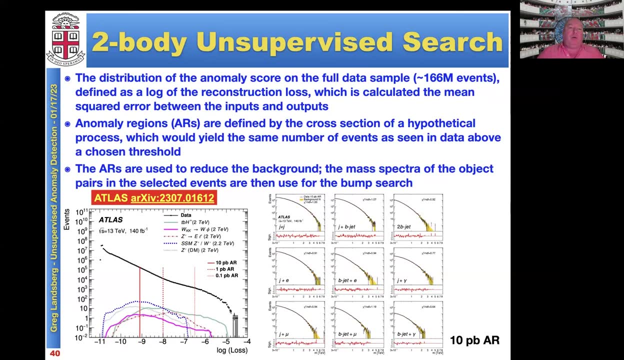 of the latent layer. Then you train on 1% of randomly selected collision events and you apply this autoencoder to 99% of the events And if you do so, you see the distribution of anomalous score which is shown on the bottom left. 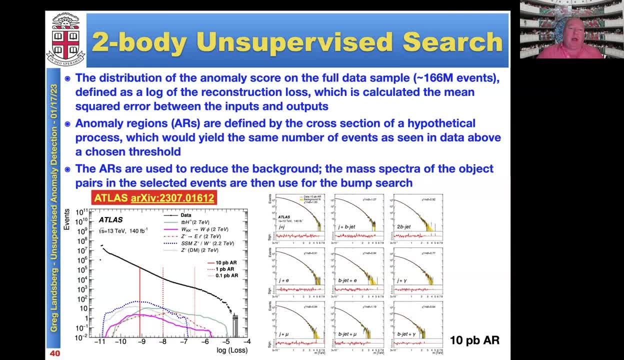 So it's a log plot. So you see that most of the events have anomalous score, which is low. Here the anomalous score is defined as a logarithm of the reconstruction loss, And reconstruction loss is the mean squared error between the input variable and the output variable. 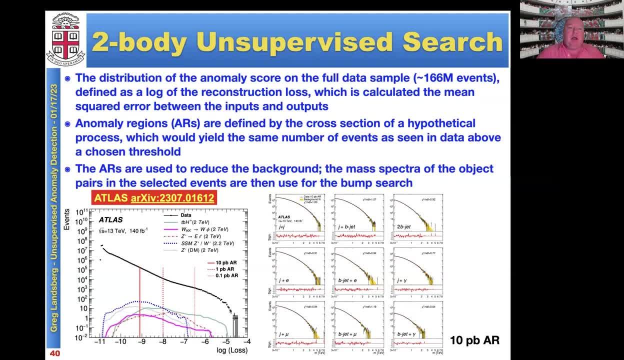 of the autoencoder, just as an example we discussed, And by looking at this distribution one could cut on the value of this anomaly score At certain levels. they chose to cut at about minus nine, which happened to correspond to effective cross-section. 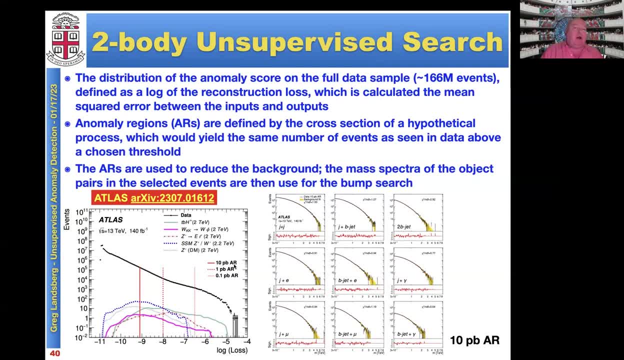 of the events above this region of about 10 picobar. So you would be sensitive to signals which have cross-section of the order of 10 picobar, But they also consider it a more restrictive regions if you cut at 10 picobar. 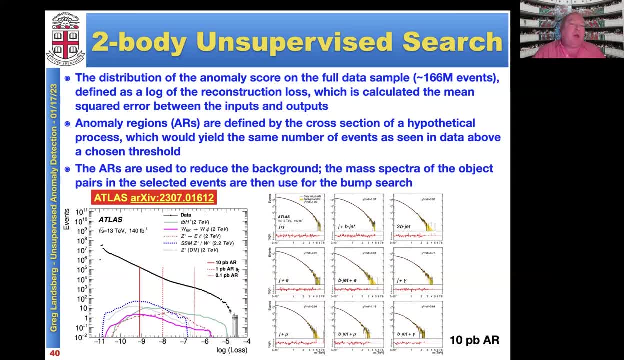 At eight minus eight you get to something called one picobar signal cross-section. And if you cut even harder you get to 100 femtobar cross-section. So by changing this cut you can look for more and more rare processes by reducing the backgrounds by many order of magnitude. 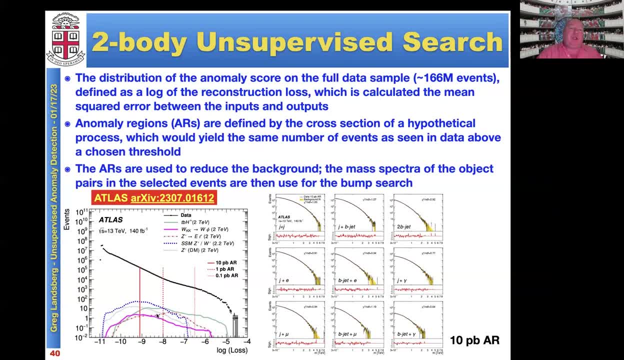 And at the bottom you see how different new physics models- hypothetical new physics models- look at this anomalous score And in general you see that they have longer tail in the anomalous score compared to the data, which is dominated by standard model backgrounds. 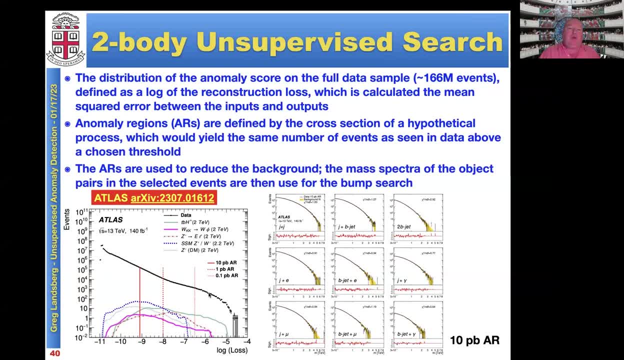 So how do you transform this to a real distribution? Well, you select a cut on the anomalous score and then you look at the invariant mass distribution of these different pairs of objects and you look for any bumps in this distribution. So the right-hand plot is the input to a fully supervised search for signal. 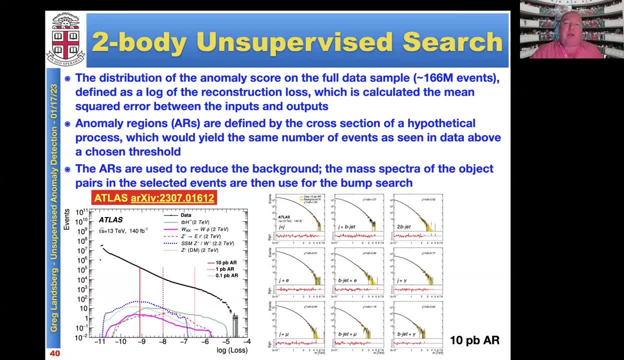 You inject the signal and you see how much signal you could inject at any given mass in order to not violate the data. So this is a fully supervised search, because you inject specific type of signal and essentially you don't even optimize against the background. 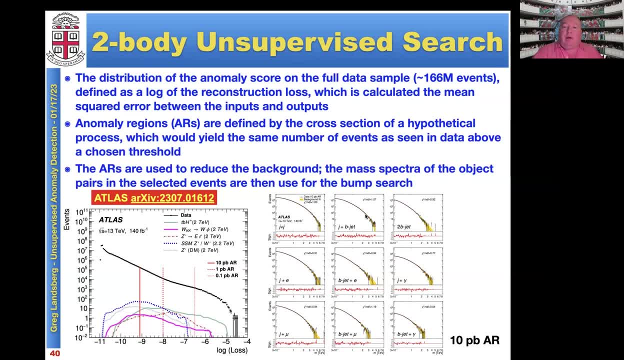 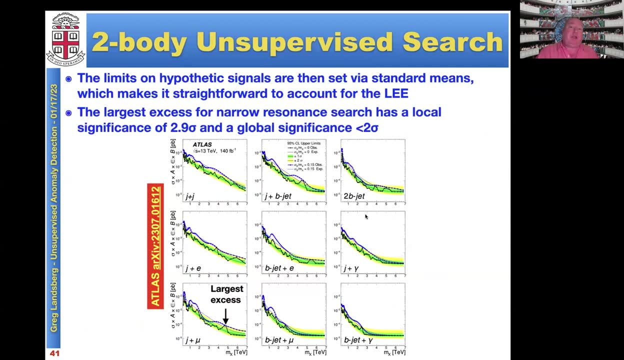 You just find the largest, The largest signal you could still add to the background in order not to violate the observed data, and you set the limit on the signal strengths or on the signal cross-section by doing this, and that's precisely what they did. 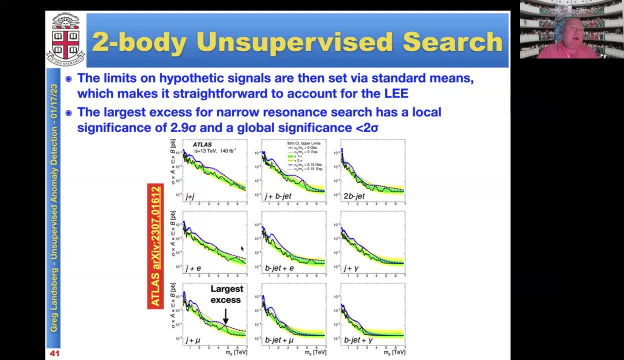 They set the limits on the various type of resonances which could decay in a pair of jets, or a pair of a jet and a photon, or a jet and a muon, and the largest excess Out of these many areas is found in the invariant mass of jet and muon. 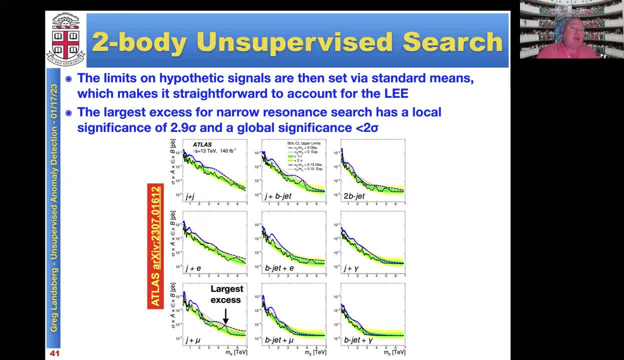 and it's just below three sigma. But since you looked at so many places, the trial factor is quite large. so the global significance of this excess is less than two standard deviations. so there is no indication of new physics. but that's an example how you could combine the unsupervised anomaly detection. 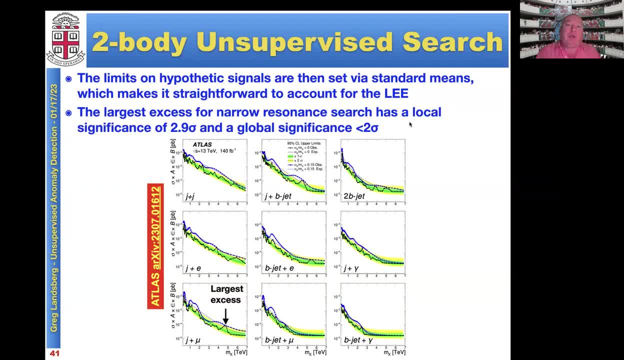 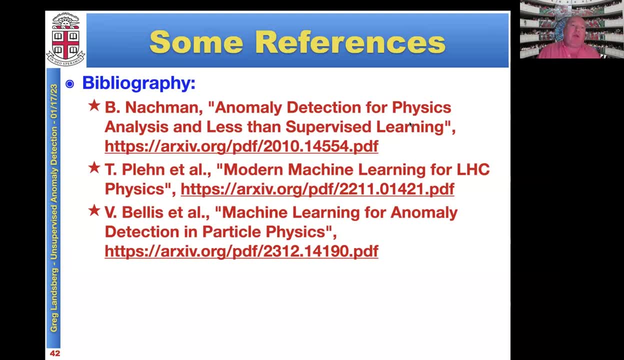 with the fully supervised Search and use. the first step is just a very strong background reduction tool and I guess I'll stop here. I will give you a few pointers to the various articles on the machine learning. You could access all of them. 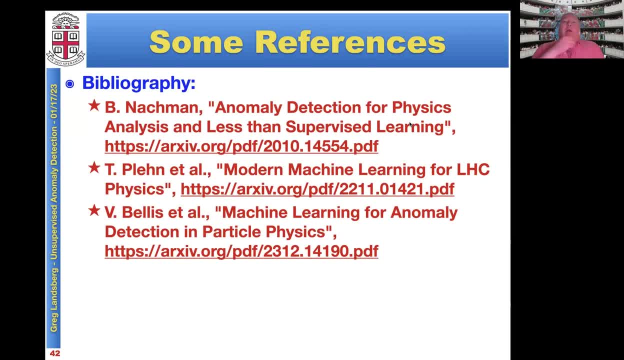 You see that most of them are very recent- 2020,, 2022, 2023, and you have more pointers in the handout. and you have more pointers in the handout out for this course, and that brings us to the exercises. 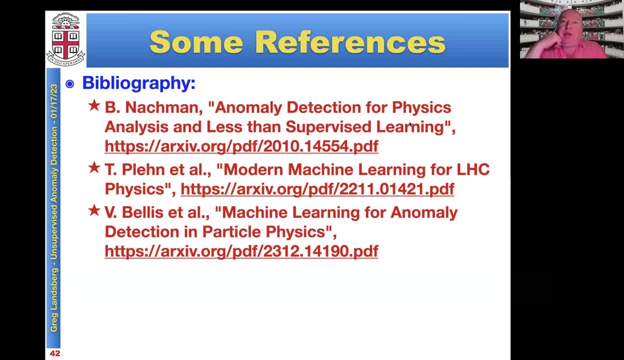 So at this point let's take any questions and then let's make a five minute break and then work through a few exercises using the Python notebook. Thank you, Greg. thank you very much. Don't be shy, Just ask questions or raise your hands. 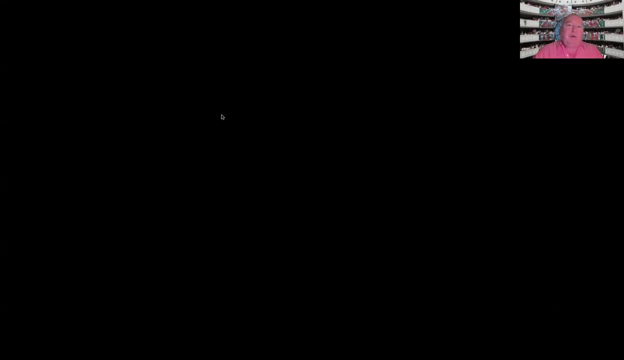 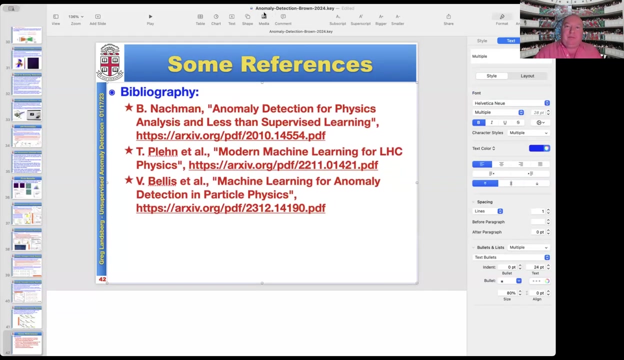 And I'll go from the full screen mode to the other mode so that I could see the questions. We did have one question concerning videos, which is, yes, we will be making videos available from the talks And the workshop exercises. they will be available as soon as we can. 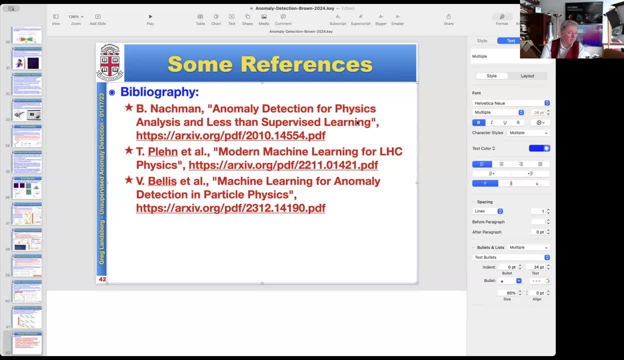 edit them and get them posted back up again. Good thanks, Don't be shy, guys. Questions: Everybody is keen to try out encoders themselves. All right, Now think about in this next five minutes of a break, think about some questions. 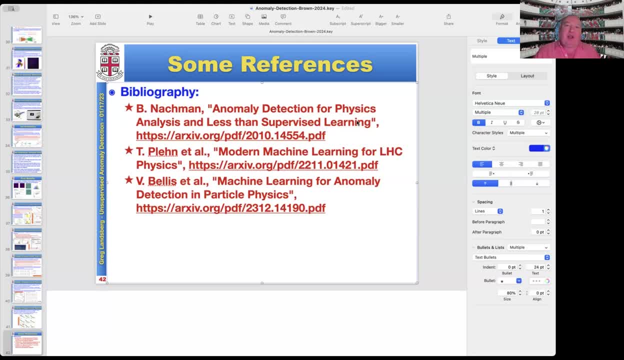 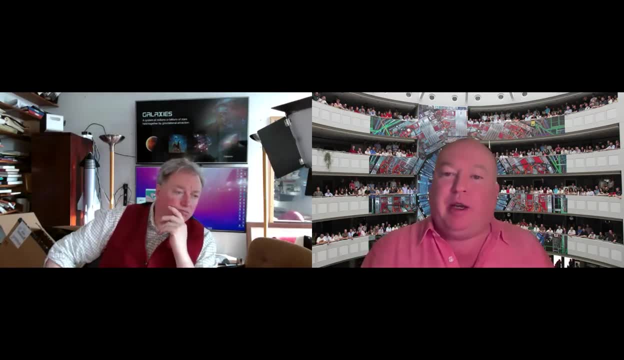 If you have them, then we come back. Let's do this And I'll stop sharing at this point. We could stop the video and then in five minutes we'll resume with the hands-on exercise. I hope by now you all have an account. 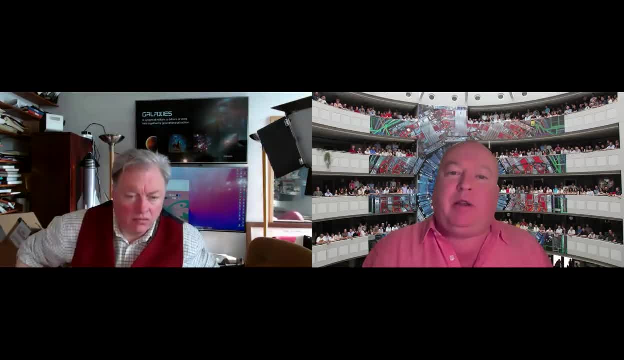 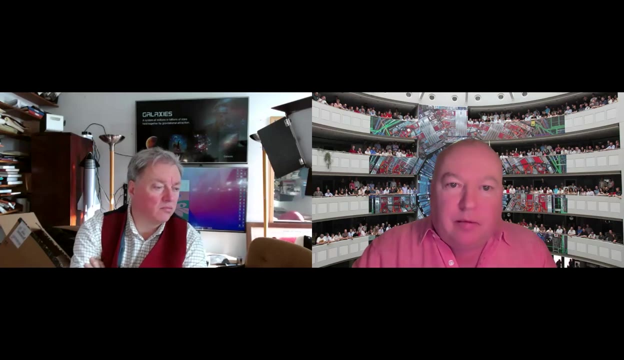 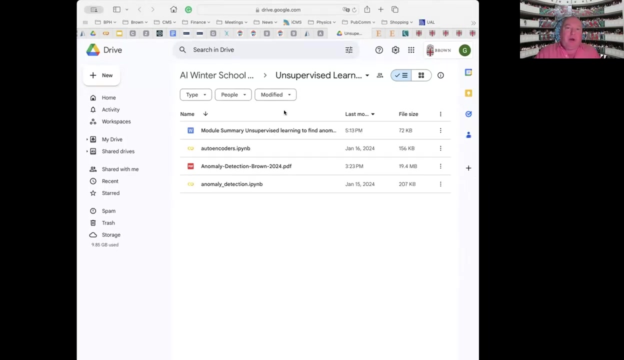 which is compatible with Google Colab, And what you need to do is to go to the Google Drive. In fact, maybe I should just share my screen and show you what needs to be done. So this is my screen of the Google Drive. 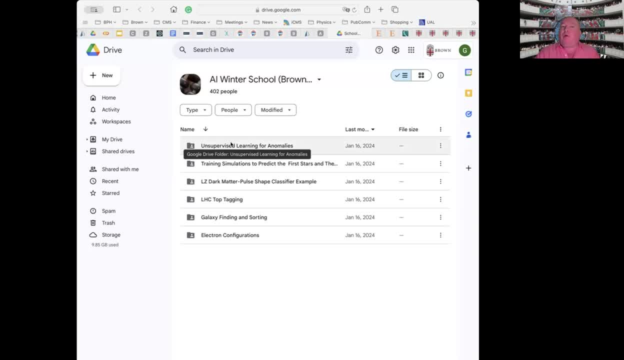 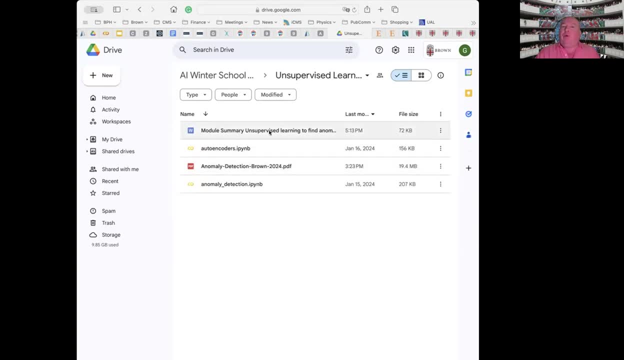 This is AI Winter School and you need to go to the folder Unsupervised Learning Phenomenes And there you'll find you'll find my talk module summary, which Lucas and I worked on, which has a little more information and some more references. 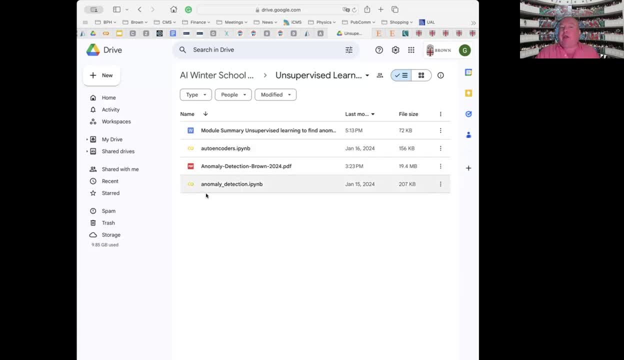 And then two Python notebooks- out-encoders and anomaly detection, which you should copy to your own Google area, because you don't have right access to this Google Drive. You only have read access so that people do not modify the code for everybody. 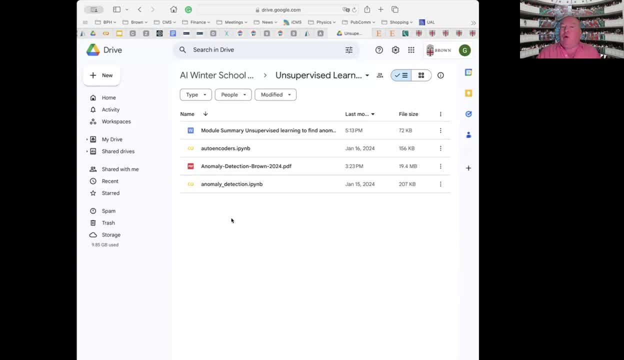 So what you need to do is to copy these two Python notebook to your own Google Drive. You could do it by using make a well, actually organize and then move- or make a copy and move it to your area, And then in five minutes we'll run the exercises. 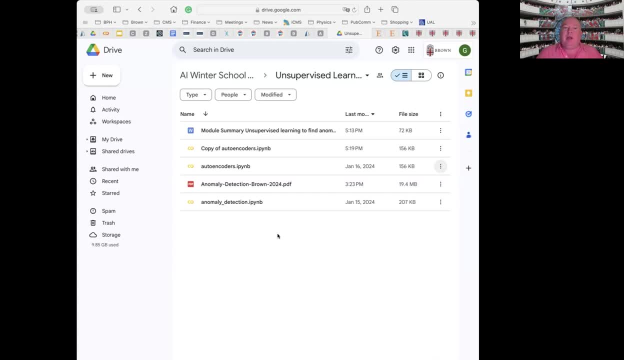 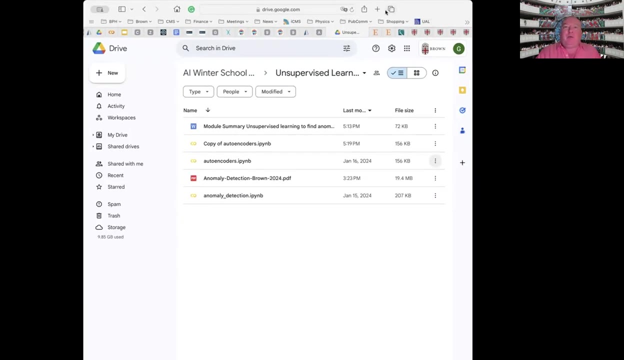 and we'll try different configurations, out-encoders and things like that. This is not very CPU intensive, so you you should be able to run all of these on GPUs without running over the free quota of Collab. So at this point let me stop sharing. 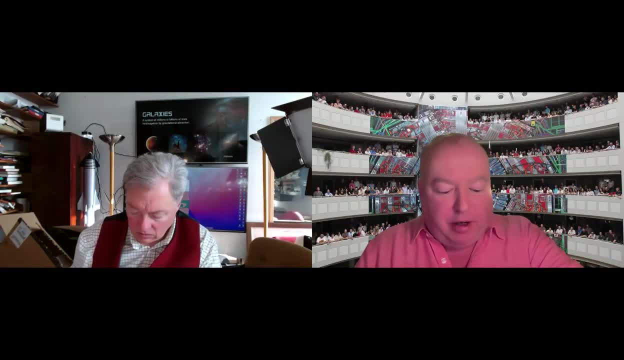 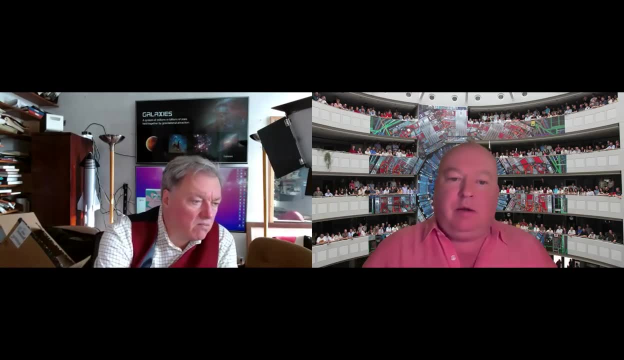 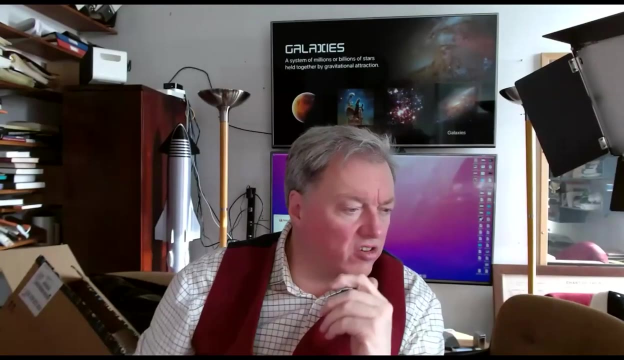 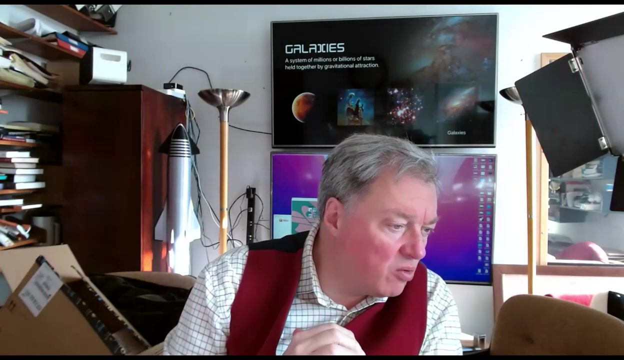 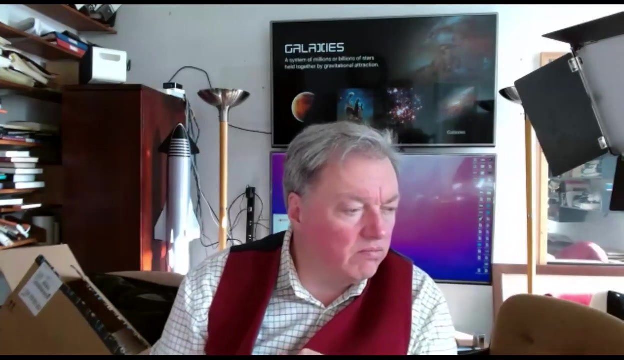 and let's have a five minute break and resume at 11.25,, I guess. Thank you, Greg. So there is one question. I see somebody posted concerning what was the LLP loss function you introduced, Right? So let me try to answer. 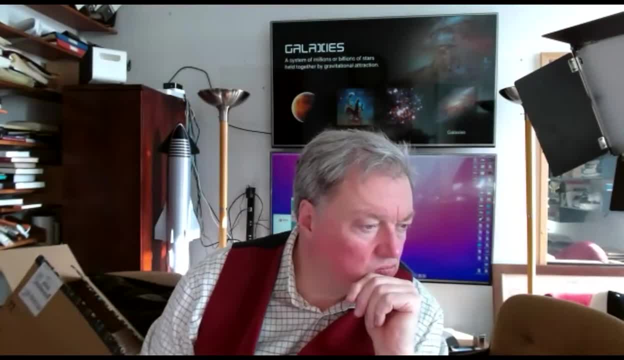 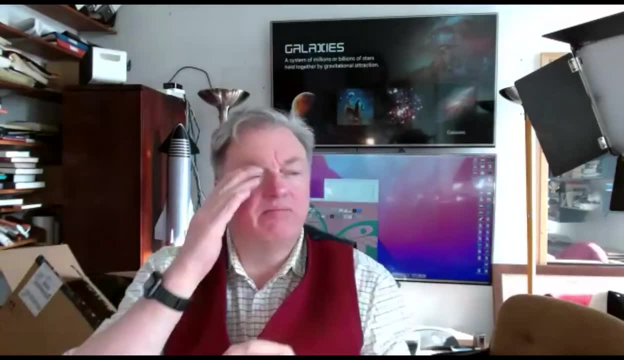 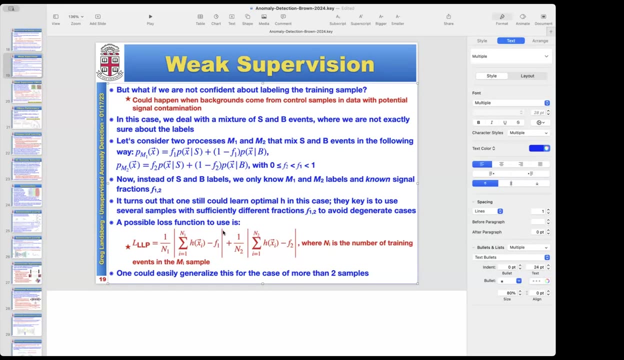 Need to find it. It's under the Q and A option in the Yeah. yeah, I saw the question. I'm just finding the right slide and sharing it. So this loss function. oh, I'm sorry, I forgot the squares. 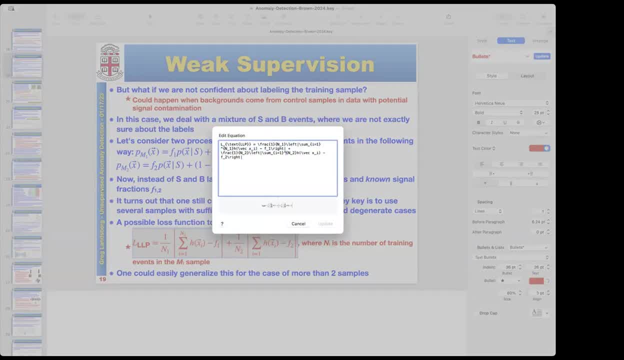 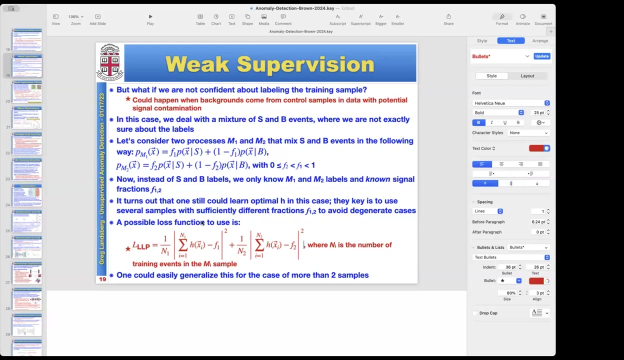 So this loss function really should have squares here. This is just the MSC minimal square function, So now it should be correct. So you basically take the first sample and you minimize these things. So this is just like. the F1 is a fraction of the signal. 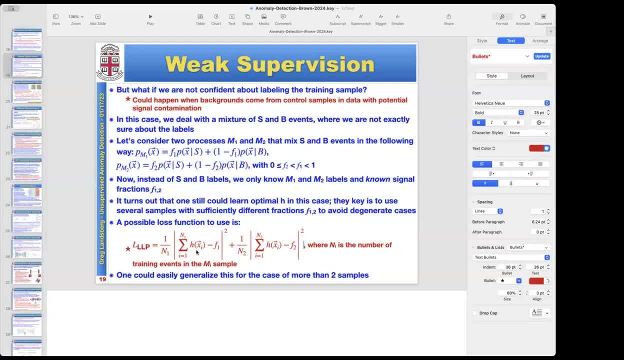 So you try to minimize the difference between your prediction and the signal over the events in the first sample And you do exactly the same for the second sample. So it's really just a MSC sum over the two samples And the reason it's called LLP. 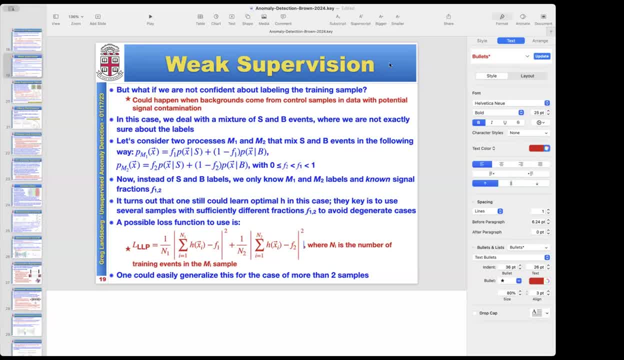 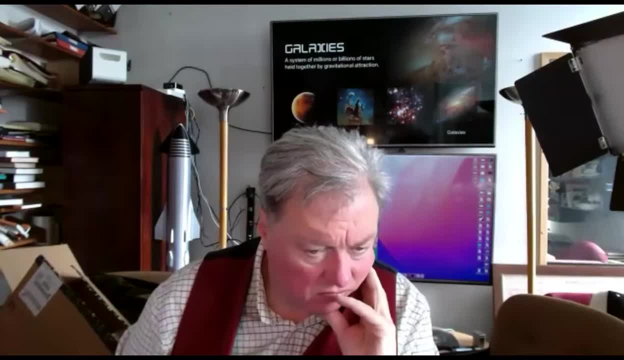 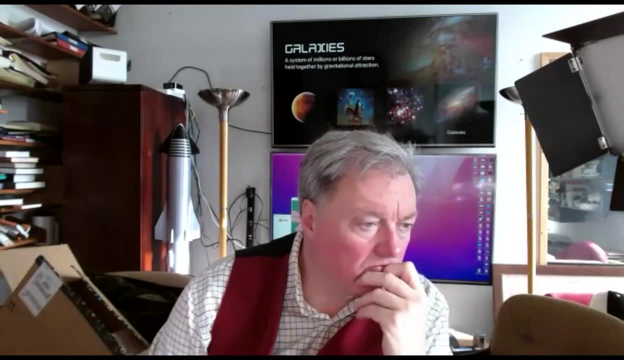 I don't really remember. It's an acronym for something, But it's not long leaf particle, it's something else. We'll let me have a sip of water and be back in a minute, So if anybody's having any access issues, 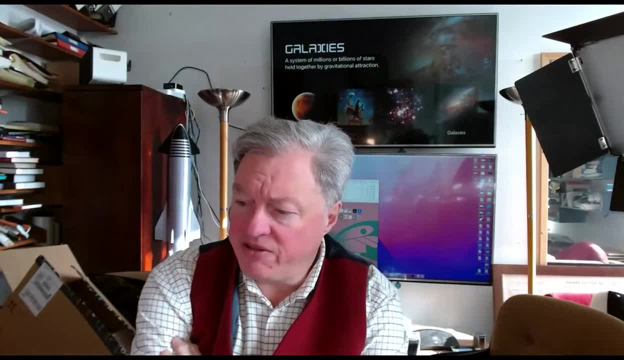 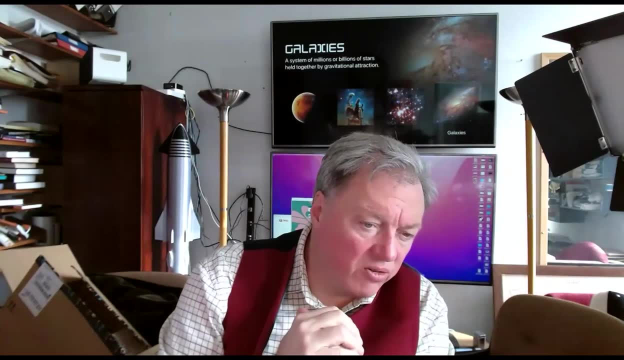 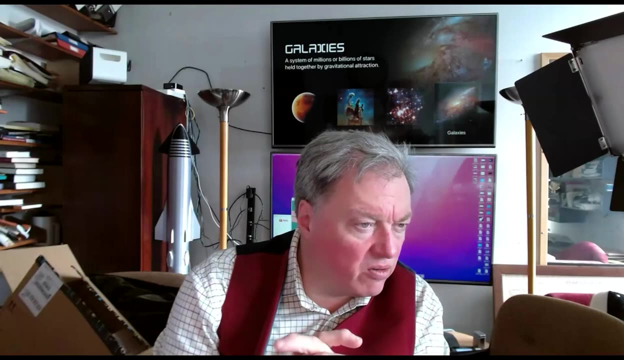 there is a Slack link on the front page of the Indigo Conference site. If you go into that Slack just follow the link: register. you'll see there are people ready to help support you if you do have sort of access issues. Just again to repeat the easiest way. 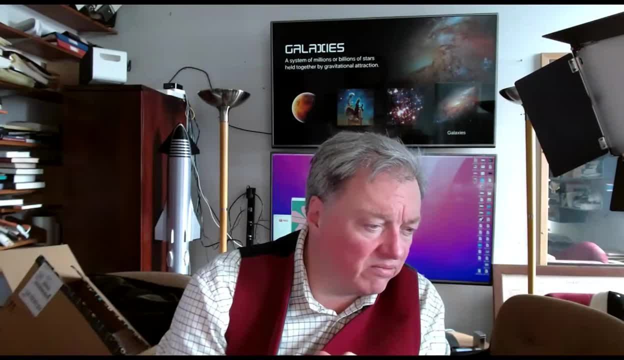 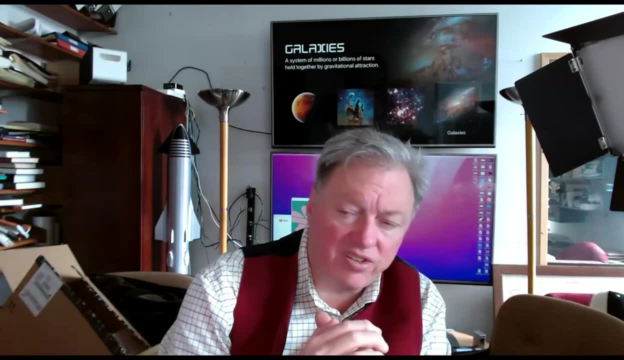 that is going to work is you just make sure that you're using an email address that allows associated with it does allow you to link to the Google Thrive system and also Google Code. So that's the email address. It's a very, very easy way to do this. 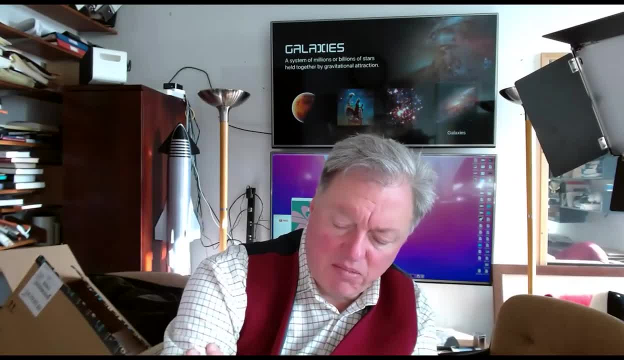 but it's a little bit more complicated than that. So, if you're using a Google Cloud, you're going to use this with the Google Cloud. you're going to use this with the Google Cloud, which is the Google Code. This is the googlecloudcolabcolab. 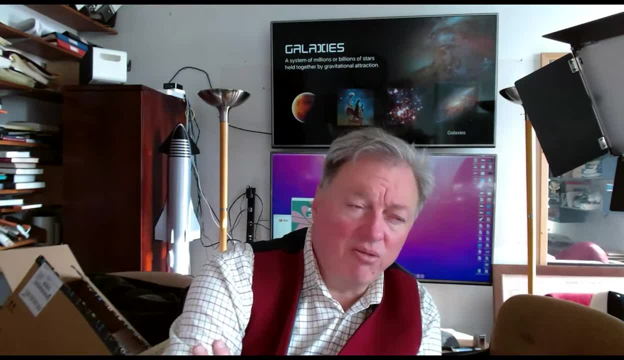 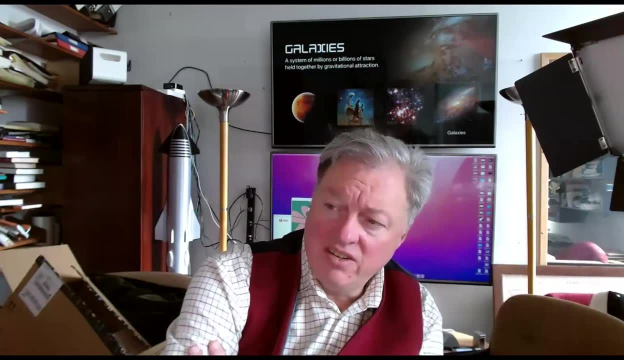 which is this Python notebook free service which we're gonna use to allow you to sort of get a very easy access. So you wanna make sure that the email address that you have given us does allow you to run on the Google Colab as well. 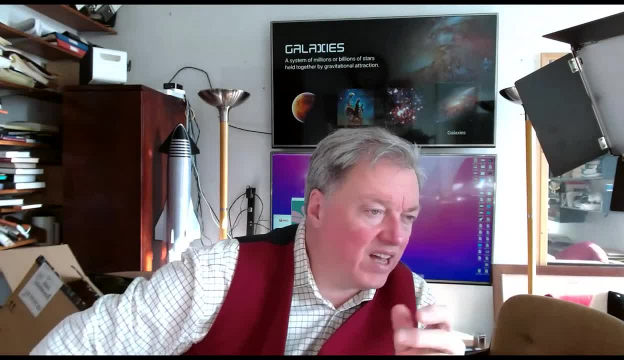 Re-register If it turns out that you have abused an email. you want to make sure that the email address you have given us does allow you to run under Google Colab as well. email that isn't valid for accessing Google services, then just re-register again and we'll. 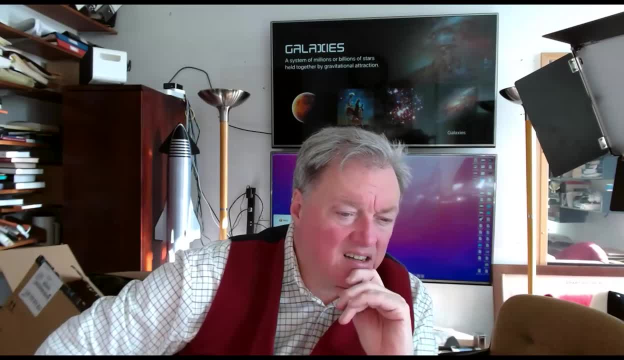 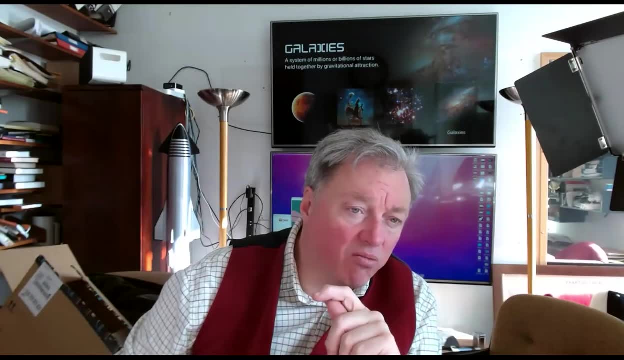 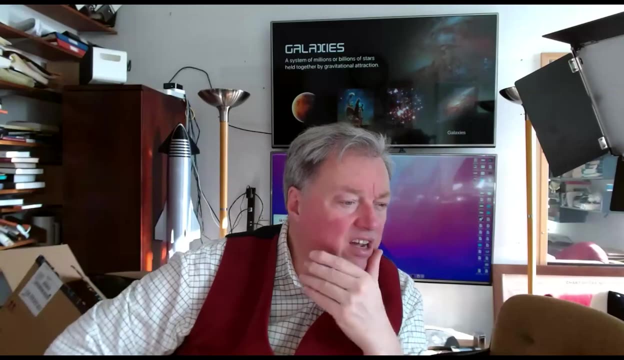 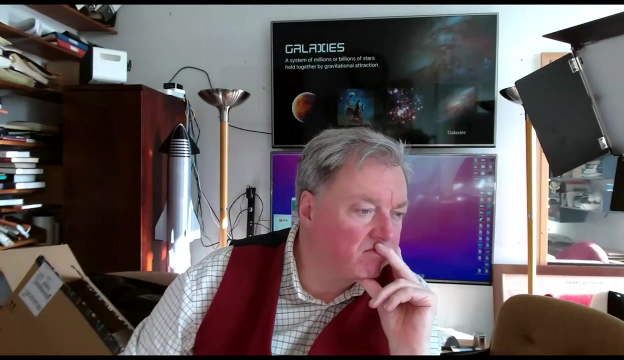 make sure that you get access. Also, use the Slack link. Come onto the Slack and use the registration channel and we can react to that immediately. OK, I hope that will ease any technical issues you're having. There are a couple of questions I see on the chat. 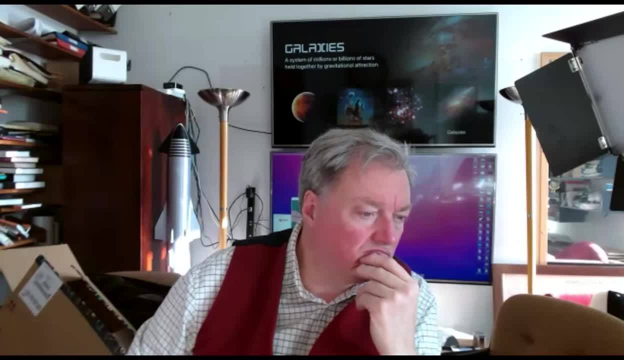 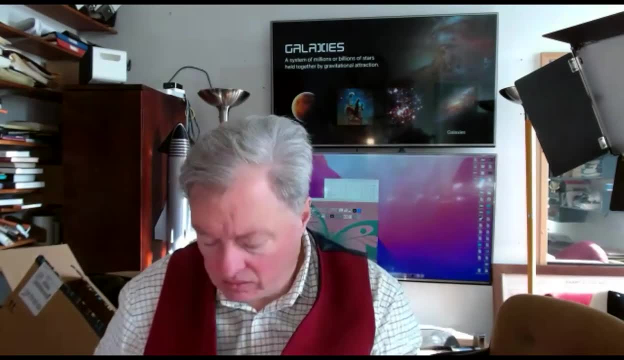 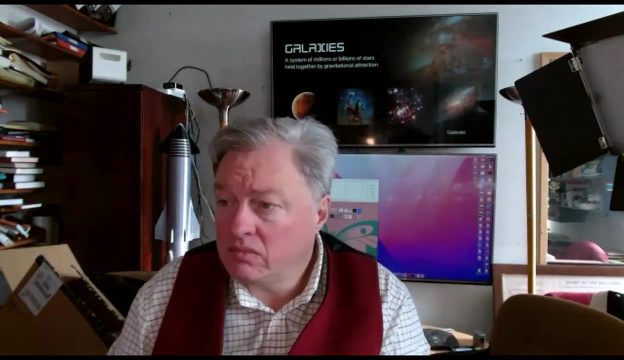 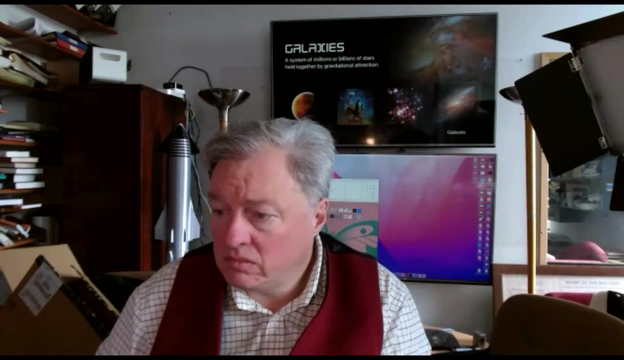 So yes, so there was one. The square will go inside the summation. Yes, that's correct. I think I typed the changes too quickly So I will double check the formula and put a new. PDF is the correct formula And the Slack link is on the very top. 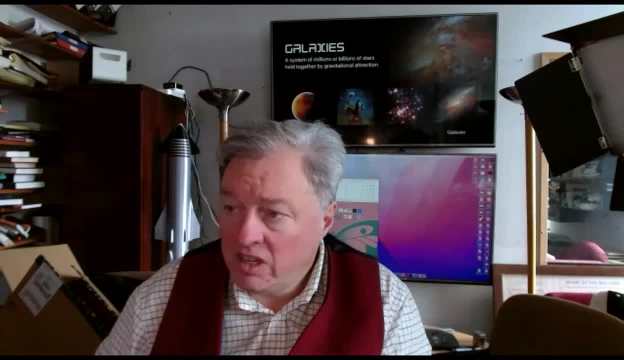 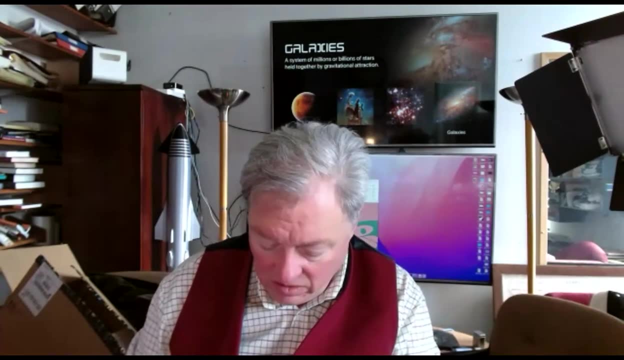 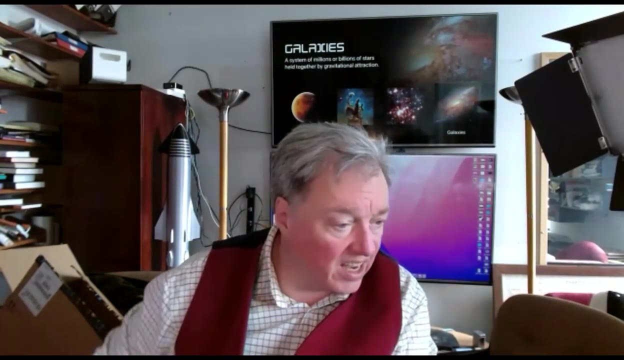 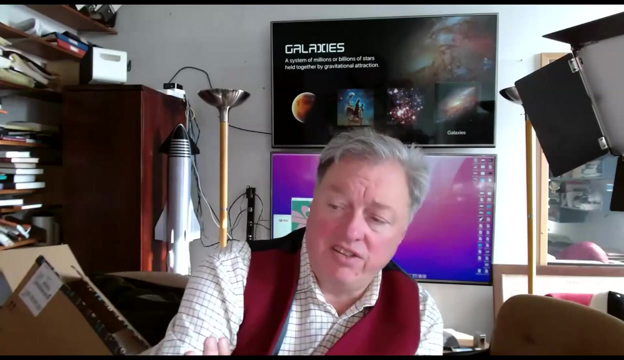 I could copy it again if people want. So here is the Slack link. So, Greg, it's available. It just Just Just Just a new overview. Yeah, I see it. It's on the conference front page. Yeah, 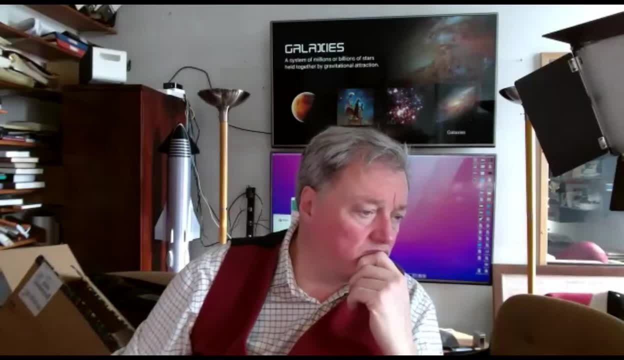 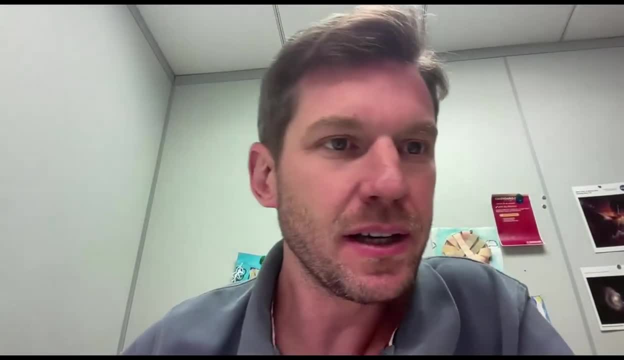 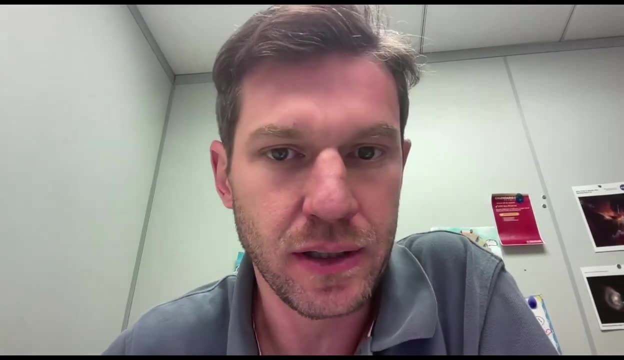 All right, So maybe we should move to the exercise. We will do a few things. Lucas, you want to take over? Sure, Yes, Hi, also from my side. So I think we should start with the autoencoder part. Yeah, I think let's start with autoencoders. 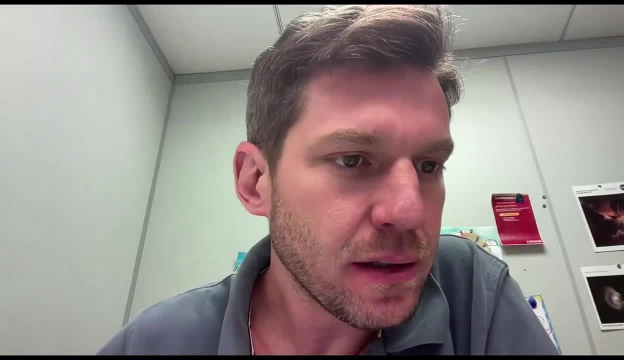 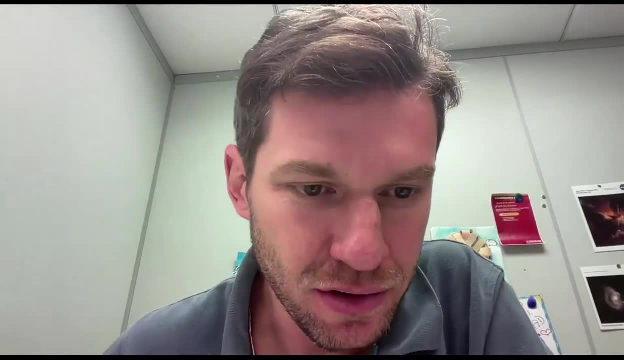 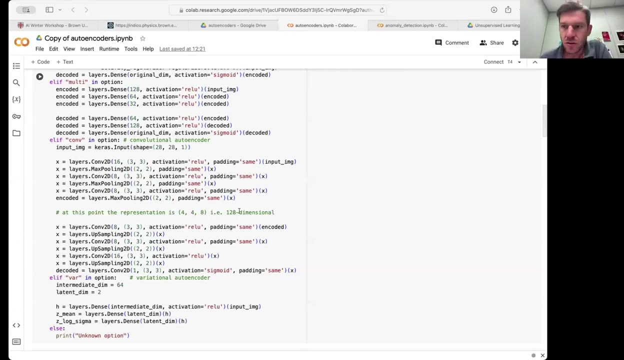 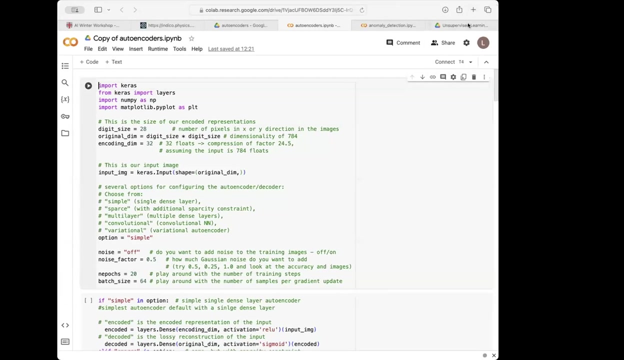 do a couple of exercises. Yeah, Let me share. try to share my screen, Rick. OK, yeah, Now I'm host so I can share. So can you see my screen? Yes, we can see your screen right there. 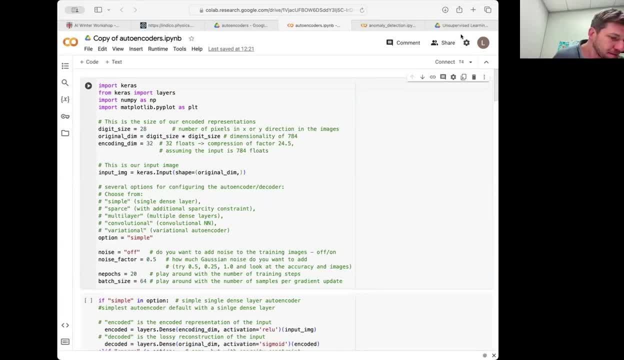 OK, perfect. So the way we organize this, all the tunable parameters are in the first block. So you You only need to modify first block, unless you want to do something a little bit more sophisticated, like changing the architecture. Yeah, 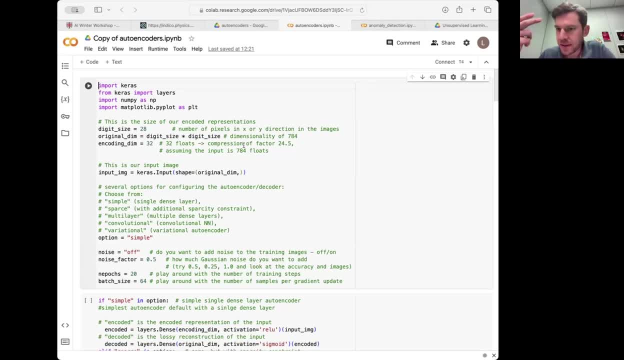 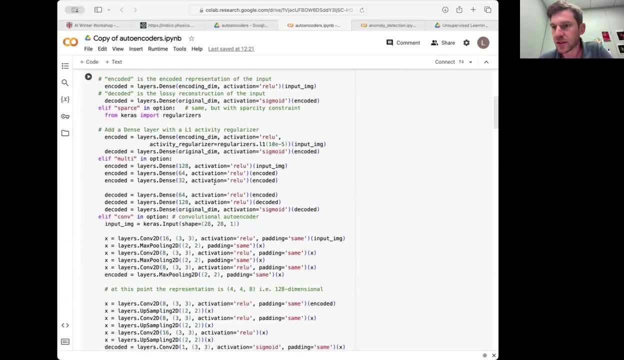 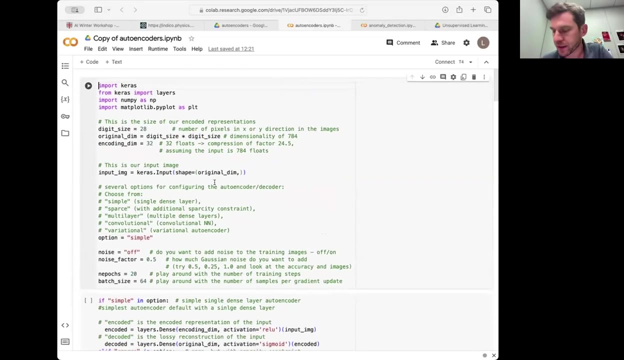 And one thing is that here we use data sets that are available on the internet, So it's not using that physics related for various reasons, and also to make the exercise simpler and easier to run. Yeah, Yeah, And it's not something that's easier to run during the limited time we have. 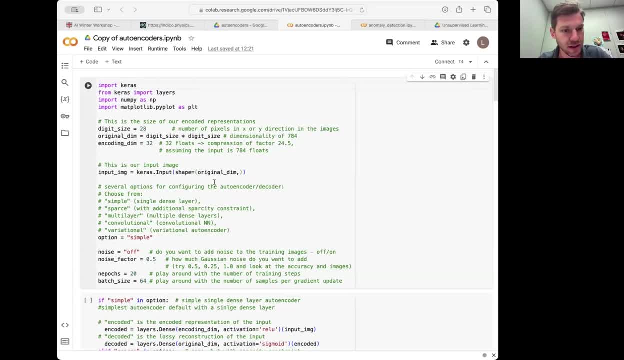 But nevertheless, the techniques and the tools and the conclusions are, you know, you can translate in any kind of problem that could benefit from these approaches. So what I would add this actually is to start, I mean the students, if they are, unless you know. 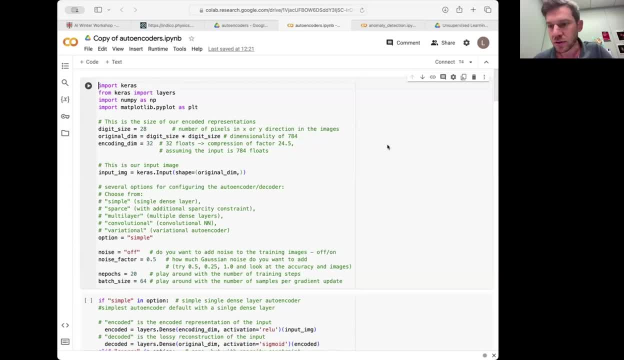 someone has issues to open the notebook. Yeah, So this is just this out. Otherwise, I think we can start running the notebook, So you can either click on. you know on this. You can see my point there also, right? 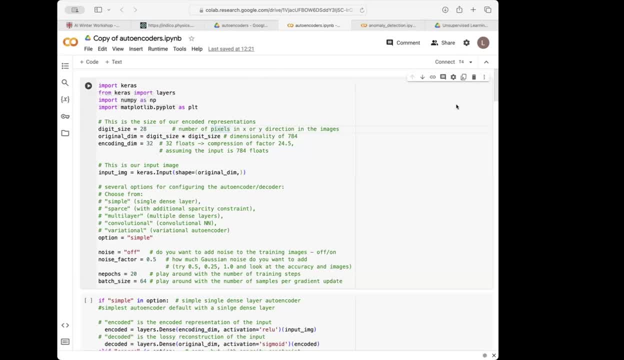 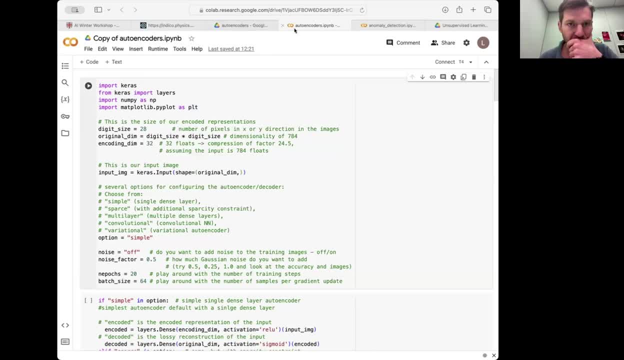 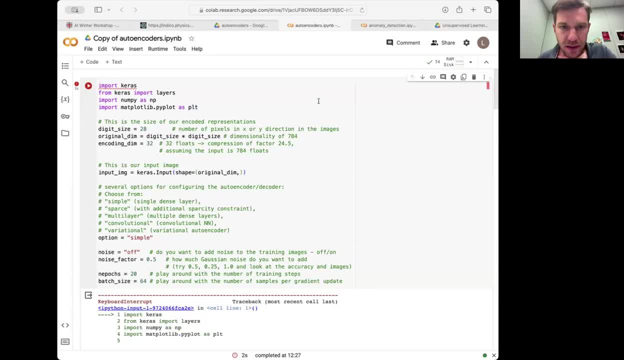 OK, nothing is then the message, so send the instructions, i think, yes, we'll, we'll. we'll deal with those questions, lucas, you, you focus on your own, okay? so, yeah, i'm trying to keep us. yeah, to have a look at the meeting chat also. so. 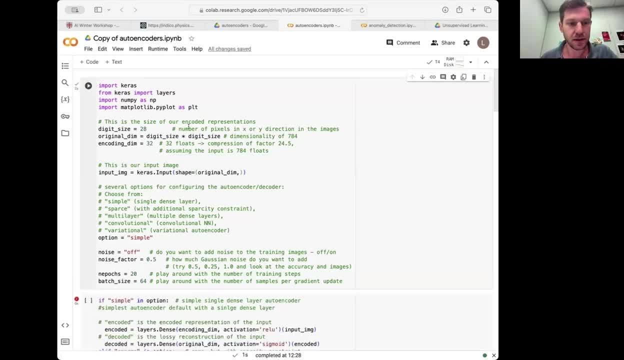 you know, the first thing is to start. i mean, as greg said, here we set the main parameters. for instance, you know, we have an image, so we have to define a pixel size. so here we use a size that is the same between the x and y dimensions of the image. and so you know, since it's the same, if 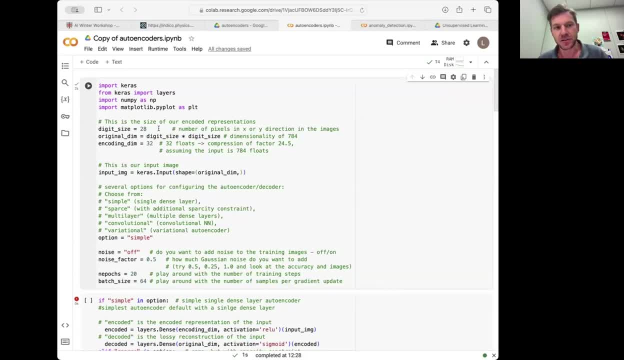 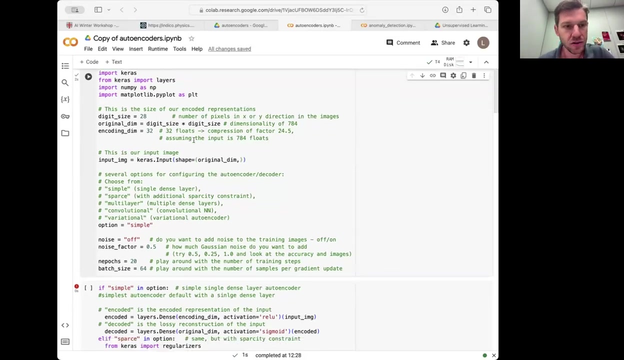 effectively, the original dimension is the multiplication of the, of the of this parameter here: 28, 28 times 28, 7, 184, and we want to, to, to, to encode it in the dimension of 32. so, yeah, there are notes here, so you can also, you know, follow them after the exercise if you have. 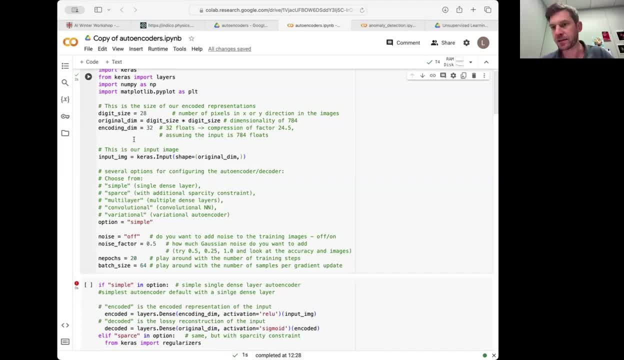 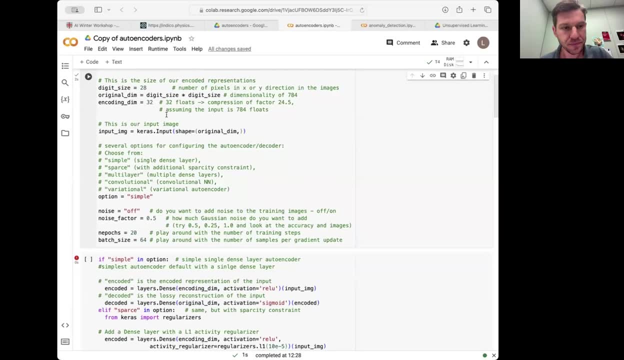 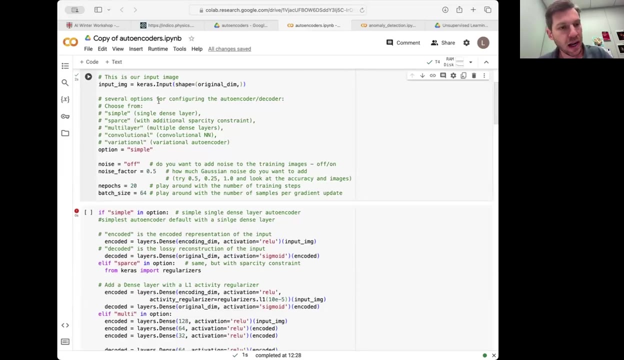 questions. so i'm not sure how familiar you guys are with keras, but here is how we import the original image and i think we can start with a simpler. i mean greg, in his talk, described to quite a few of the options that we have to develop the autoencoder and the decoder part. so i think first we can. 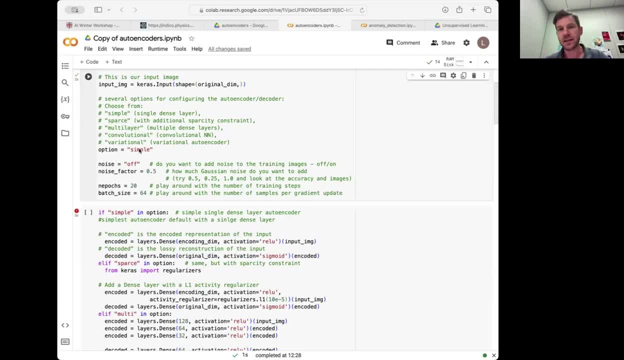 start with a simple option which is a dense network, so effectively is a. it does linear transformations effectively. but there are also other options. this is a single layer. we have also the sparse option which i think greg mentioned. add some robustness on the training so it doesn't use all neurons. we have a multi-layer perception so we actually stack. 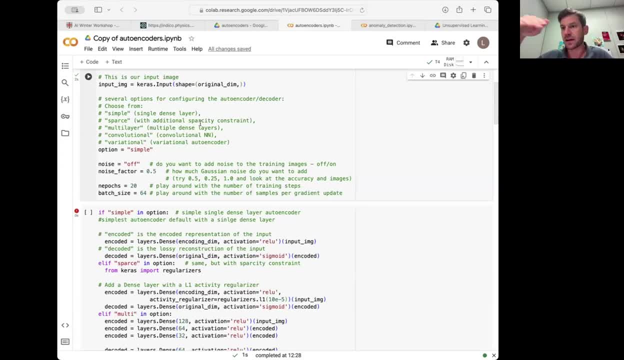 several layers, so several linear transformations. then we have the convolutional neural network. so this you know, you run a convolution, a patch across the image to identify features in the image. and then we have the variation of auto encoder which is effective. with the greg discuss, we have a functional form and to capture the features of the image. so let's. 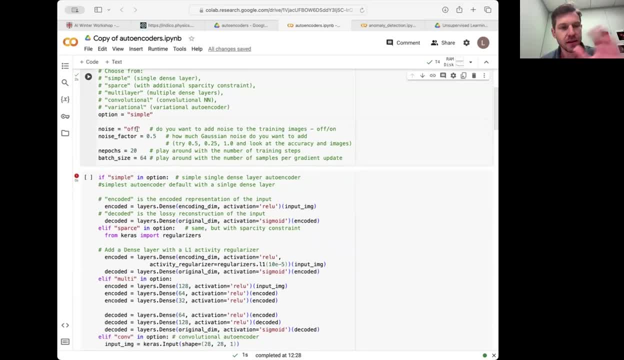 start with a simple one. i assume: yeah, this is also if you want to include noise in the samples to disturb the images, to give a more difficult problem. other options is how many epochs we run so actually, uh, how a full described, um, when, with a full training, like a full pass over, uh, the network. 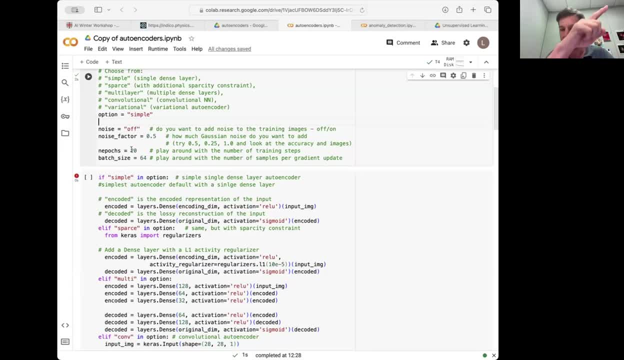 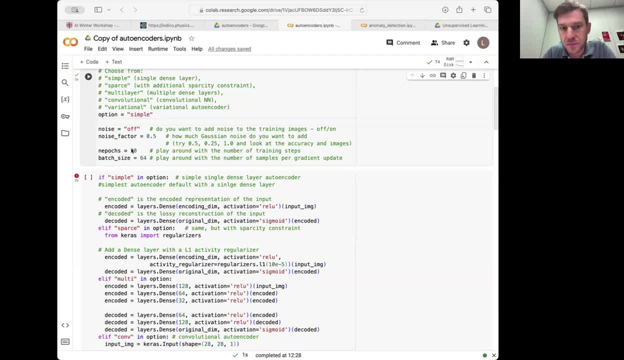 start getting uh. getting lower and lower value means that the training is improving. the network learns more and more information. the batch size is how many, the amount of images we will use in each epoch for the algorithm to learn. uh. we put 64 here. these are hyper parameters, so this: 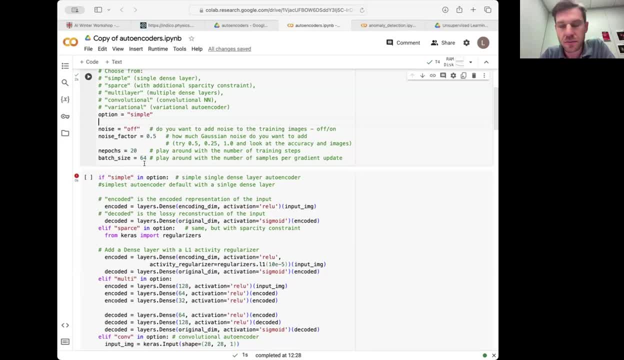 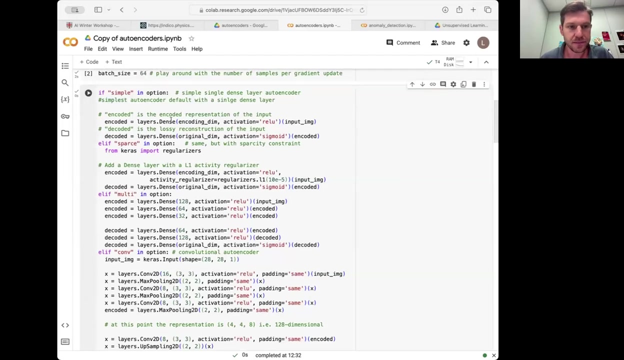 typically you want smallest batch sizes, but also depends on the complexity of the model and, to large extent, all these parameters are kind of a trial and error. so okay, after you can go back on this thing. so let's start. let's run the second cell, selecting the simple option. so what is doing here? as we said, here we have a single. 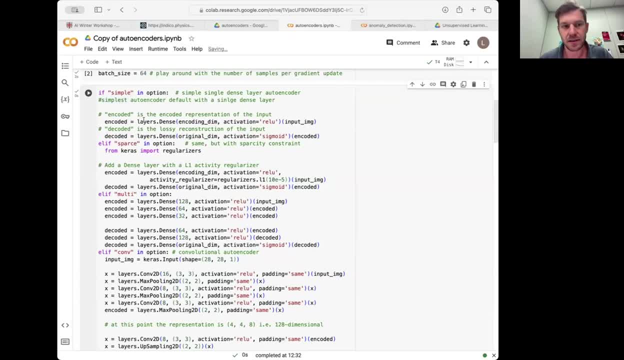 layer and this in keras. this is defined as layersdense. this is the dense network, and then, as human brain works, right, we have a set of inputs and then, if we see something interesting, we activate the neuron. so this is what it does. so this is a relu, is rectify, linear activation. 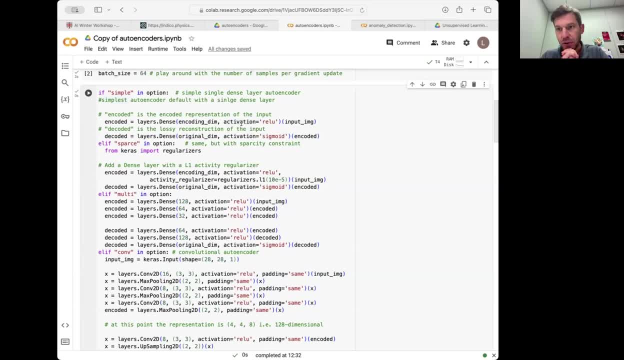 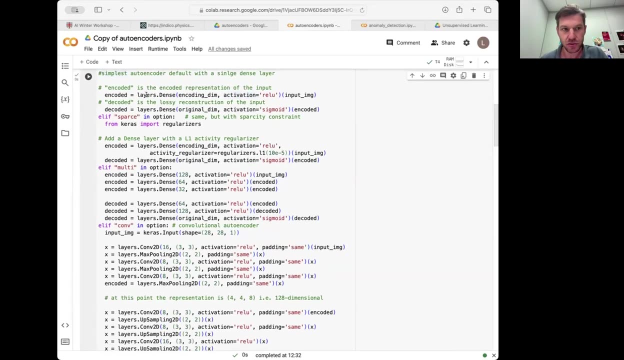 function add. it's a non-linear one, so if it passes some threshold, then you know as a human name- the network fires effectively and uh, this is for the encoding part and then for the decoded part we have an action activation, we have a sigmoid, so it will give effectively a probability range from zero to one. uh, 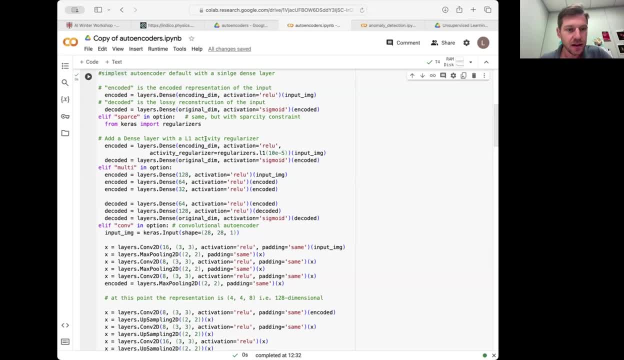 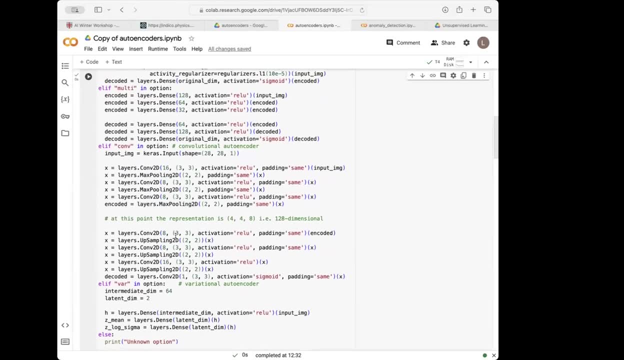 yeah, as an out, i think. i don't know, greg, what do you think, but maybe we can discuss later the other, uh configuration. yeah, i think we could. just- you don't have to do all the examples- i would maybe. okay, yes, layer noise and uh, something like that, yeah. 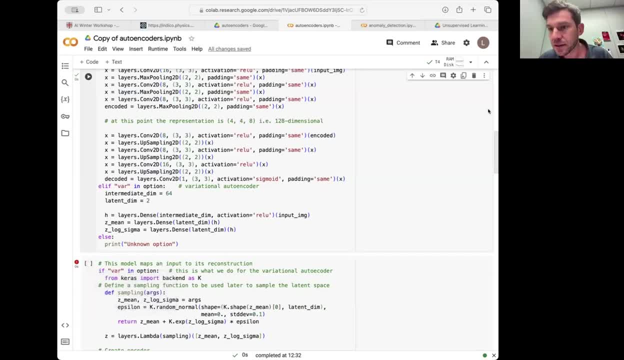 so let's go down once first to see that everything. yes, sorry, somebody posted a question saying: is encoding underscore dim the same as the number of hidden nodes in the latent layer? uh, on the on the q a, yes, here it is. so if, if lucas scrolls a little bit up, you see that we 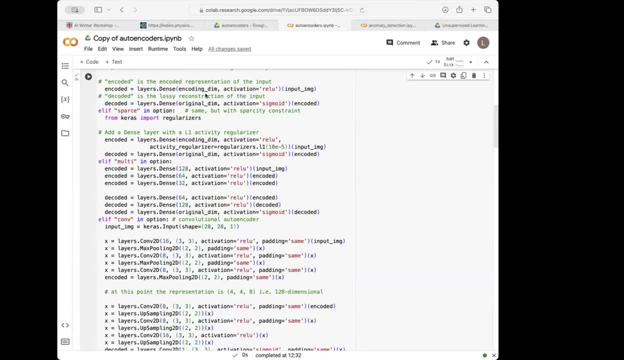 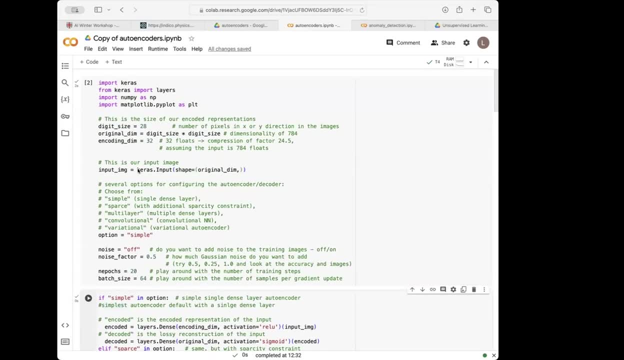 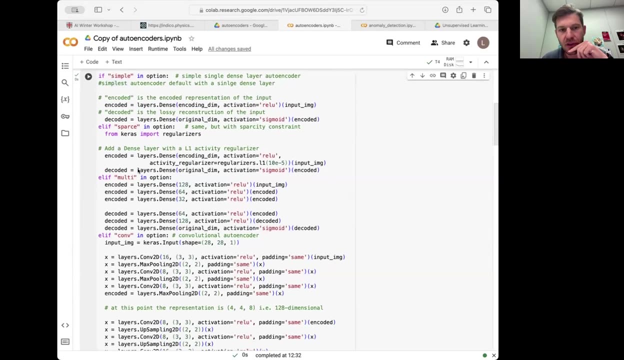 uh, included this one layer with the encoding dimensions. that's in the encoder. yes, layer decoder is single layer and encoding dimension is essentially latent space because there's only one. Yeah, Thank you. So we compress 784 pixels from 28 by 28 image. 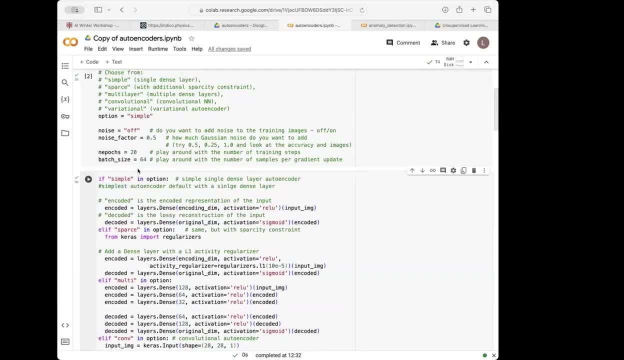 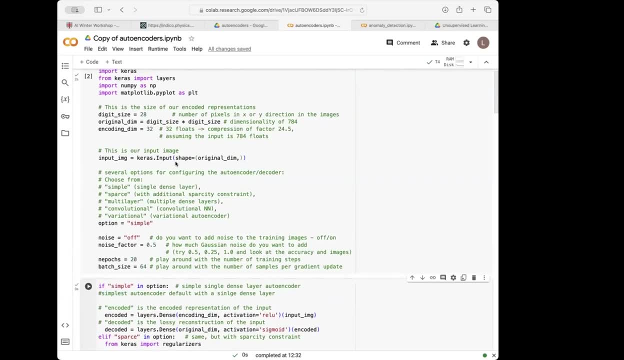 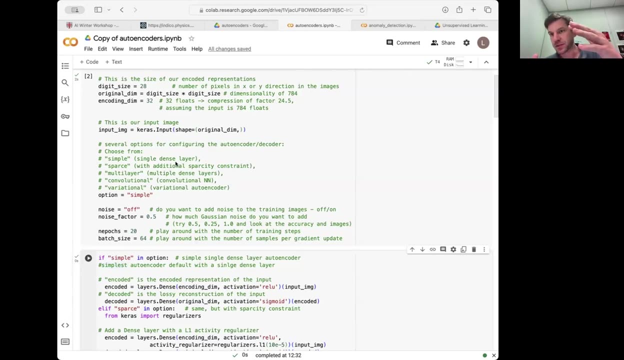 into the 30,, whatever, 34. Yeah, 32. 32. Yeah, It's compression factor of nearly 25.. Yeah, so the idea is, you have your image, you start compressing it, you, you collect the most important features and then you start the 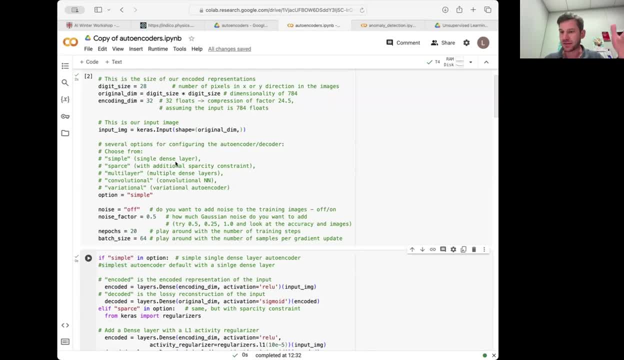 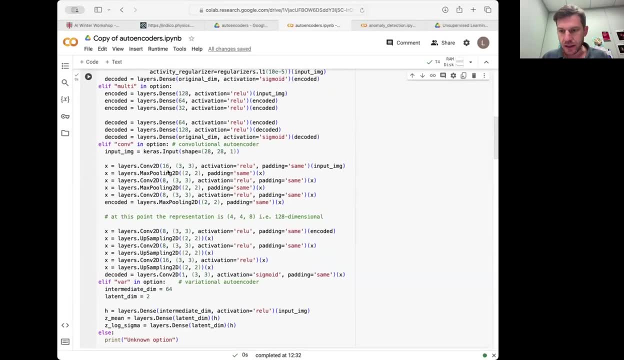 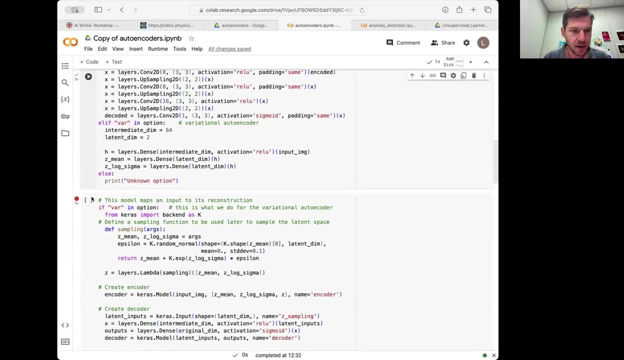 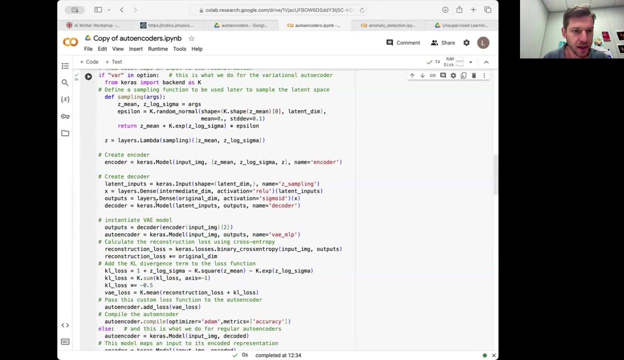 compression and the output will be the same image, as you have a same, Okay. Okay, then this is the next element which keeps: stay with a simple one, and then we run, then the third cell. So this is actually- maybe I can So- actually, this gives us actually a summary of the. 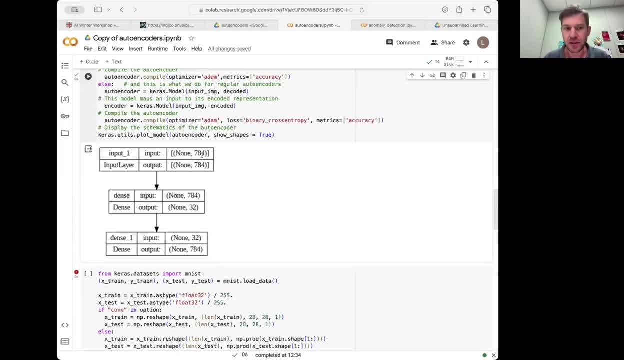 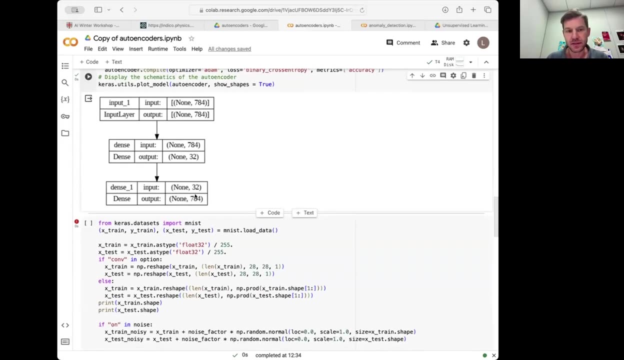 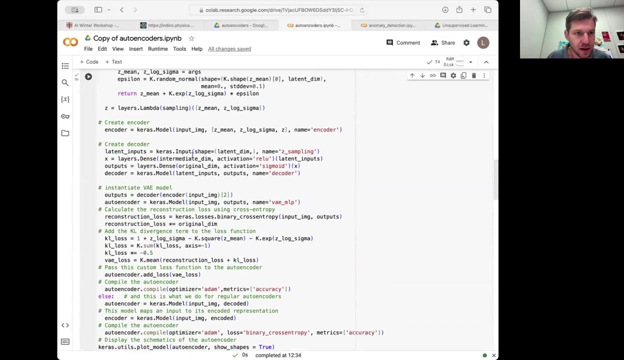 networks. As we said, we have one input layer. you have the input here: 784 pixels. We decoded 32 with a single dense layer And then we decode it and go back to the original image. So in here maybe you can identify. 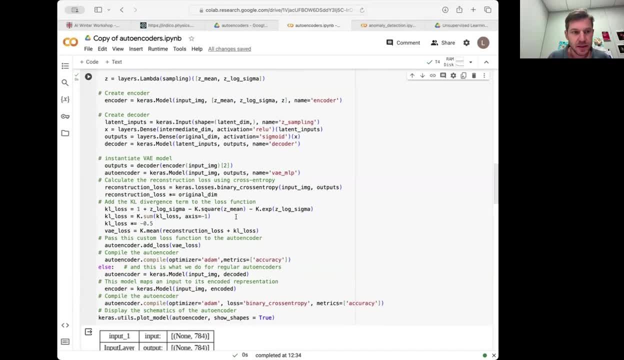 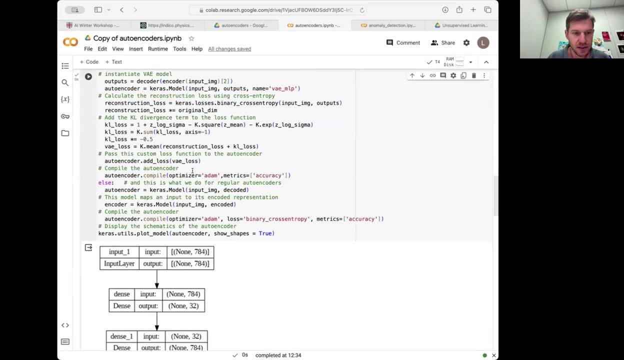 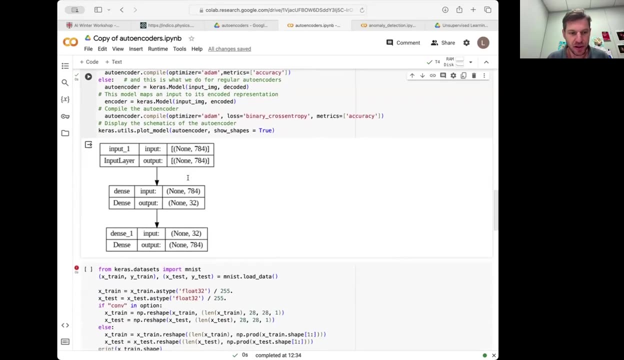 some parts like, for instance, what is very important is the- yeah, I mean the- loss. okay, we're going to discuss later. I think, yeah, I don't know, Maybe we can run and go back and discuss it later, if you have questions, but, or when we do a. 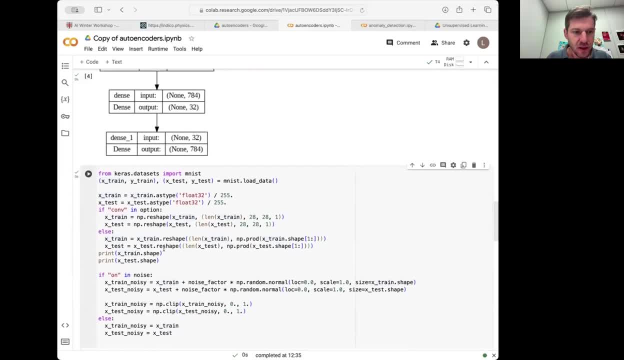 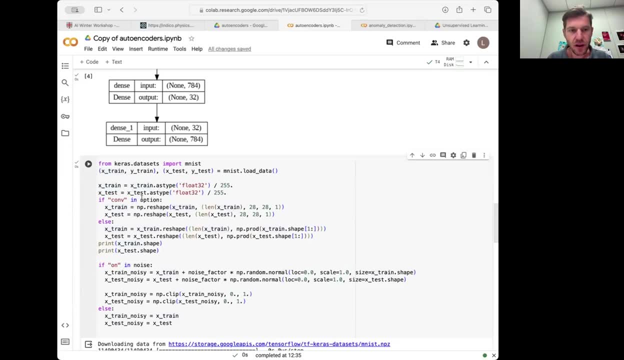 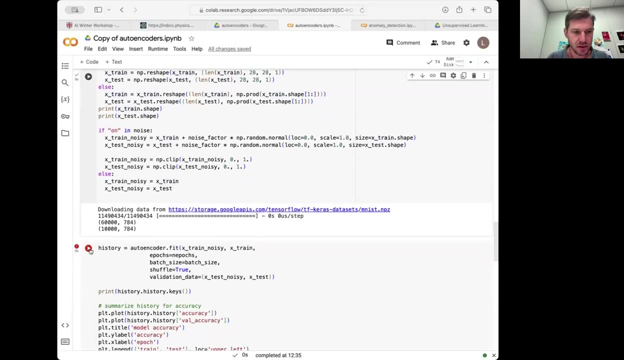 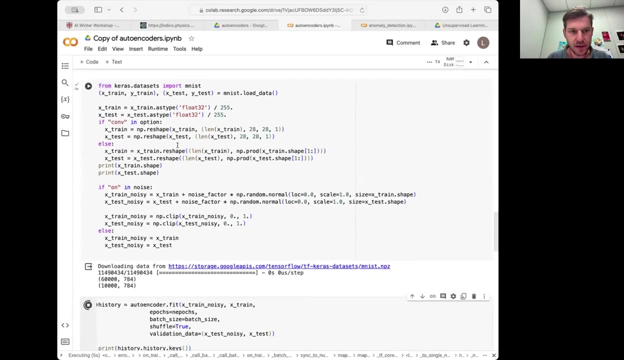 more complicated problem. but here is the point that we are doing the training. So this it's sort of looking: yeah Well, here we get the data and we do the training on this cell here. So you see, the different networks is going to run to 20. 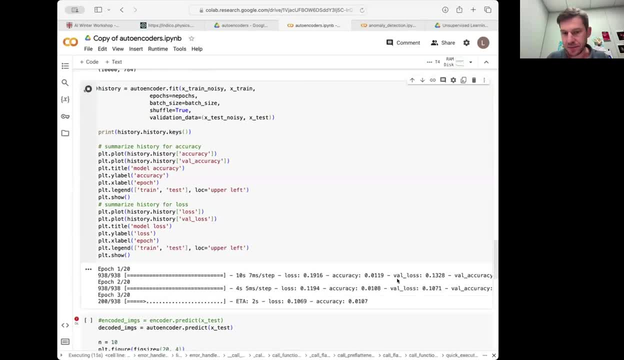 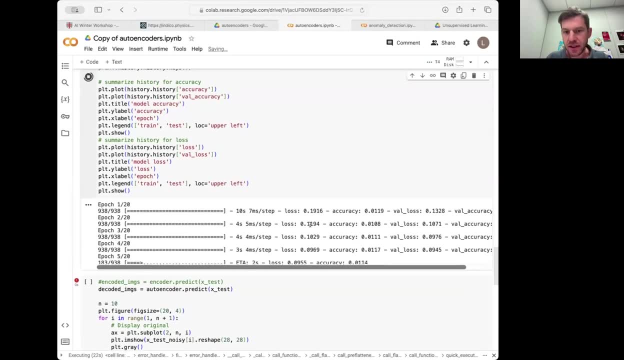 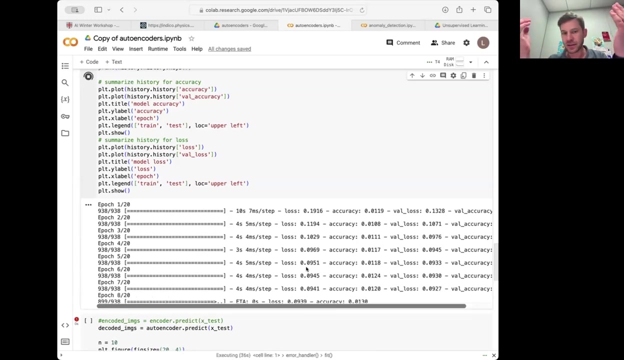 epochs. This is the loss function, This is the accuracy, This is the loss value. So what you see- and this is actually what you would expect- actually is that the loss start getting lower and lower. So, in principle, what it does, it compares with the truth and goes. 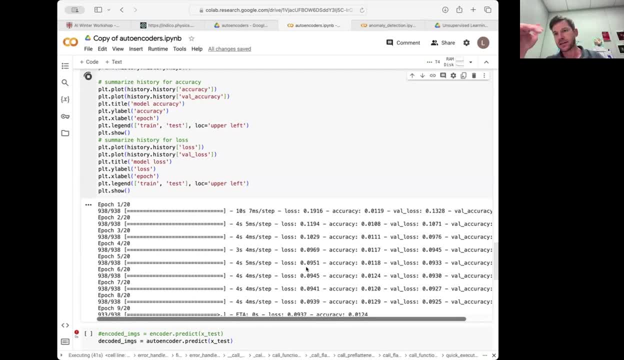 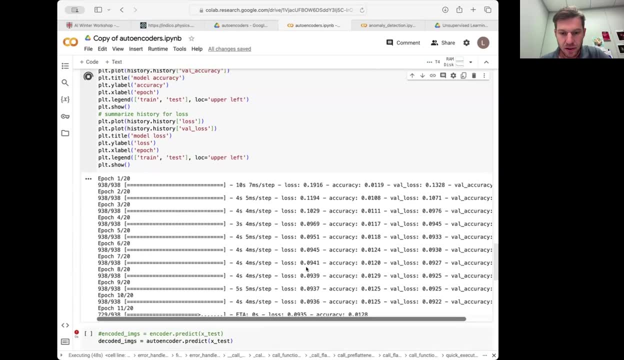 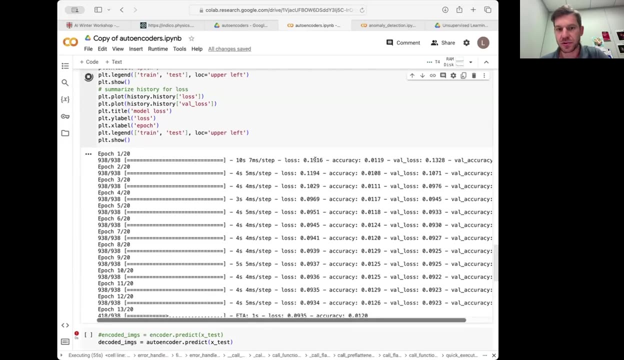 back with the back propagation, improves the parameters, and then we do the training And, yeah, in principle, after a few epochs we start converging, which is, I think, kind of. what we see is that from 0.19, and then it goes down to 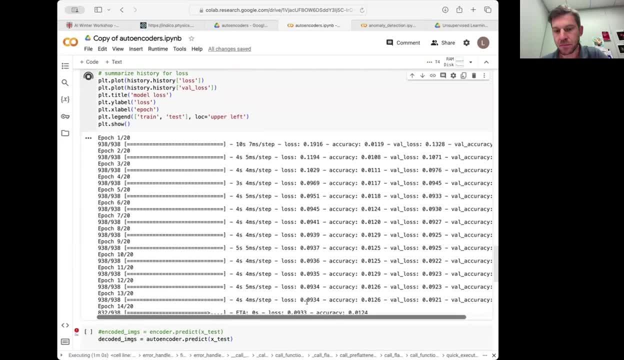 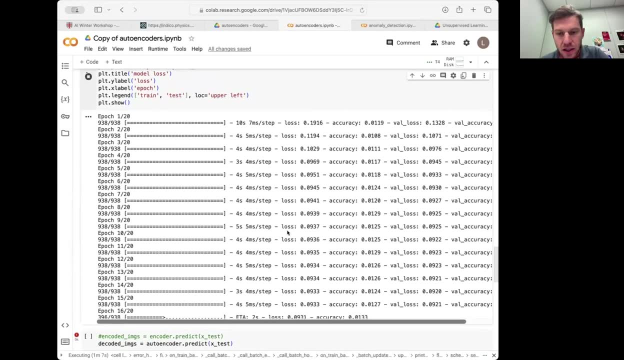 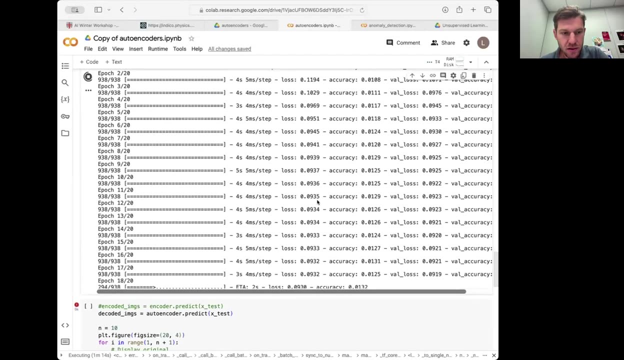 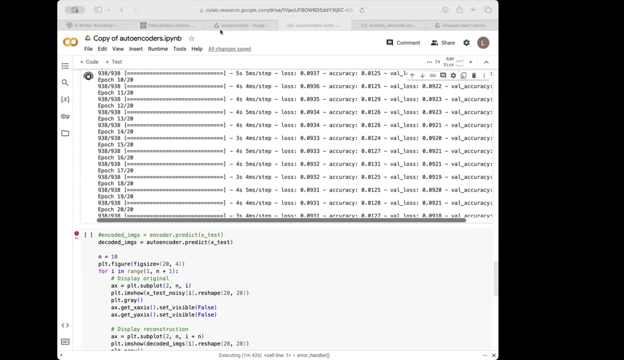 0.10,, 0.9, and the improvement. gradually it gets smaller and smaller as we go to higher epochs. So at this point it stopped training. but it will collect the data and do some images so you'll see how the loss function changes the steps. 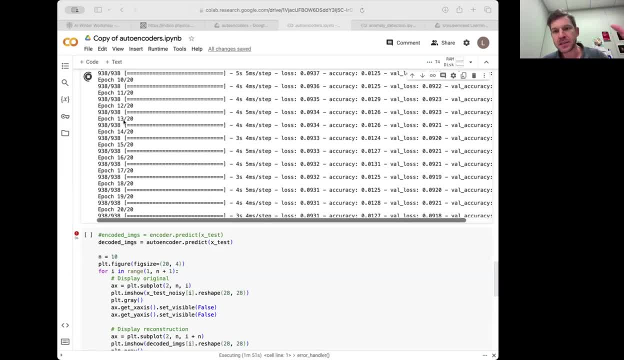 Yeah, So each epoch is like passing through the entire training data set. Then we update the weights, I mean the network- update the weights in order to minimize, to try to go imagine as a function in multi- dimensions, and then gradually starts to find the minimum. 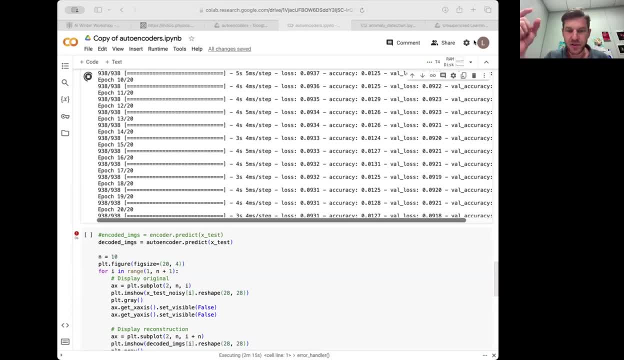 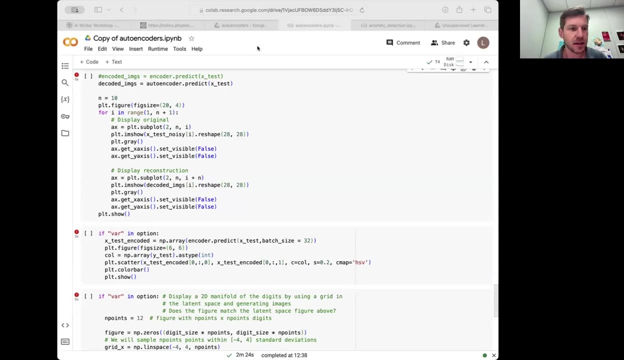 So another thing that we should try to find the minimum and then, after passing one more, one time, after the entire data set, improve the weight of the network. And then, you know, this goes on until, in this case, until reaching 20 epochs. Now, this actually. 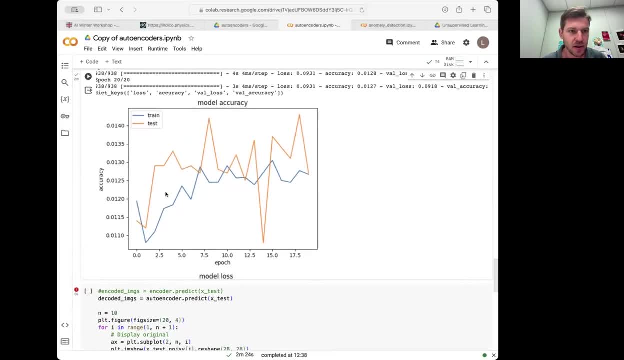 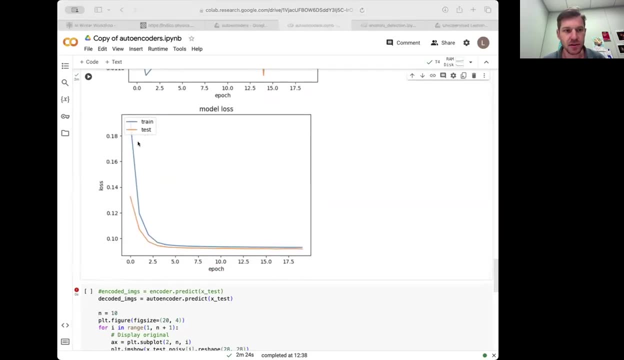 again. can you see the plot here? So this shows the first plot, shows the model. okay, maybe first let's go to the loss. So two things here: the blue line that says train it. So what do we have? the sample that consists of training and testing. 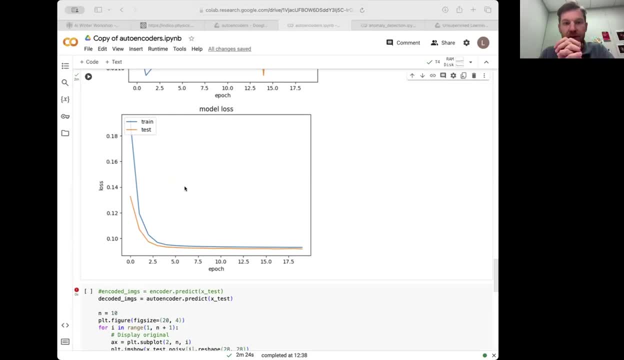 them. So the training data set: we split the sample in train data set, which is usually the largest fraction of the sample, And then another orthogonal set of events, set of images, that is, a tensile sample. So what we want to see is actually that. 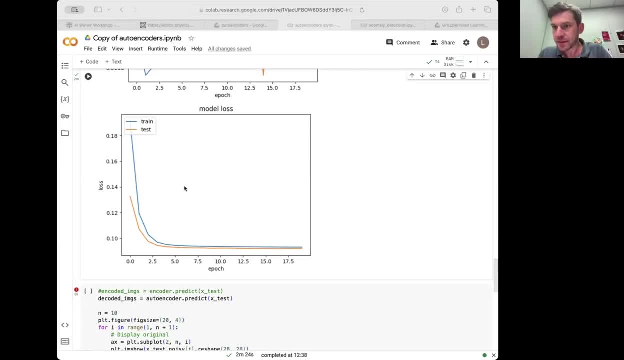 that what we train, we train on the training sample and the performance that we get on the training sample is more or less the same as in the test example. Now it's important to check this, this metric, because if, for instance, we wouldn't do, 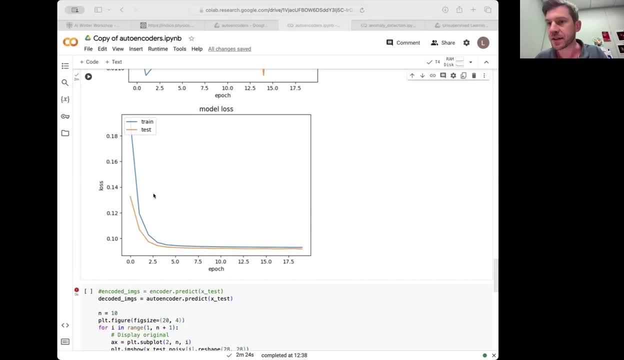 this we have a problem. we can take it, for instance, this overfitting- if it learns very well the data that I've used for training, but we cannot extrapolate it in unseen data. If this was the case, you would see the 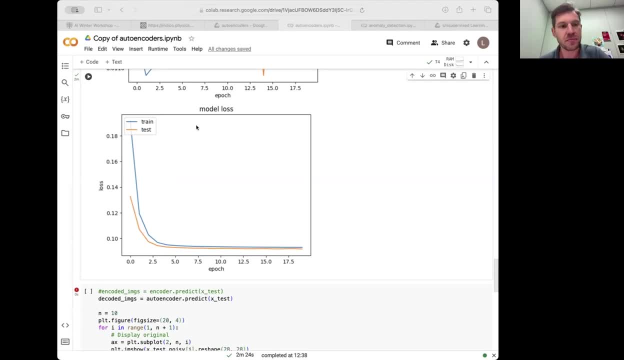 the testing distribution, the orange one to be much higher than the blue one. Here, the fact that the the orange one is lower than the blue one, it's actually a good thing, And it's probably because we have some dropout. So when we train to avoid, 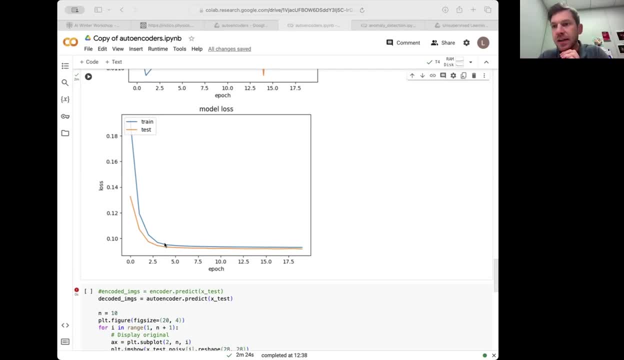 overfitting, for instance, we can remove some of the nodes, But when we test it we include the full capacity of the model And this gives better performance for testing. this is great. You see that actually even a couple, three, four, five epochs, the you. 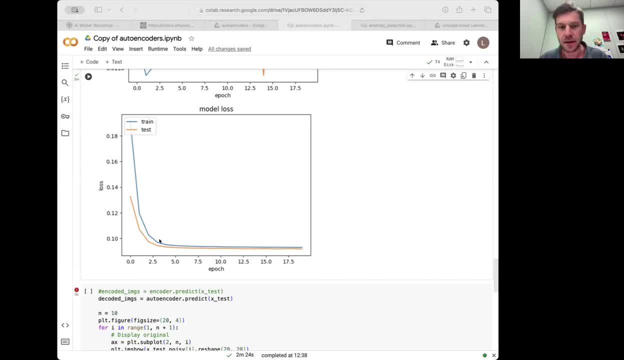 know the training it's kind of. it gets very close to the optimal. Maybe, if I can take this opportunity, one thing that one could also take a particularly more challenging problem problems is the learning rate. So it's how the steps effectively that the network 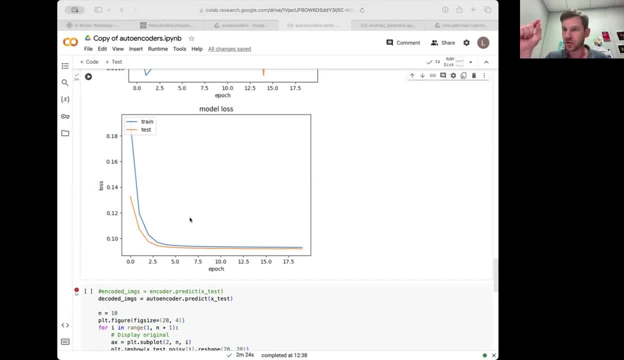 that the algorithm takes in order to optimize the values weights. So you know, if you, if you pick very small values of this learning rate, you may end up having a lock, ending in a local minimum and not finding the global minimum give the 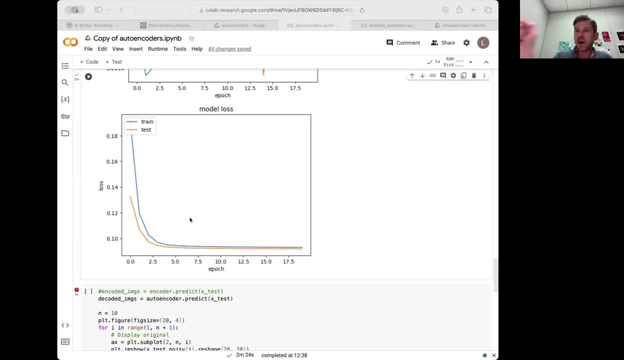 optimal result. If you get very large one, you may bounce around your function but not really lead to the low rate, the low local minimum In real time application. one technique that one could try is to use a decay learning rate. start with a. 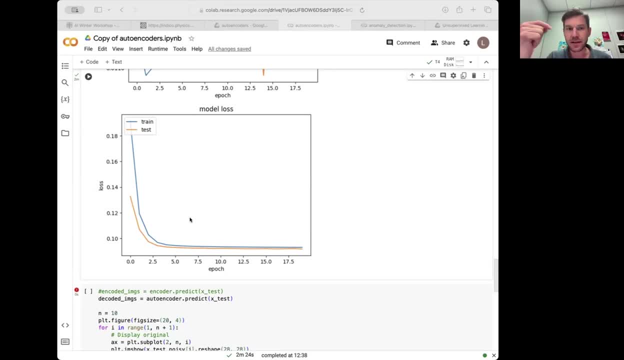 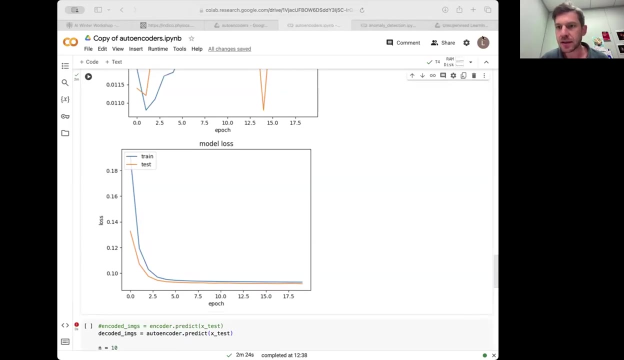 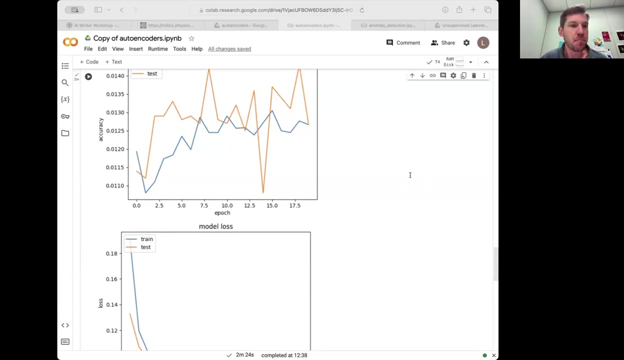 relative larger learning rate And then, as you go on, the epochs start reducing. me with some functional form, can be an exponent, etc. Okay, And what else here? The other thing that we could discuss is actually the accuracy, which is actually a metric that measures the proportion of correct. 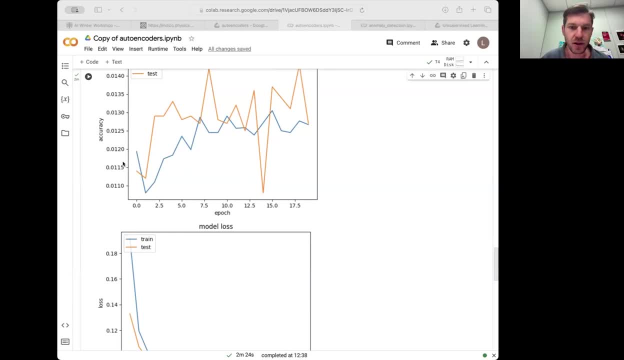 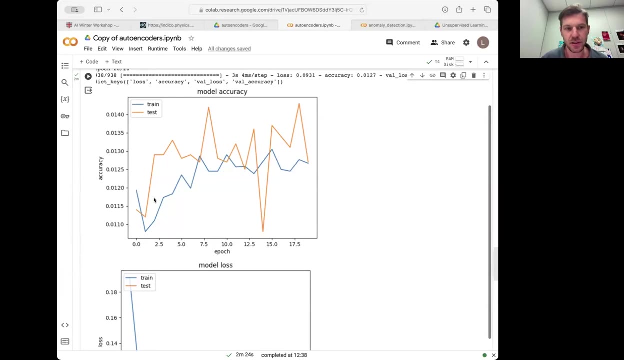 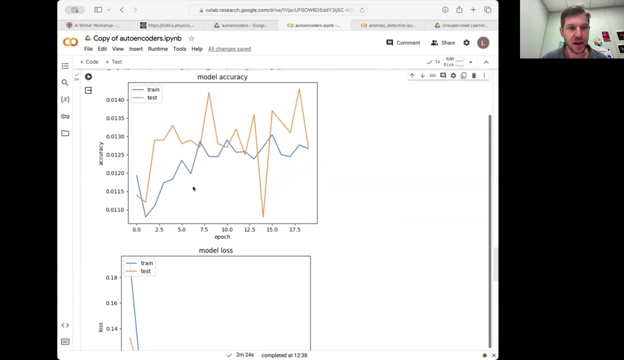 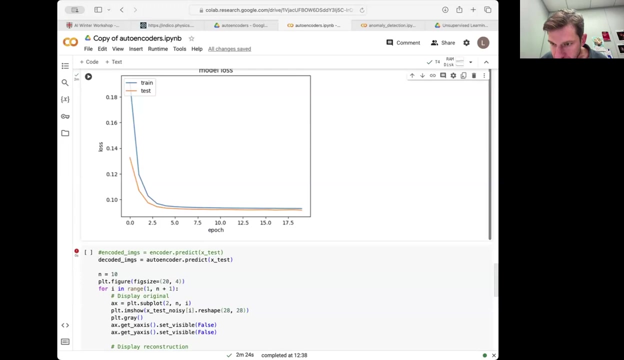 predictions among the total number of cases process And you see the accuracy increases, as one would expect, with respect to the total number of cases. And then you see the accuracy increases as a function of the number of epochs, both for the testing and for the training. So there are some messages. Yeah, I'm. 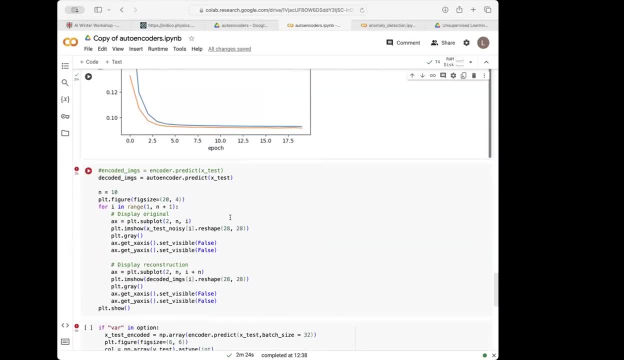 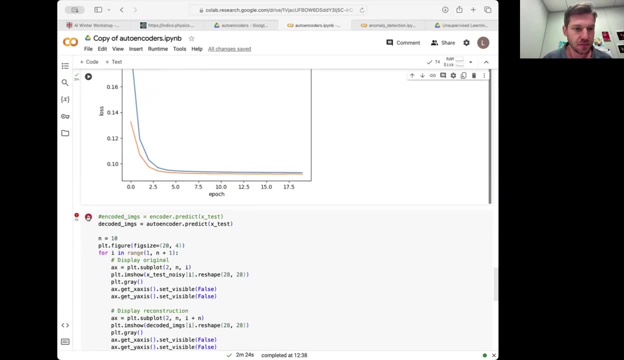 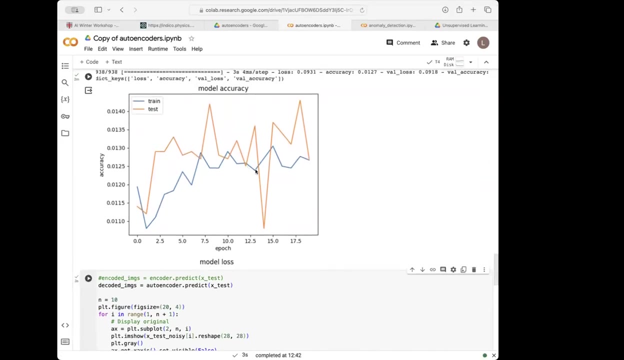 answering: Okay, yes, yes, I think we can run, unless, Greg, you want to add something here We can discuss. you know, maybe notice that accuracy is not very good in this case because it's a very simple autoencoder is just one dense layer And you will see other examples. 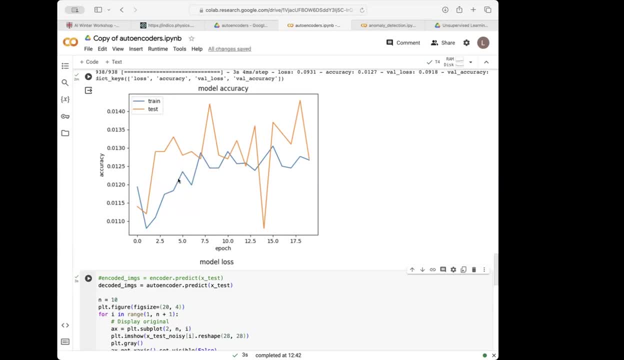 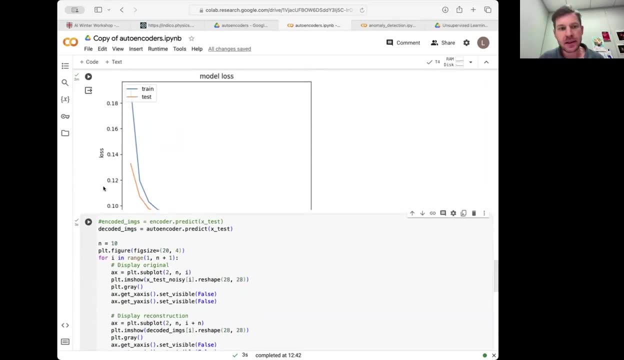 where accuracy is significantly less oscillating and much higher. Yeah, So yeah, in general, the goal here is to, you know, to have examples of how to develop these techniques. usually, you know, to have like a good performance you need much, much larger data sets, complex, more complex. 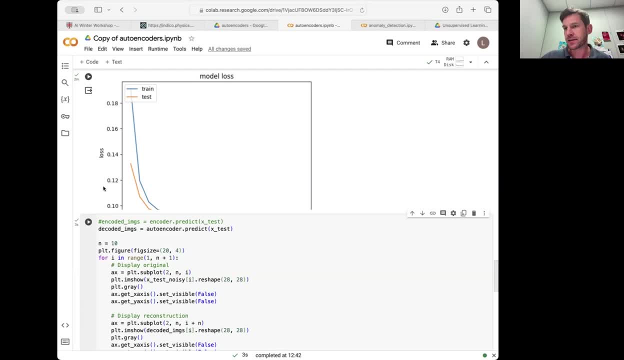 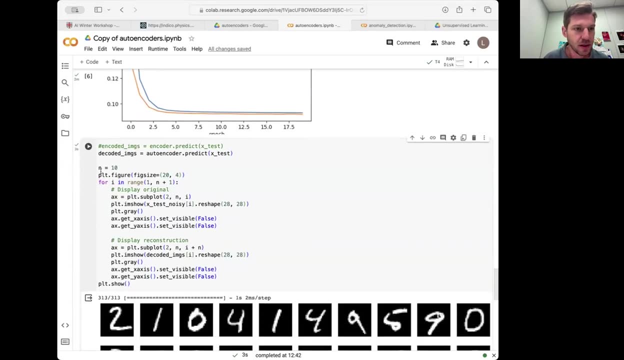 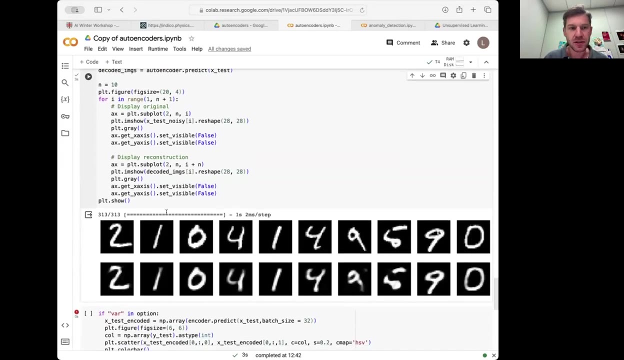 applications. but it's like a recipe, you know, adding one extra layer is simple. This is served as an example here for your actual research, progress, progress projects. Now running the next one is actually shows the original. I mean, we're trying now actually to predict effectively numbers right on the 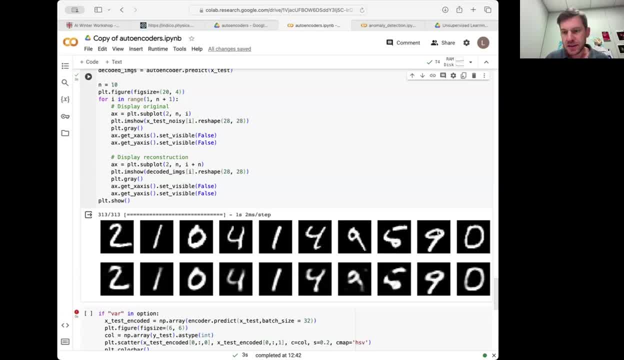 top row are the original numbers And on the bottom row is the reconstruction, what we achieved by with this, with this autoencoder. So the reconstruction is pretty reasonable. I mean more complex numbers, you probably more fuzzy ones. you see there are some. you know it's more poor performance. 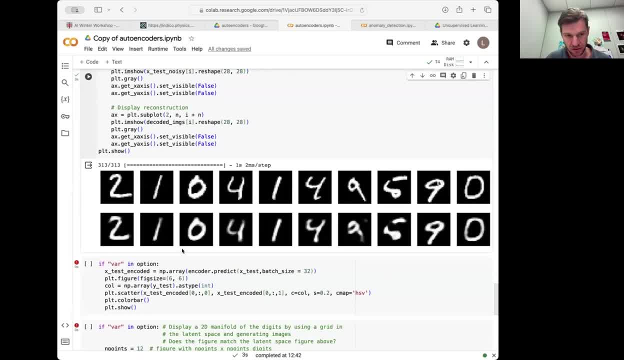 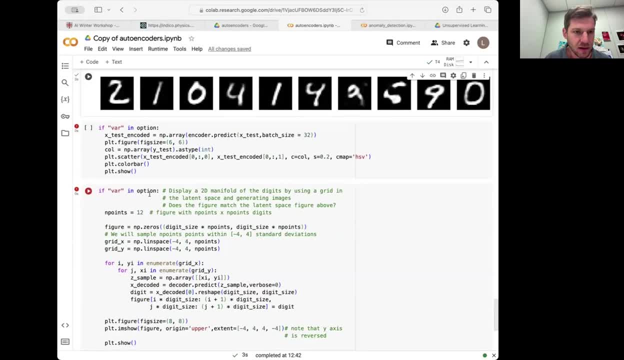 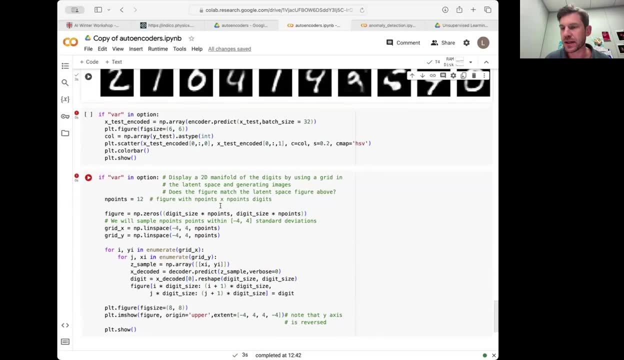 But I mean we will review again. this image is the bottom row. when we have a more complex algorithm. Yeah, I think we can skip this too, And maybe we can try a more complicated algorithm or add the noise in this case: run the same thing, but adding noise. 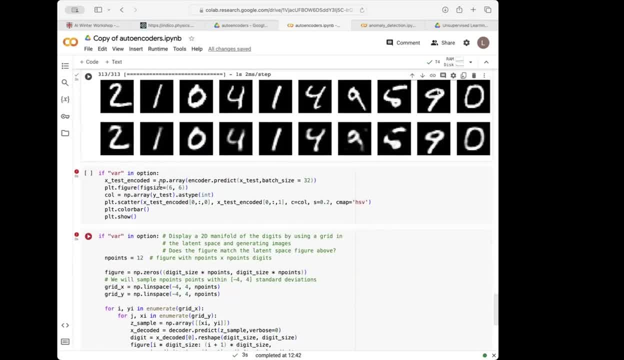 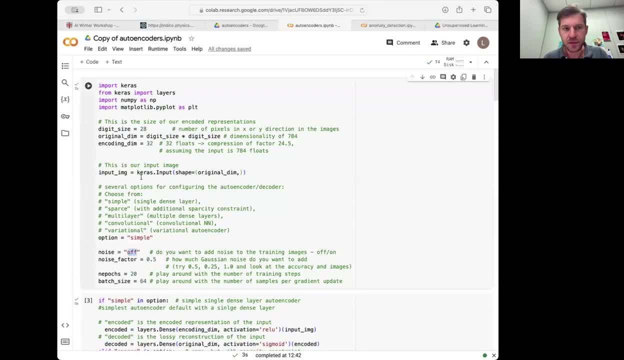 Maybe just the, let's run. maybe multi layer is the noise, Multi layer with a noise, Yeah. So let's go back to the first one, The first cell You have to change here and then we have to change, Or maybe, since it's fast, I would say: 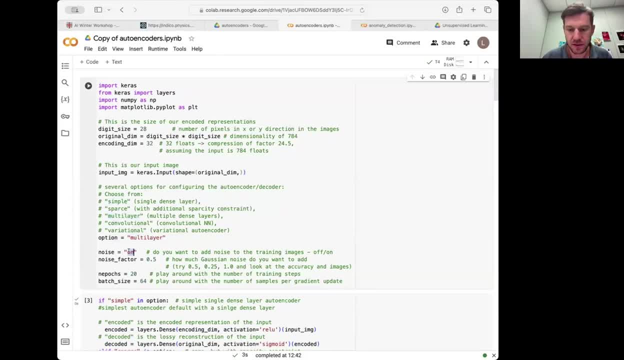 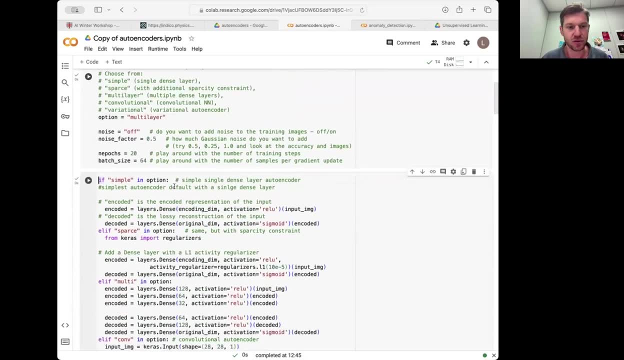 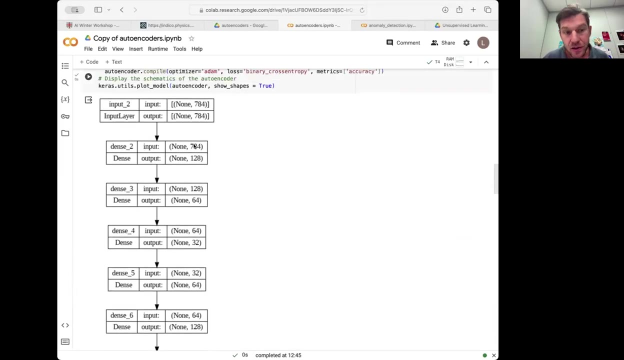 look, let's run the multi layer one with noise off, Just to see what we get, And then we can do it faster. now, So effectively, we just have to go to the results of click to run all of the cells. So here you see, we increase. So we are talking about here. 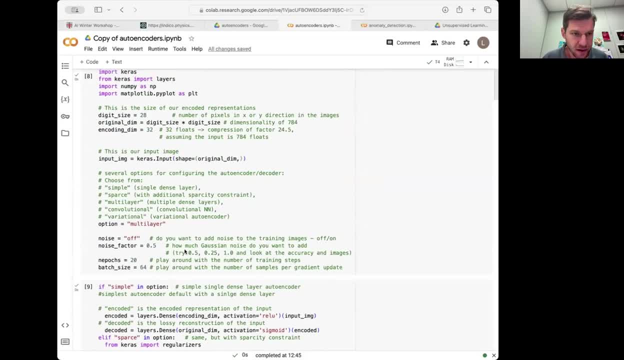 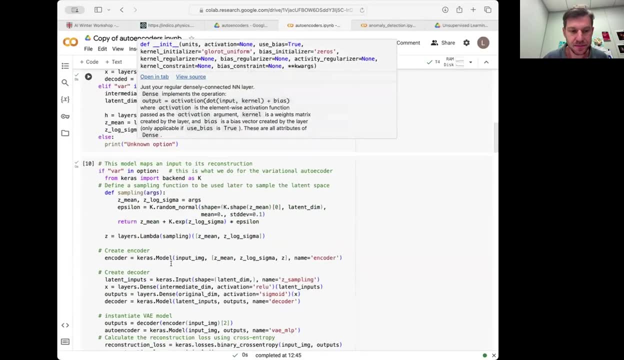 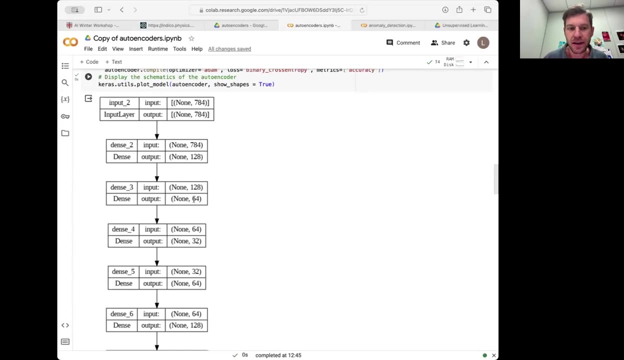 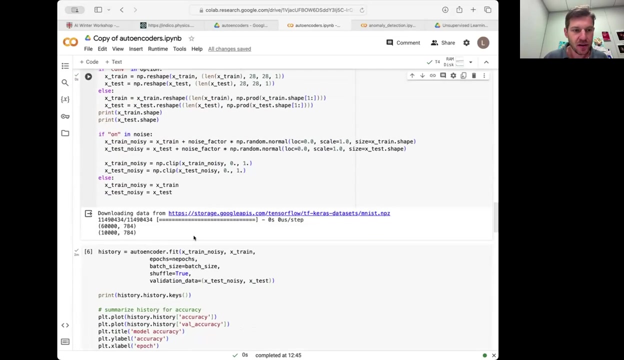 four layers, no five layers. Let's see really simple one, Yes, one, two, three, six layers. So this is shown. this is useful to understand what the network is doing, how many nodes you have. I don't think we need to run this one. 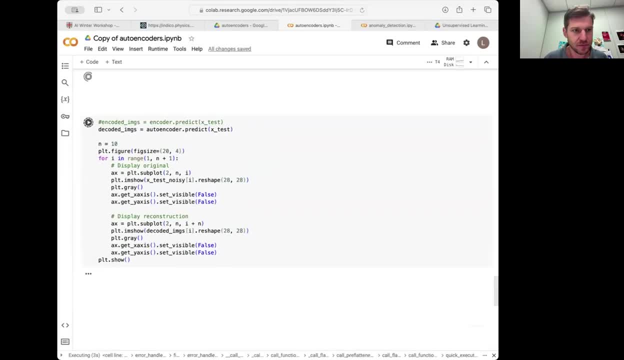 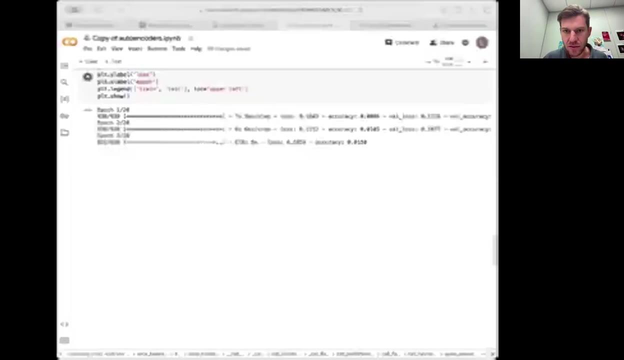 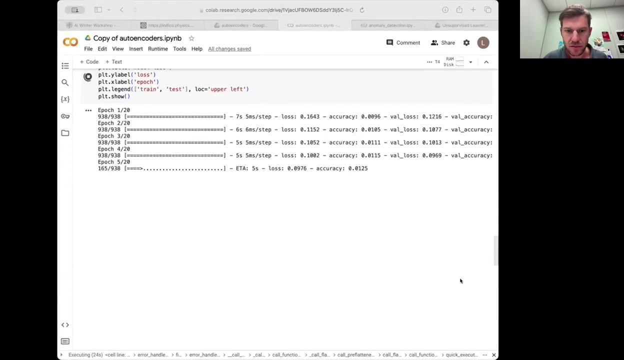 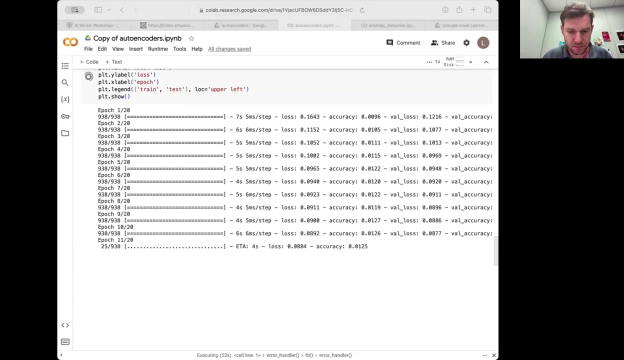 This one. So I assume if you have trouble running the code, you would drop a line. Yes, but if if you had to do it, you would just take this line. Now, if I can, I would go back to the first one and do it a little faster. 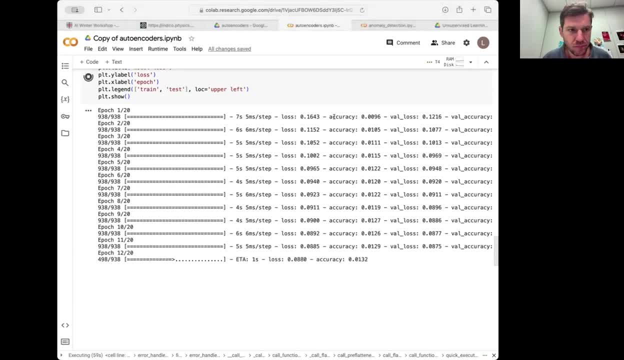 And that would get me to the screen, right? Yeah, and if if it's not there, it would get me to the screen attached so I could set it up. OK, So that's the idea. Yeah, So there's the full cell here and then the rest of the data, less than that. 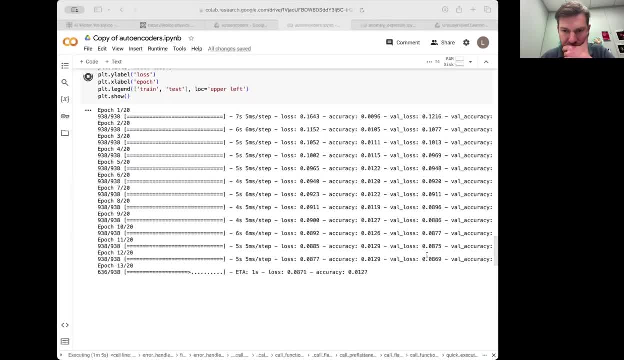 you have tochant it to the other side. Wait, is it working or not? Yeah, you have to 95% of it. So that's the big deal, Which is I mean? I'm going to look for it. Yeah, I don't think that's working. 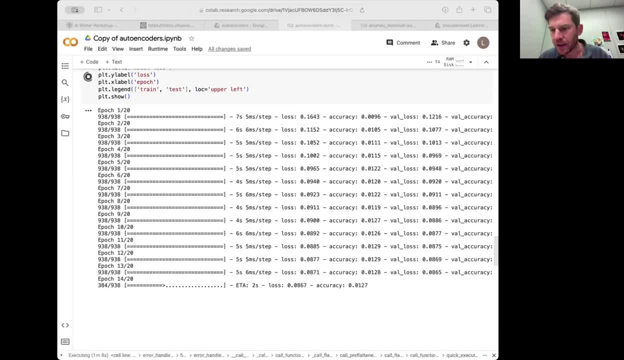 There is one question. it's in the file, OK, Right. So Yeah, there is one question, Yeah, Okay, Yeah, you answered it, And also depends on the task you want to do, if you want to do classification or regression. 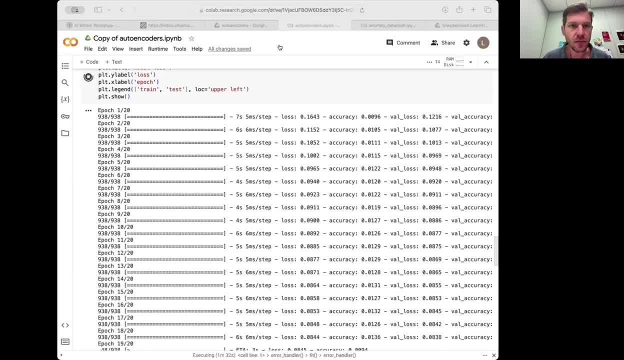 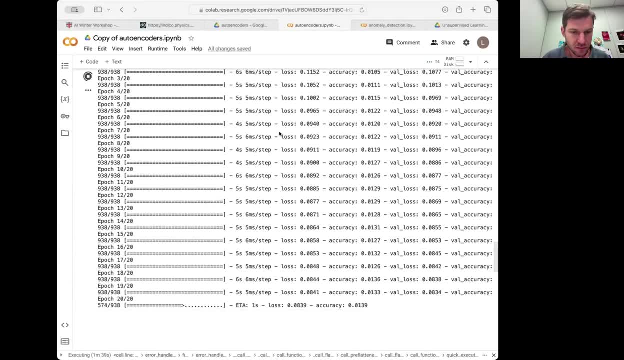 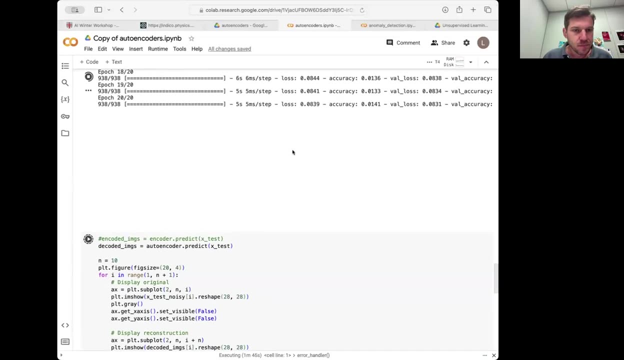 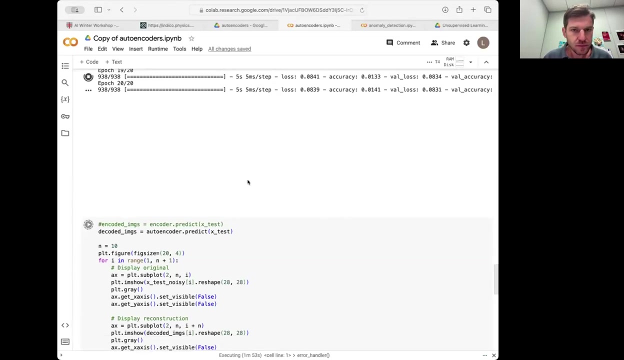 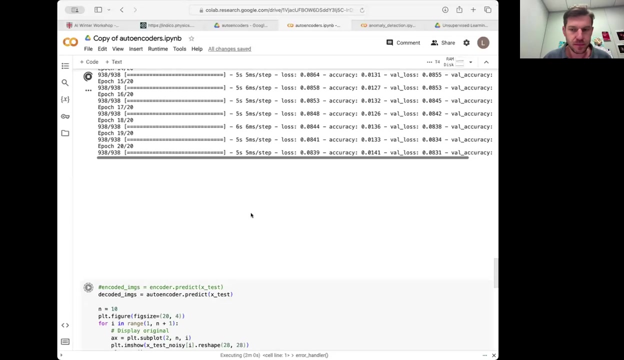 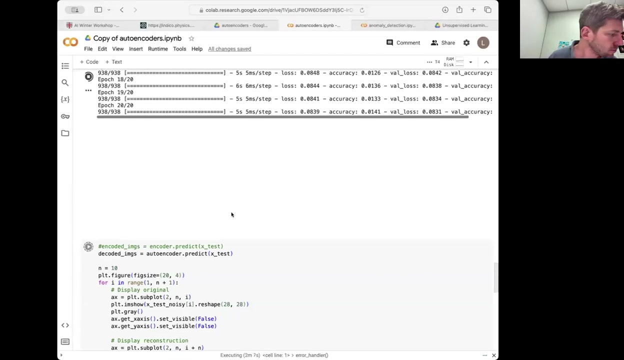 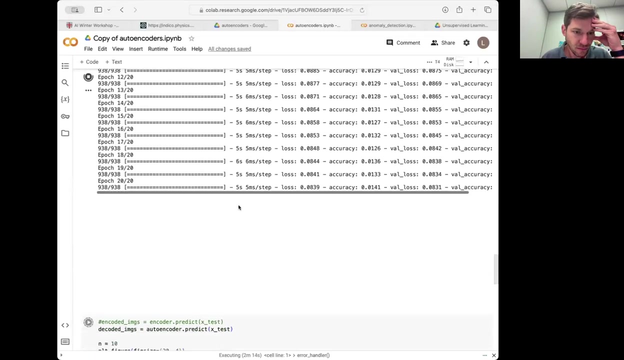 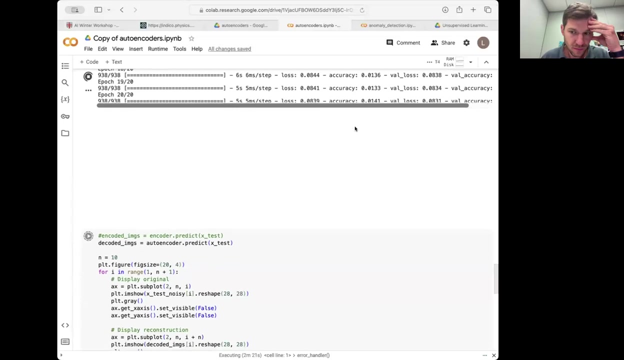 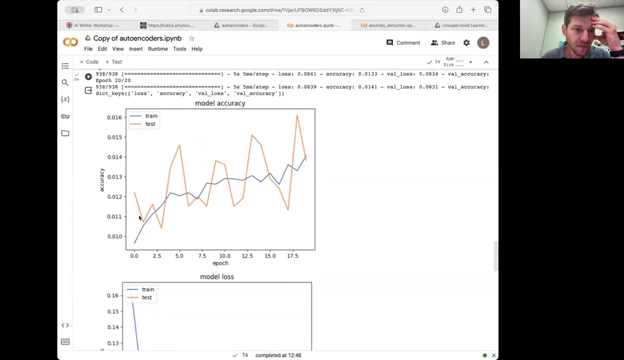 We do different losses, We use different losses. So here improved a little bit. of course there are some fluctuations that you see here in the testing. For example. these are statistical fluctuation in the testing sample. it's much smaller, has much less images than the training sample. 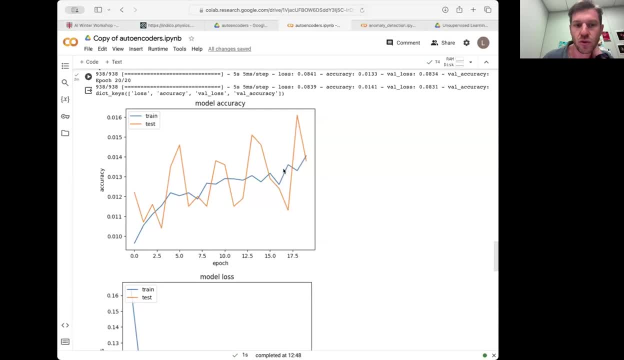 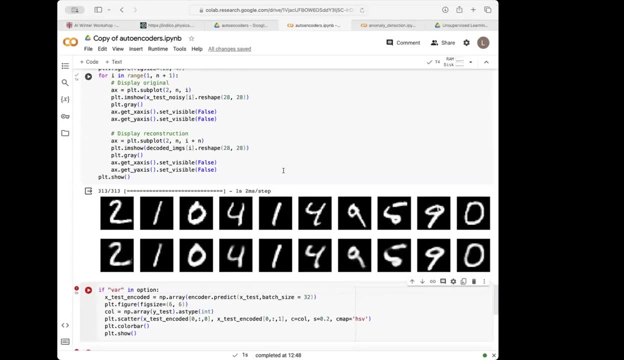 So that's why it fluctuates more, But in general, you see, the blue line improves. with respect to the single layer. Yeah, just to give some idea, this MNIST dataset is 10,000 images and I believe we use 9000. 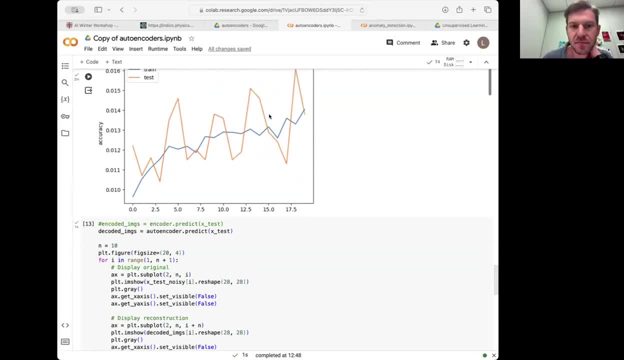 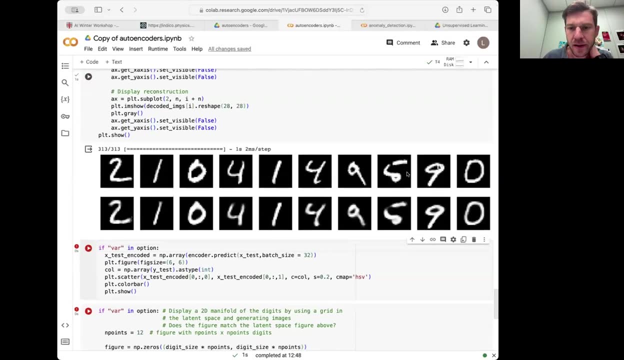 for training and 1000 for testing. Yeah, So for this case you should not worry Like about these fluctuations here And here you see actually that here you know five that was more tricky. here looks a bit better than what was how it was with a single layer. 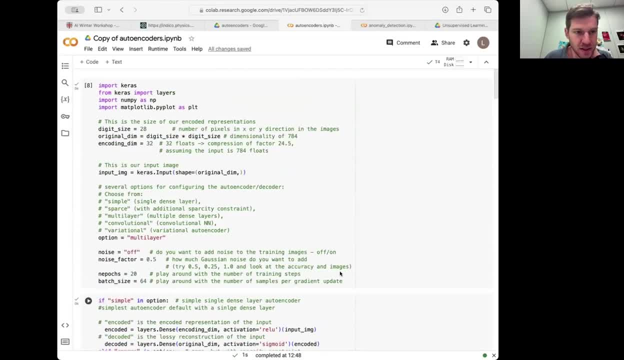 So now let's repeat this exercise by adding noise, with the same, just changing. including noise make it a little bit more difficult, the problem, or more difficult. So let me actually keep. I'm sorry, I'm sorry, I'm sorry. 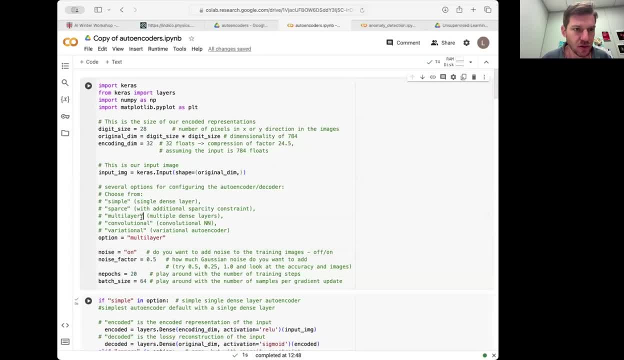 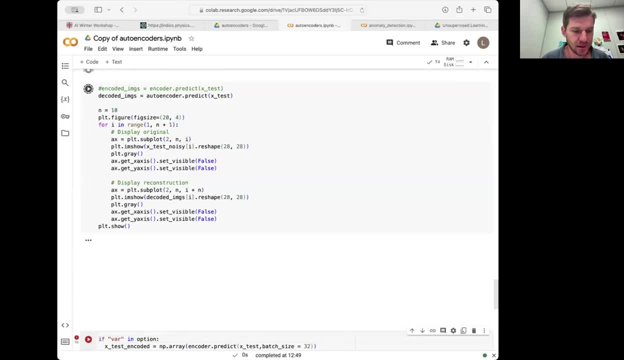 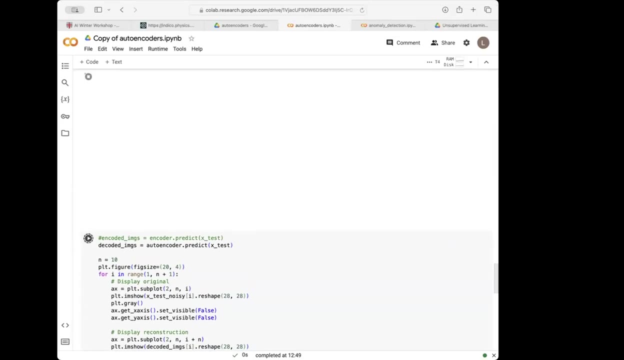 No, No, You don't like that. No, So let's run all the cells again. So here the way we include noise. we basically train on the images to which we added the random Gaussian noise. So random pixels are just lit up with various intensities and just Gaussian. 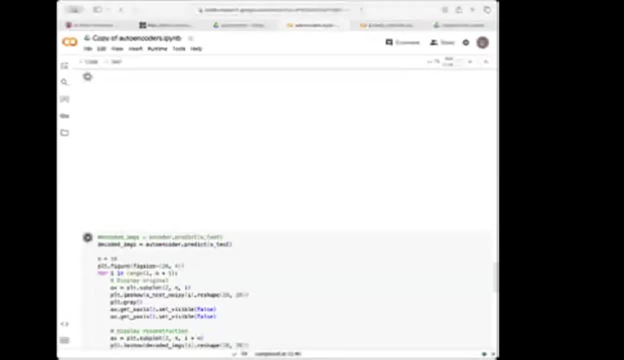 Yeah, Yeah, by just gaussian random noise. and what we do? we feed the autoencoder these corrupted data, but we compare it with the original images without the noise. this way we teach autoencoder how to ignore the noise but still not ignore the interesting features of the data set. 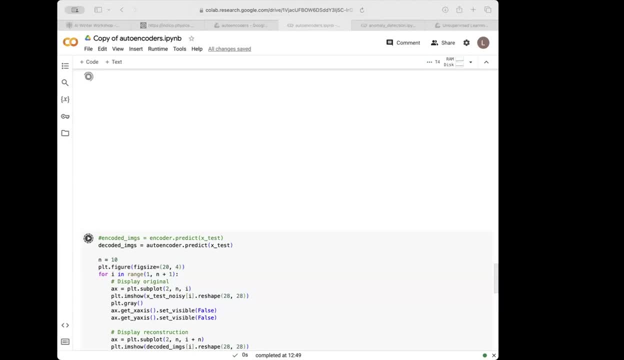 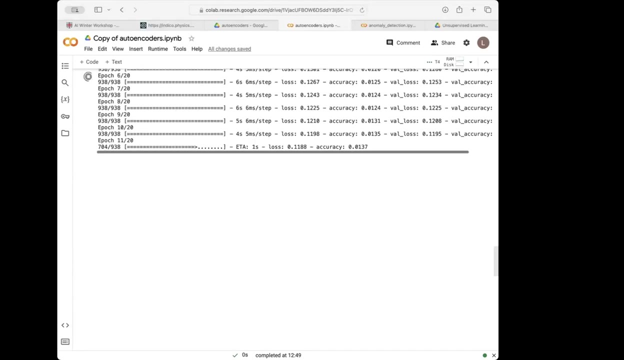 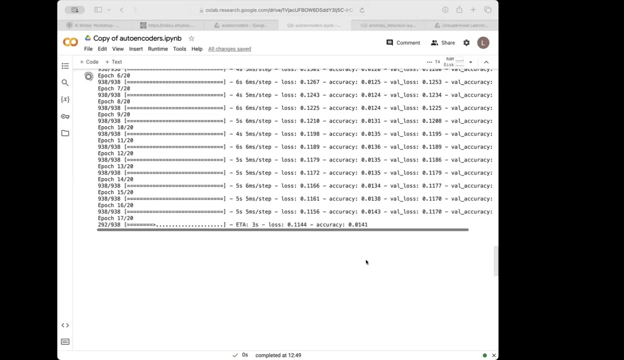 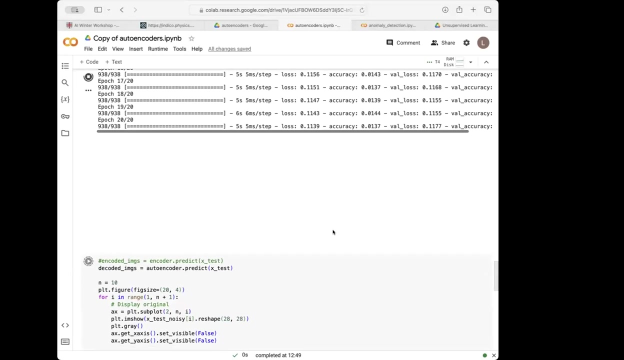 and you would see quite dramatically how it really cleans up the data. you, you, you see that the loss functions is higher than in previous case- it was about nine percent- because you're now really losing some of the features because you want to remove noise. that's good. 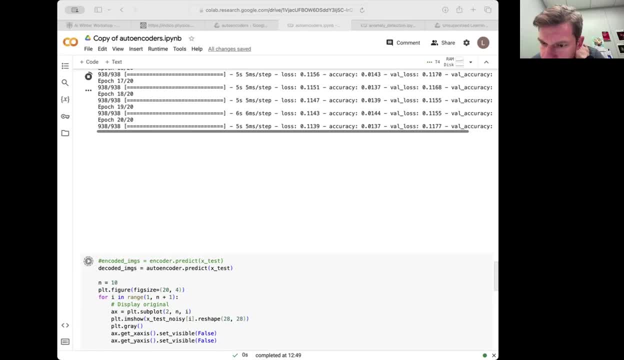 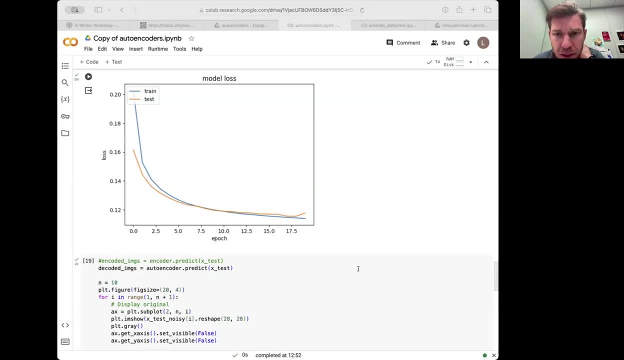 there is a question: where are the square terms supposed to go in the llp loss function for which supervision? so the llp loss is using the mean square error approach, right, and i think, if i remember correctly, is is the sum. so you, you have like the, you go in, but you have the. 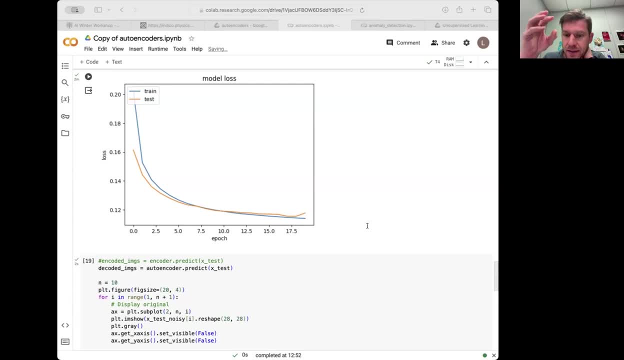 uh, you have one is the predicted. you have the, the, the predicted portion, which is um, sorry, okay, there keep coming questions, but let me answer this. so there is like you have the prediction minus what the truth. this is square and this all is within a sum across all your bodies and 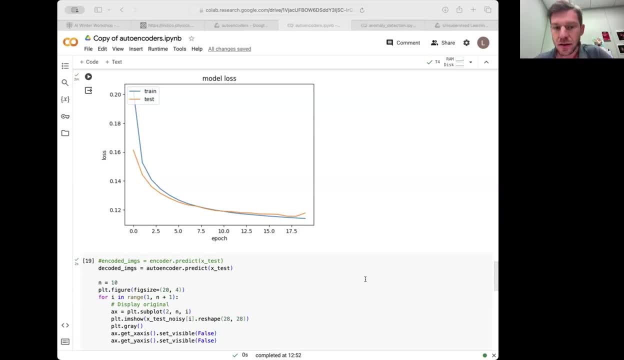 and divide by the sum of the number of bodies. So this is something like this. So it's there where the square goes, Right? Actually, I looked at the original paper. My original formula was correct. So the LLP laws they used, they didn't have squares. 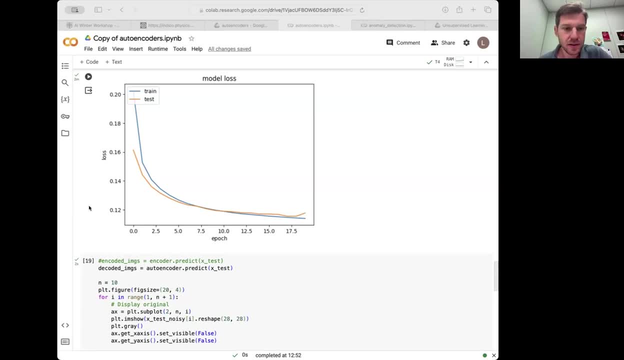 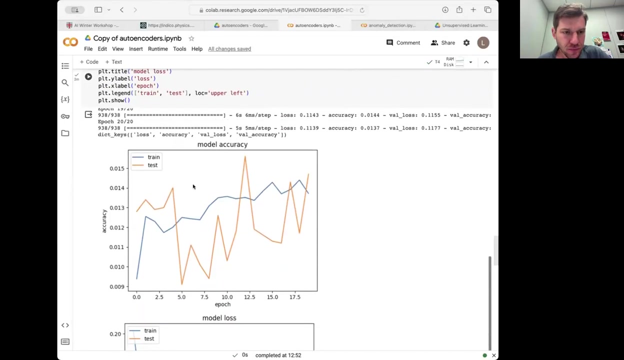 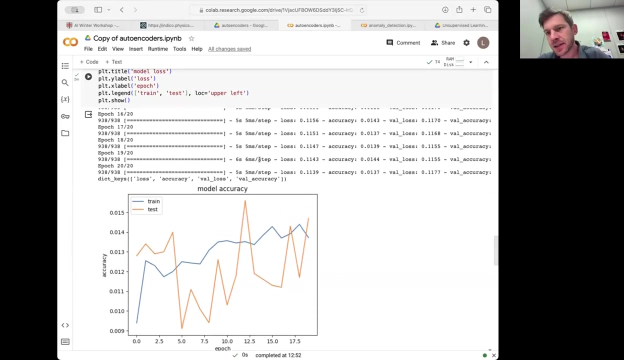 They just had-. Oh, they didn't have in the original. okay, So I'll correct my slides back. And so there is one question: Can we don't get exactly the same curve as mine? I don't think there is some. well, the events, the weights. 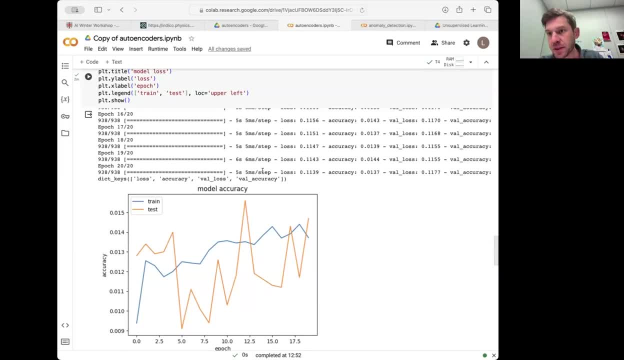 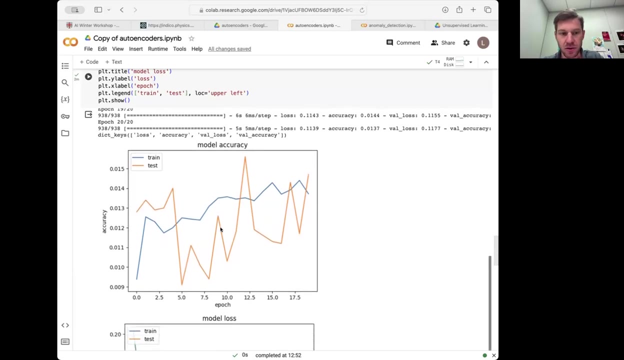 so there could be some effect from it. should be very similar, though right, Because the weights are initialized. There is some randomness, there is some. you know the initialization of the weights is random, So this could cause some difference in the accuracy or the laws. 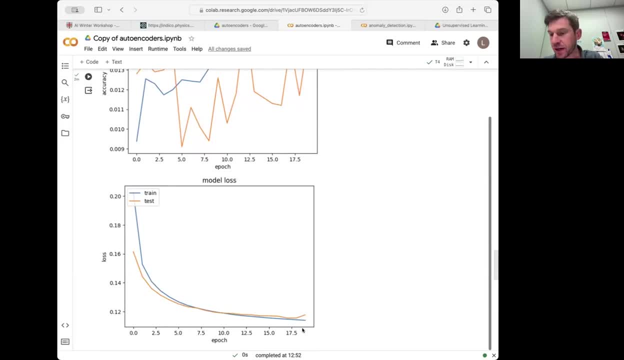 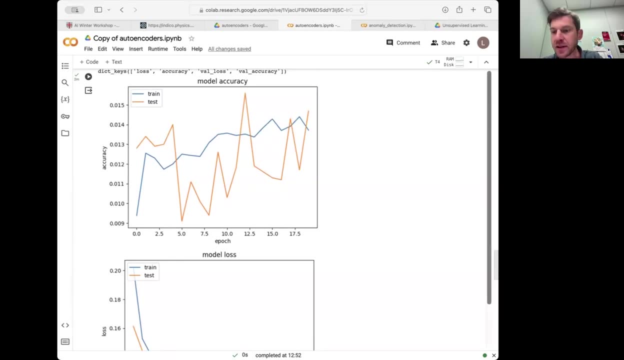 but I would believe this is at the beginning. Then you know, after you train a few epochs, it should be very, very similar. Ah, yes, You mentioned it. yes, Initiate the difference. This could be, but it should show up at the very beginning. 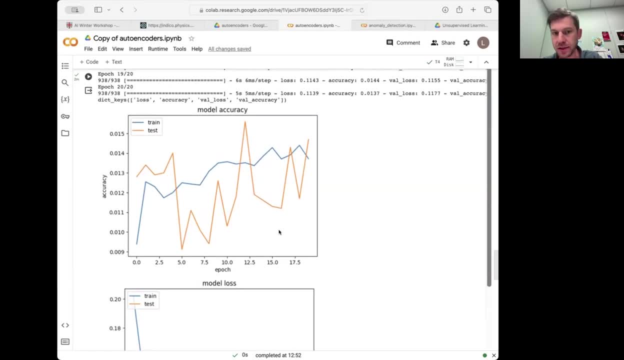 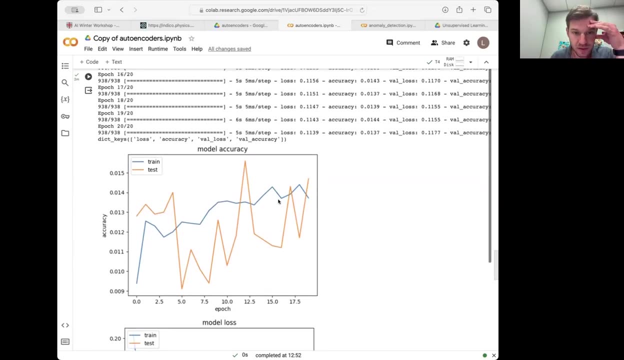 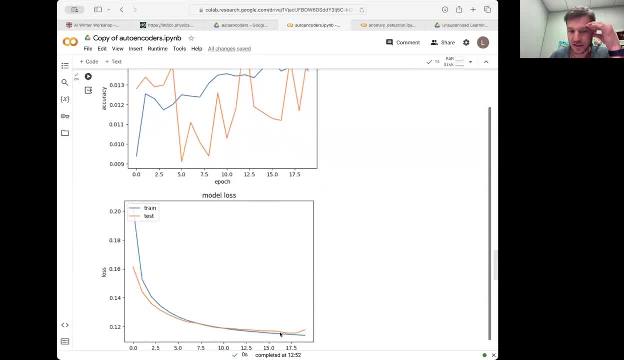 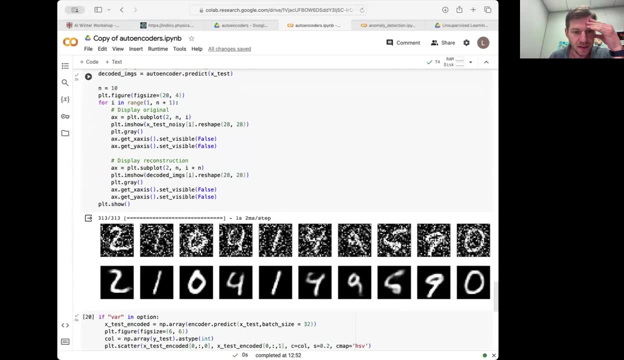 it's higher, it's larger. Also, the loss plateaus at higher values. it is expected, And this is how the image looks like with noise right, So we'll give a more difficult problem, but nevertheless it seems that the algorithm is. 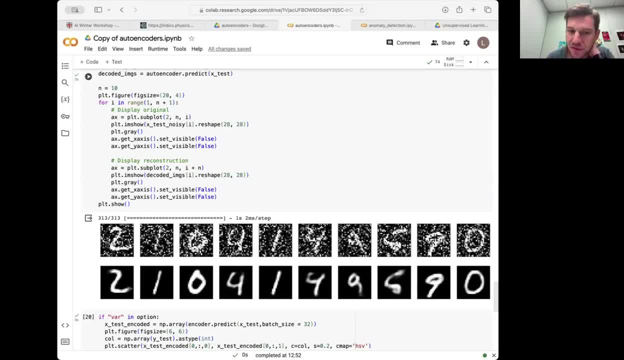 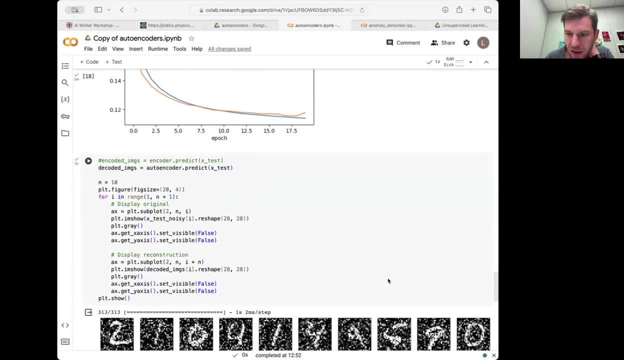 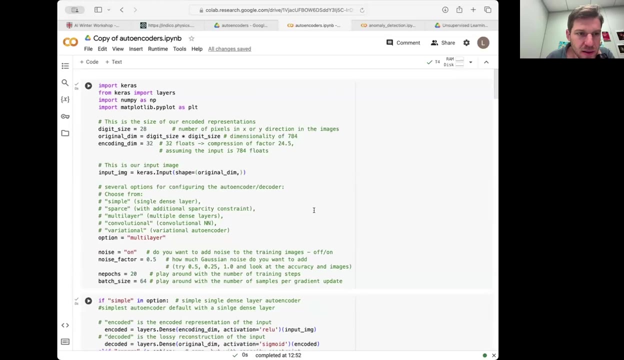 is is able to understand. figure out the, figure out the important features and don't mess up actually the prediction with respect to the noise. So maybe shall we. I would say let's do maybe variational and then Black. 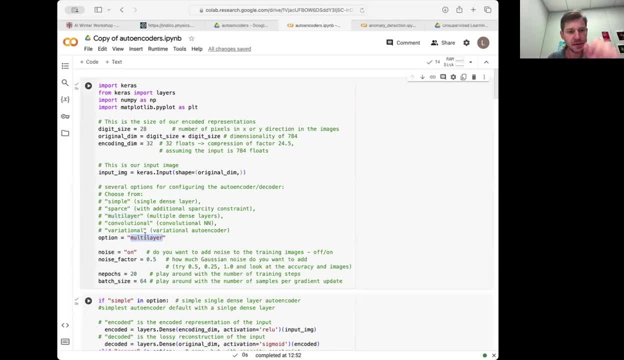 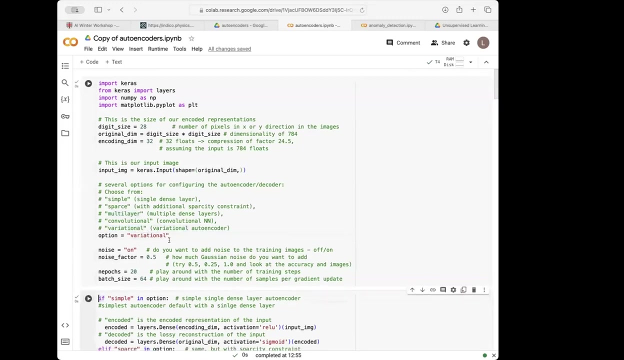 Uh-huh, Switch, Yeah, Yeah, to the second notebook. yes, variational. we could just maybe point out where this kl loss function is coded. so, yeah, yeah, let's do variational. so let's start running, and you know, maybe without noise, so that we don't, oh, yes, without noise. 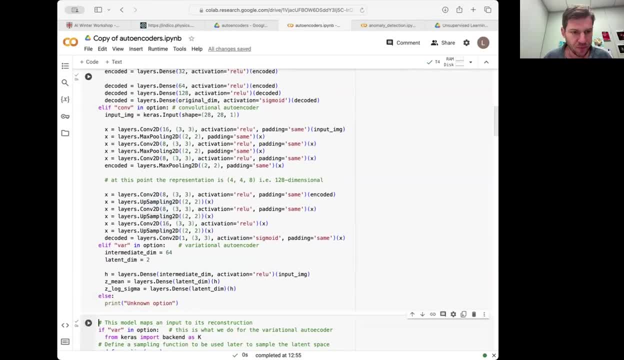 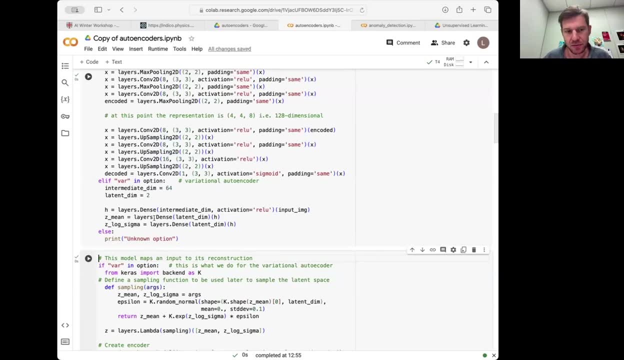 i think here you know, there's not much to add here with respect to what greg discussed in his slides. here we have, here we chose usually the gaussian, you have the mean and you have the sigma, and it shows two latent dimensions so that we could visualize the latent space. so, latent space. 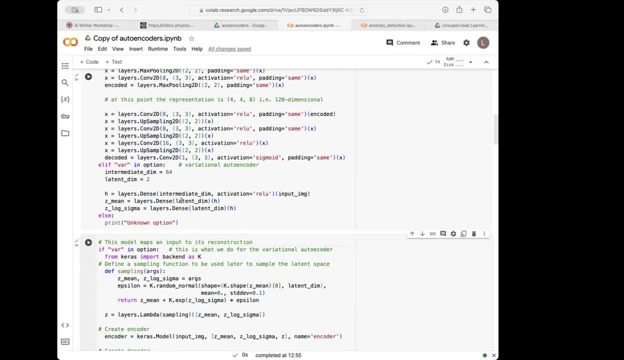 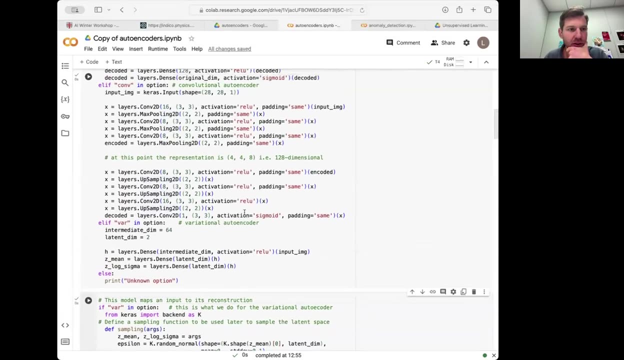 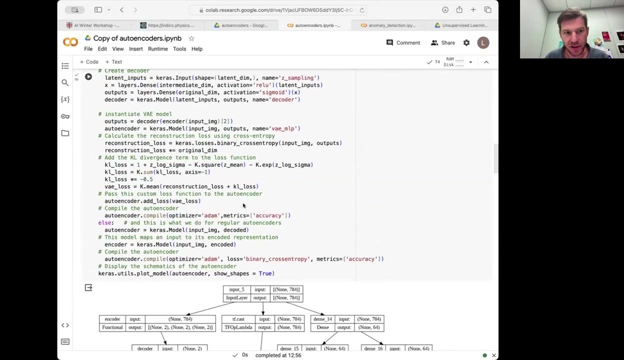 because now it's not a point, it's a whole function distribution. each point is encoded as the distribution, so you really have a two-dimensional space: x and y. think about this. so we encode everything in this two dimensional space. yeah, okay, and this is much more complex now, but let's take it like: try to. 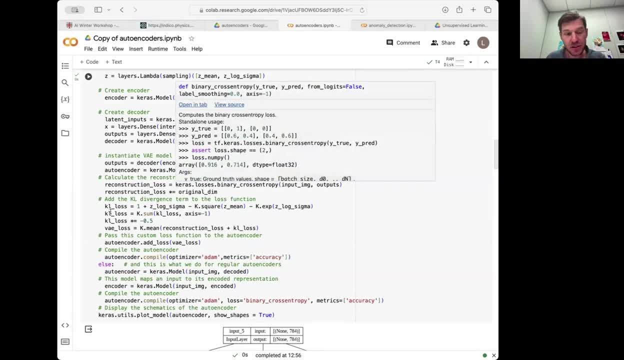 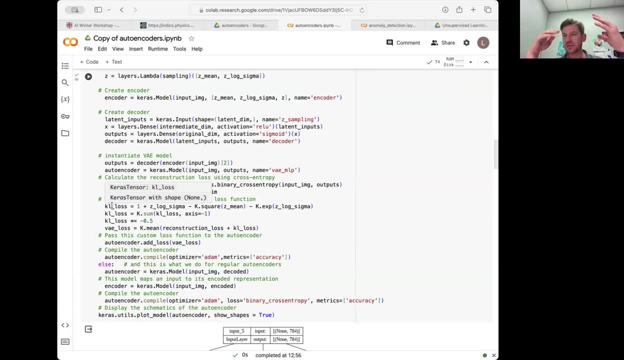 i mean the concept the same. but the other thing is that we try now we use this kl. the tool marks it's kl divergence, so we effectively think you have two distributions and you have to. you want, with this kl, this loss function, using the kl criteria, is to see to minimize, to optimize the weights of the network by minimizing the distance. 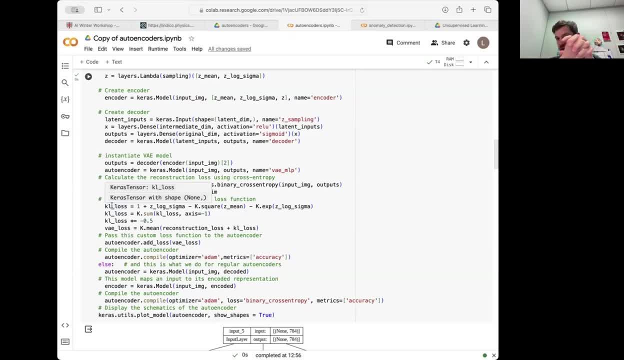 between the two distributions, effectively what the kl does. so it's a metric of how different are two distributions. so you minimize both the reconstruction laws, which is just how well you reproduce the image. but the second trial realization term tells you that we want two galaxies to be close to each other. 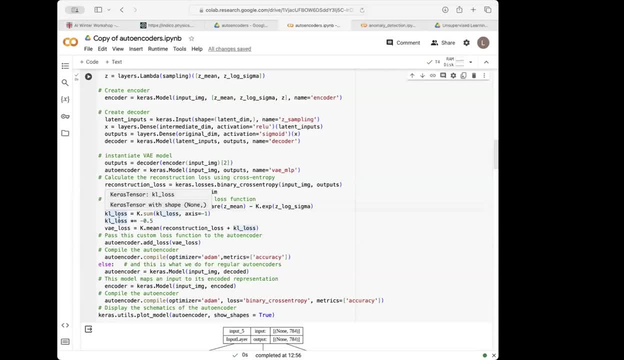 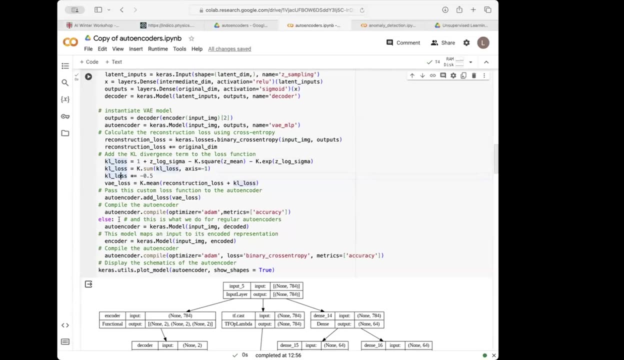 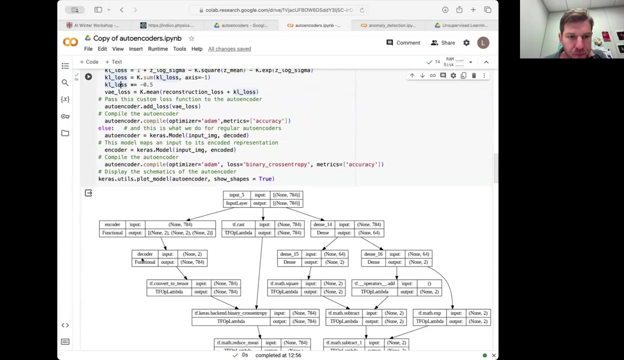 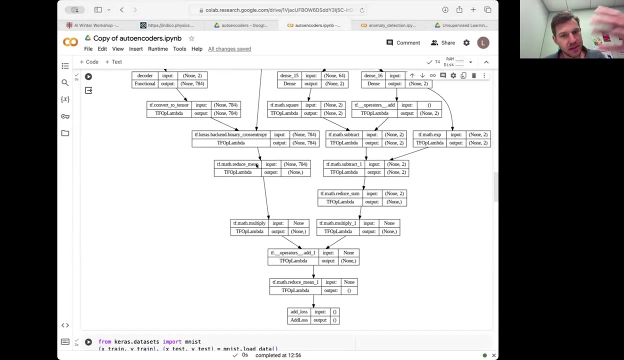 yes, but basically that ensures continuity of the space. two spatially close- well, two images which have very similar features would end up with very similar encoded distributions. and this is just the kl loss for gauss and distribution, the formula i gave you in transparency. yeah, and this is actually, you know, as we discussed earlier. but now, 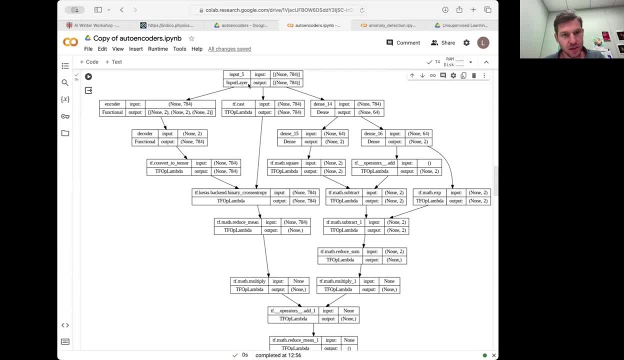 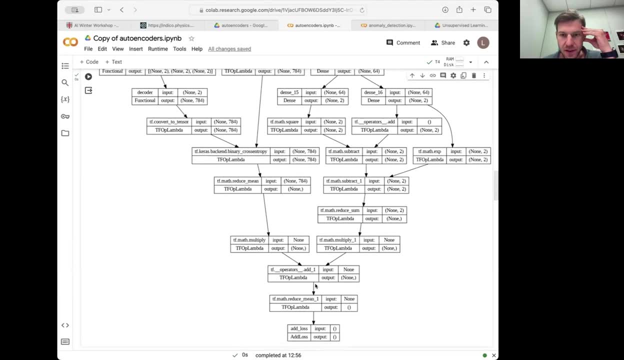 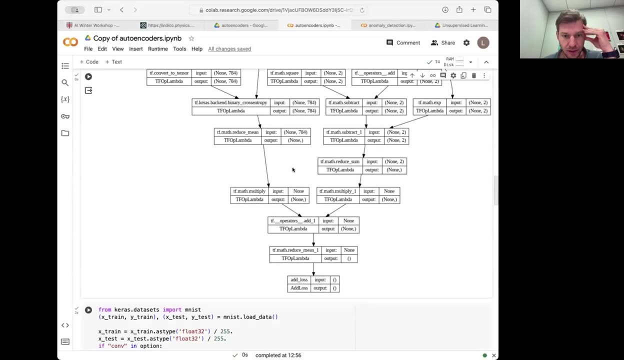 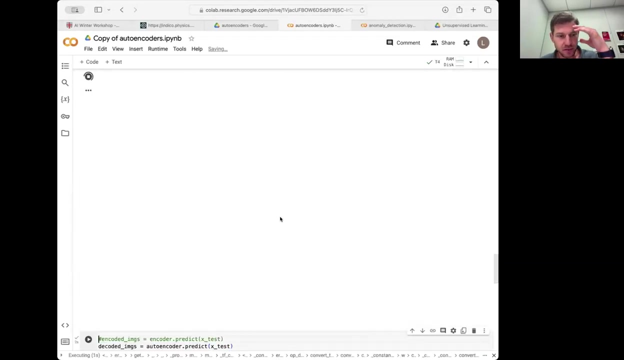 the network is much more complicated. so this is actually particularly useful in more complicated networks to figure out, to effectively, you know also to spot in issues on the design and understand how the network works. here now let's run also the steps, and the train take the most time. 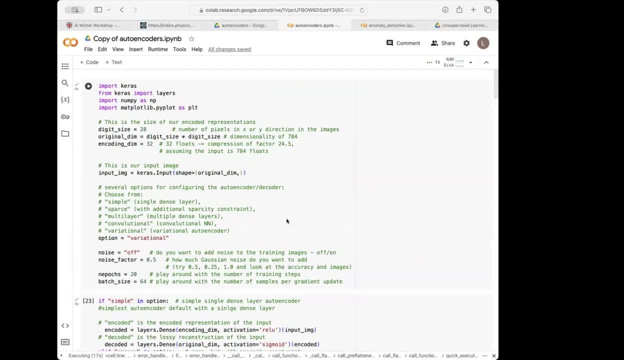 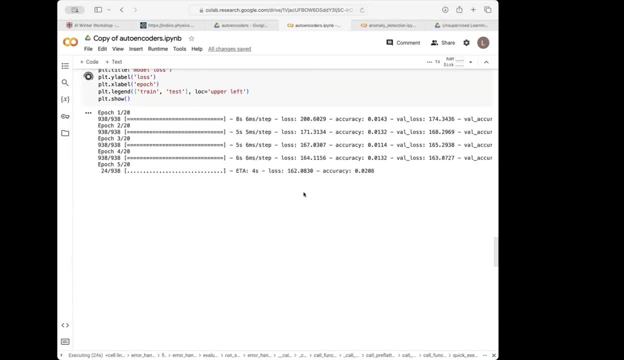 i removed the noise right. yes, yes, you did. yes. now the loss is very different here because the loss has this significant KL component, so it doesn't have the interpretation of the reconstruction area, some average between the two chirps. It's important that it decreases. 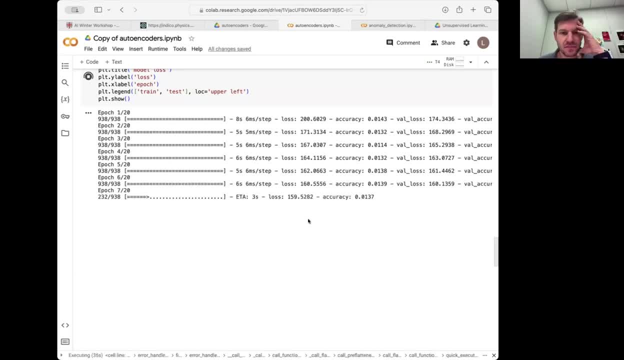 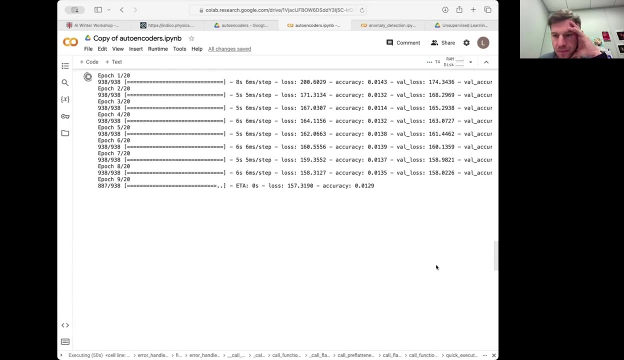 but the absolute value is not so good. Yeah, There's also another question: Can you use a model that is trained on no noise data and predict the noise data? Yeah, so this goes more on the anomaly detection. I mean, for instance, in experiments. 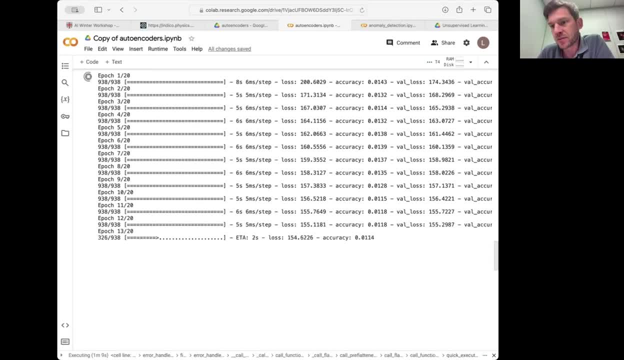 Greg actually gave an example. I mean you train on a hypothesis that you know on the background- for instance, a process that you know very well, processes or jets that you know well- and then you try to look for something that is abnormal. 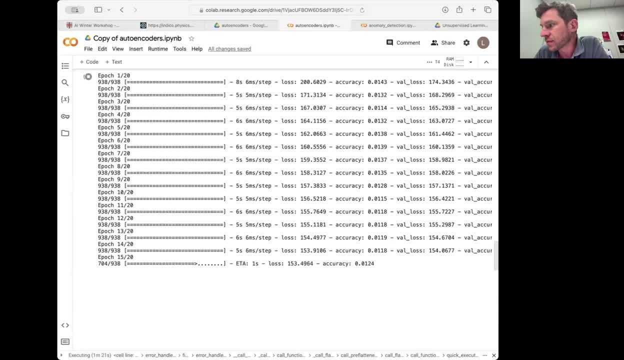 This could be because it's a jet structure, for instance, that we haven't thought or is not in the physics we know It's called the standard model of particle physics. We also try these things to spot malfunction on the detector, for instance. 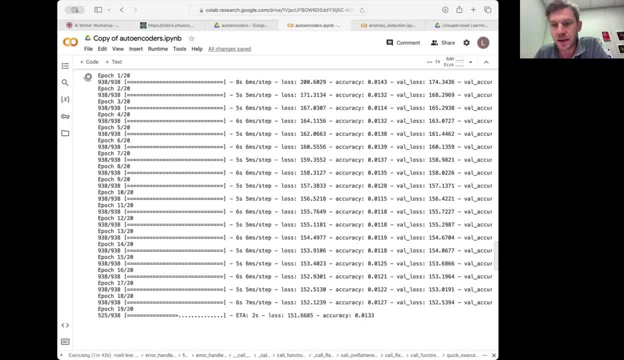 You train using, using, let's say, data taking periods that are very short, that you know that the detector works well, and then you test it on data taking periods that we haven't seen. We call it runs. I mean, and if it is something different, differences. 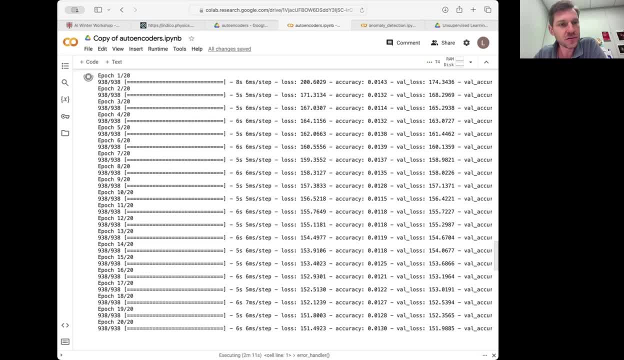 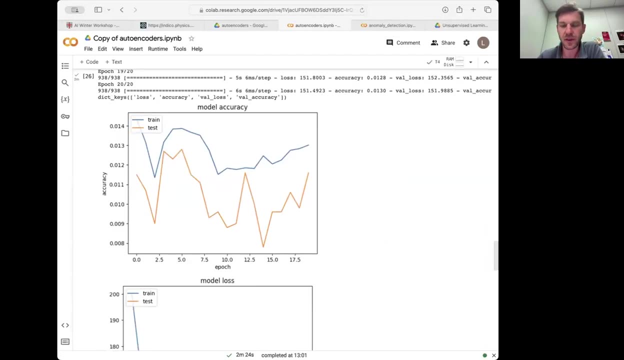 I mean, depends also you have to the region you select on the loss function you then you pay more attention on the specific part of the detector. So, yes, this is something that, yeah, we do, I mean, if you train on no noisy data. 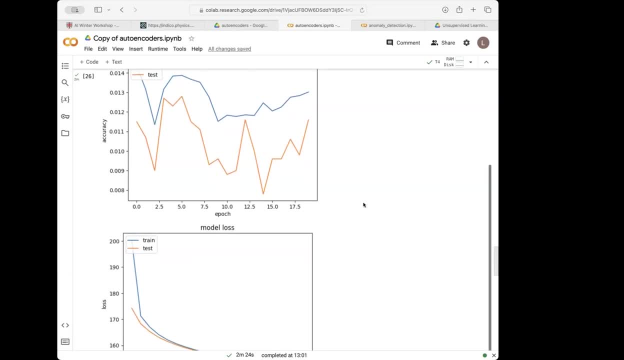 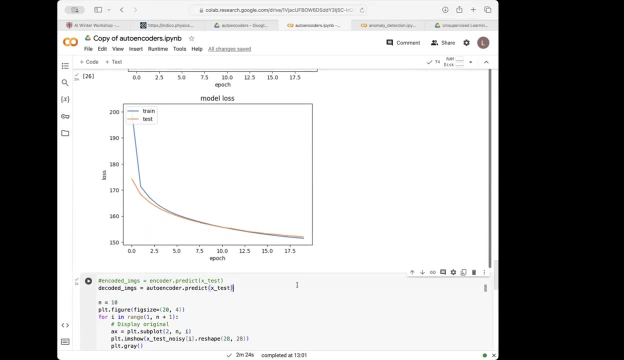 Yeah, you could try. I mean, just play around with this, just swap out noise and no noise. You probably generate some noise by having to try this. but yeah, Yeah, Yeah, Yeah, I mean this is again. 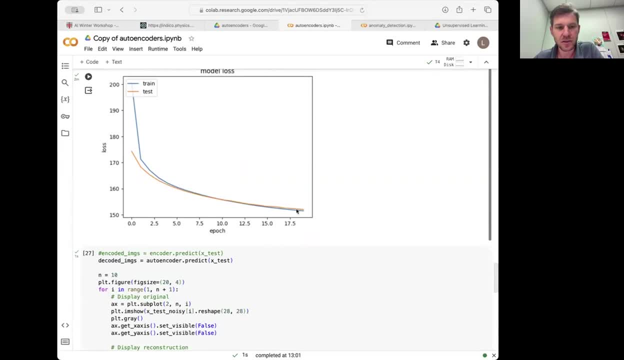 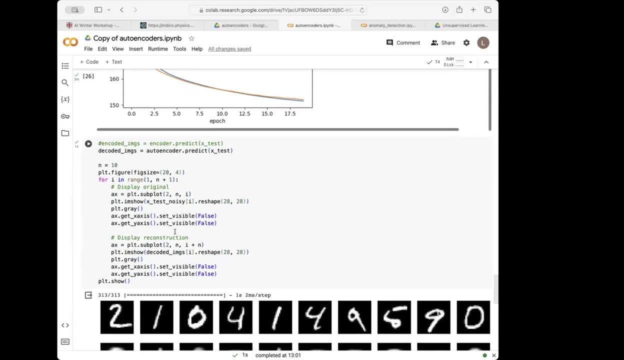 model accuracy and the loss, as Greg said, improves. you know it improves, but also for the reason that Greg mentioned, effectively it's at much higher values Here. 20 steps probably are not quite enough. You see that we still-. 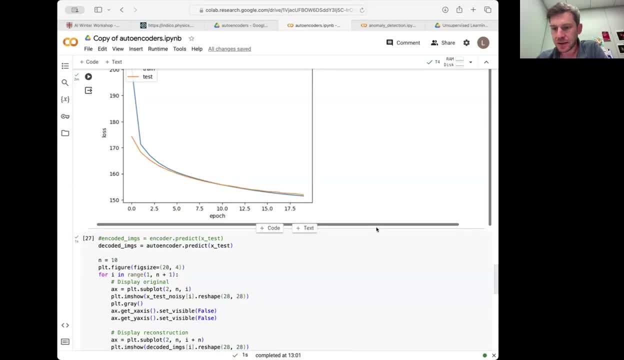 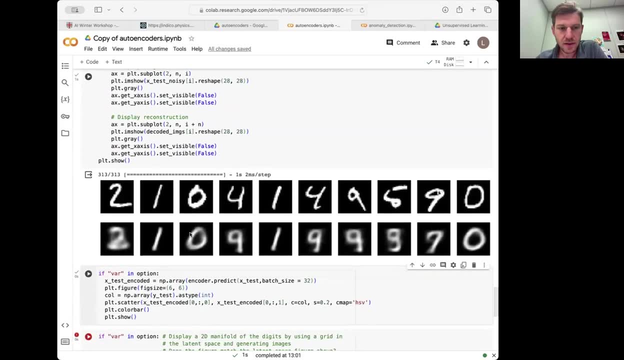 Yeah, it doesn't reach the plateau yet, And so you see there's some errors. Four is reconstructed as nine, for instance. Yes, But if you train a little bit more you would actually have better. I know that when I run it with 50 steps. 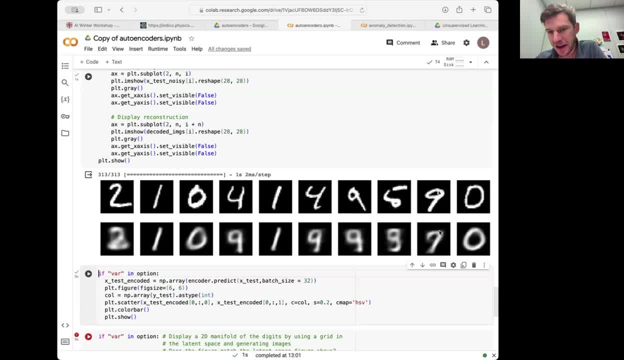 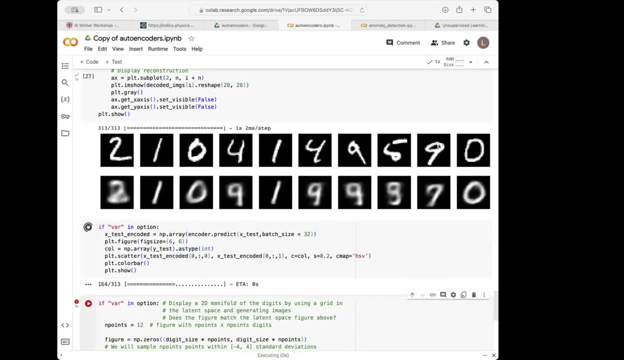 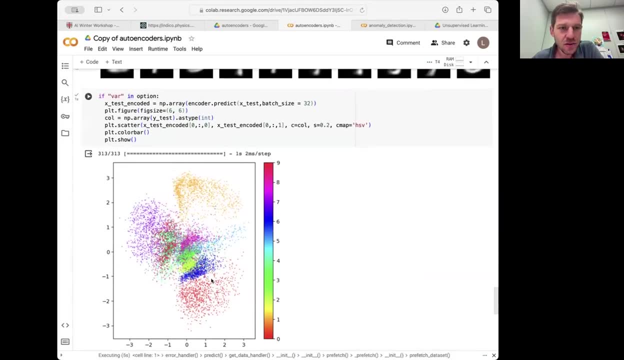 it was much more accurate. Yeah, Here, the nine here could be, as maybe I'm not sure if it's nine or seven. Yeah, But let's see, because the color maps are really-. Yeah, Yeah, Yeah, Yeah. 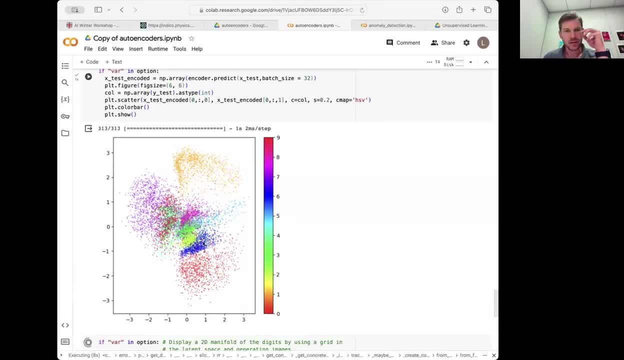 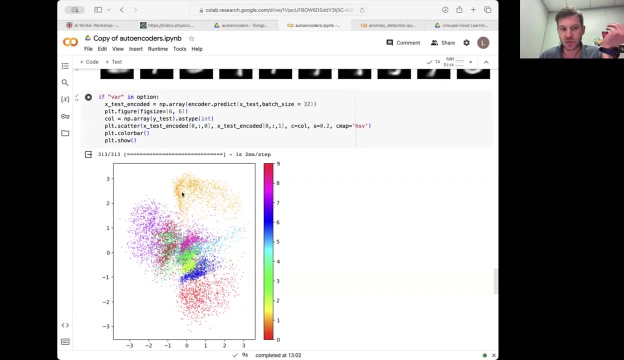 So this effectively shows you. this would be like 10 classes, right, 10 categories, but it doesn't know a priori how many are the categories. So what it does? it clusters, it positions in this two-dimensional plot. 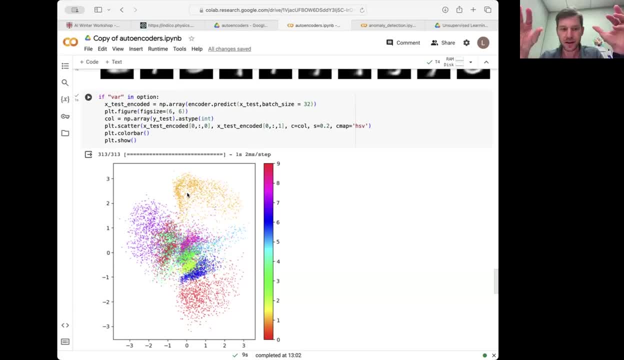 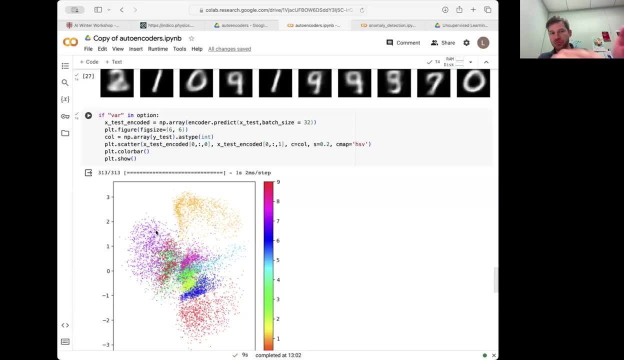 different numbers to different areas. So, in a nutshell, what it does identifies that the different numbers have different values And features. And you could think, okay, we do it with numbers, but someone, for instance, I don't know- 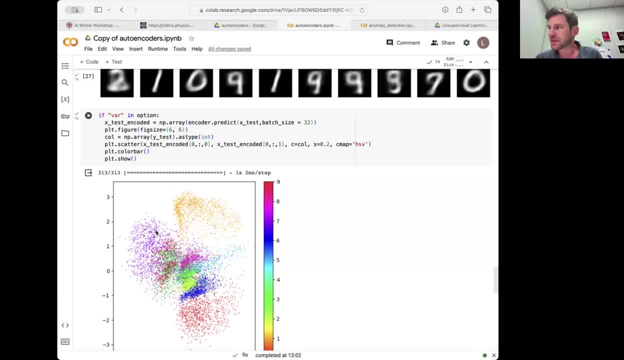 in problems to be even unrelated to physics. if you have different cases a priori- you don't know how many cases you have and you want to classify. you have, like I don't know, different animals: cows, dogs, cats or something else. 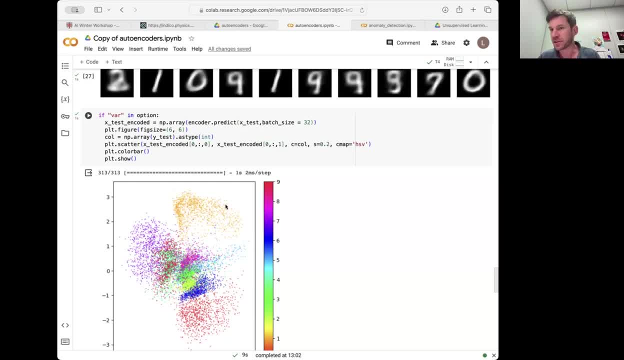 then you can use this code and it will create clusters of points, clusters of images in different regions, And yeah, I mean this is a kind of- you can think about it also as a clustering problem, Now, of course, I believe, for instance, 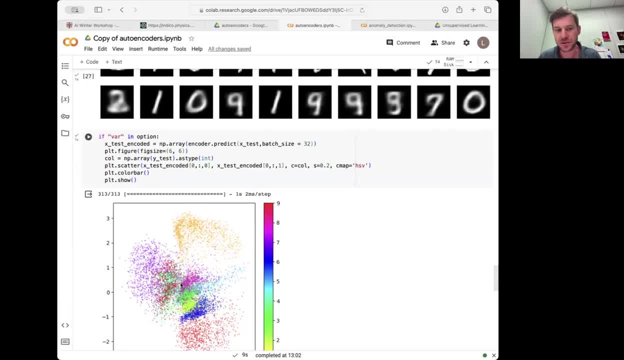 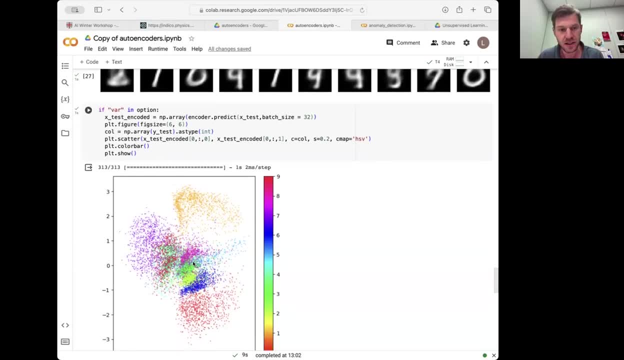 four and nine could be close to each other here, because there is some confusion. I mean those that are closer. the algorithm has some more difficulty to separate them. Would be interesting to see how this image improves. It should improve. I mean, Greg tried it up to 50 epochs, but you know. 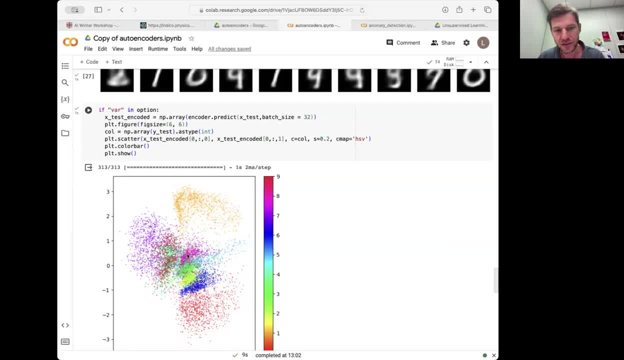 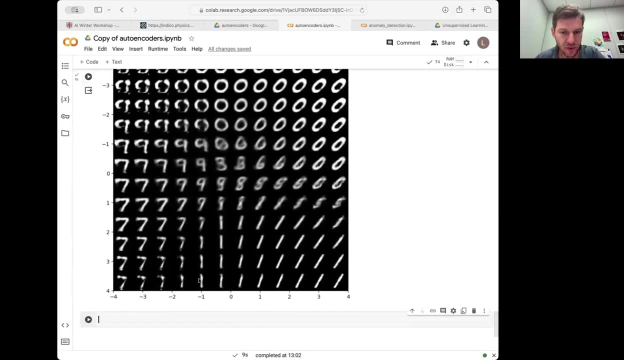 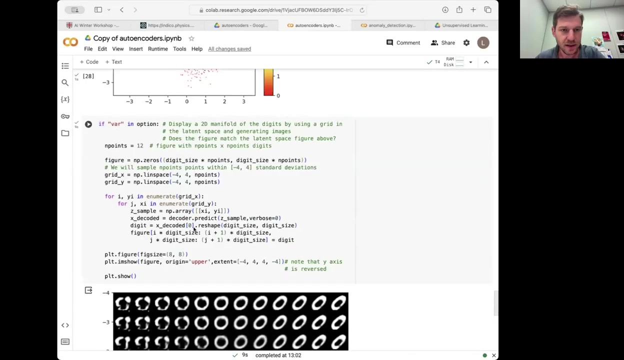 if you want to play- I mean later in your free time- you can train more epochs and see that actually, these different colors, these different clusters become more and more distinct. Yes, so I think this is the same dimension. yes, exactly as what we see here. 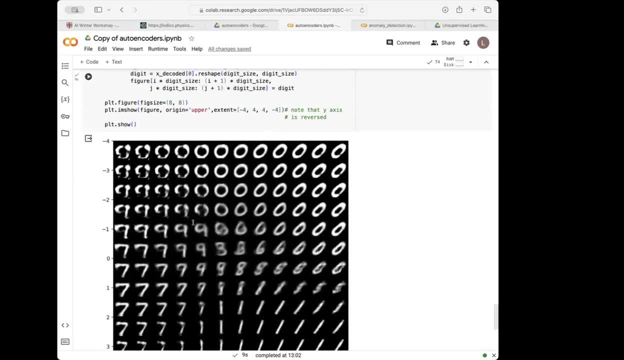 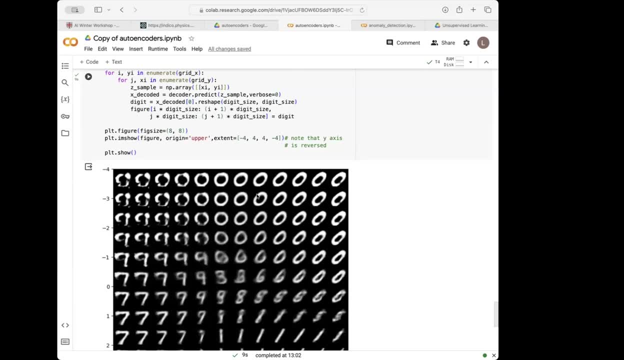 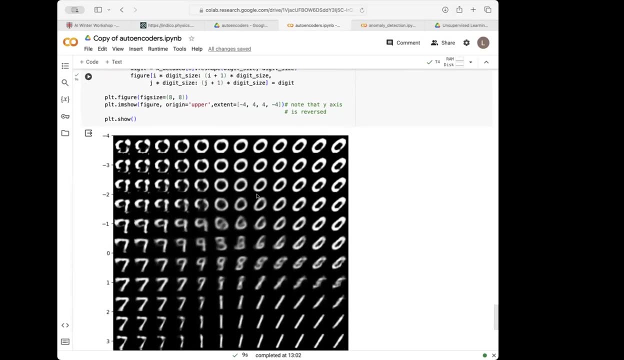 So in principle, Yeah, exactly that there is minus. so the problem is that the way this image is created, you cannot easily plot them so that they correspond exactly to the map. So the minus four is at the top here. 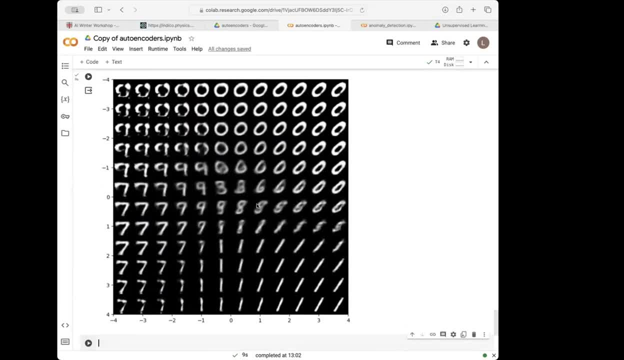 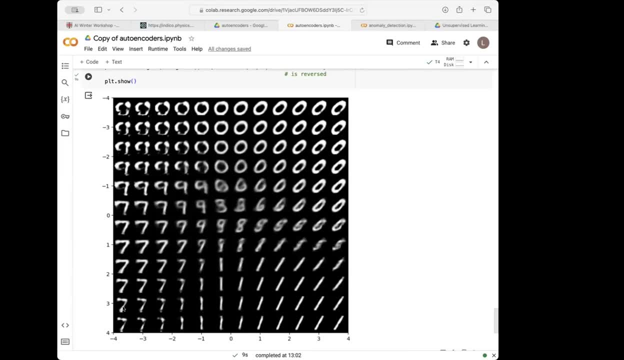 and plus four. Yes, yes, it's just yeah. Essentially you could compare, let's say, where these sevens are concentrated. So that's X of around minus four minus three and Y of you know. 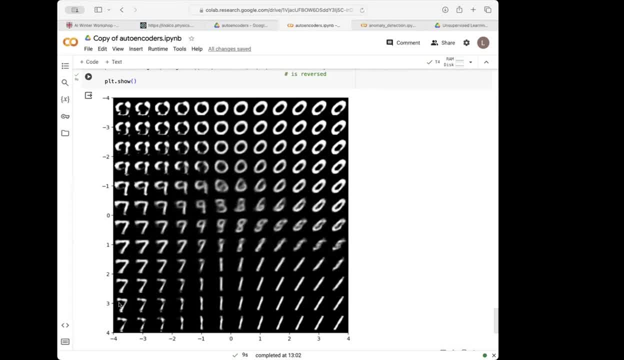 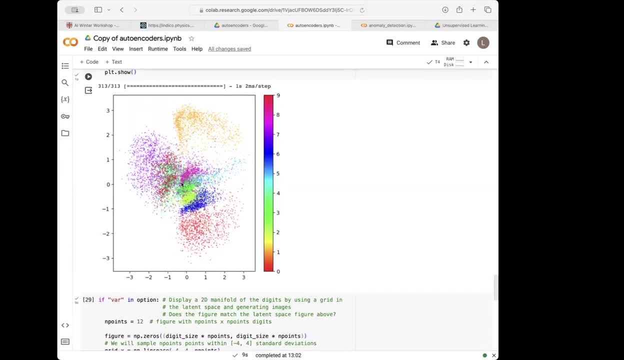 Yeah, Sort of zero, near zero. So we could go back to the color image and look at minus three and around zero and you see this violet cluster which is seven. So that allows you. yes, so what this manifold you see at the bottom? 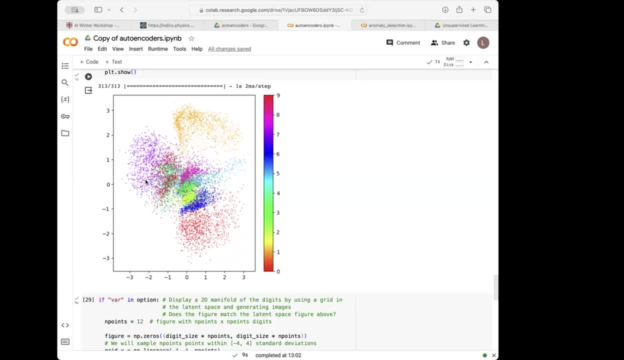 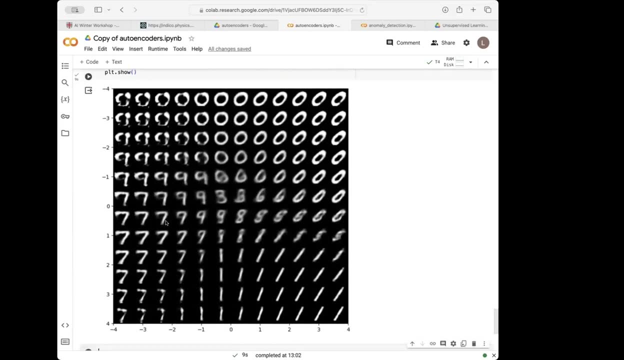 essentially we take a rectangular grid over the entire space minus four to four, and some of this is not even populated by the train data. But we generate images which kind of merge from one digit to another And this is not very visible here. 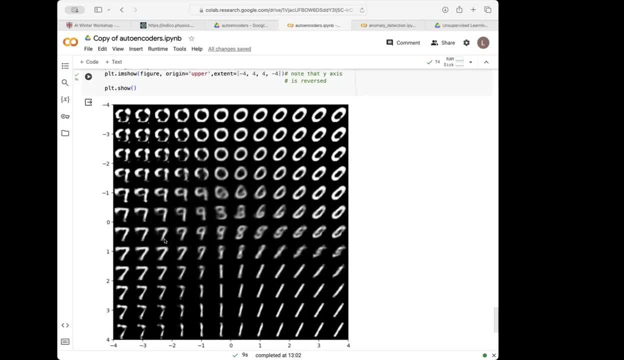 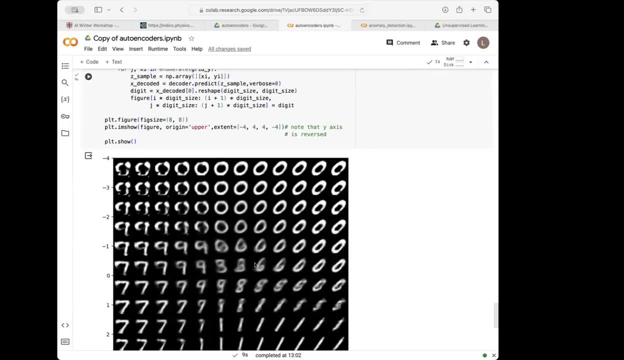 because the training wasn't sufficient. but if you train for 50 folks, you see very well how nine becomes three and three becomes eight and all these positions. So this is how you could. you know, if you have cluster of cats, cluster of dogs. 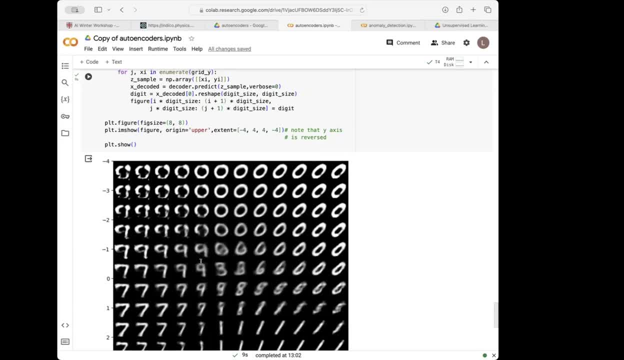 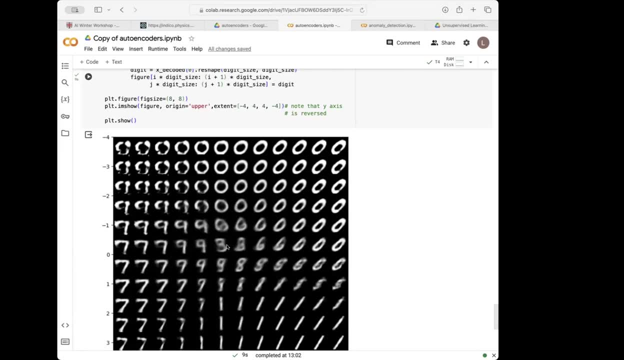 you could take a point in between and would be: cat which looks like a dog or something similar, Yeah, Or you could create some artificial animal by picking a point which wasn't even occupied by the train data. So that's how people generate images. 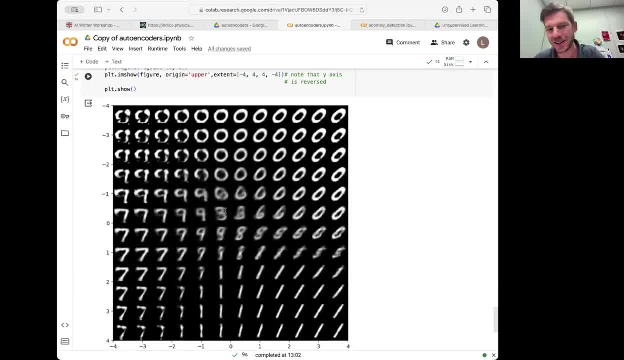 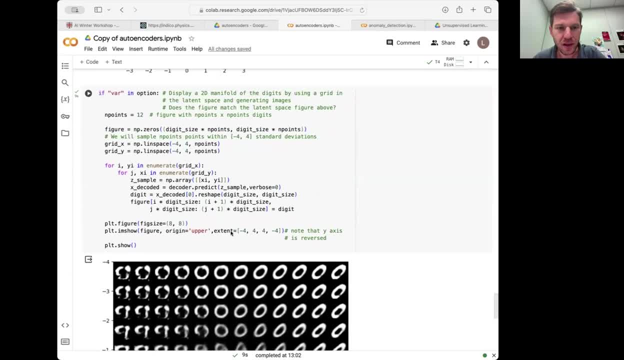 Yeah, Then you start here. there is some confusion. This will start clearing up the tree if you run with more epoxy. It's kind of cool to see this, But the interesting thing is that it generates the images which it never saw. 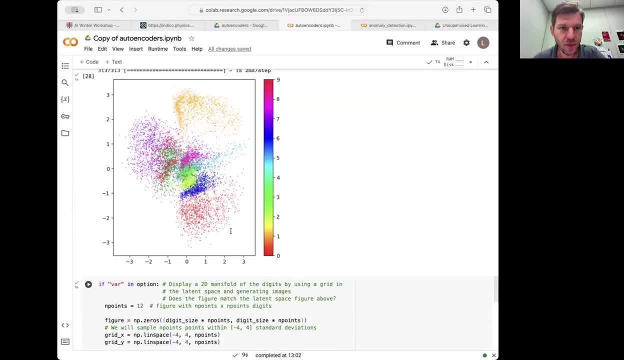 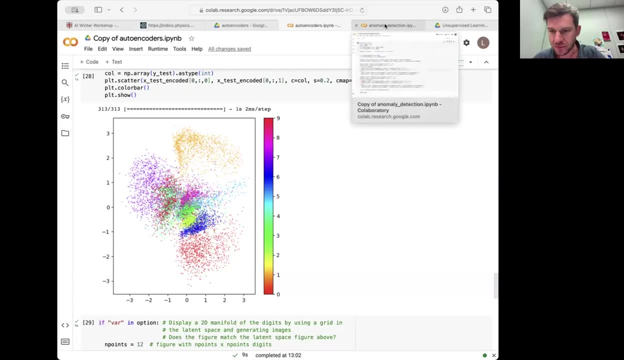 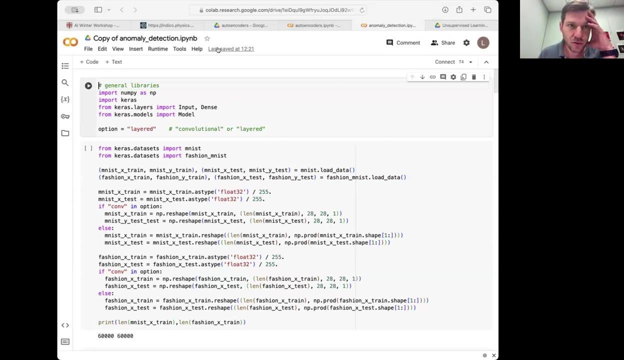 Never seen. yes, yes. So I think now we have 25 minutes left, We could do the other mode. Yes, Yes, that's interesting, That's really a normal detection. Yeah, So let's go. let's open the next one. 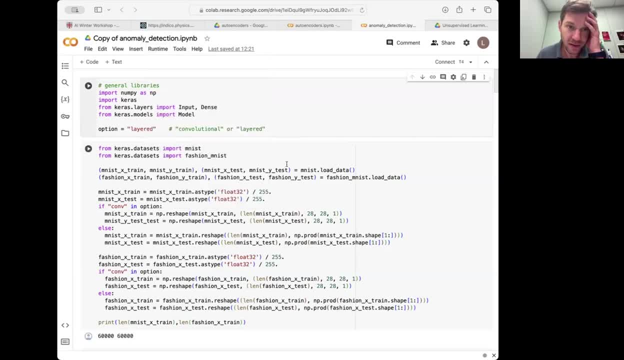 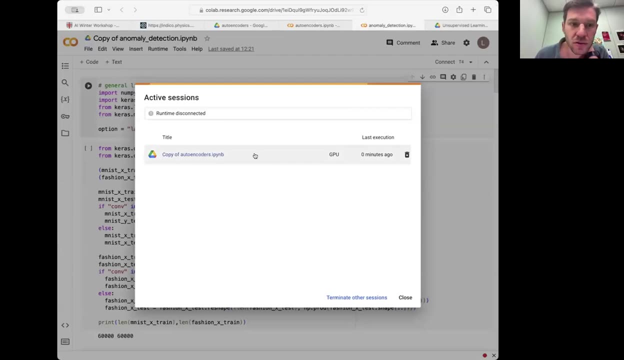 So you have to disconnect and I think you can delete it on time. And no, here, yeah, here. So okay, Yeah, when you try to run it all, you will ask to disconnect run time. You just feel free to terminate other sessions. 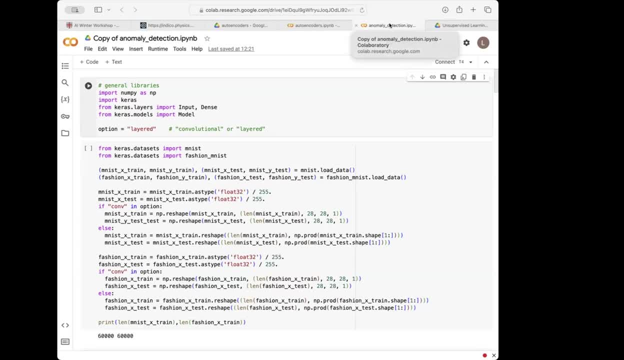 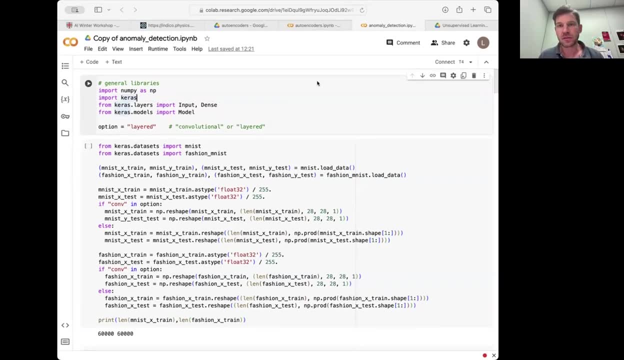 and focus on the- Just leaving the resources on Google for that. they won't allow you to run two daily sessions, So, assuming you know everybody's in the other notebook, Let's start running it here, Okay, so here it's kind of related to a question. 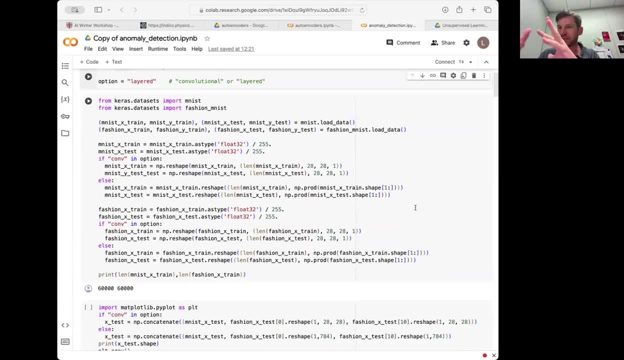 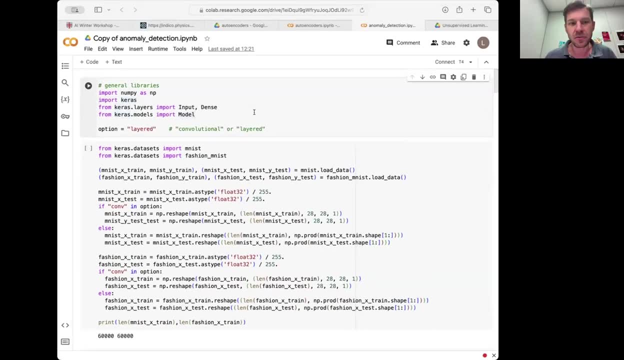 that was, I don't remember the name. but if we train on something and then predict on something else, for instance, or you know how it would be classified Here, we train on a process that we know and try to see, we compare the reconstruction loss. 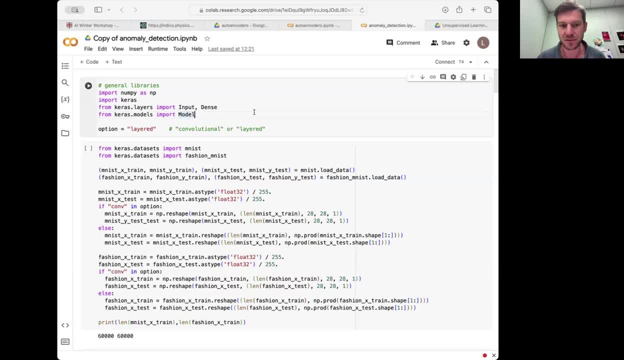 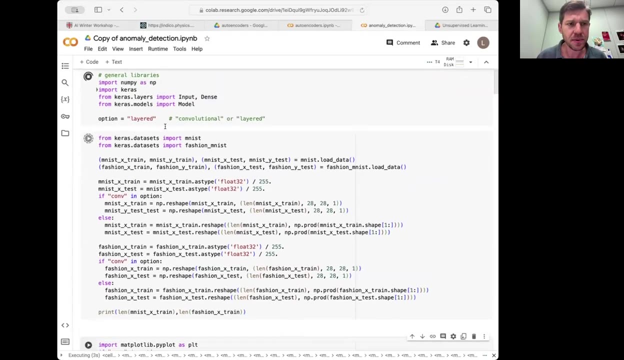 and if there are differences, this is kind of an anomaly, something that we were not expecting, or the network hasn't seen, And yeah, Yeah, it's, yeah, let's keep here. So here again the first cell. 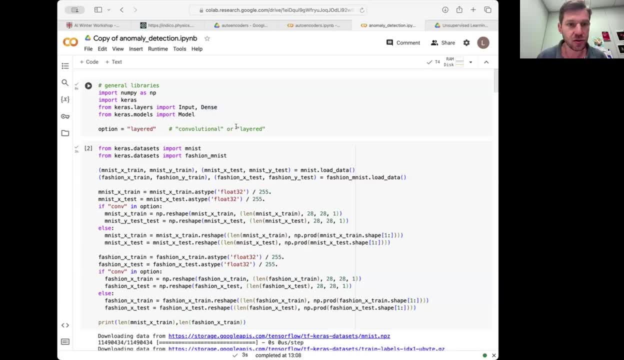 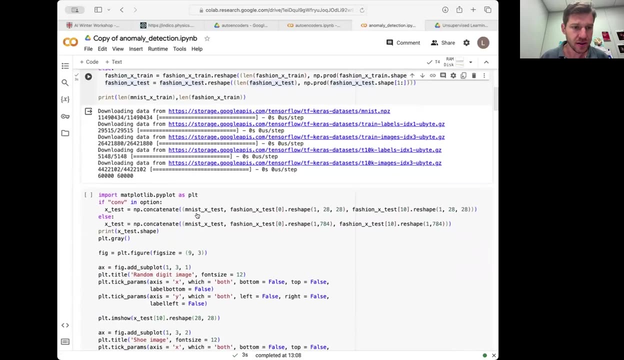 we use the first cell to define the configuration, the values, options. Let's keep the simpler one, which is with dense layers. The second one is to get the data sets, training and the testing that we split them to create the images. 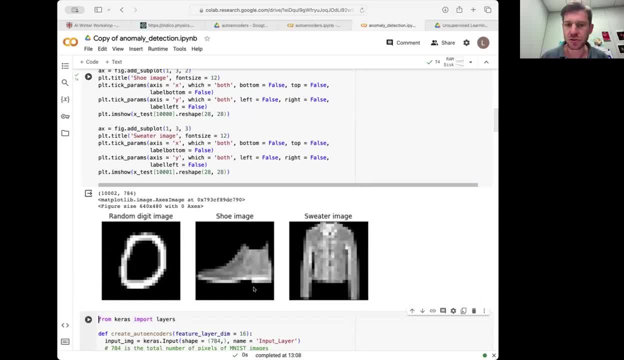 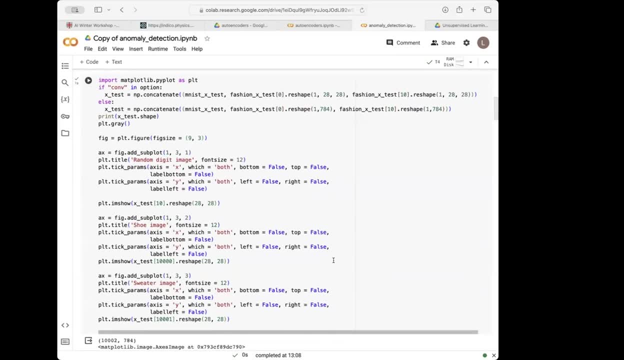 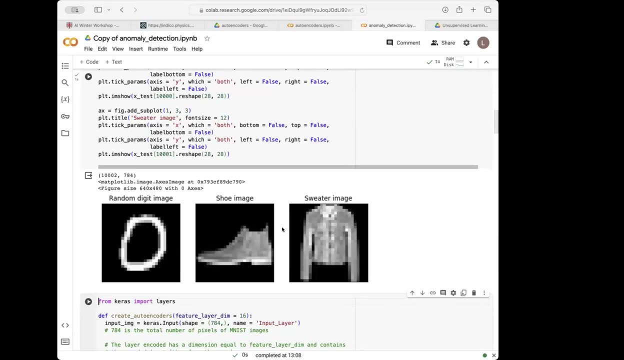 Let's have random image: have a shoe and then we'll have a sweater. So these are anomalies. so we train on these same digits as before, so it learns how to find zeros, ones and nines, And then we confuse it by. 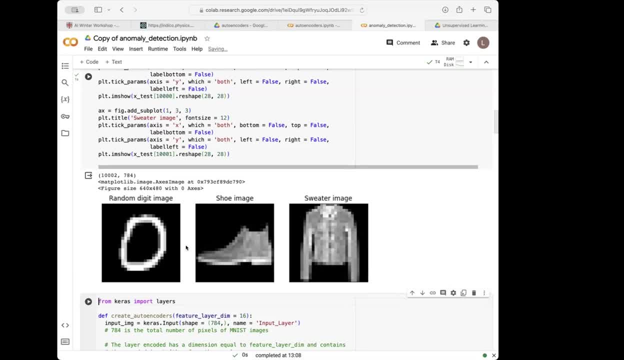 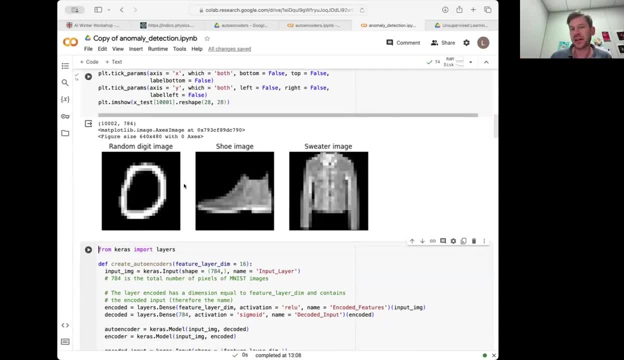 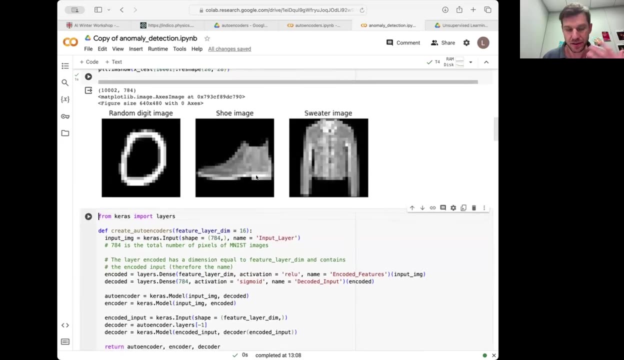 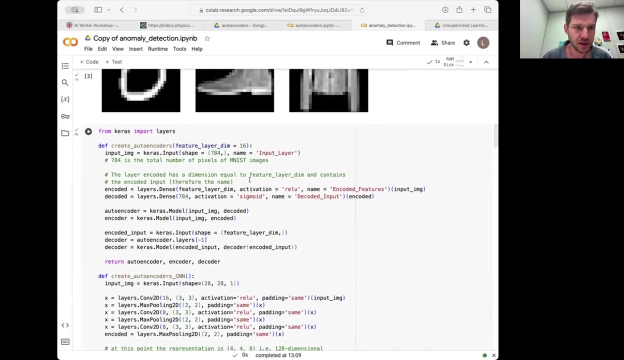 an image of a shoe or an image of the sweater. yes, let's see if it finds it them anomalous or not. yeah, so then on the output, depend where we select, we will. you know we look more or less anomalous events or images. let's say so, do this, run this okay. 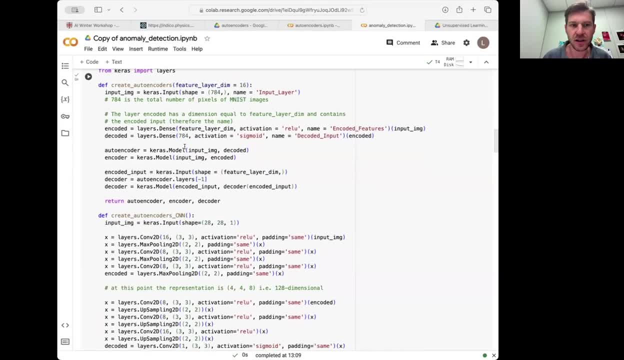 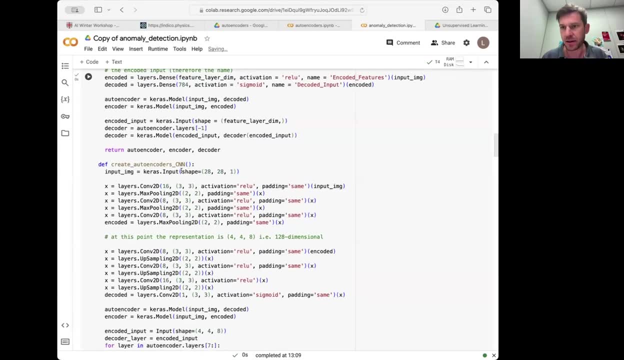 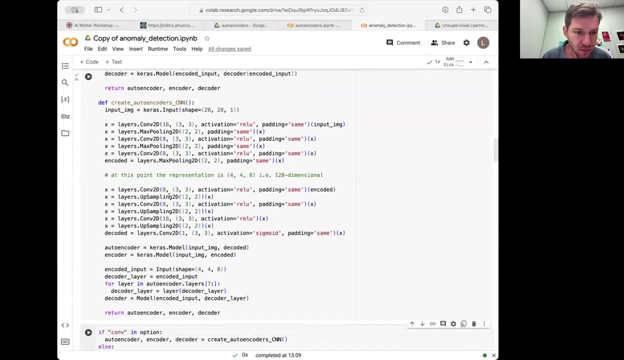 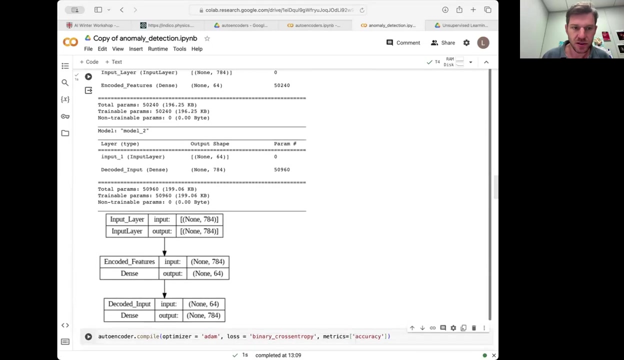 so here, where we create autoencoders, this is very similar to what we're discussing earlier, so we can skip it. maybe when we run again with the cnn, with the convolution networks, just go very briefly here and discuss a couple of things. so this is a similar thing. some, some parameters of our 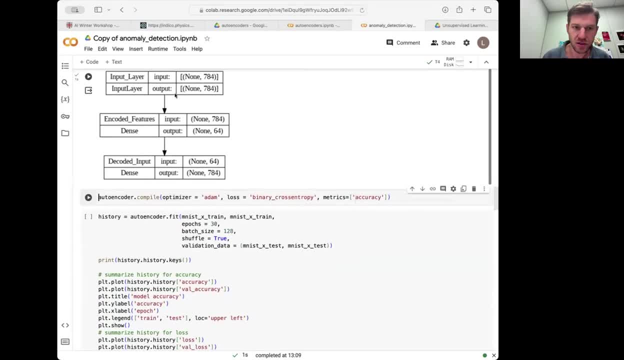 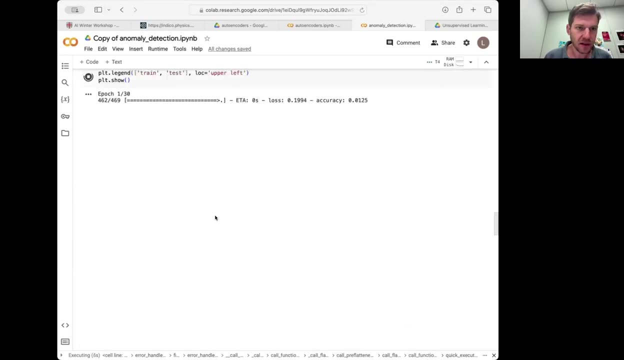 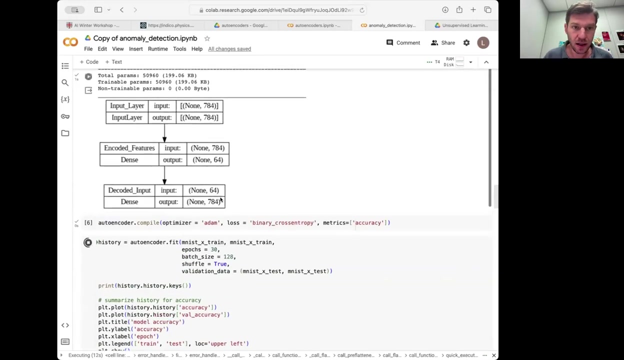 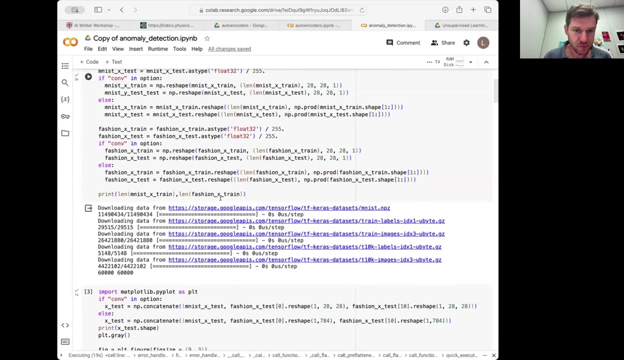 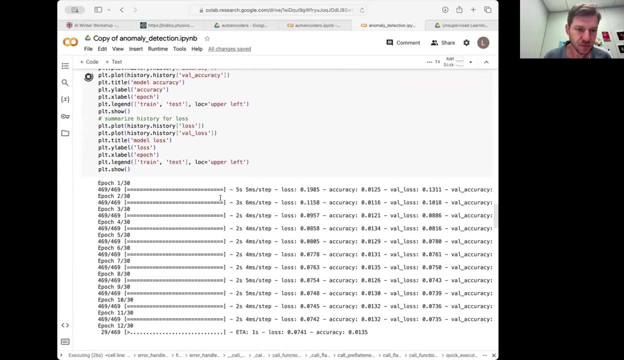 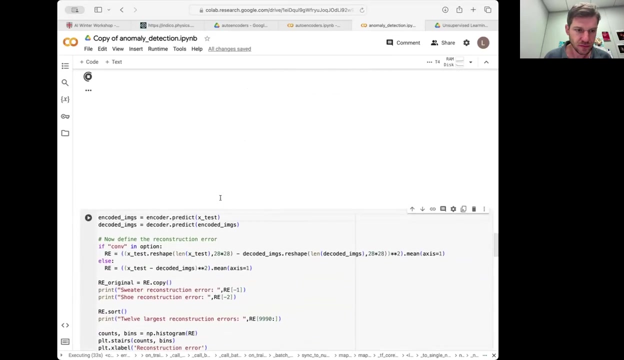 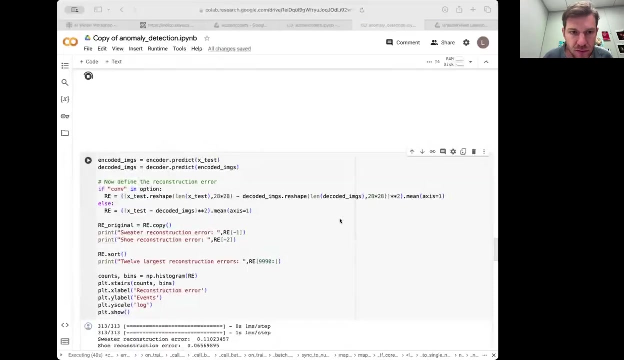 of our algorithms, the simple dense network, the laws, the metrics that we use. and here is the training. here are 30 epochs. remember. we are using the same input data set as in the previous exercise, right, which is numbers from zero to nine, and we use our set. 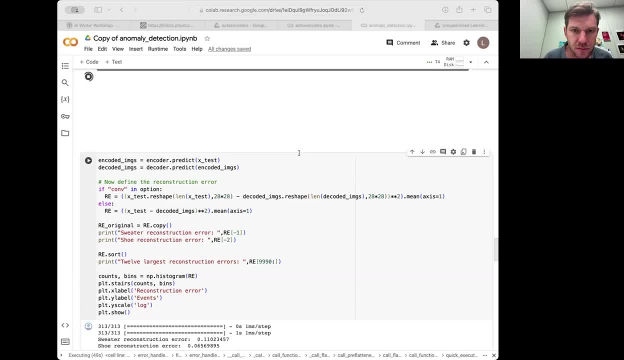 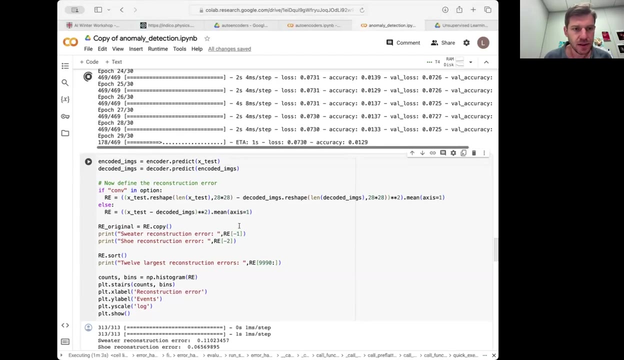 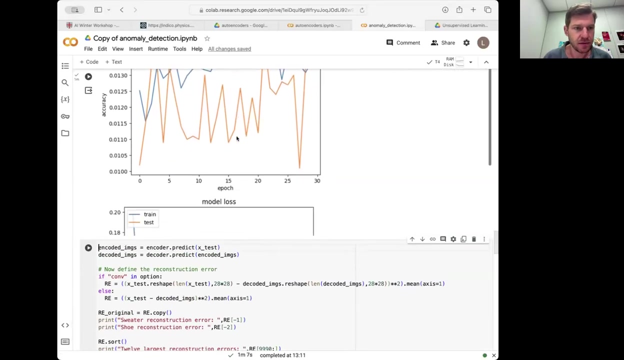 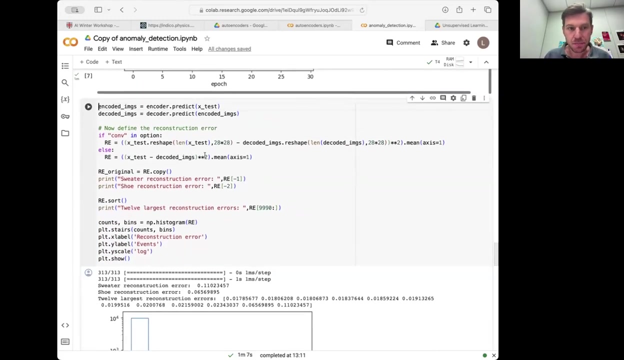 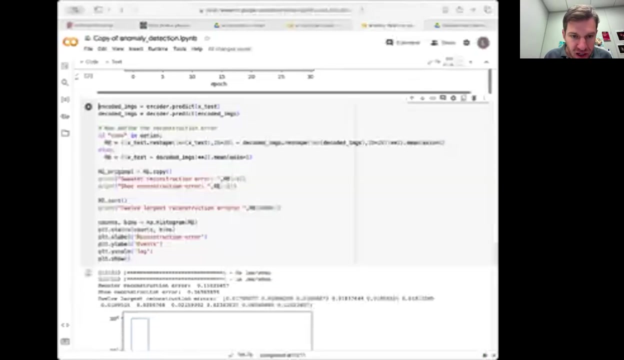 that And while we are waiting, just to tell you here you see the accuracy. fine, that shouldn't be different, really, from the previous one. the difference here is coming on this part here, where what we do is actually in these lines, we calculate the reconstruction error. 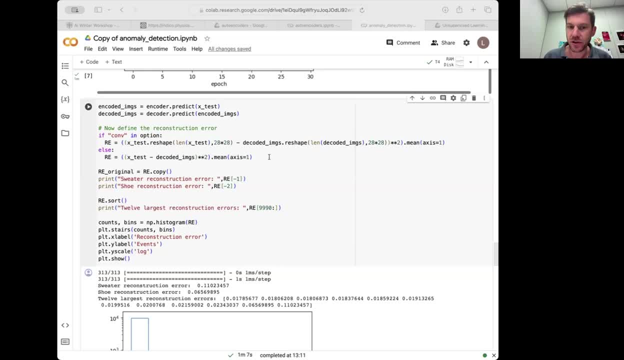 that you see as Re here for its test image, right? so in principle, this is a square difference between the original and reconstructed images that you see. well, you didn't put square. I know you put squares right. yes, for the convolution. 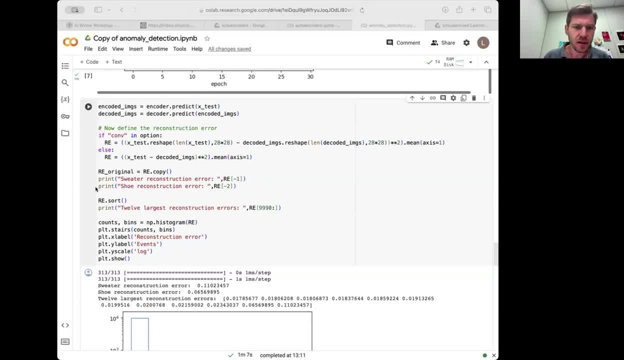 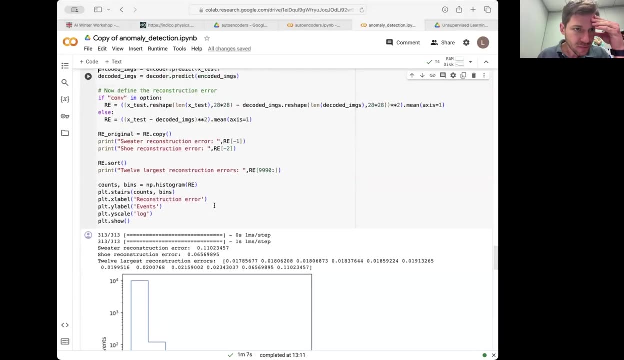 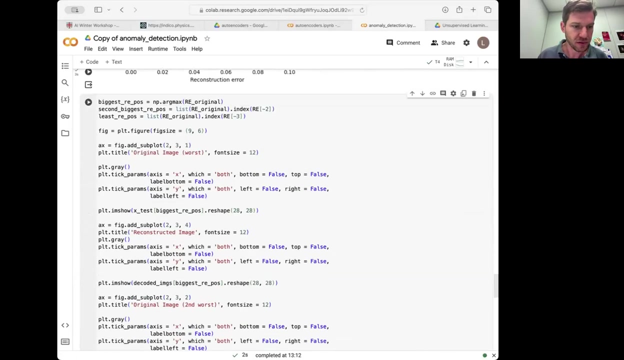 And yeah. so the largest errors we have means that we have anomalous images, which, in our case, would be a shoe or a coat or a jacket. So I didn't run this, no, it's from before, okay, so yeah, so this is anomalous. 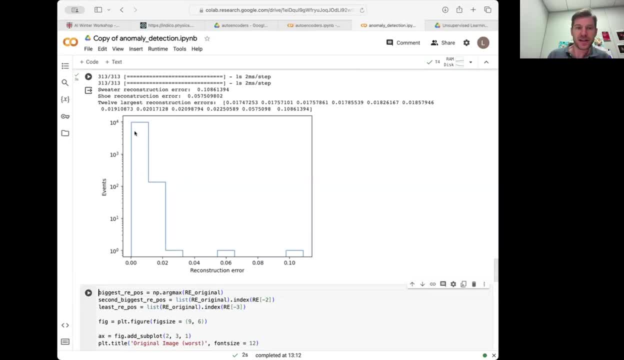 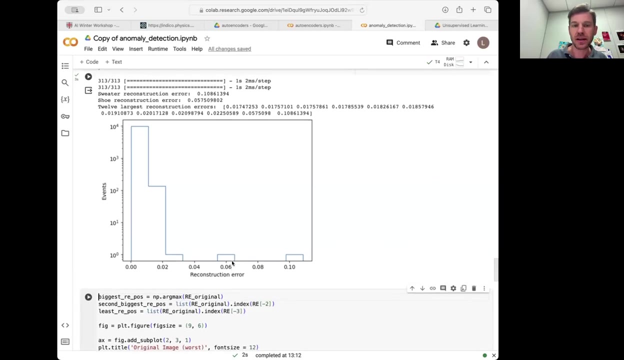 So what we do in practice. so these are cases that the reconstruction error is very small. so it means that probably these are images that the algorithm was trained on. The higher we go to the reconstruction error. this would be like images that look more like: 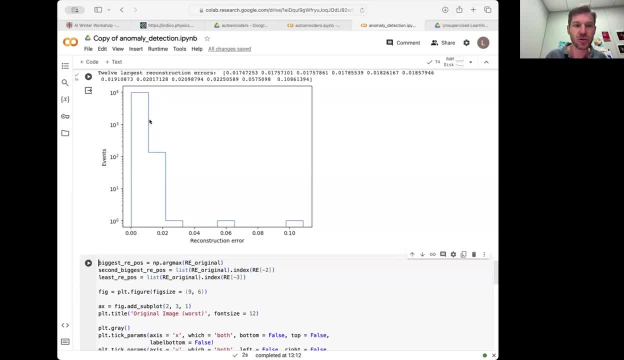 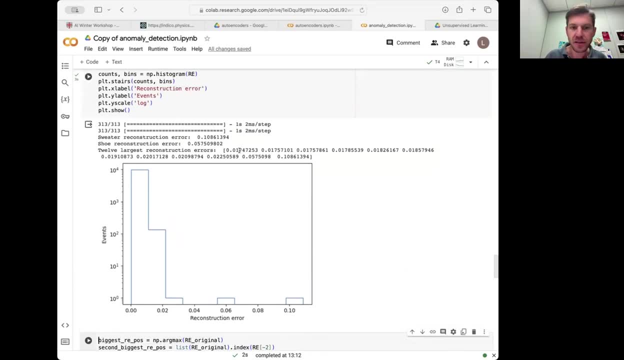 anomalies not seen. the algorithm hasn't seen. Of course, you know we have to train more images and you will see a distribution here. okay, And here are the larger reconstruction errors that you can see visually in this plot here. 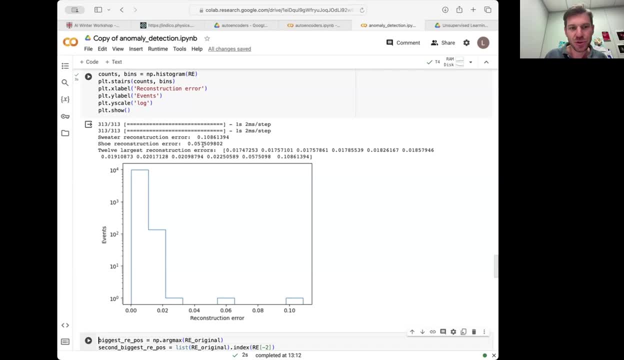 And actually you can see which kind of makes sense. probably the shoe has actually smaller average reconstruction error than the sweater. then in this case you can cheat, you know which are the images and we can see actually. so it's more, it's easier for the algorithm. 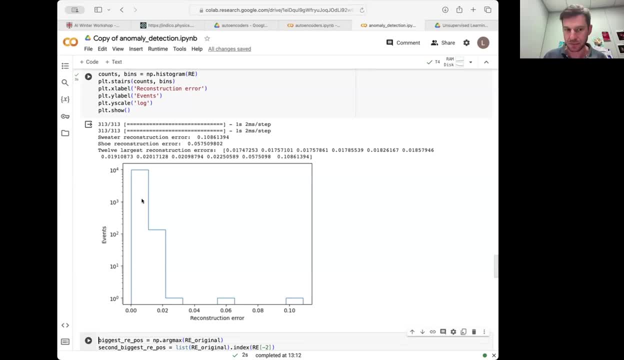 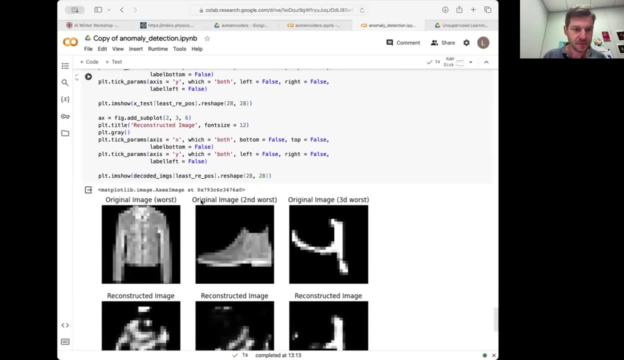 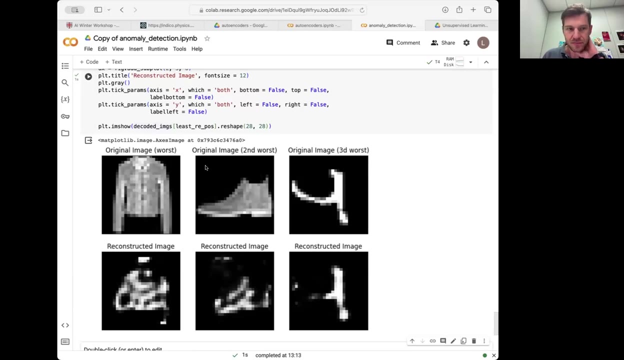 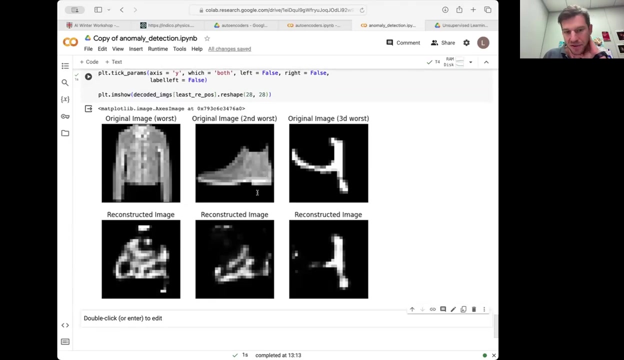 to discriminate between sweater and numbers than shoe and numbers, And let's run this also cell. so this is actually what will be the original image, the worst one and the reconstructed one. Of course, we train with 30 apples. it's a simple network with just 10 K events, but 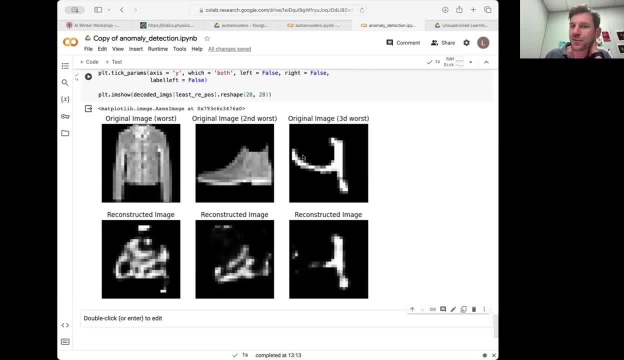 you see, actually, that it works pretty well To figure out. also, the, the distribution error. Okay, Yeah, the the most, the, the worst images. so the number, in the case the third verse, is a number, a shoe, yeah, okay, it looks like a shoe with some imagination and sweater. 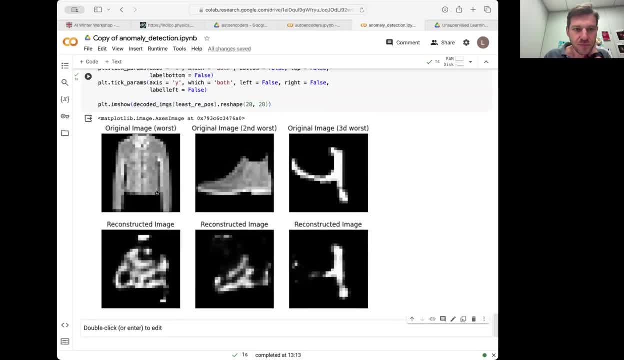 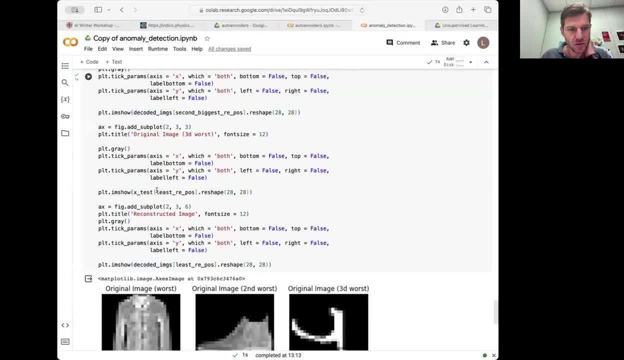 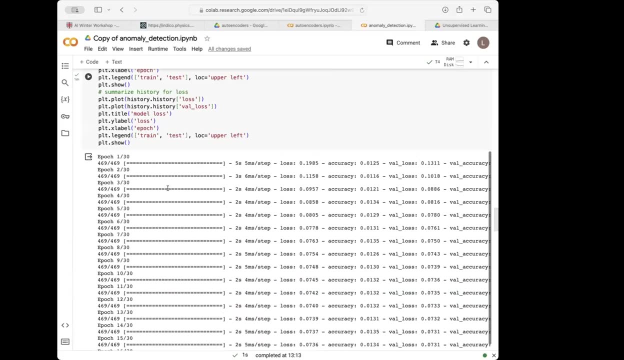 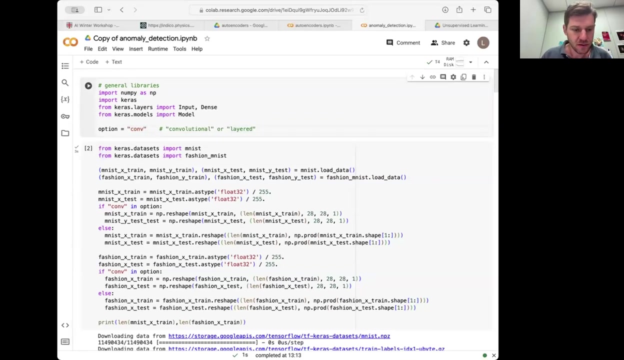 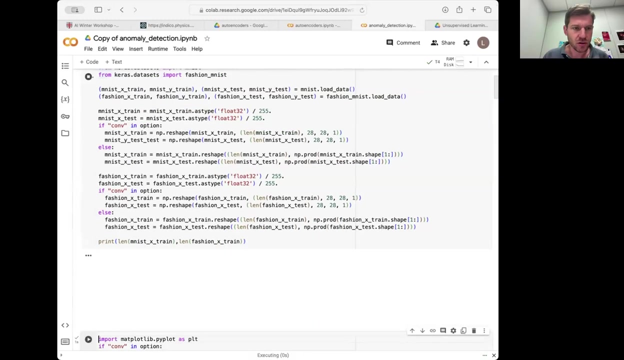 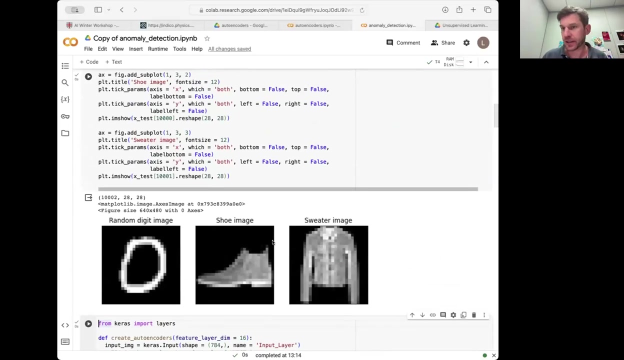 um, yes, so maybe we can run also the cnn and then, yeah, we could run a cnn. yeah, i think convo should work. but okay, yeah, yeah, uh, so let's run the cells. i would just want to make a couple of comments. uh, so these are the same things. you will see the same things. 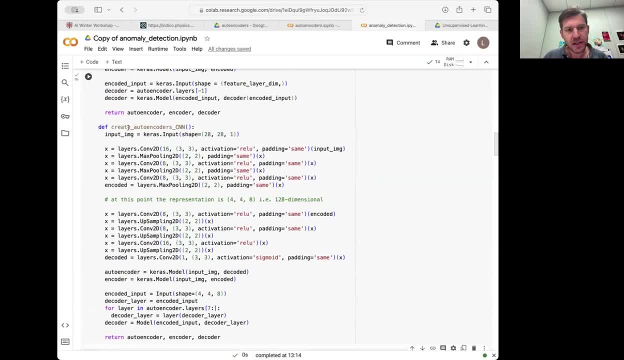 here, here. so here i just want to make a couple of comments. here is where we define the convolutional neural networks. we have the image, we define a path, we we define the number of filters we have. then one thing that we do is actually, for instance, this is more like: 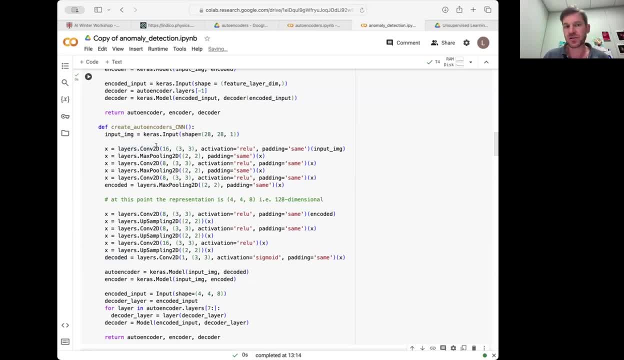 based on experience. you see that here after the first convolution layer we don't put the second, we put a max pool. so what we do is we define a window, in this case the two by two. you have the image after the convolution, with downgrades, downscales the image size. then we put a max pool in two by 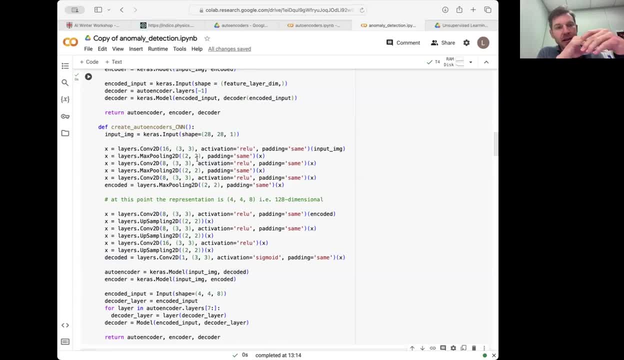 two, the reason we do. there are a couple of reasons. first of all, usually when we have images to avoid, to avoid picking on on irrelevant features, we do some pre-processing: we rotate them, we translate them, etc. doing max pooling first of all makes the training not so sensitive on this. 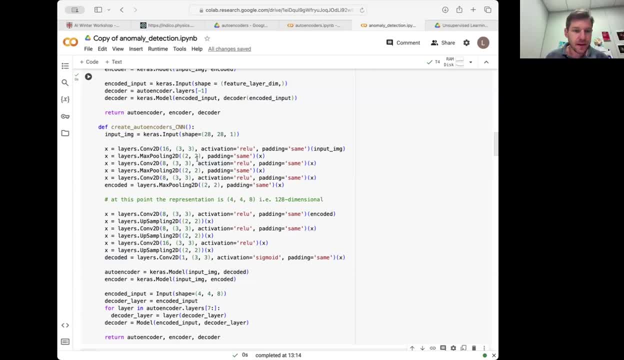 on small differences in the between the input images. the second thing is that you can do what we do with pooling is: we have imagine the image has some numbers, so when in in a two by two window in this case, we can pick, for instance, the sum, we can pick the. 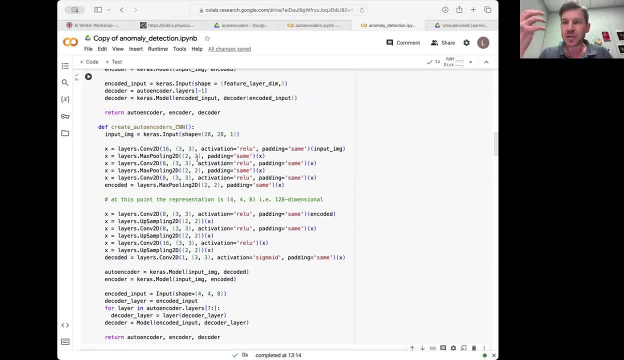 maximum. we can pick the minimum of all these numbers. these allow us to reduce dimensionality but also focus on more important features of this- two by two, in this case, window- and makes also the the network more robust- avoid over training, for instance. so this is why it's a good advice to use max pooling. 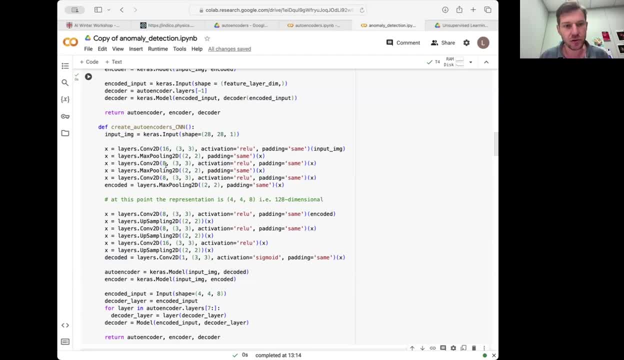 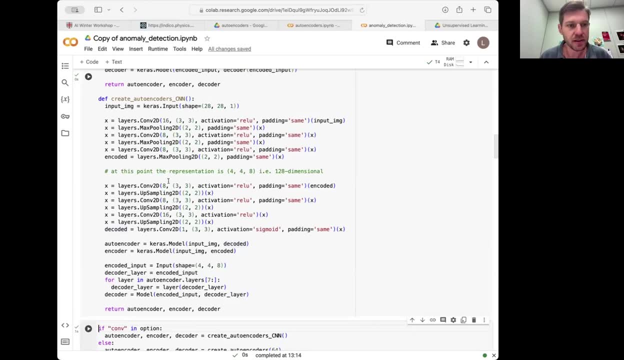 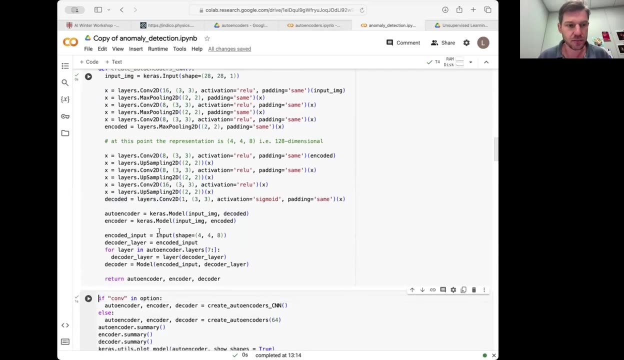 before running the second convolutional layer. so just something based on experience. similarly, you know, this is when we are encoding the image and here we are decoding the image. the same concept that we were doing up to now, except that now you up sample rather than you really have something. now you have to make. yes, 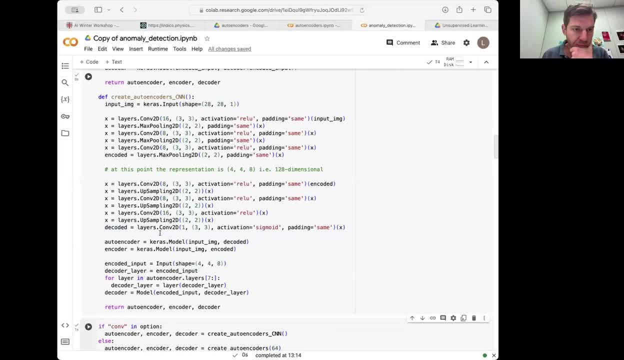 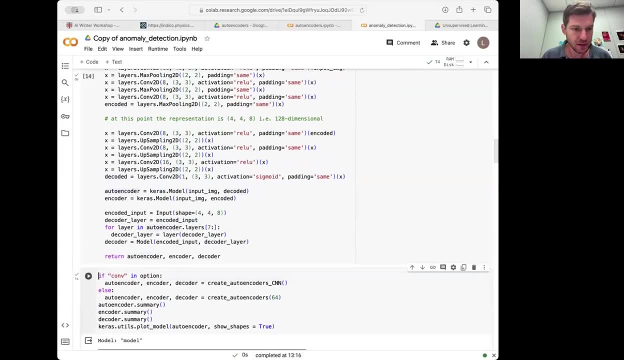 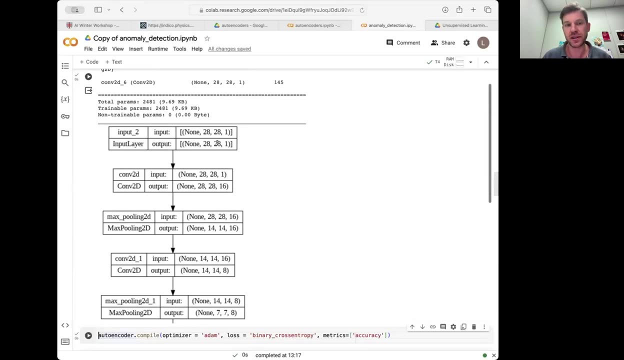 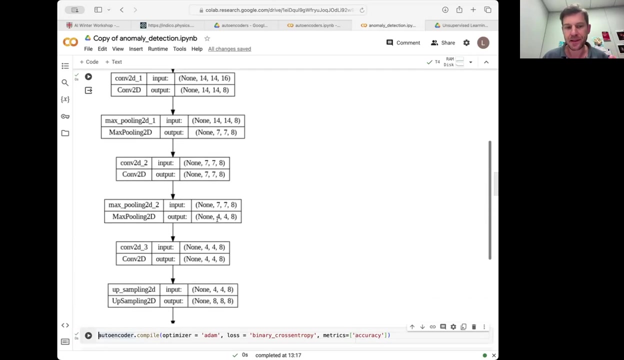 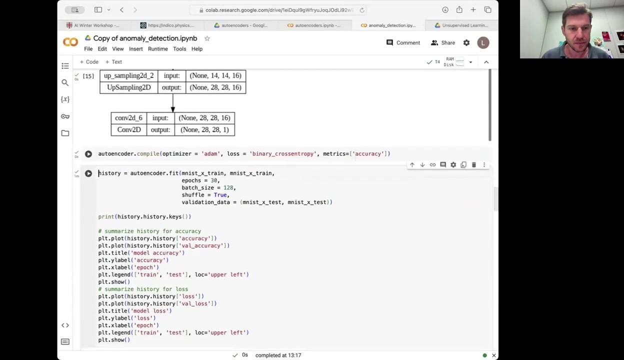 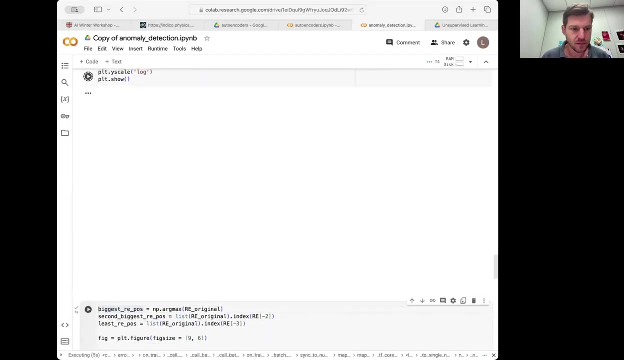 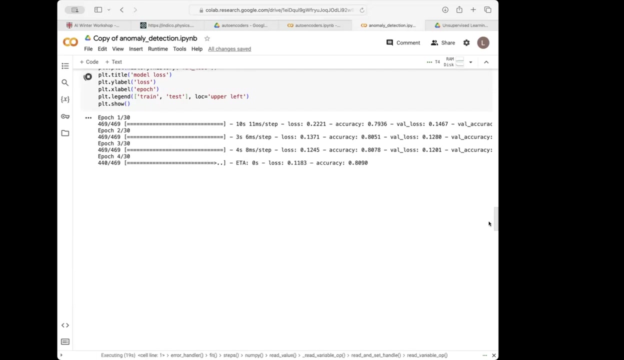 exactly the image, go back to the original dimensions effectively, and you can actually see all these things. later we have a 22, 28 by 28 image here. then we go for times 14, blah, blah, blah, and then we start up something again. So now you see that accuracy is really pretty high. 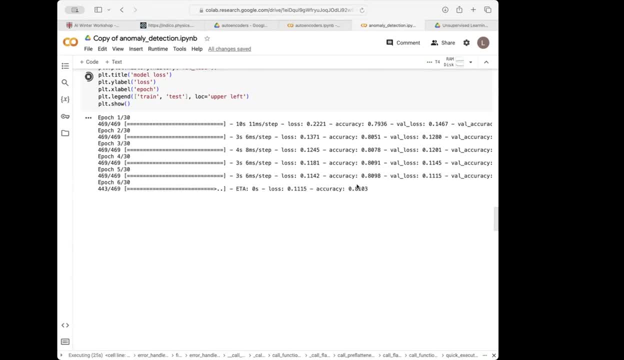 It's pretty close to one. So this is the case where accuracy is really very good, because convolutional networks are very good for processing images. They basically operate like images because they have pixels. Their neurons are pixels of the image. So you see that accuracy is much better. 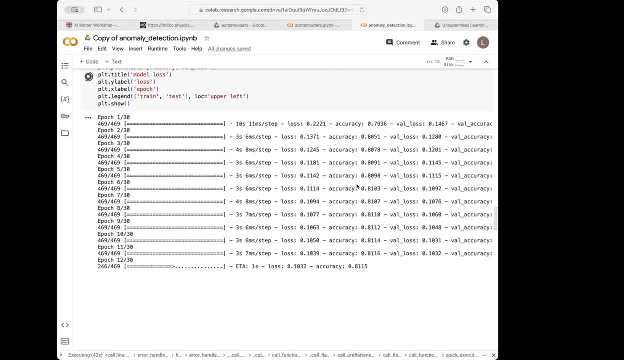 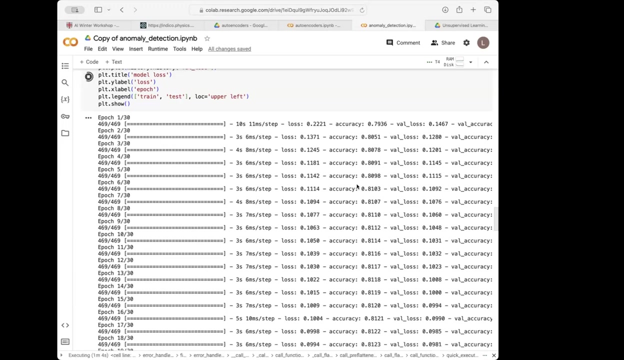 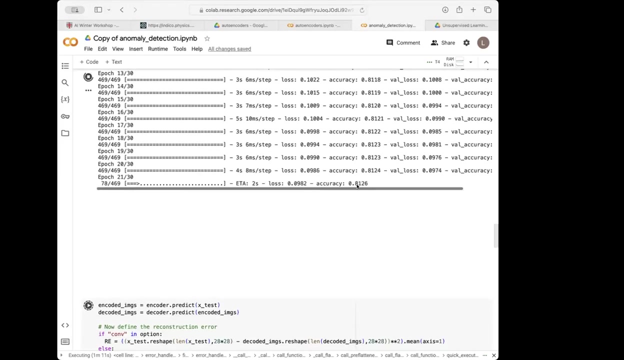 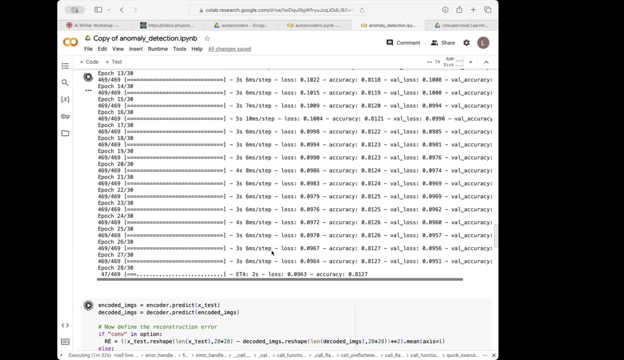 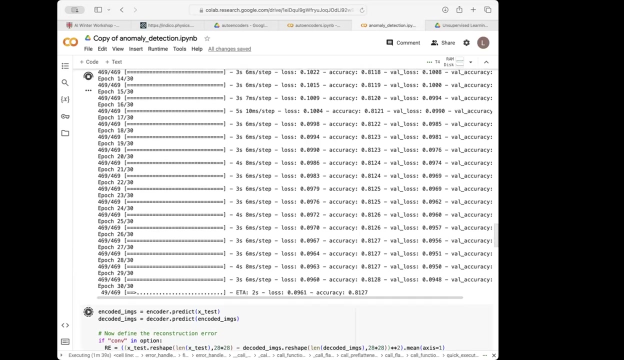 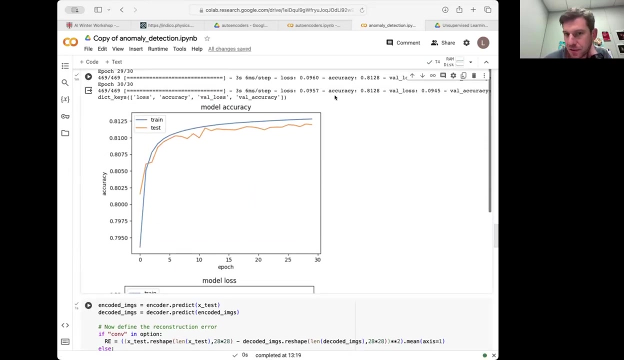 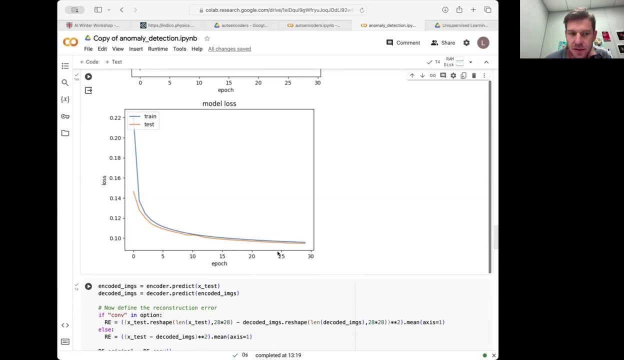 and you see the plot which shows that it's pretty healthy. Thank you, Yeah, and you see now- actually you were seeing here, but you see also visually here how much improved and the lows not similar value. So, and this is the reconstruction error here, 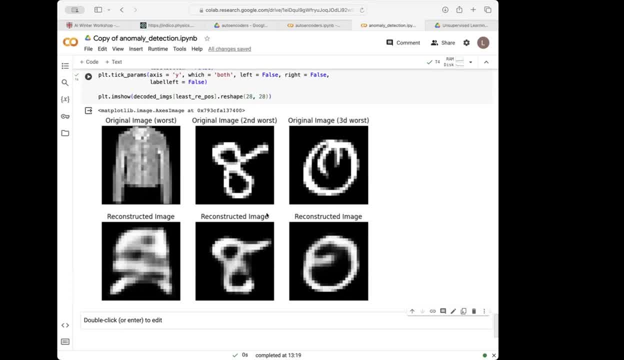 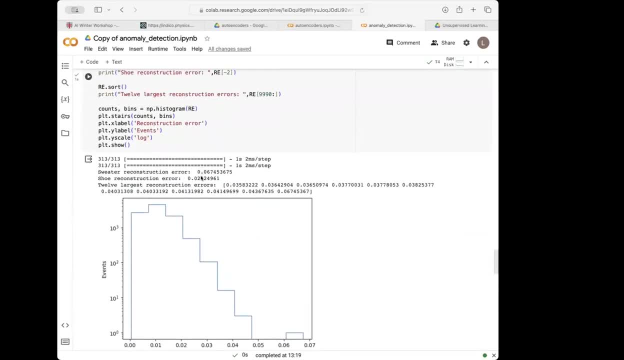 So you see now, shoe is not really an anomaly, It's even somewhere in the middle of the distribution. Yeah, because you see, the mean value here for the shoe is much closer. I think it was 0.05 before and the sweater was 0.010. 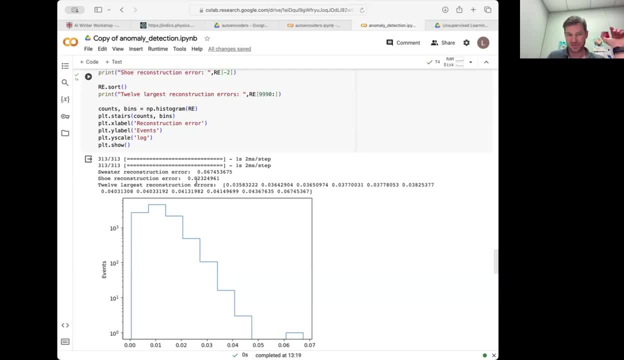 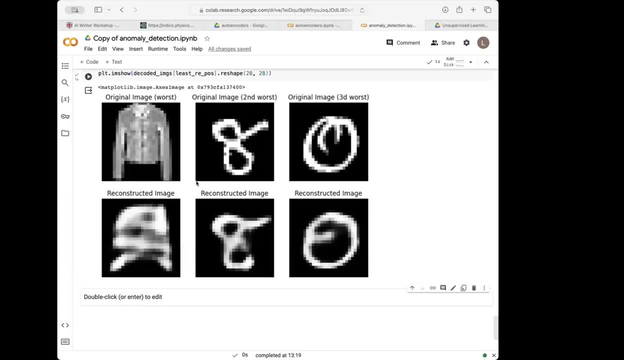 Now it's a factor of two or more, closer too, Yeah, so shoe is not found as an anomaly anymore. That tells you that you have to be careful. I mean, it's clearly an anomaly, but not this thing, This training. 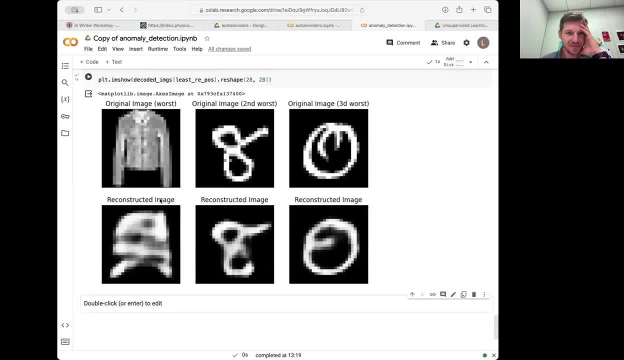 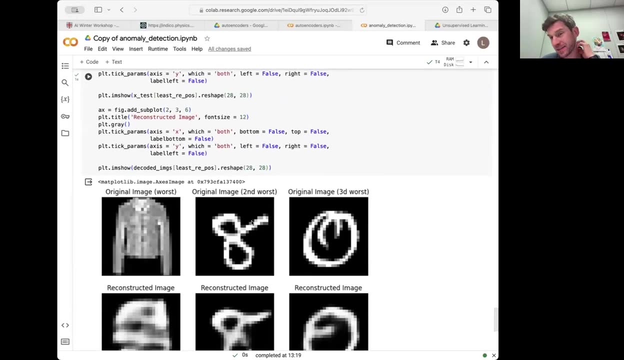 Yes, Couple of digits are rather poor, but they're still nicely reconstructed And the sweater is not reconstructed at all. Yeah, Now, there could be many reasons. I mean, I don't know, in this dataset we're using, there is some pre-processing. 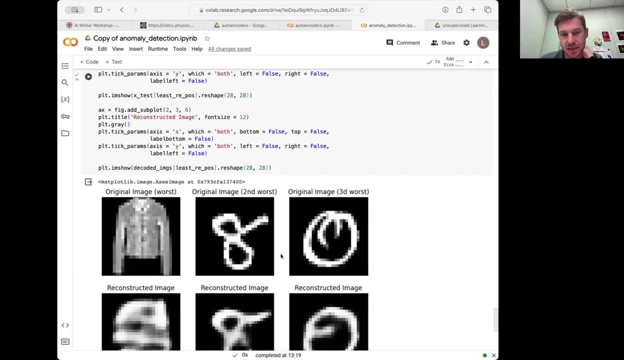 Also, you need many more images, and probably yeah, But this is something. also you have the code. you can consider it As a challenge actually to try to improve this. Yeah, try to maybe find cats among dogs, because there are many of these MNIST datasets. 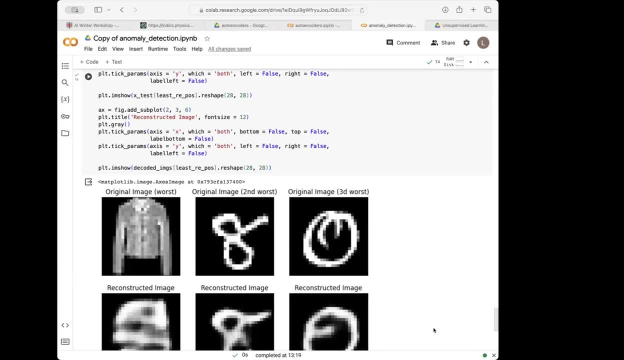 So you could get sets of specific animals or specific flowers. Not all of them are 28 by 28 pixels, So you might need to change the dimensionality of your whole thing, But if you work with MNIST datasets, we use just two: fashion for the shoe and sweater. 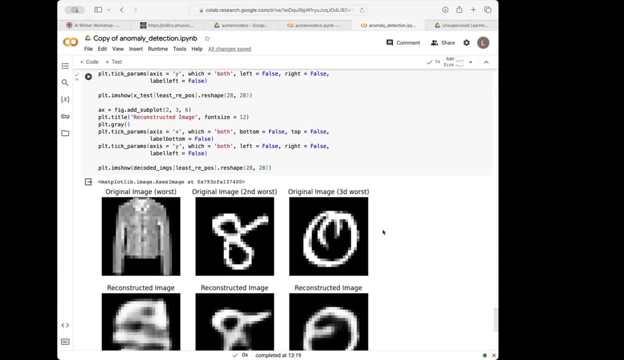 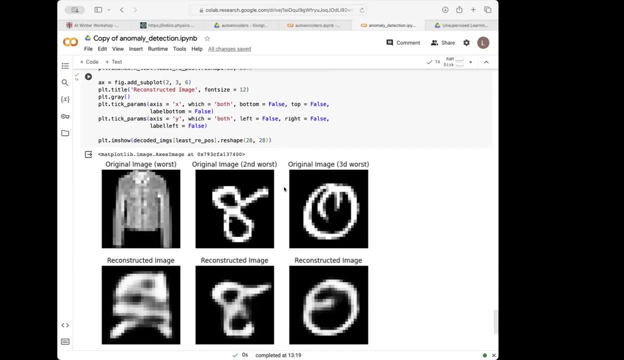 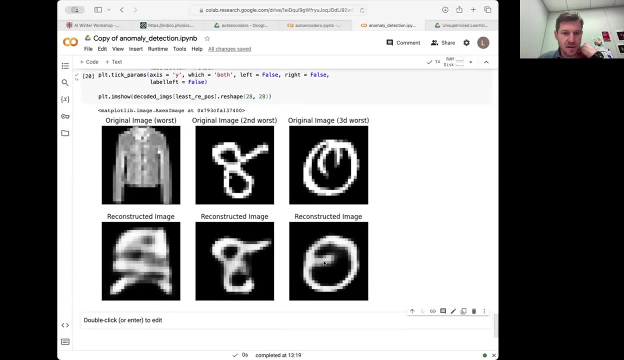 And digits. for the other one. You could try to train on fashion images and then see if you could recognize distinguish shoes from shorts, things like that. So an infinite amount of things you could do and play around. Yeah, Do you have any other questions? 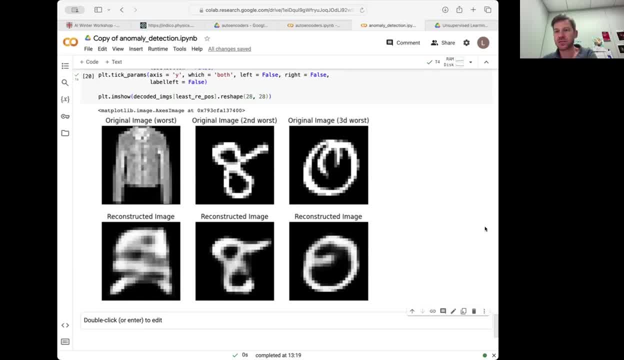 No, Okay, Thank you. Yeah, Do you have any questions? So I haven't checked the chat for a while. Yeah, I'm looking at the chat. Okay, thanks, It's difficult because you have a phone. Yeah, it's too hard to do both. 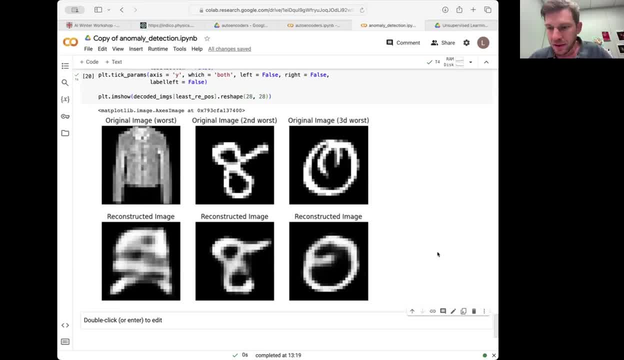 Yeah, And it's on my laptop, Yeah. So there's a question. If the reconstruction error of the anomaly shoes and shorts is even lower than normal, how is this model useful? Well, that's the big problem with this anomaly detection. 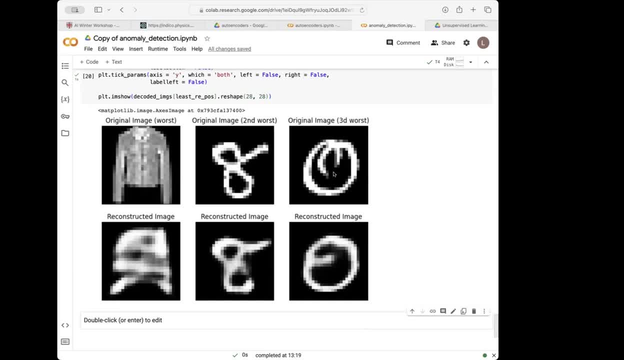 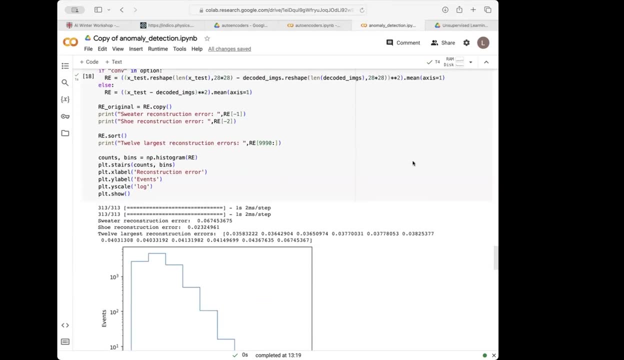 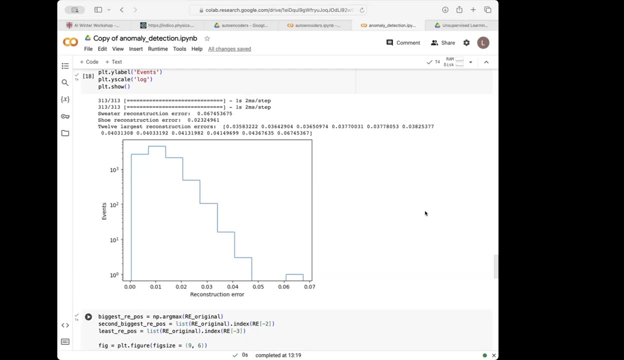 because you don't really have probabilistic way of saying you know how often you would detect something as an anomaly. This is because of this Pearson theorem, So you could only compare two things in a proper way with probabilistic interpretation. All that anomaly detection does- it tells you that certain images 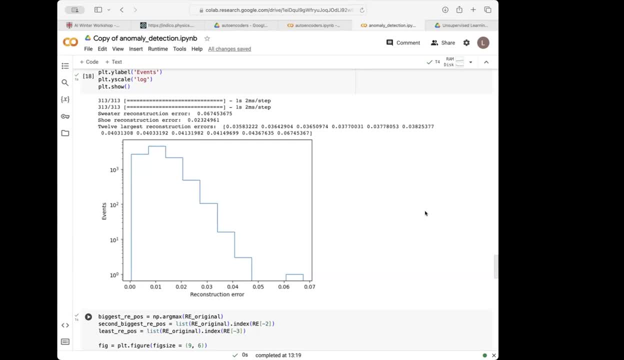 do not look like they come from the training sample And it's very hard to say why. So you saw that the simple network seems to identify the shoes and the sweater as correct to outliers, but more complicated network, for instance, didn't think that shoe is an outlier. 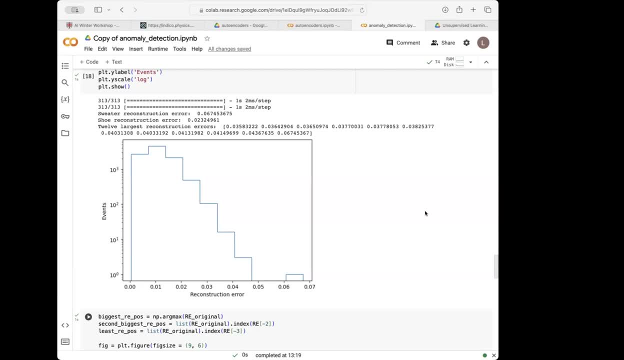 And we don't know why? right, Because we don't really know the intrinsic of this latent space. If you use variation out of the encoder for this problem, which you could do, you could just replace convolutional with variational from the previous exercise. 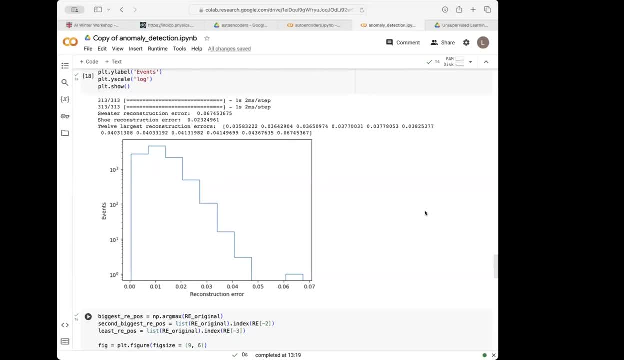 then you could open the latent space and see what's going on. So you would see where it would put the shoe, where it would put the sweater with respect to the digits, And there you could try to figure out how to change the network to. 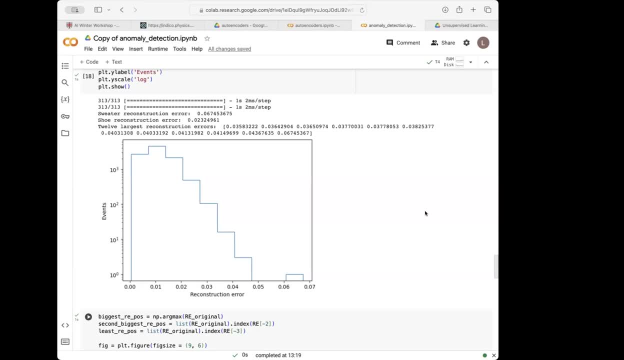 make it more prone against errors like calling shoe a number. But there's a long way to go. There's a lot of things you could do just by playing. These are simple examples which we just used so that they run in finite time to show you a few various options. 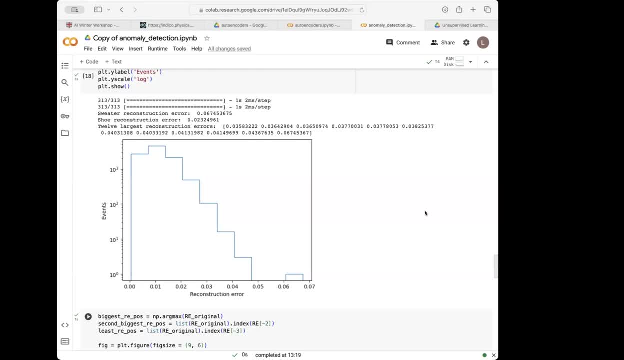 and just bring this idea of outlier encoders, which is a very powerful tool, and anomaly detection. Yeah, I mean you could use more filters, because now, you don't know, maybe it just looks for circles or some smooth angles. I mean we don't have so many filters there. 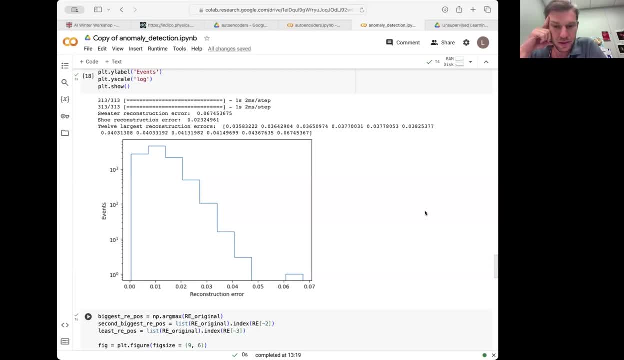 so it could be, and confuses. There's a shoe with some digits, So there is a lot of seven or something, or four has a little bit similarity in shape. Yeah, Because it depends how you do it. The filter is just numbers that you multiply. 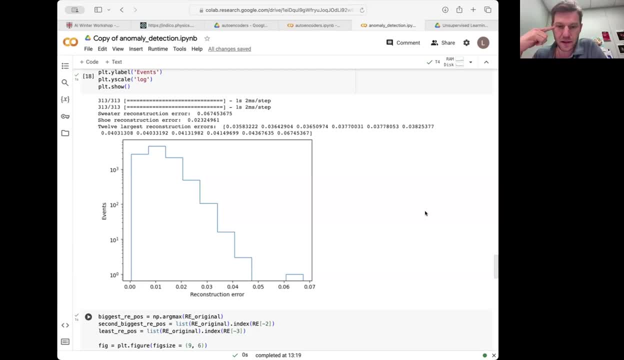 You make this gray scale. It's a scale from zero. Each pixel has a value from zero to one, And then you slide the pixel, the parts- I mean the convolutional kernel- across the image which has some numbers. Could be zero, one, zero, zero, for instance. 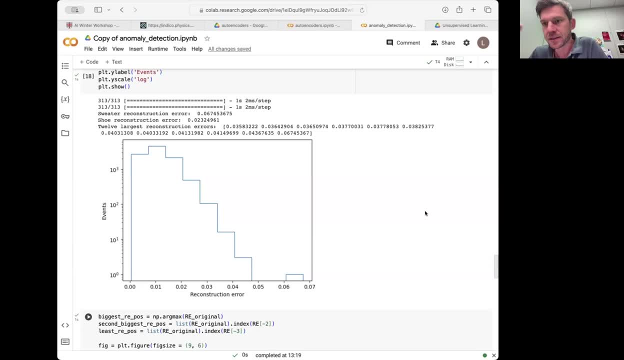 to pick some edges And you multiply this and then it has a new image after convolution. But each filter is designed to identify different features And you have to. just one thing is to put more filters. That can be a nice exercise to play with. 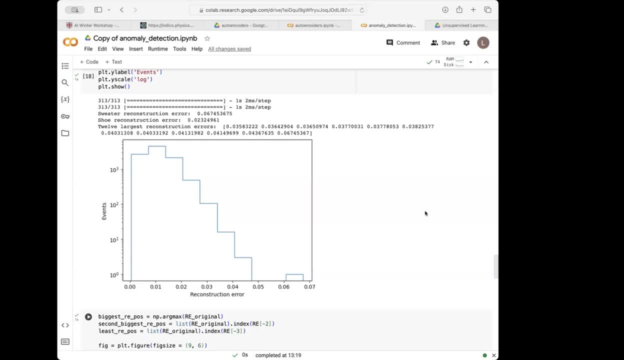 Yeah, So a lot of this is really trial and error Because unfortunately we don't really have a good theory of machine learning training. This is an interesting statistical mechanics problem which some people are trying to solve, But so far there's a lot of black magic there. 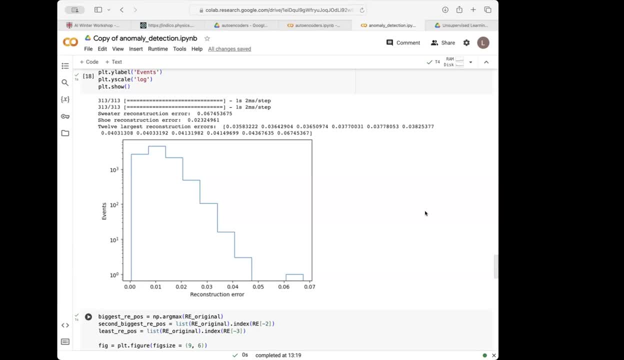 So you try this, and it's well known that certain configuration are more stable for certain problems. So that's how people figure out. you know this max pooling thing, you know what kind of loss functions you use or what kind of problems. 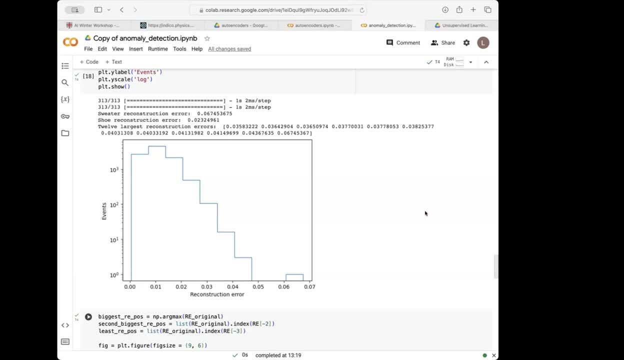 A lot of this is just know how, Which you learn by just doing and running different examples. So I think Rick wants us to wrap things up, which is about time to do right. We have five minutes. Thank you Really appreciate everything you've done. 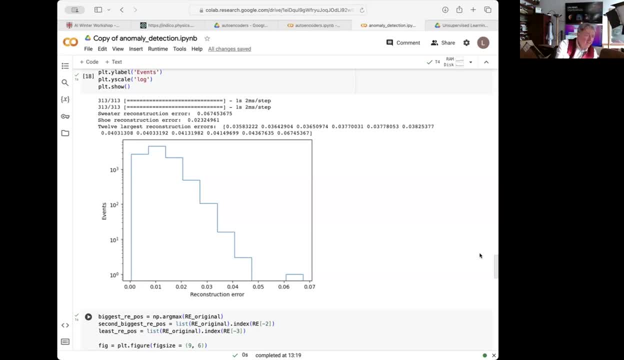 So please do let us know on Slack If you have any issues with access or anything that we need to refocus on, because I think we tend to lose the questions from the Zoom. Actually, I do see there was a. there's an open question on the Q&A system. 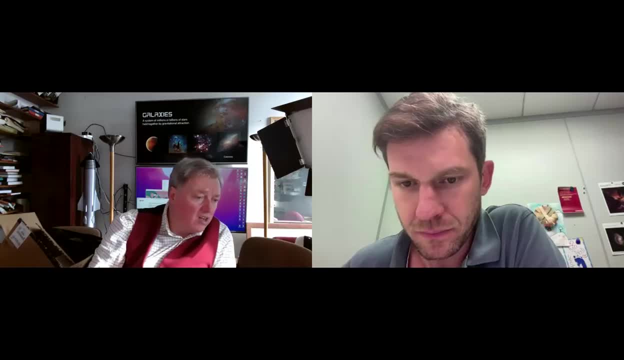 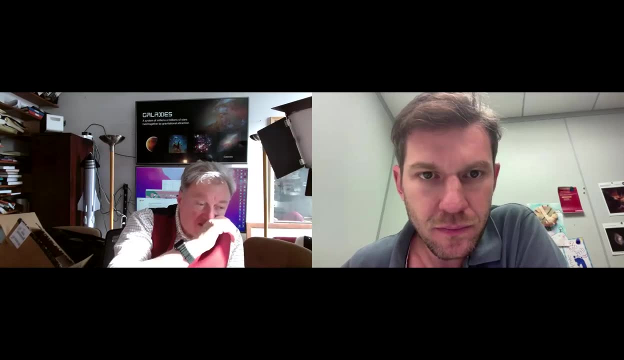 saying, if I understand correctly, encoding and decoding dot dot dot. That may be one that you want to address quickly, But just before you do that, I just wanted to say to people: yes, do use the Slack link If you. if you're having any support issues, we can try to address them there. 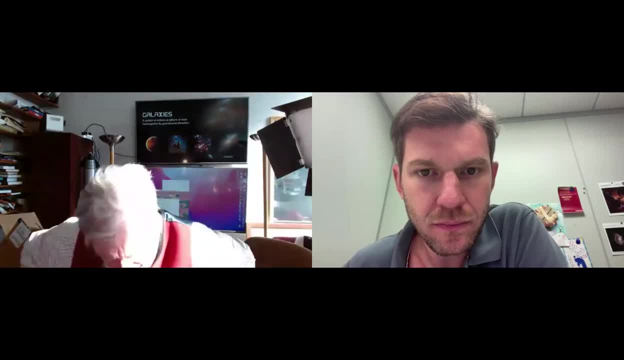 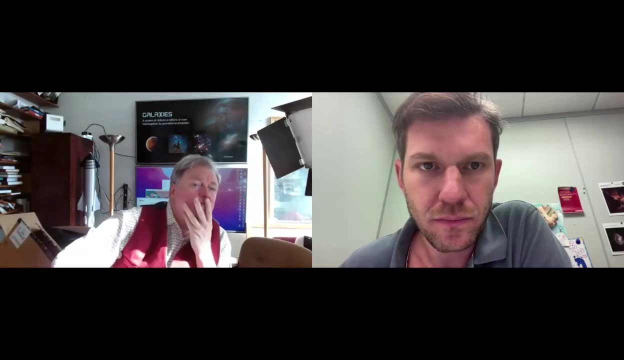 So I try answering this question very quickly. So the question was that encoding and decoding could be any function, an inverse function respectively. Do you think it's possible to encode and learn from a data set by going to a different space, For instance full space? 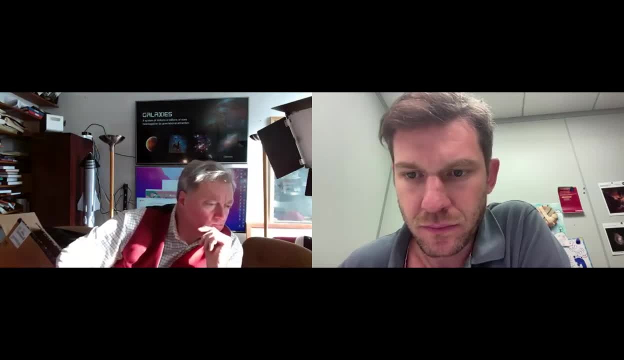 I'm especially interested in using our encoders. in astronomy We're working in frequency. space has a better chance of separating signal in the best way. So if you're having any support issues, we can try to address them there. So I think if you're having any support issues, we can try to address them there. 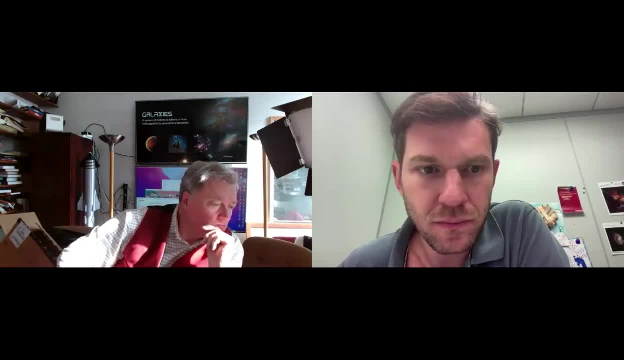 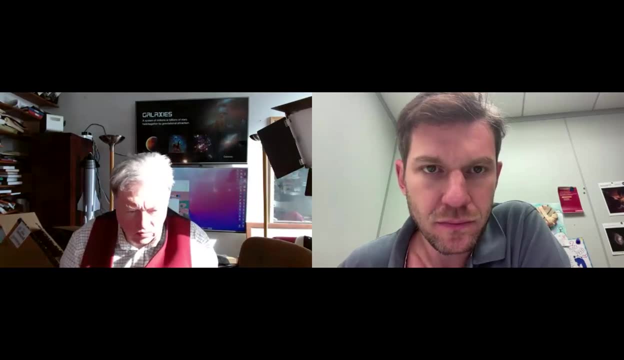 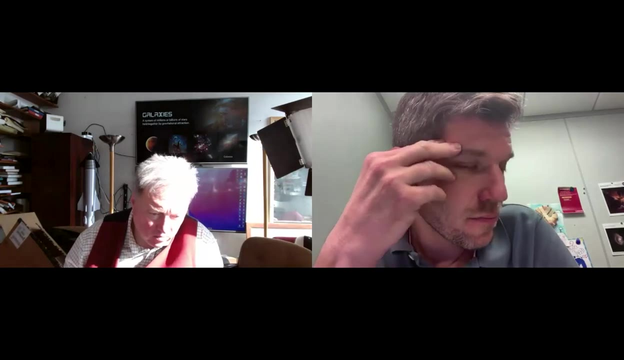 background. Yeah, I suppose this is possible. In fact, you don't even have to have decoder and encoder with very similar architecture. As long as you match dimensions. you could imagine that encoder and decoder could have different dense layers, number of layers, because the training 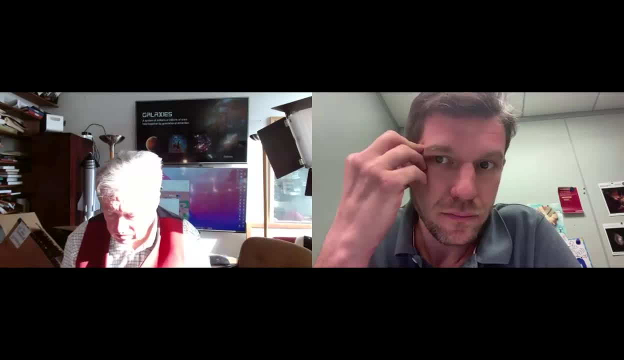 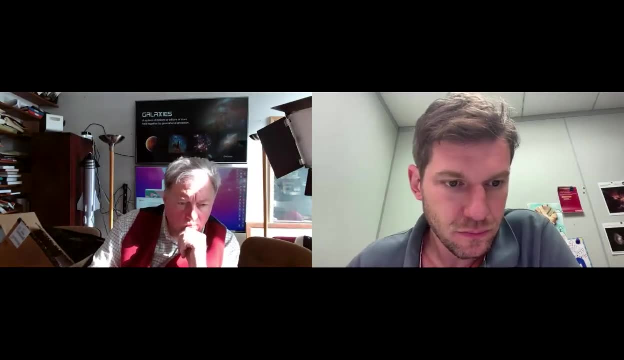 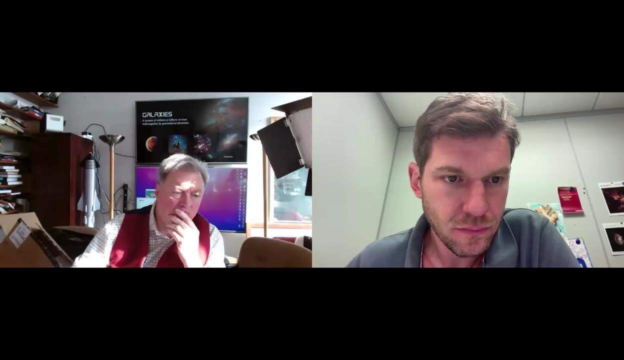 would make things work as correctly as possible. You would find that certain decoding functions and encoding functions are just much more powerful for your problem. But indeed, working with 4ES space is perfectly fine, But for that you don't really need machine learning, You just 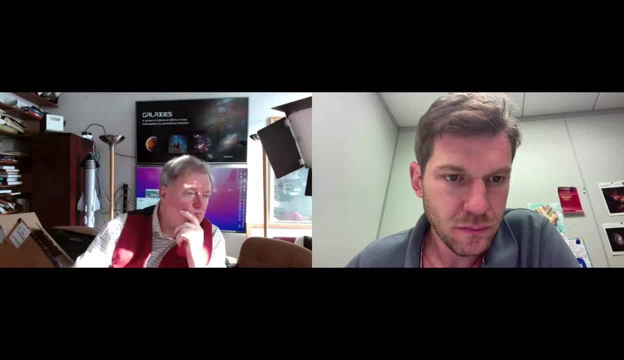 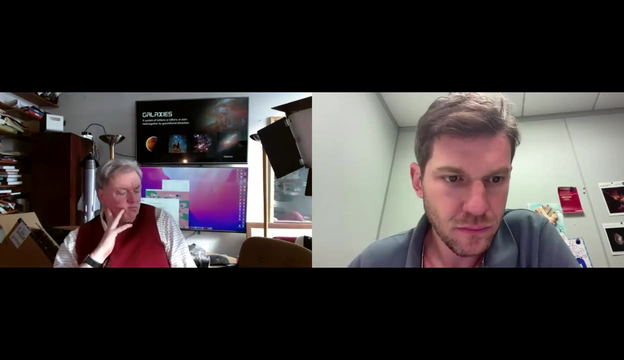 basically, instead of images, give 4ES samples, The images. anyway, for the convolutional network we use them as images, But for dense layers we flatten them. So we flatten them in one-dimensional array of 784 numbers. So you could certainly 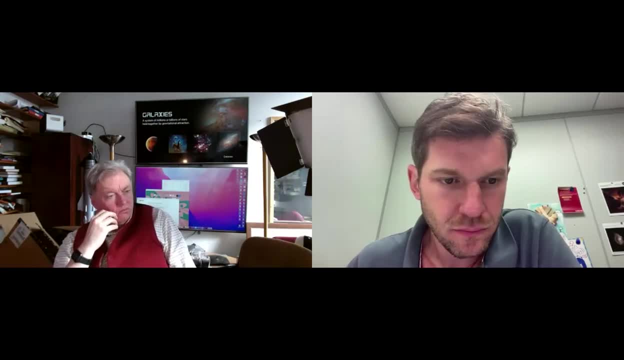 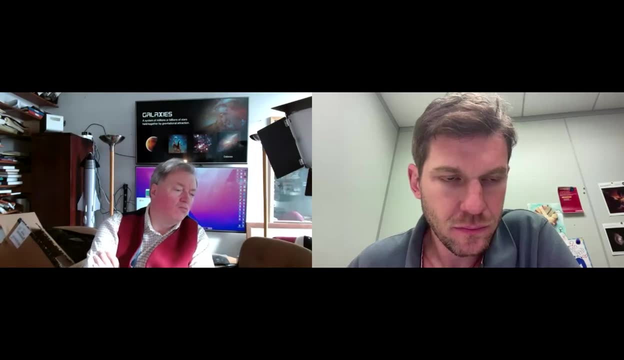 And you do Fourier transform beforehand if you want to. The neural net wouldn't care what your inputs are, as long as they're properly normalized. Usually it's a good idea just to normalize numbers between 0 and 1 to make it easier for the network. But other than that you could use 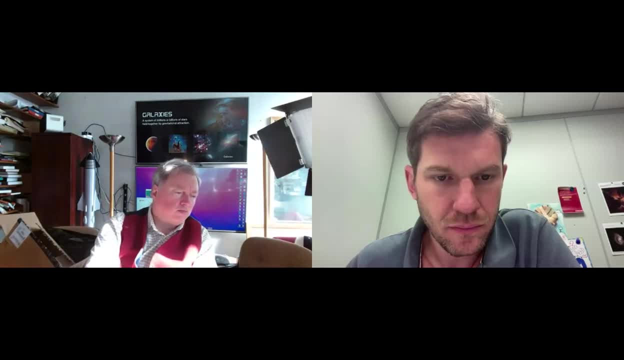 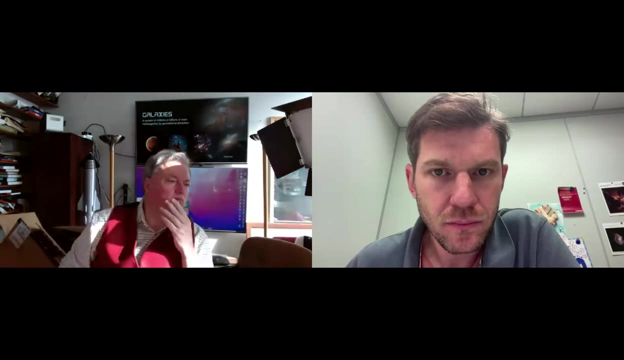 any set And there was a second. Apologies if this wasn't really answered. What is the proportion of anomalies to missed digits in the test data set? None. So for testing and for training we only use digits. There was no fashion, So fashions were. 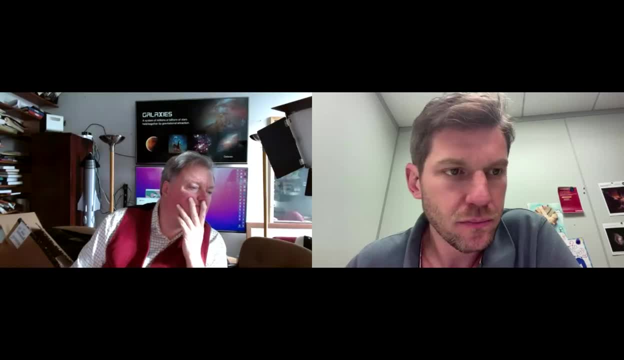 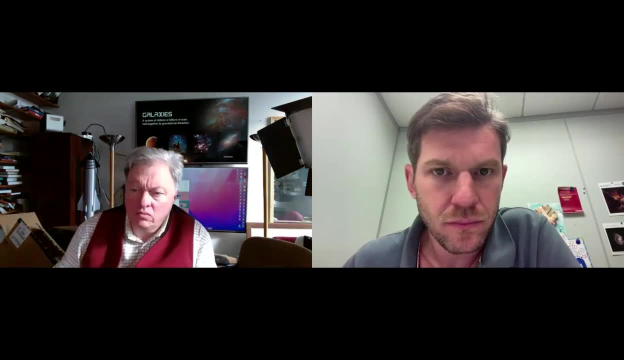 These two fashion things, the shoe and the sweater. the decoder never saw Encoder and decoder never saw. So we just train it on digits, data set, pure digits, no anomalies. And then we throw these two anomalies, But I bet you, if you throw a couple of these extra images in the training data, 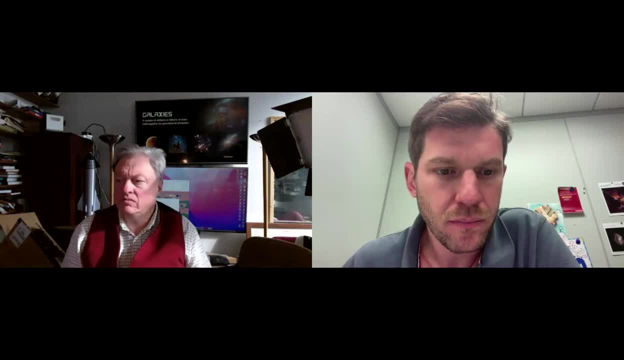 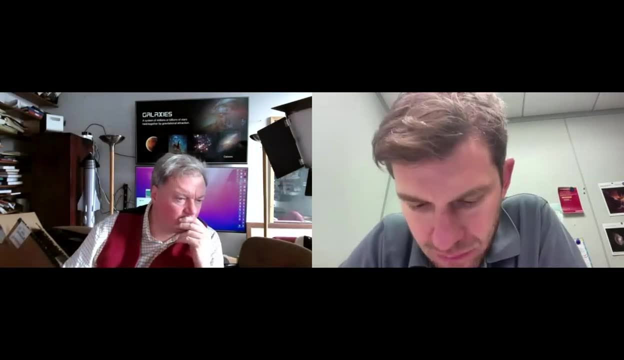 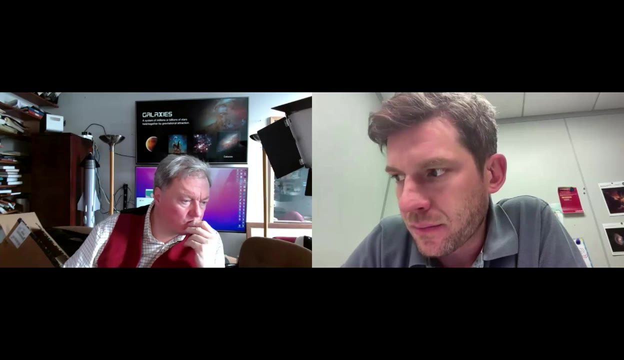 set, you won't be changing much, because that's exactly Why we could apply this on a sample with a large background but small amount of signal, Because the dimensionality reduction ensures that you pick only on the most important, most frequent features of your training data set, And having a very small proportion of the signal wouldn't mess. 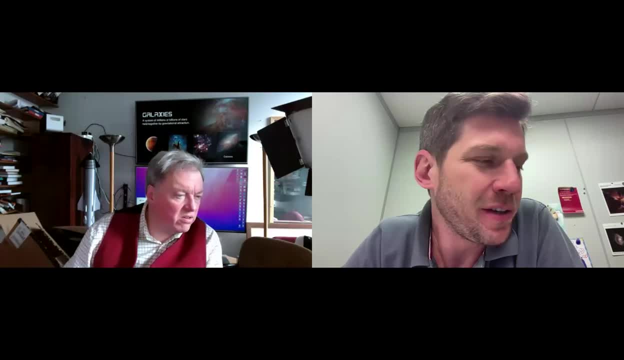 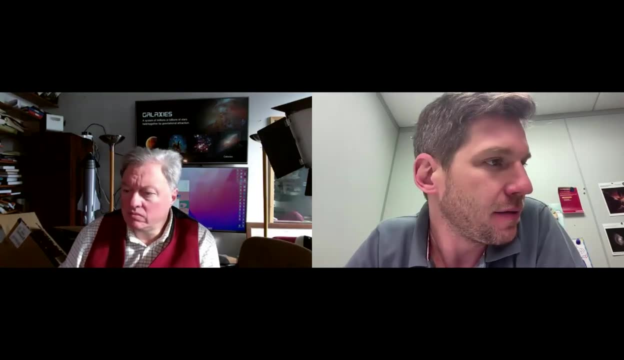 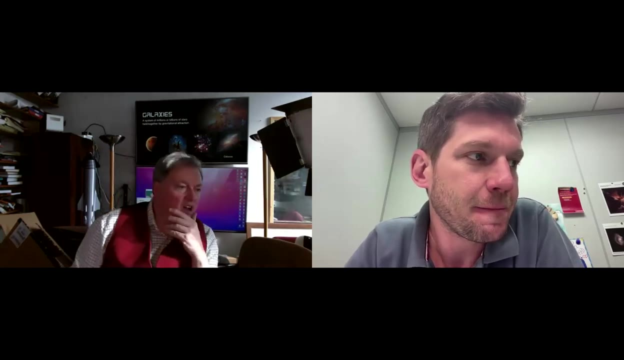 things up. That's why you reweight your signal in background when you do classification. You have relatively similar population, Right, Having a small fraction, it wouldn't matter. Okay, I think we should wrap up there. We're at the half hour. Thank you again, Lucas and Greg.